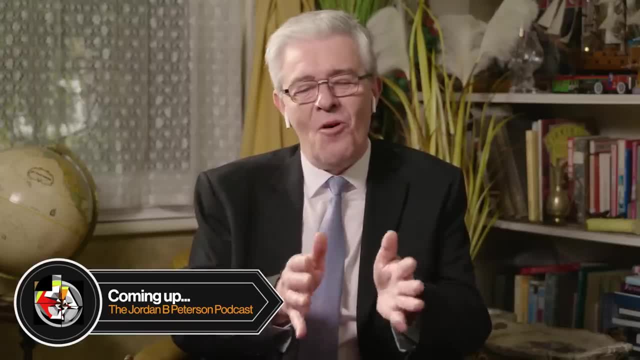 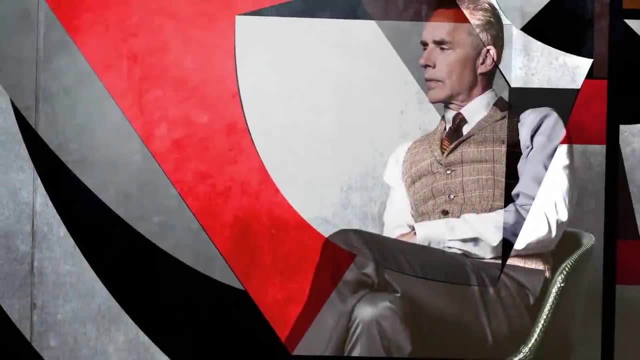 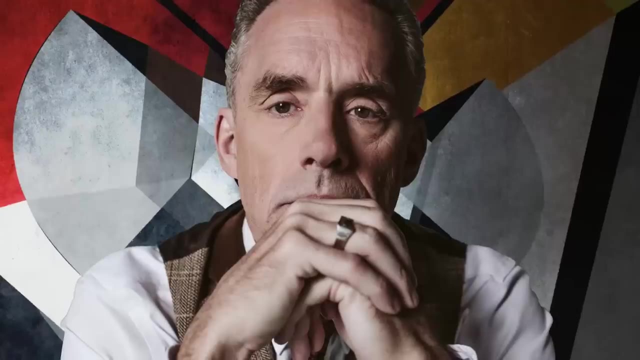 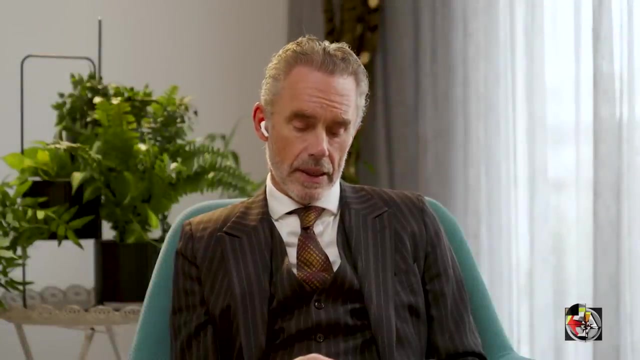 just is the uncertainty, And the closer you get, the more the less uncertain, And all the evidence suggests exactly as you say: it's dopamine. Hello everyone, Thank you for tuning in to watch and listen. I have the great privilege today of 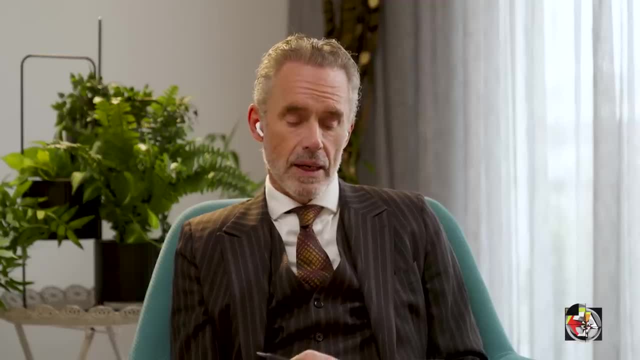 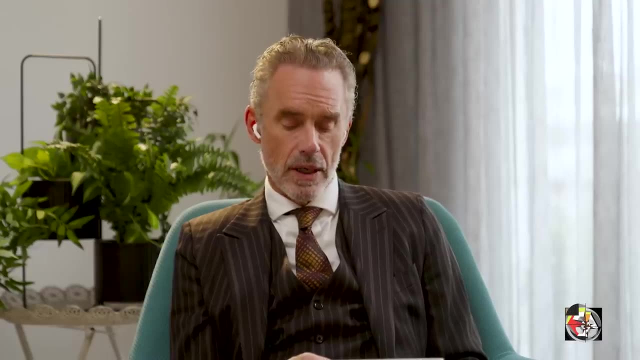 being able to talk with Dr Carl Friston In addition- let's say in a signal addition- to the recent conversation I had with Andrew Huberman. Dr Carl Friston is arguably the world's most renowned neuroscientist, a professor at 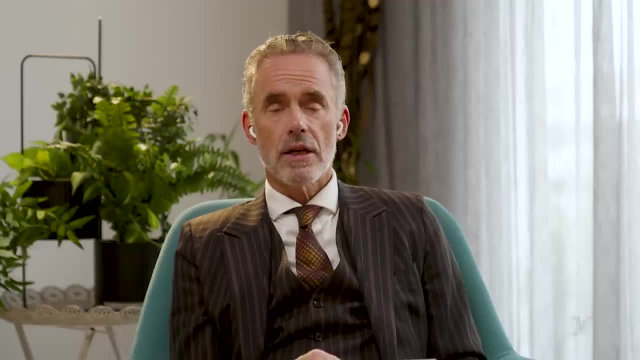 University College London. He is one of the world's leading authorities on brain imaging. 90% of the work published in fields employing such imaging relies on methods he pioneered. Dr Friston is also well known for his work on many of the topics of the book. 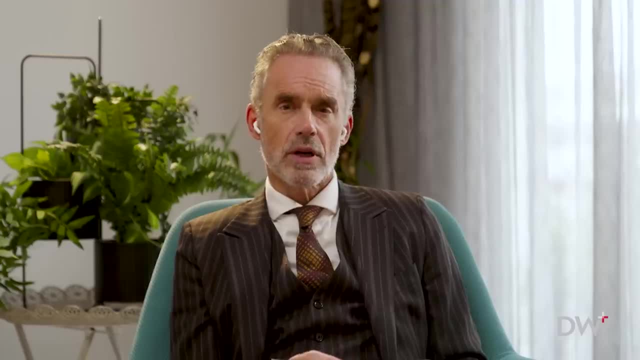 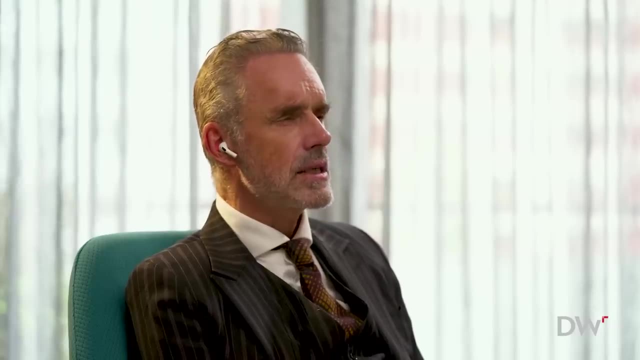 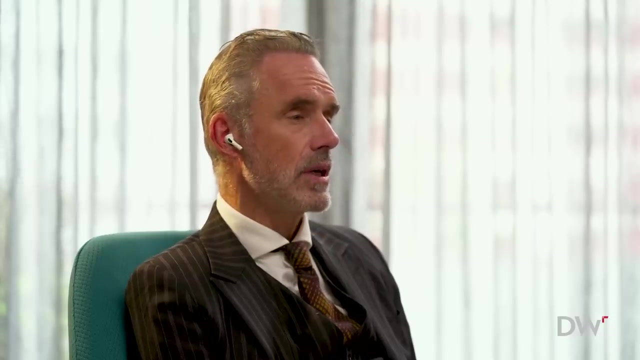 topics we will discuss today Work I find even more exciting, at least conceptually speaking, than his work on brain imaging. We will discuss the ideas that concepts and precepts, categories- that's another way of thinking about it- bind free energy or entropy, The idea of computation. 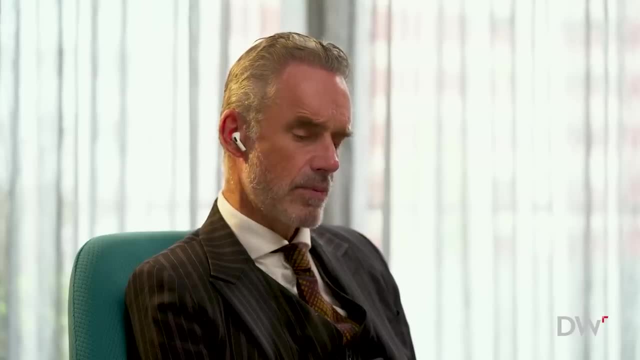 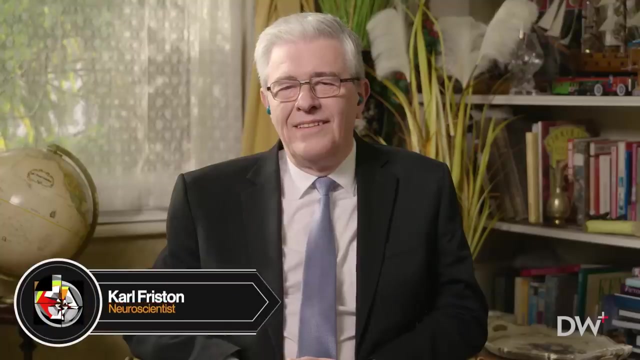 especially the kind of computation that approximates brain function as hierarchical, The theory of predictive coding, An act of inference. Welcome, Dr Friston. It's very good of you to agree to talk to me on this podcast. I'm really looking forward to it. That's a great pleasure to be here. Thank you. 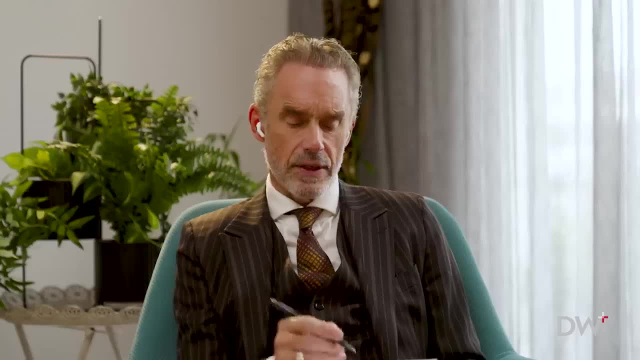 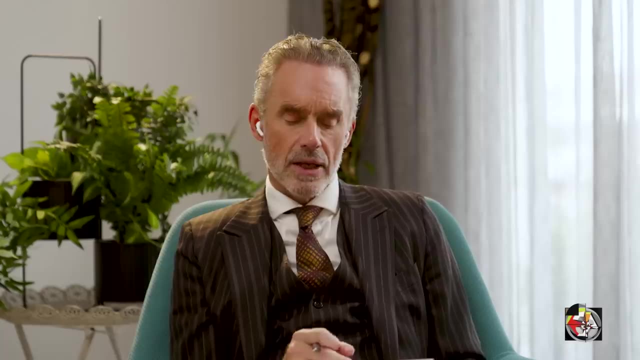 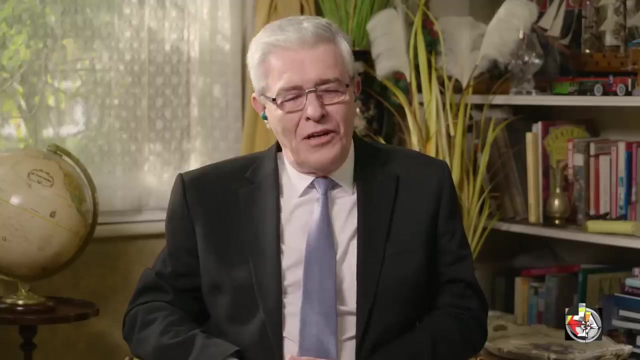 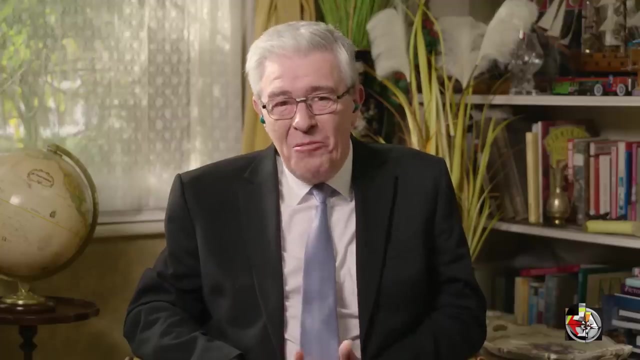 So let me start maybe by helping people understand this idea of hierarchical computation and the binding of entropy, And so if you could walk through that briefly, then I'll ask some questions, if that seems appropriate. Yeah, sure, So the binding of free energy and entropy, that sounds delightfully Freudian And I don't mean. 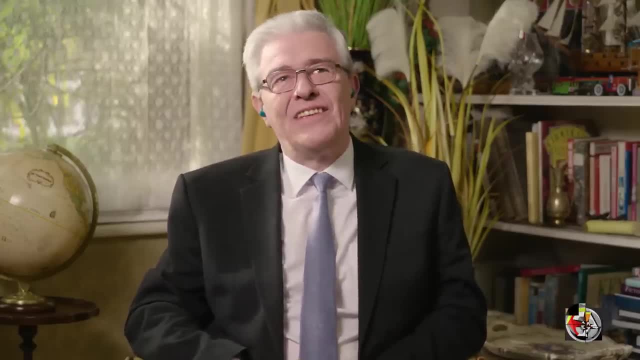 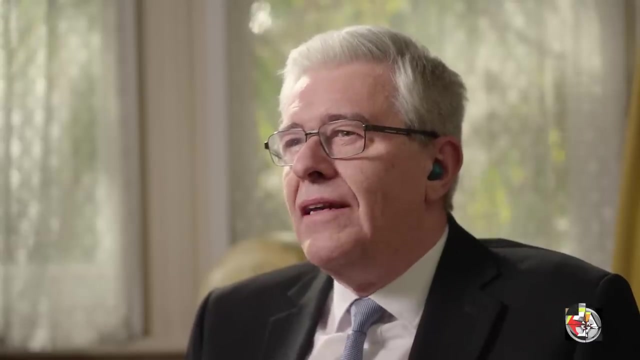 that in a sort of disparaging sense. I think that some of the truisms and the insights of that era have now proved themselves in modern formulations of computation, information processing, sense-making in the brain, And one nice link there is to think of free energy as surprise. 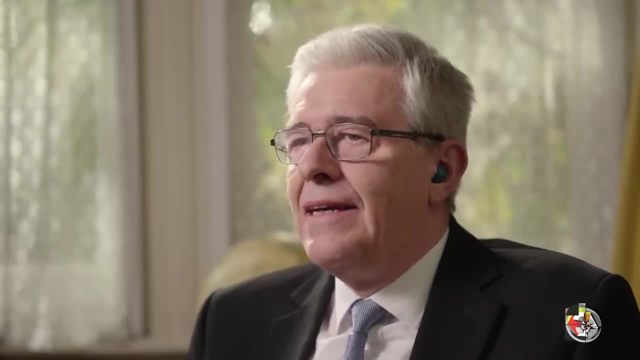 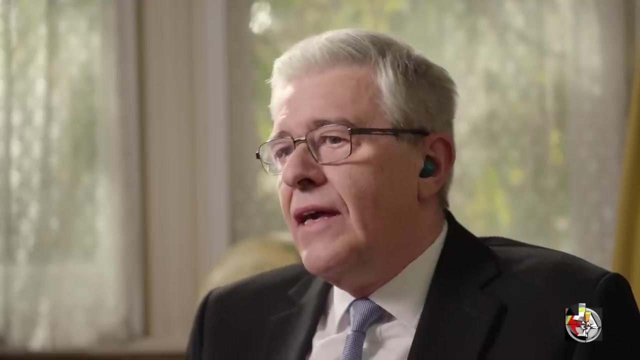 So one way of looking at the way that we make sense of our world, bringing explanations, concepts, categories, notions to the table that provide the best explanation for the myriad of sensations to which we are exposed, is to see that process as a process of minimizing surprise. 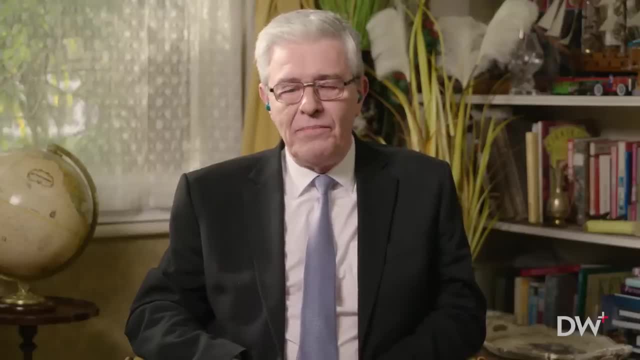 So binding free energy. I think can be read very simply as minimizing surprise. But of course, to be surprised you have to know that there are a number of things that are going to be. to have something you predicted, you have to have a violation of predictions, so immediately you're. 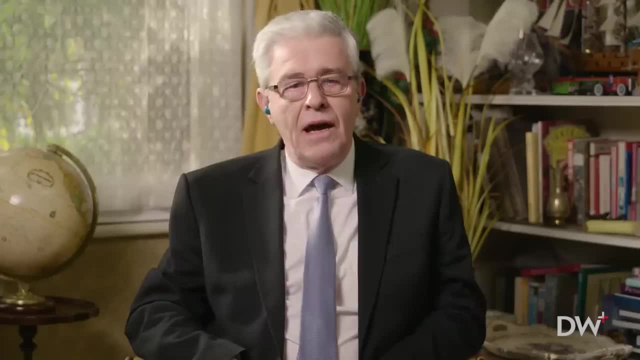 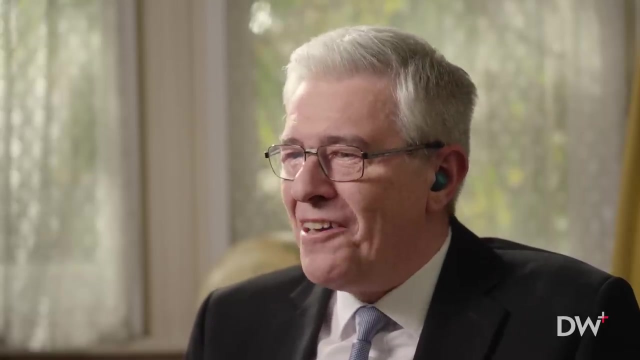 in the game now of predictive processing- predicting what would i see if the world out there was like this, and then using the ensuing prediction errors to adjust your beliefs and update your beliefs in the service of minimizing those prediction errors, or minimizing that surprise, or minimizing, minimizing that free energy. and you artfully introduced the notion of hierarchy. 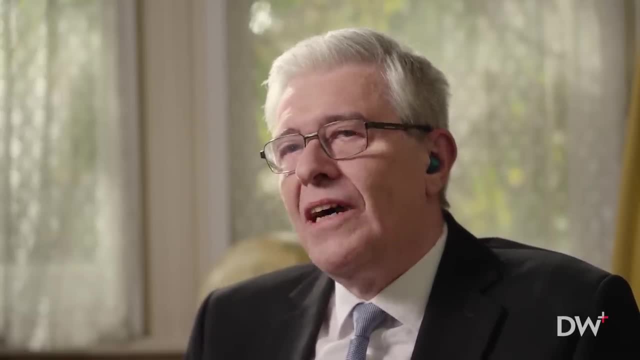 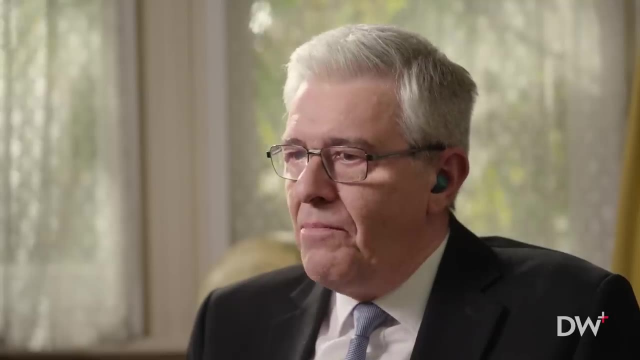 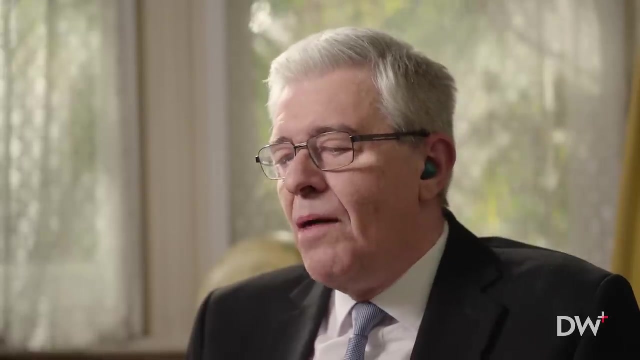 in that question- which i think speaks to another fundamental point, that in making sense of the world, in making those good predictions, we have to have an internal model, sometimes called a world model, a model that can generate what i would have seen if this was the state of affairs out there. 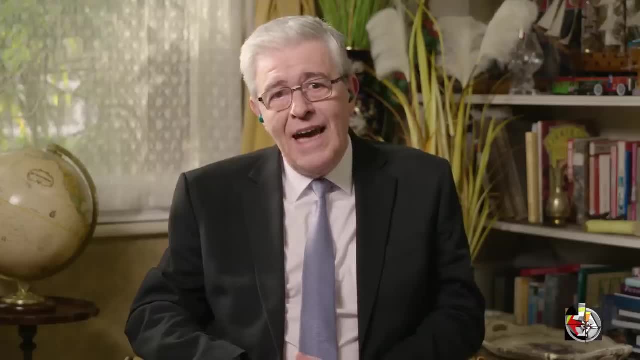 and that notion of a generative model i think is quite key and holds the attribute of hierarchy simply in the sense that we live in a deeply structured world, very dynamic world, a world composed largely of creatures like ourselves that has this sort of hierarchical nested structure that has to be part. 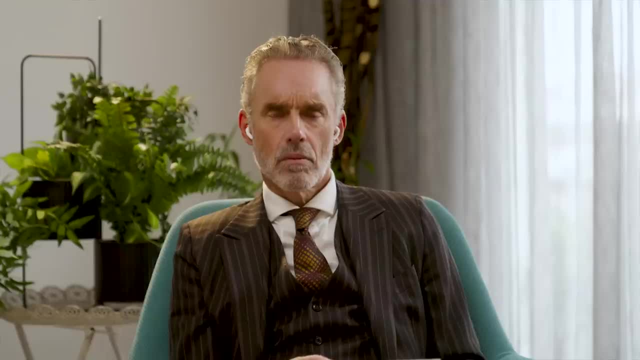 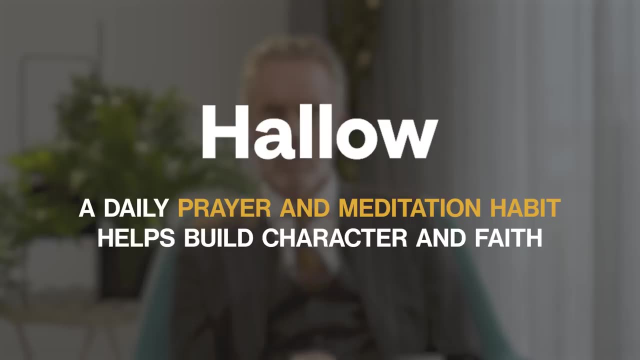 of the models that we bring to the table. to understand it, post-modernism is tearing our world apart. the one thing that may be able to unite us is a mass return to our judeo-christian roots. at the individual level, that means developing our 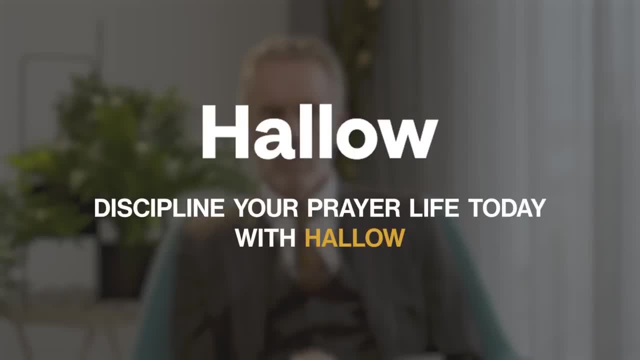 prayer life. there's a ton of literature out there on the benefits of secular new age mindfulness meditation, but what isn't talked about nearly enough is the power of a consistent prayer life. that's where hallow comes into play. hallow is the number one christian prayer app in the us. 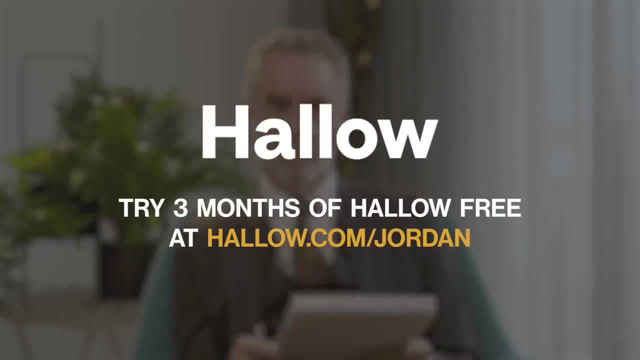 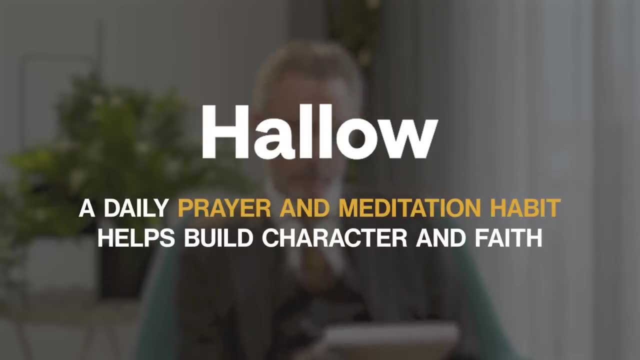 and the number one catholic app in the world. hallow features over 5 000 prayers and meditations, including daily prayers to help you build a habit of prayer and gratitude. bible reflection with jeff cavins and father mike schmitz to help you grow in knowledge and understanding. 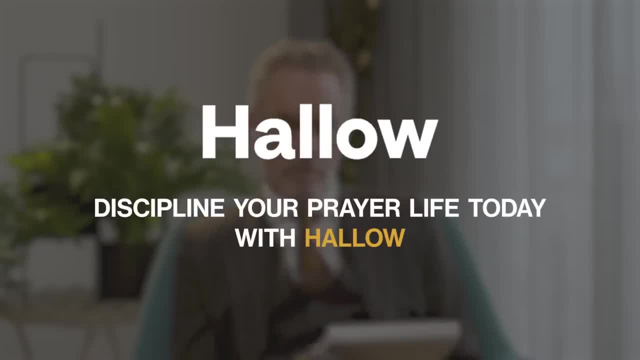 meditations to help you prepare for sleep and rest each day, reflections with bishop baron and much more. use hallow as a foundational tool to grow in gratitude and character each and every day. try it free for three months by going to hallowcom. slash jordan, that's hallowcom. 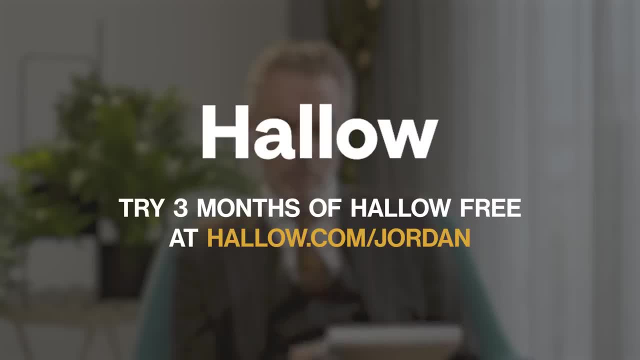 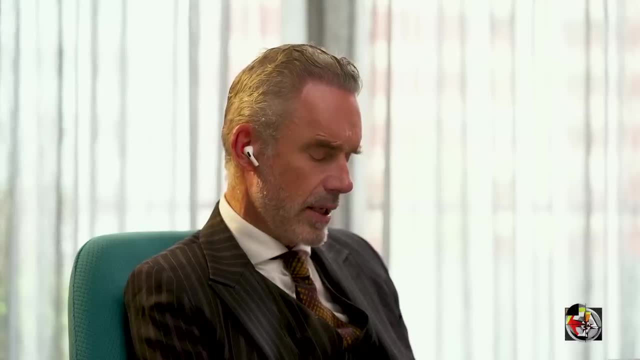 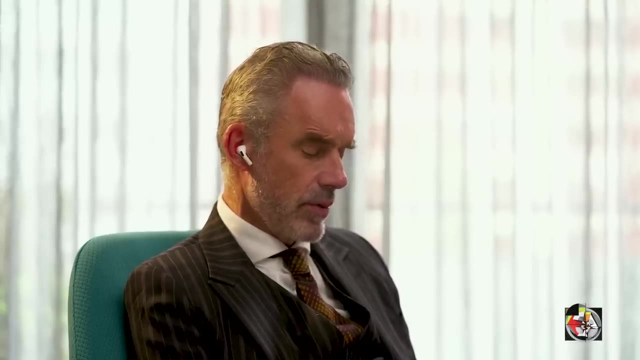 slash jordan. ground yourself in fundamental truths with hallow today. okay, so i encountered these ideas, i would say, first reading a book back in 1982 by a man named jeffrey gray, who was influenced by norbert weiner and by general cybernetic theory, and he regarded the hippocampus as, at least as part of the 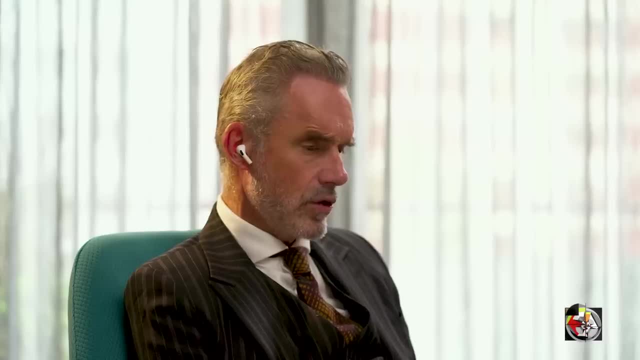 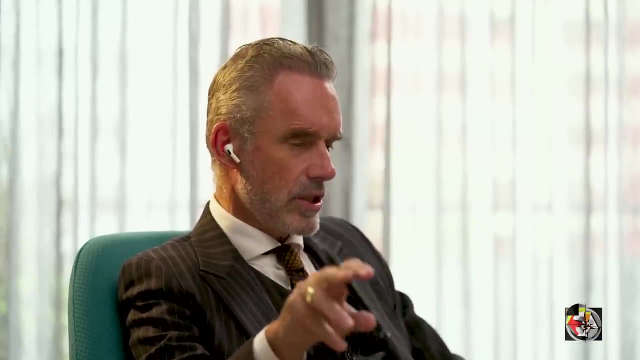 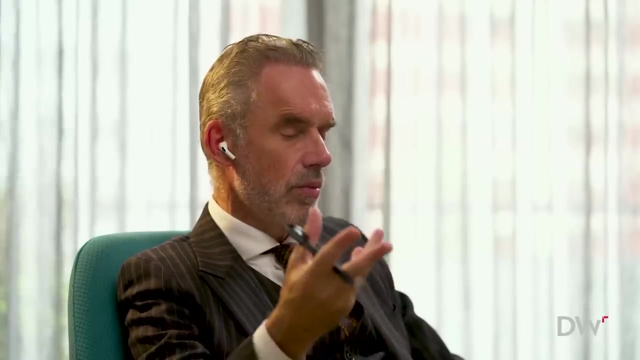 central part of the brain involved in contrasting expectation, let's say the way you expect the world to lay itself out with the way the world is actually laying itself out, indicating that surprise was a uh. what was the prodroma to anxiety and that anxiety, in some sense, was an indicator of the magnitude between 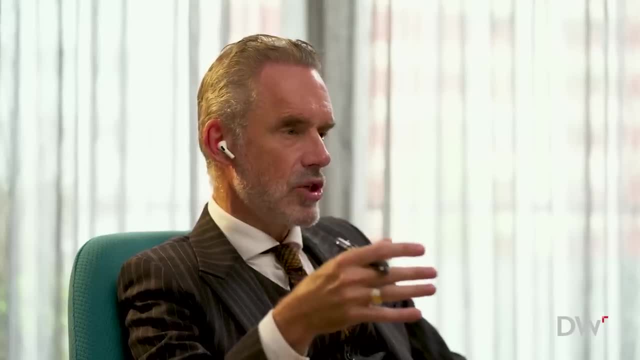 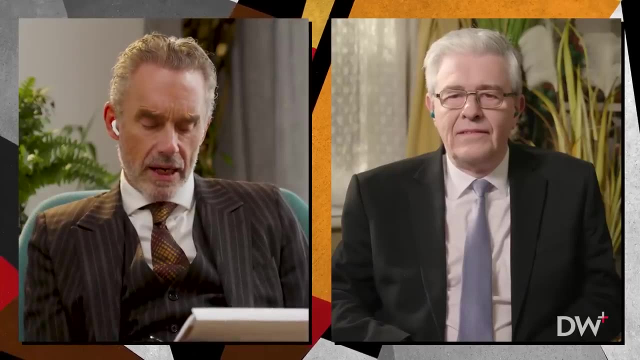 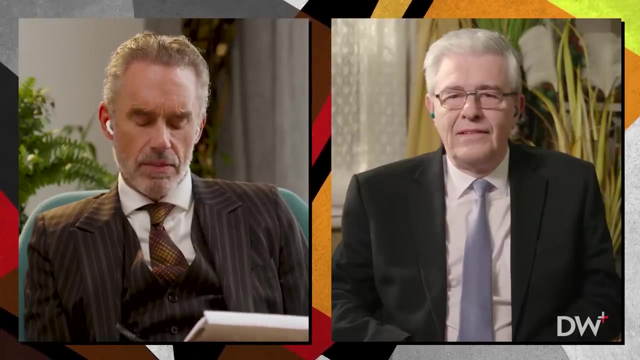 the magnitude of mismatch between expectation and reality. so i i want to ask you a couple of questions about that, because i thought a lot about gray and i i thought about gray for like 40 years after reading his book and also as a consequence of encountering your ideas much later. um, the 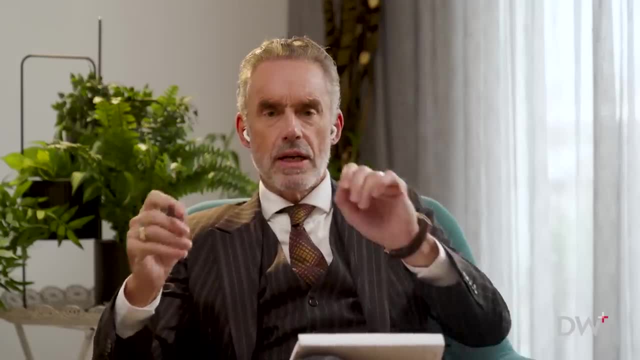 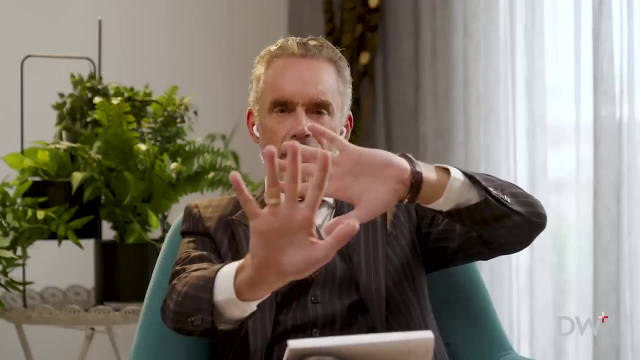 the cybernetic model of expectation is predicated on the idea that you lay an expectation on the world and the expectation is a model, and then you have incoming sensory data and the sensory data is the world, and that now and then there's a mismatch between the sensory data. 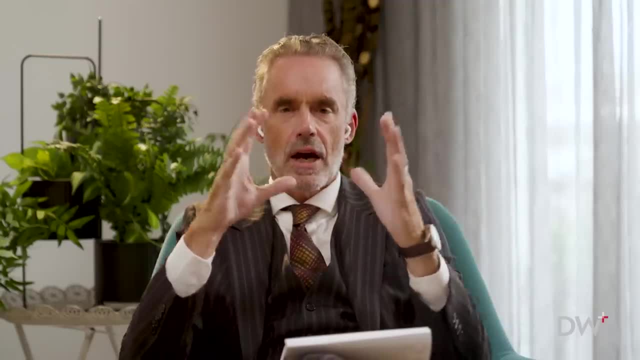 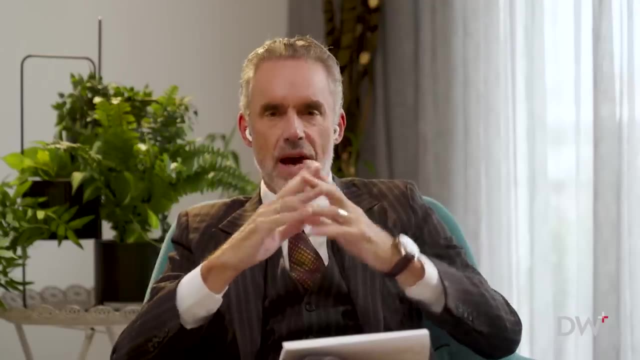 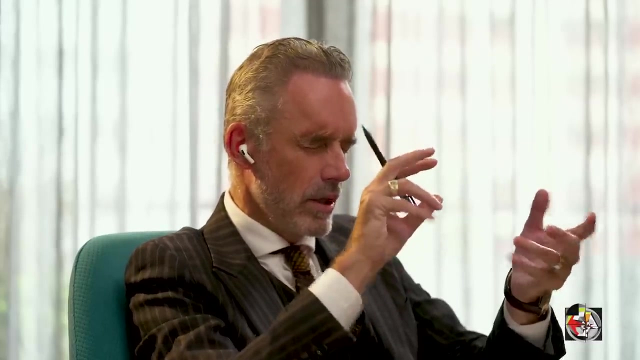 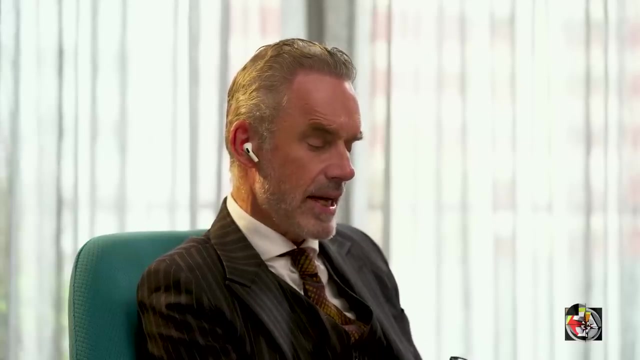 and the expectation, and then you have to modify either the representation or the action pattern to reduce that, that mismatch. but then i thought, well, wait a second, there's a. there's a weird, there's a weird lack in that formula. it's twofold number one. it isn't obvious to me that it's expectation. 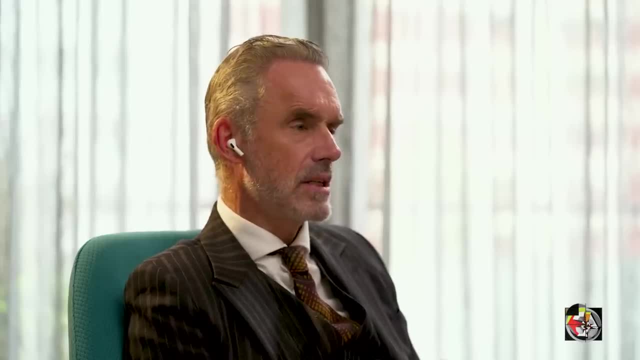 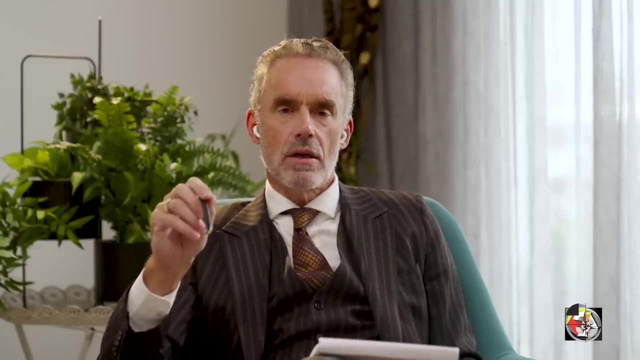 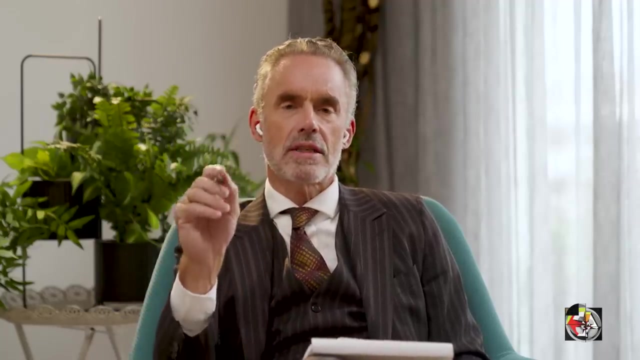 it seems to me that it's more likely to be desire, and that's a useful transformation of conceptualization, because if you use the word desire rather than the word expectation, you can infer that the models that are being contrasted against the real world are models of motivation rather than cold cognitive computation. 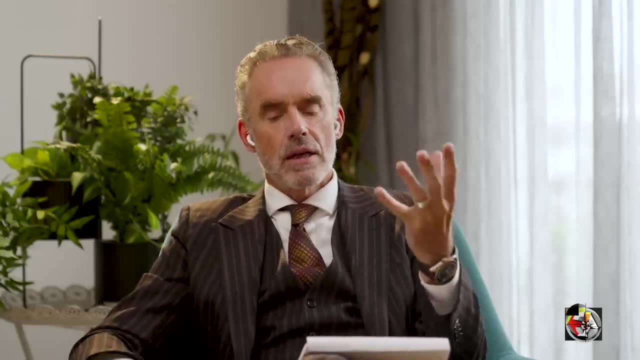 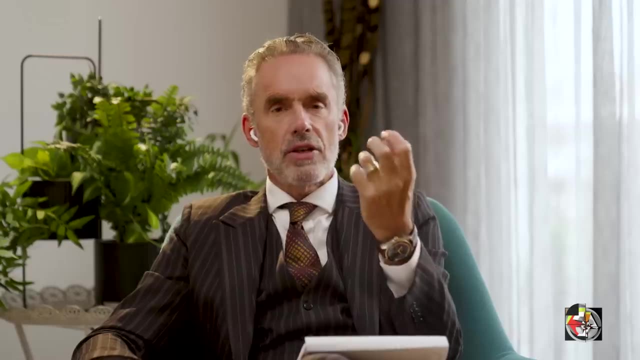 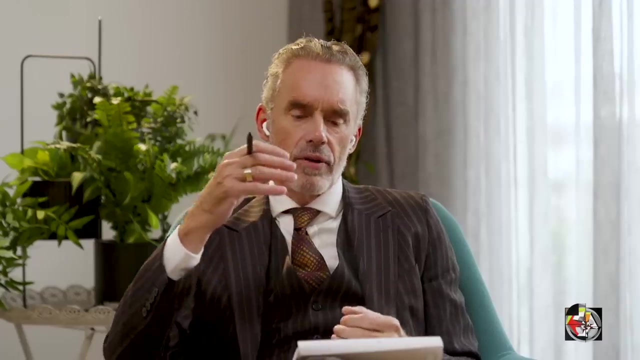 and so, for example, if i'm interacting with a woman who i'm romantically interesting, interested in, i'm attempting to bring about the realization of my desire, not my expectation, and what i'm, and that's under the pressure, let's say, of, of, of uh, of the of the demand for sexual. 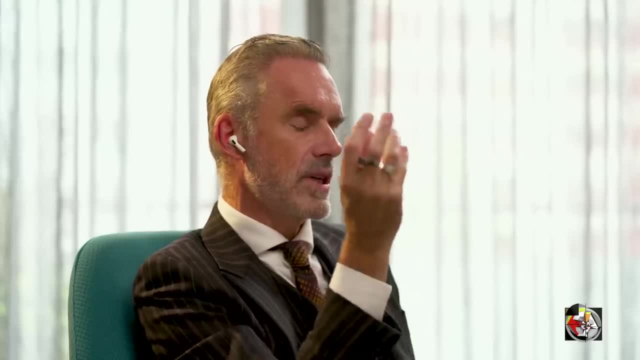 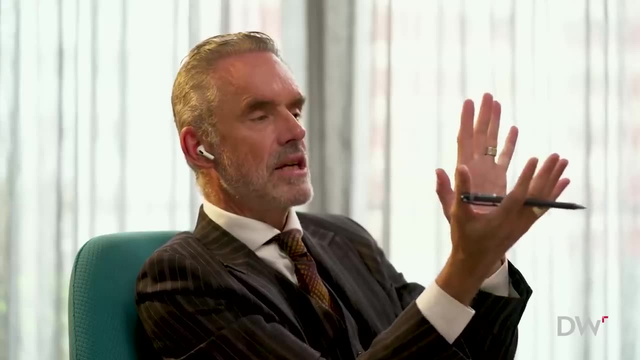 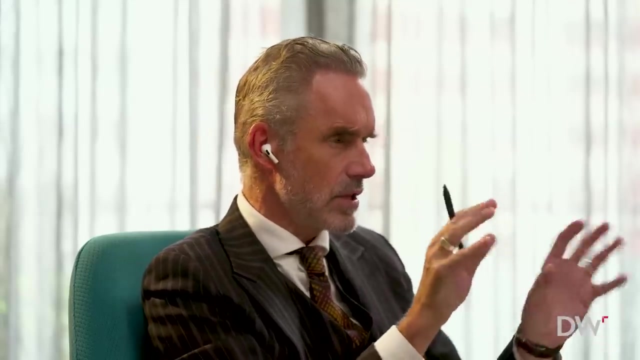 reproduction, and so the motivational state grips the desire. the desire manifests itself as a fantasy, and then the the motivation is the minimization of the discrepancy between the actual world and the fantasy. and then so it's not exactly an expectation, because it's more dynamic and alive. and then one more: uh, i hate. 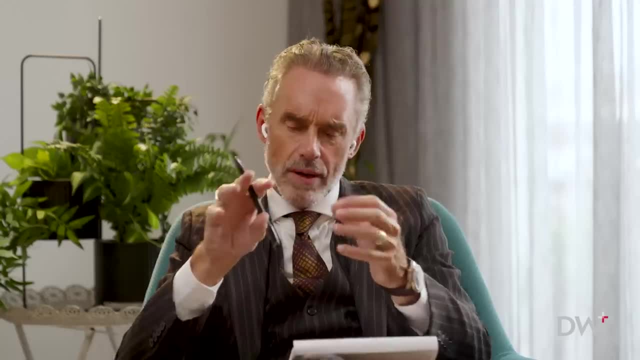 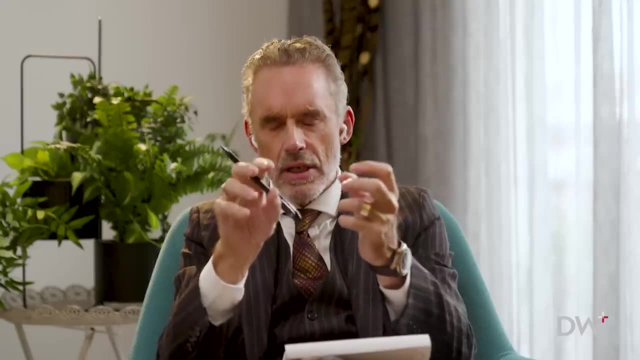 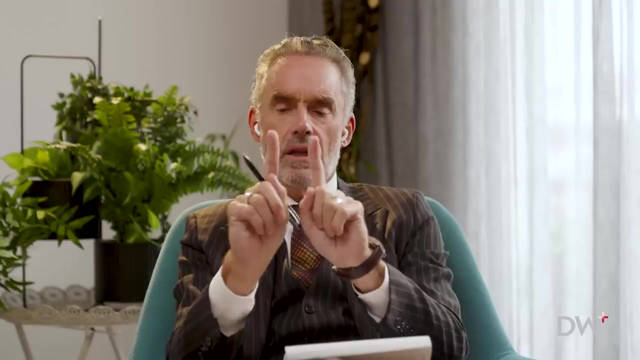 to hammer you with all of this right at the beginning. but one more issue on that front is, uh, the error, because you could imagine, and i'm interested in how this matches your hierarchical concept, if i make a mistake, such that i don't minimize the relationship between what's happening and my fantasy. 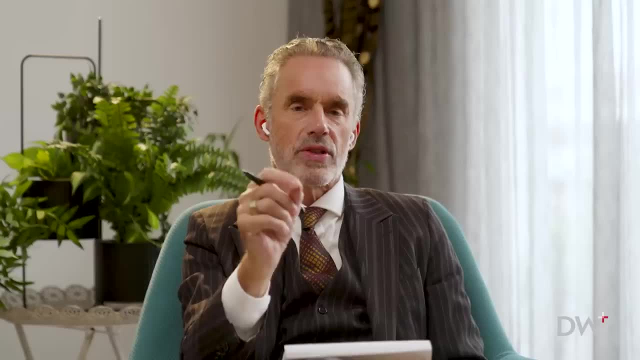 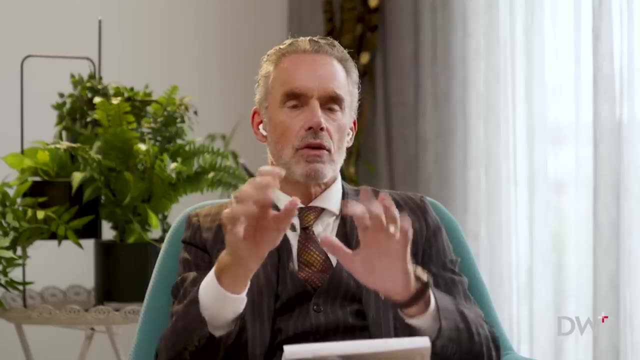 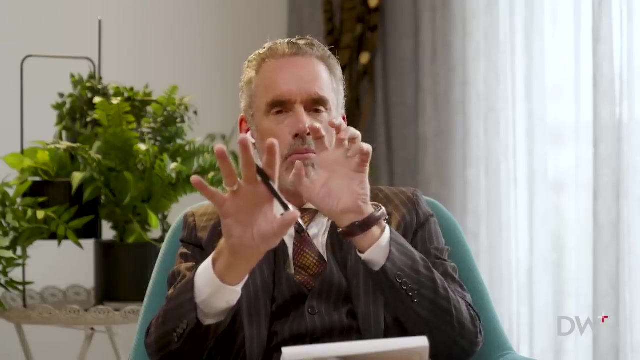 one of the mistakes i might make is a mistake of perception, not expectation or desire, because i might be seeing the situation wrong, and so it seems to me that it's more realistic to say that what you're doing is minimizing the mismatch between a model of what's happening, not this. 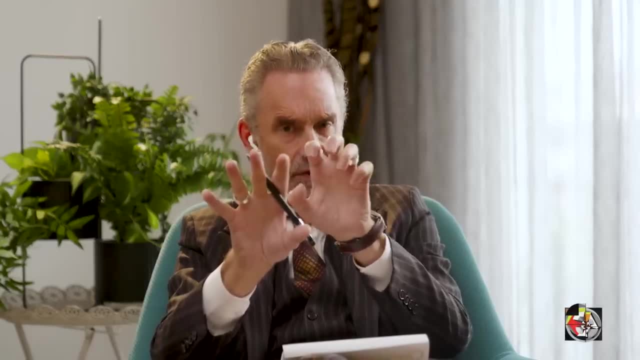 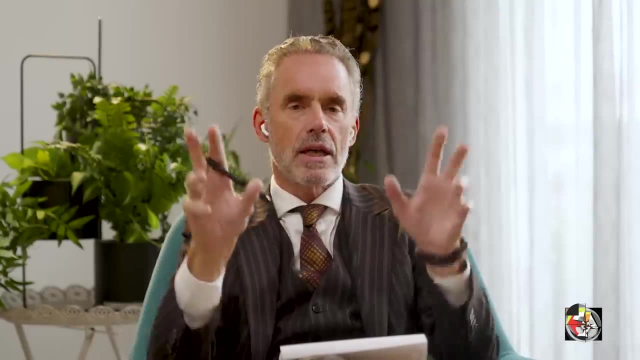 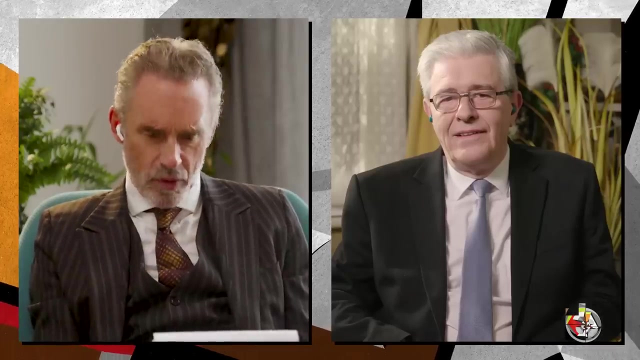 not sensory data itself, but a model of the, of the print, of the model of what's happening, the unfolding present, contrasted with a fantasy, and that the mismatch is what indicates surprise or and or entropy. now i know that's a lot of questions to answer at the same. 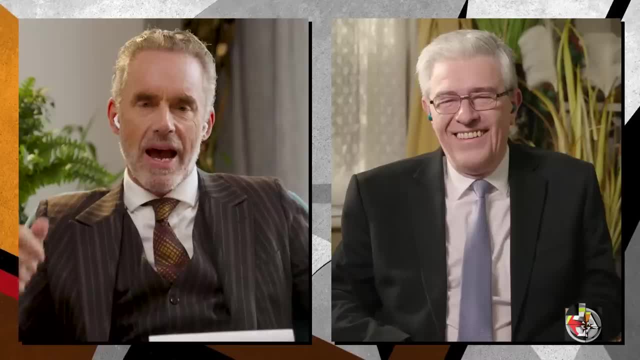 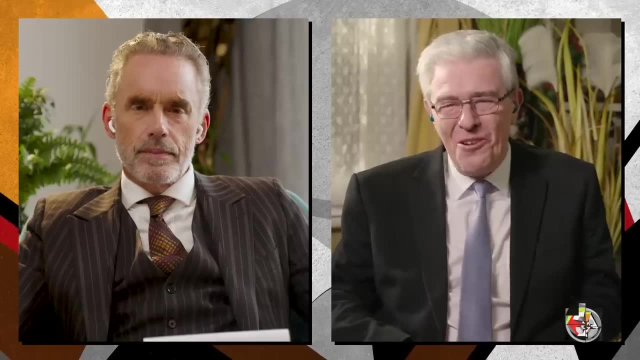 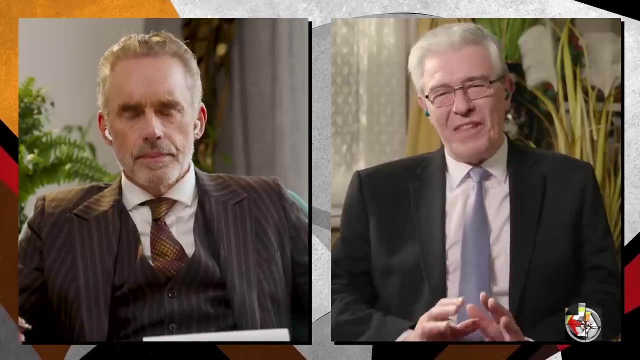 time. but that whole set of objections makes up a pattern. it does, and despite the fact you introduced a whole bunch of really important concepts there, i think it was nicely introduced and, you know, in a coherent way. so i'm just trying to remember all the exciting things you've brought to the 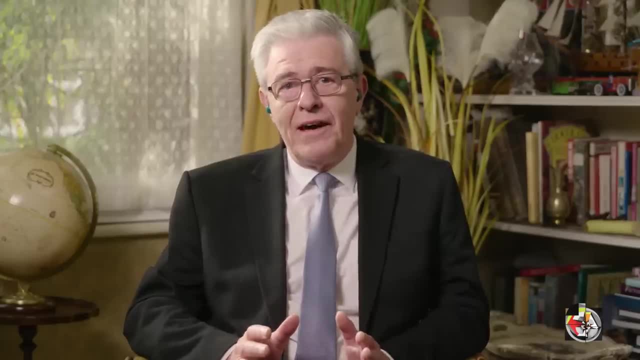 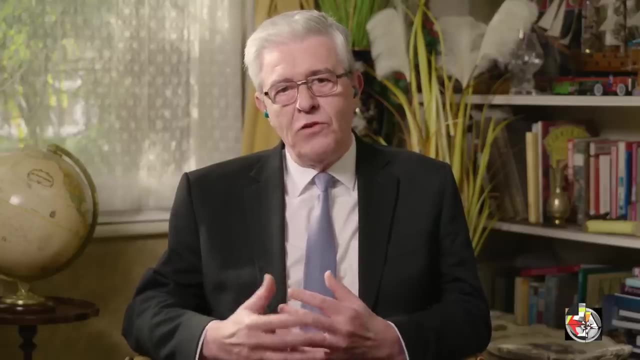 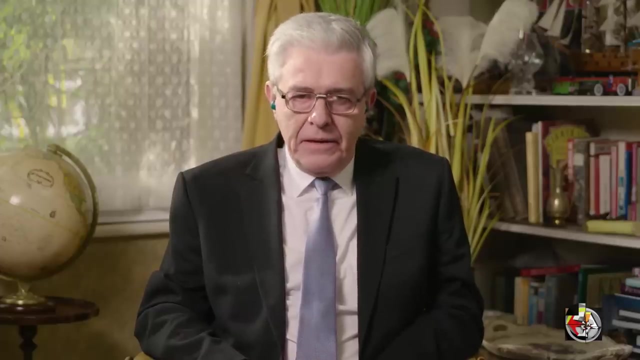 table. um, so yeah, jeffrey gray, a great thinker, um, in my um memory, sort of um, famed for understanding latent inhibition and sort of you know how you use these surprise or these mismatches or these um, these, uh, prediction errors, and it's interesting that you know you speak to his 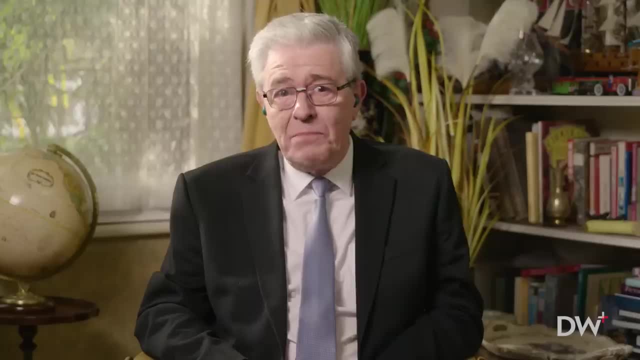 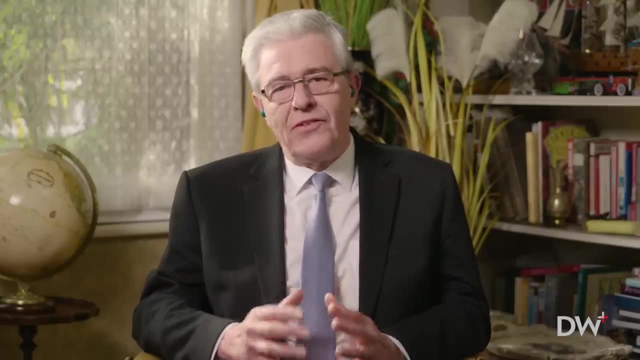 conceptual roots in cybernetics, because there's a very, very close connection between the things you're talking about and, uh, the early formulations of cybernetics by people like ross ashby. so there's this good regulator theory which i think you know. if, if your, your listeners don't know about, i think 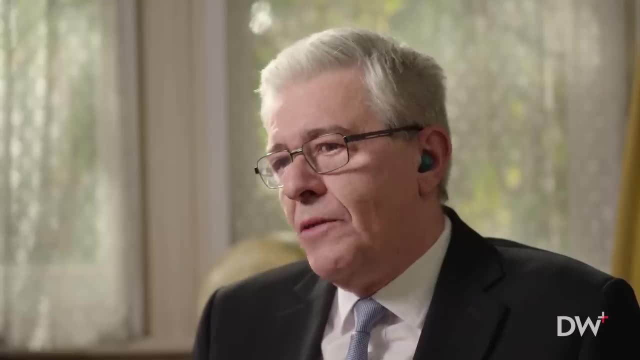 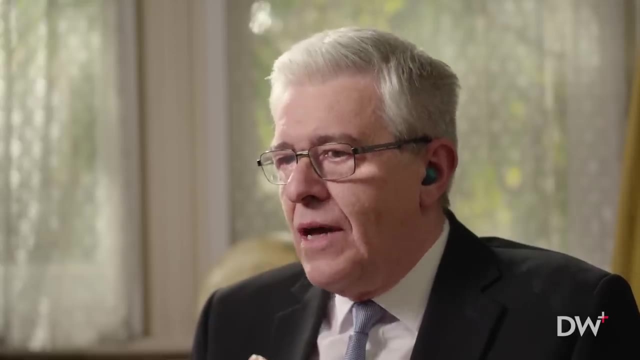 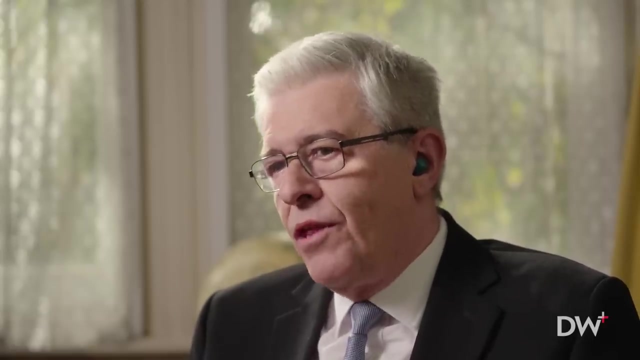 they'd like. i think you know you would like a lot. it's just the notion, and provable notion, that to control an environment you have to have a model of that environment to you know, to be able to couple with, to engage with the environment, the degree of the environment that you're talking about. 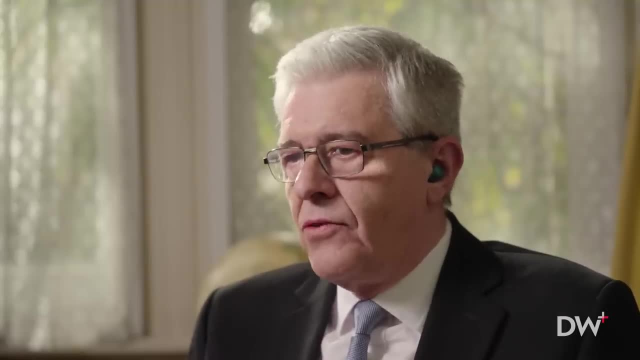 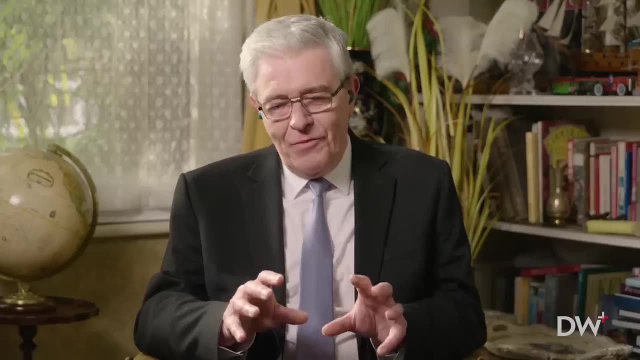 the degrees of freedom of your model have to match those of the kind of environment in which you are, in which you're operating. so i think it's a a deep connection there. the other thing, well, many things you brought you. you uh mentioned that you use the word fantasies a lot, and i think that's quite 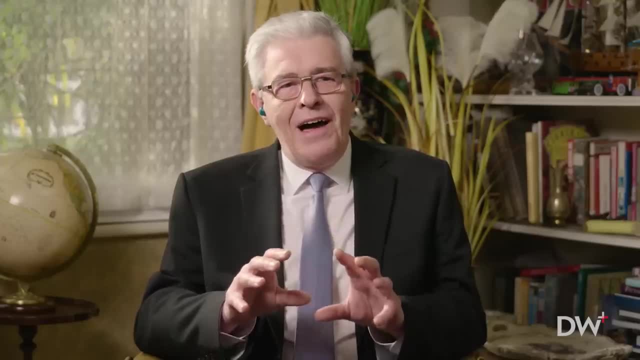 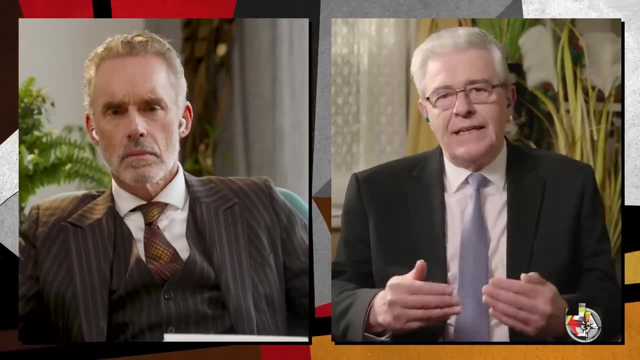 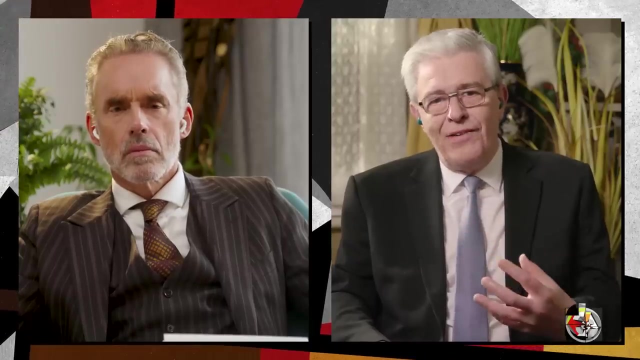 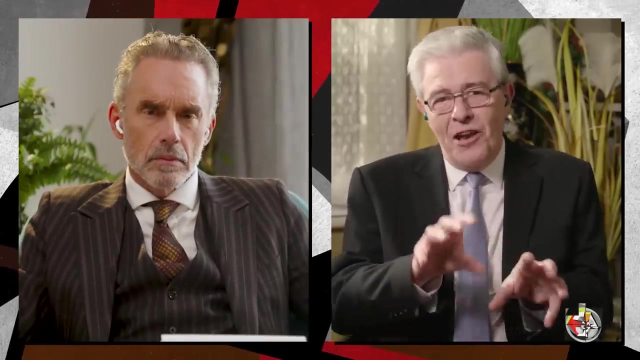 important because very often, um, i sell the brain as a fantastic organ, literally because it is in the game of generating the right kind of fantasies. and these are the fantasies, these are the motivated expectations that drive our behavior. but in noting that, in noting that you've also made a big move and an important move. i know it's a move, you know you. 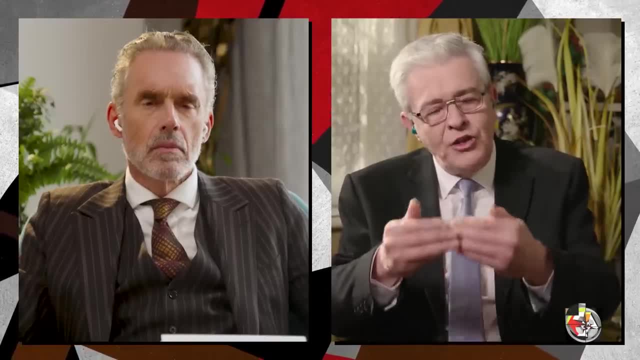 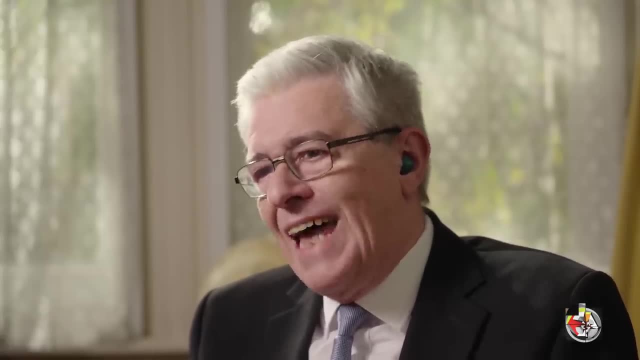 want to make in terms of our conversation, but just to contextualize why that is such an important move. you're talking about motivation. you know how our perception and action are all contextualized by motivation and what we desire and what we want to achieve, and what we want to achieve and what we. 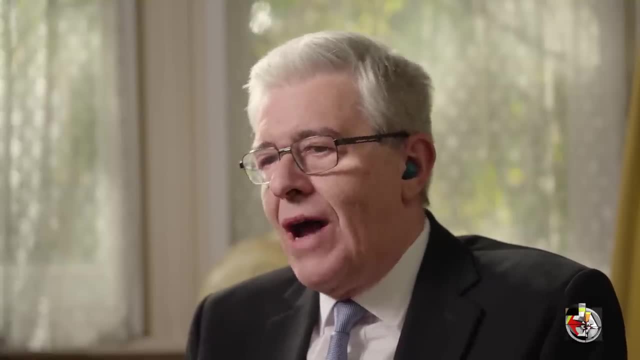 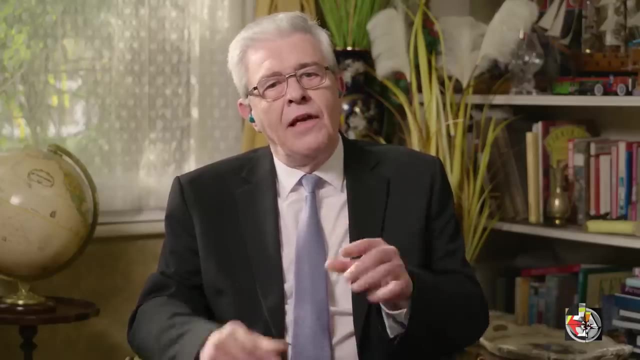 want and what the preferred outcomes of our, of our acts that's, i think. i think sort of the cracks and we'll probably be the focus of much of what we're going to be talking about. but just to say that vanilla predictive processing and vanilla predictive coding does not deal with that. it just 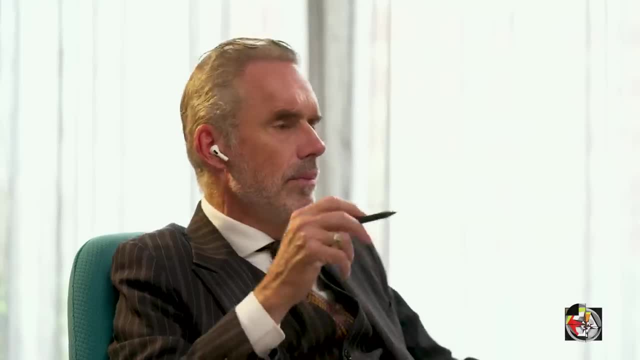 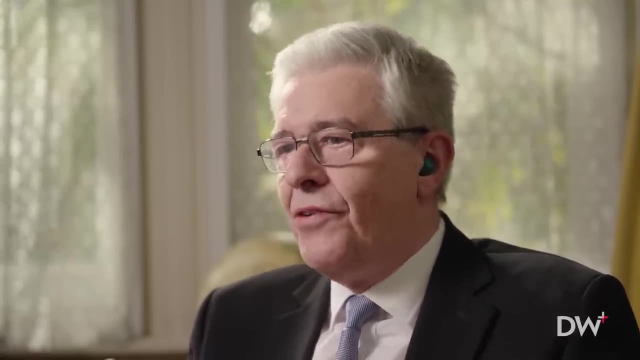 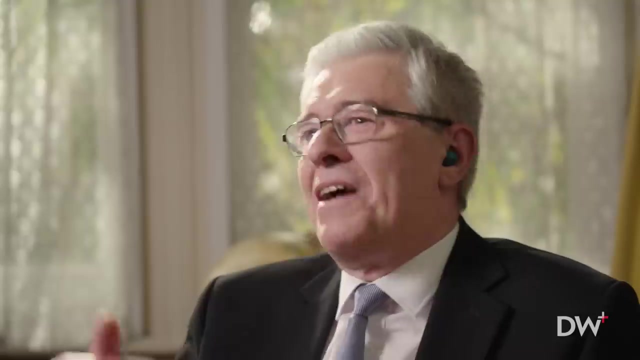 deals with sense making, so it's usually in the moment. as soon as you bring decisions and choices and actions to the table, you're immediately in the game now of making influences about the future, the future that has yet to be observed. so there are no prediction errors, it's just your expected surprise, your expected. 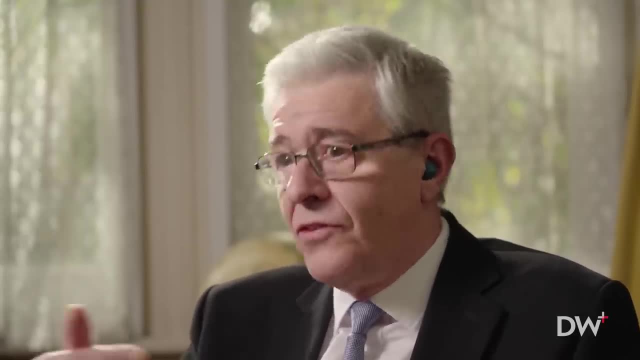 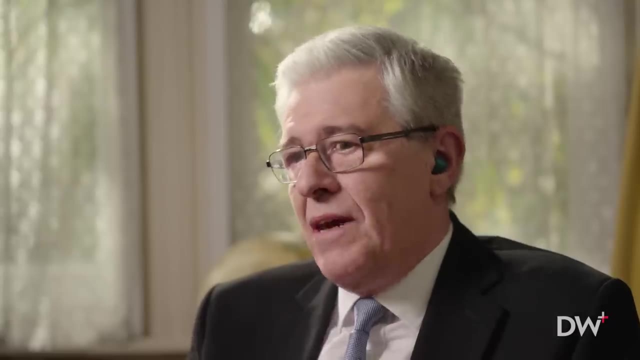 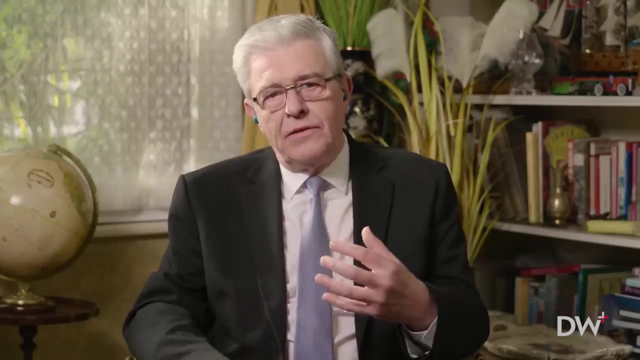 entropy or expected free energy, or your expected discrepancies between what you fantasize should happen, what you prefer to happen and what you anticipate given your best sense making at the moment. so i think that inactive aspect that that choice really does profoundly, you know, change the and takes us from simple sense making into the world of choice. 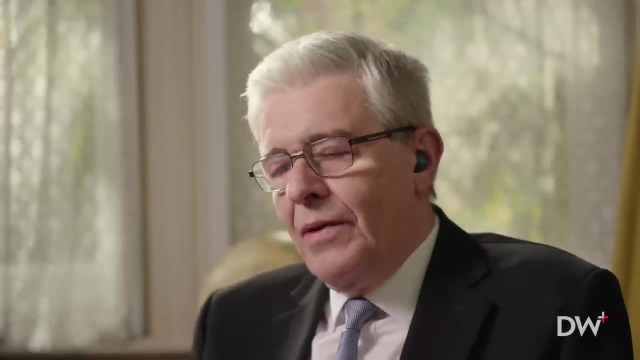 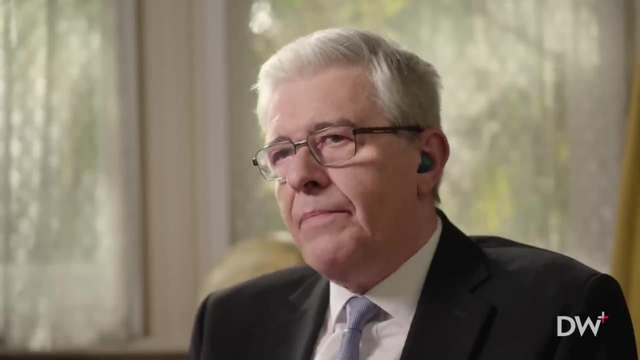 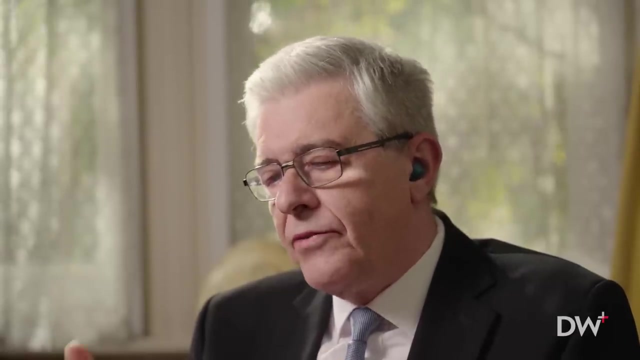 and decision making and motivation. so, um, mathematically, the way that i would um articulate that, as as a physicist, would be okay. if we're in the game of minimizing surprise and this mismatch, this discrepancy that you were describing in the moment, then presumably i will now choose the. 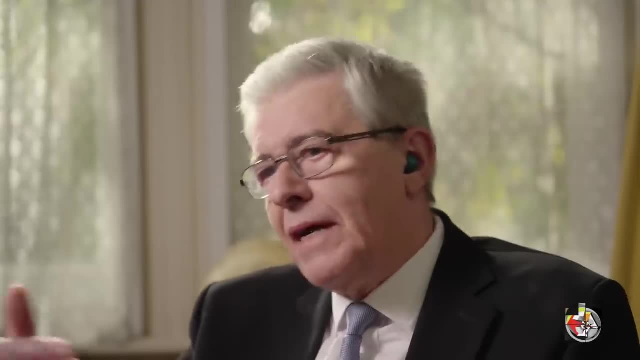 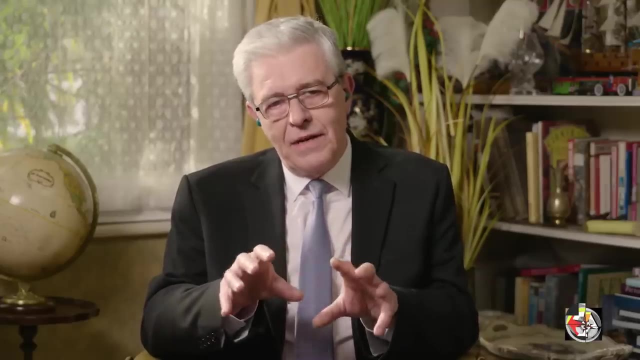 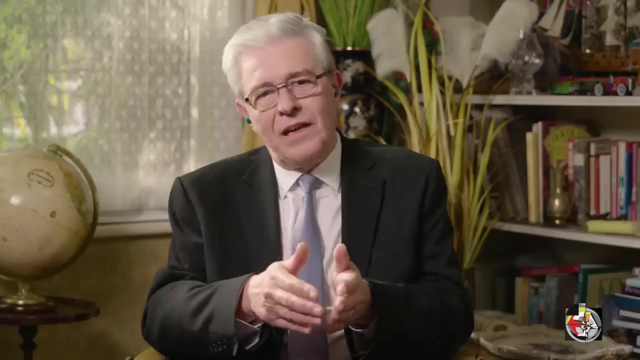 things that i do in order to minimize the expected surprise in the future. and the nice thing about articulating it like that is that the expected surprise mathematically is just entropy. so entropy, uncertainty- and i'm using entropy and uncertainty synonymously here they are the mathematical 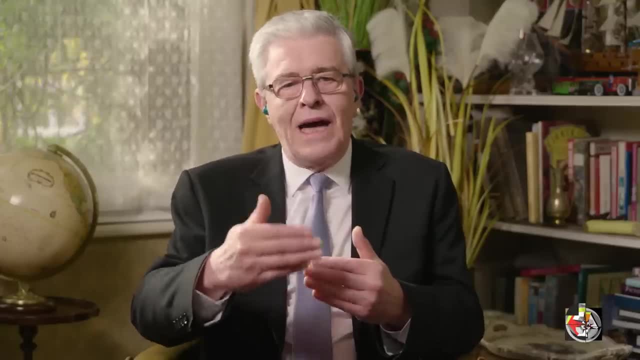 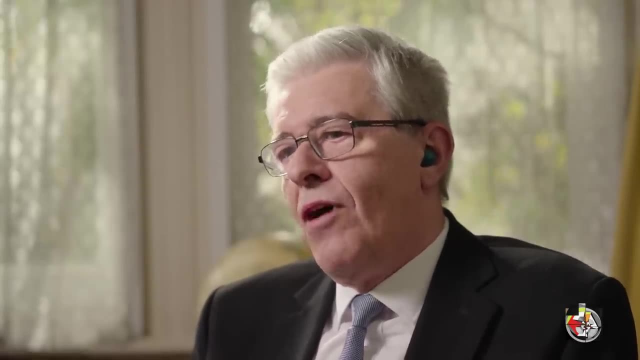 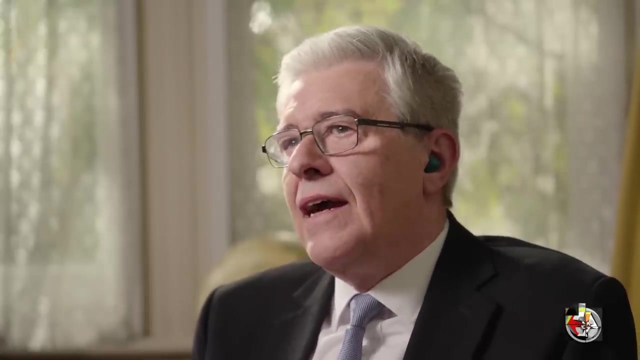 statement of the surprise i expect when i haven't actually seen the outcome yet. so in many senses, what you can say is that we are motivated to resolve our uncertainty and that can be sort of, if you like, carved into two ways of minimizing uncertainty. it can either be through choosing those behaviors that resolve. 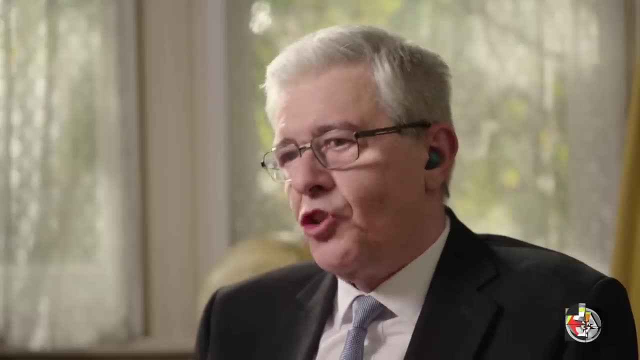 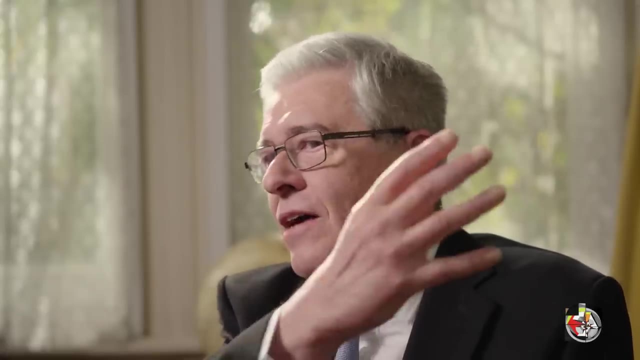 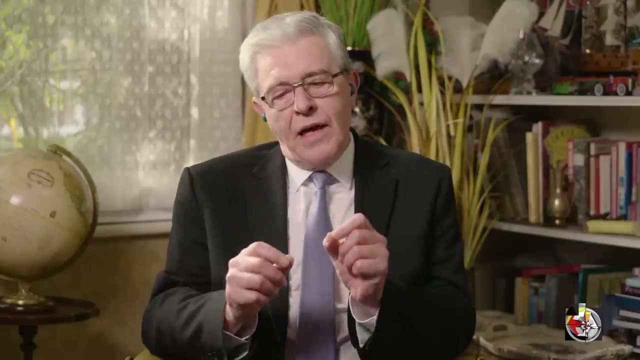 uncertainty in the sort of folk psychological sense you know, watching the news, looking over there to see whether you know my fantasies about the cause of that's, that visual flatter in the periphery of my vision was what i thought it was. was it a bird or a butterfly? but i think there's 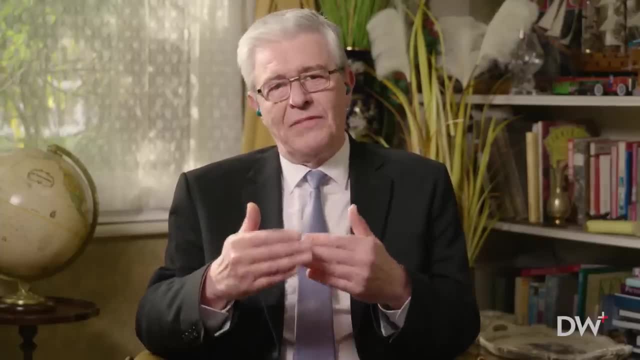 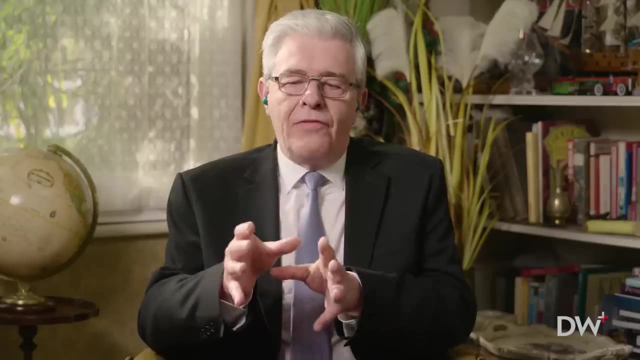 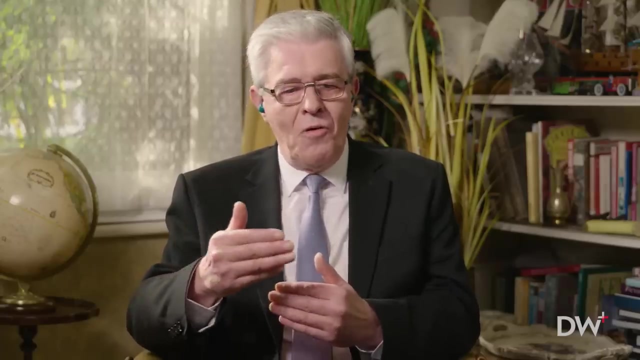 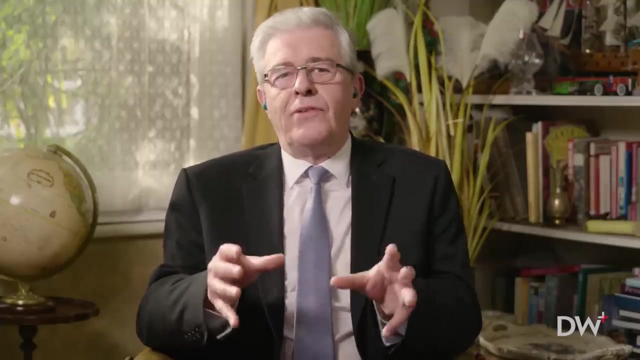 another side. well, i know there's another side to that: technically an unexpected information gain, um, or an epistemic value, um, and that's of course i. i will avoid putting myself in surprising situations, being very cold physiologically or being unloved or being embarrassed or anything that i would find surprising about myself. i will minimize my. 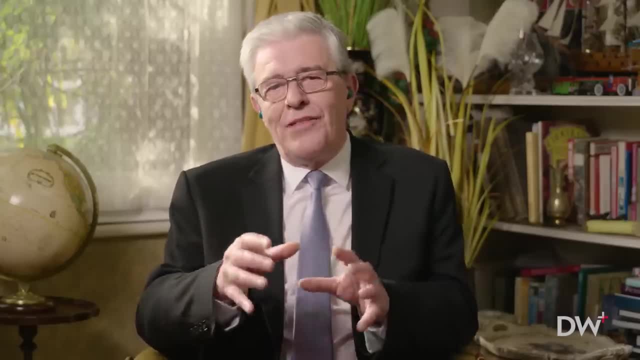 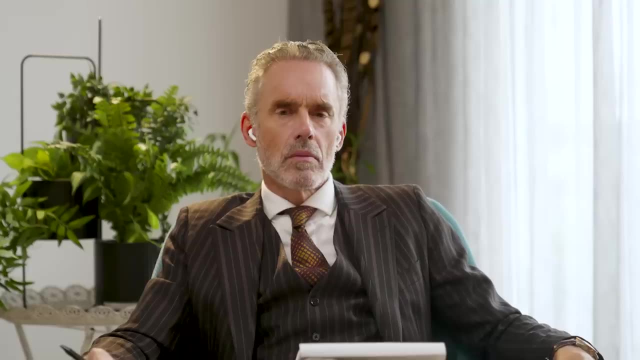 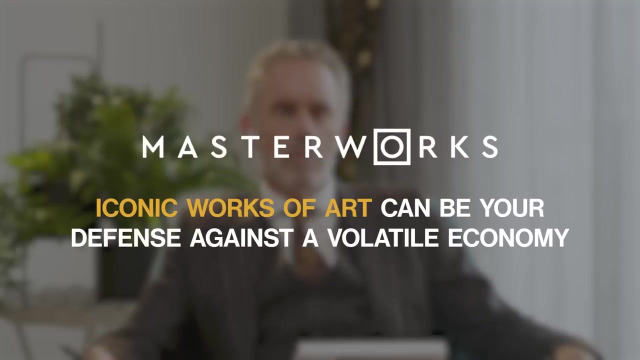 expected surprise by avoiding those kinds of things, and i think that's that's what you know at this point. what you were saying touches exactly on that. a shocking number of stocks are in the red. you may think you're doing all the things right, but in this volatile economy, many of our portfolios are just not looking good. why? according to the largest, 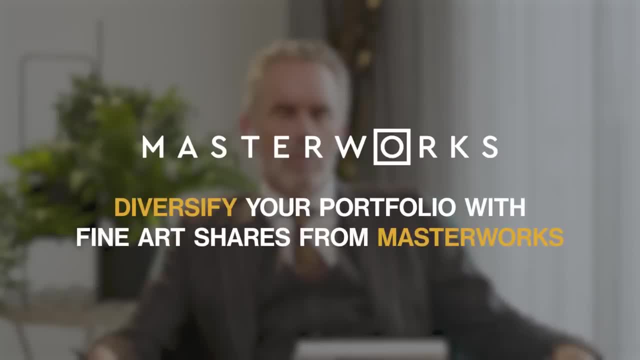 banks and firms in the world. people aren't diversifying the right way. the average annual return of the classic 60 40 portfolio is down by nearly 20 this year. goldman sachs just released a shocking report declaring the 60 40 doomed for the next decade and announcing it. this is a huge 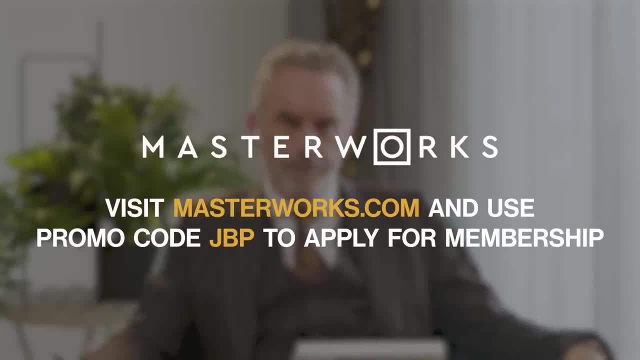 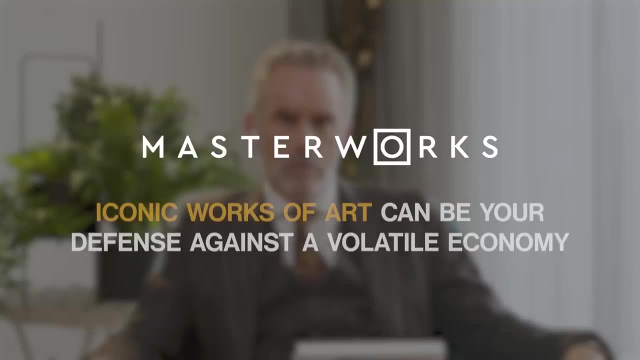 a radical reallocation from stocks entirely. Goldman will instead be investing in real, tangible assets, specifically fine art. The last time inflation was this high, some segments of the art market appreciated more than real estate and even gold, at an astounding 33% per year on average. That's why this show has partnered with Masterworks. Masterworks' 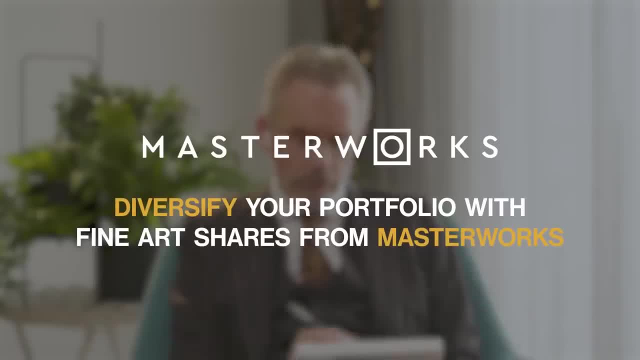 results have been exceptional: Six exits for an average net return of 29% to investors, even during COVID and in a bear market. As a result, Masterworks has had to acquire and release more art on their platform to meet demand. But you can skip the waitlist by going. 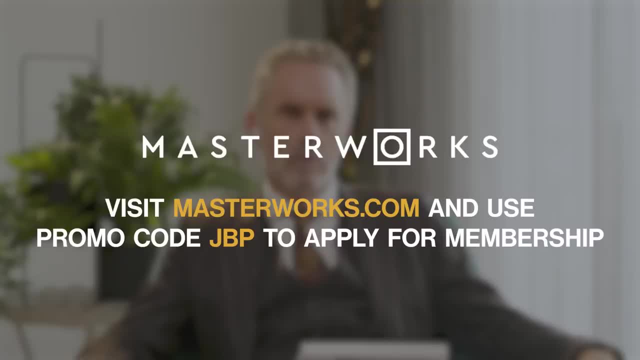 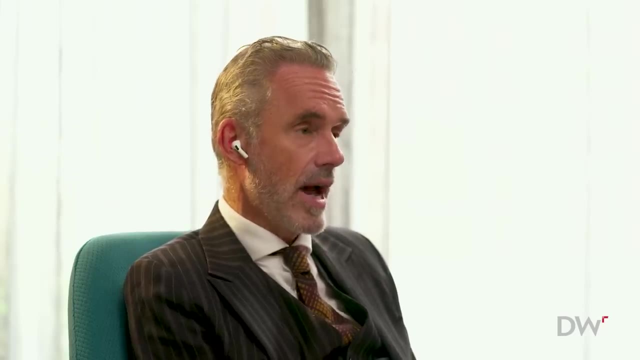 to masterworkscom and using promo code JVP. That's masterworkscom promo code JVP, or click the link in the description. See important disclosures at masterworkscom slash CD. I think people hem themselves in in their actions, even And once people. you see this. 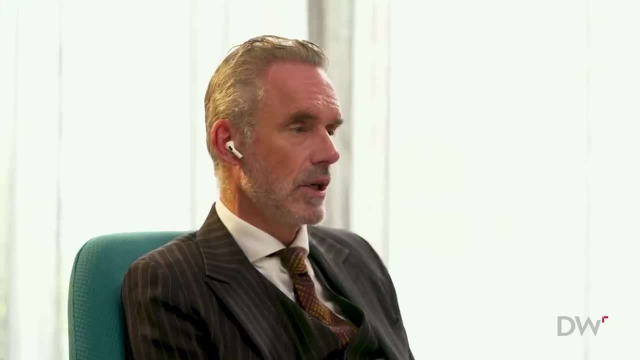 clinically is, once people develop a conceptualization of themselves which is a box, in some sense, to put their variability in, they'll sometimes simplify themselves in terms of their range of action, merely so they don't surprise themselves, And so they artificially constrain the range of their potential behavior, and that can become maladaptive if their conception of 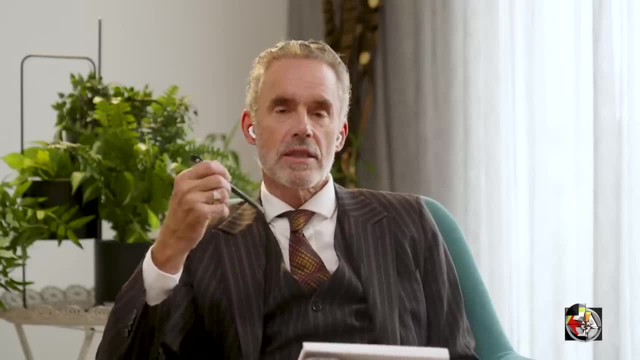 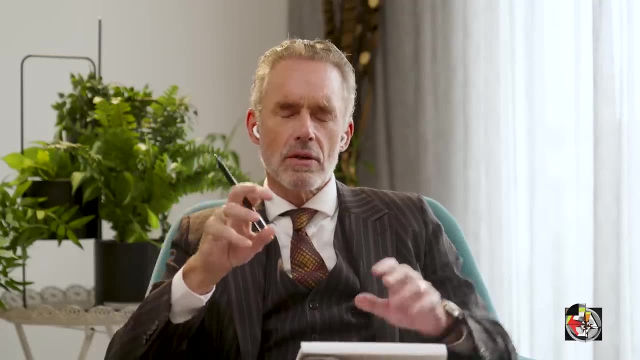 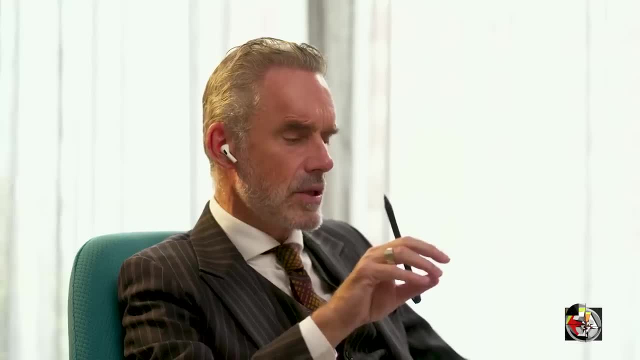 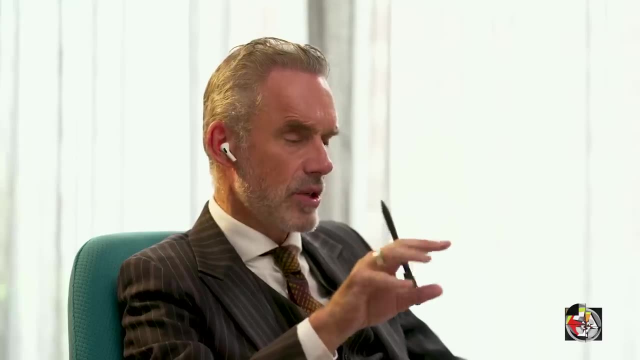 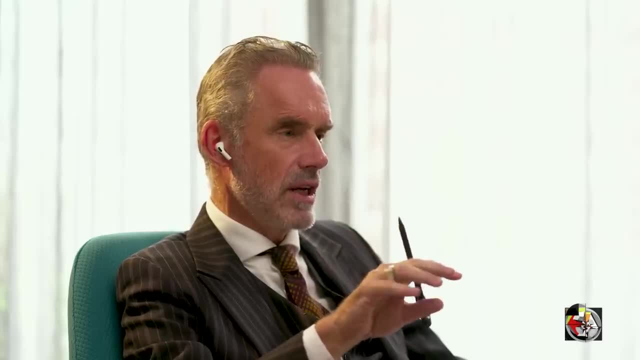 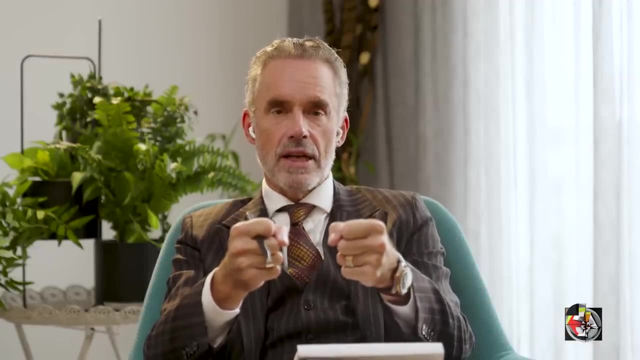 and the same as any other object in a multitude or even a near infinite number of ways. And so you could think, I always think of two goblets standing on a table And you might say: well, they're identical, but they're not. And you can tell they're not if you 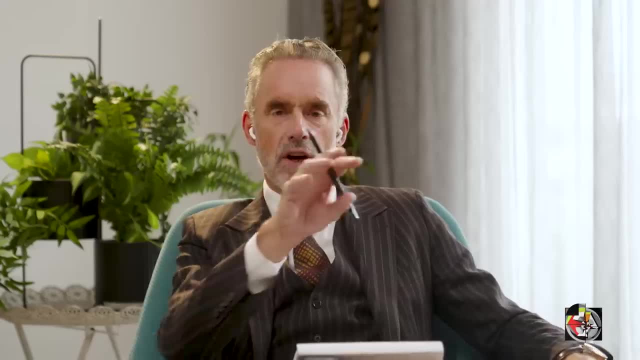 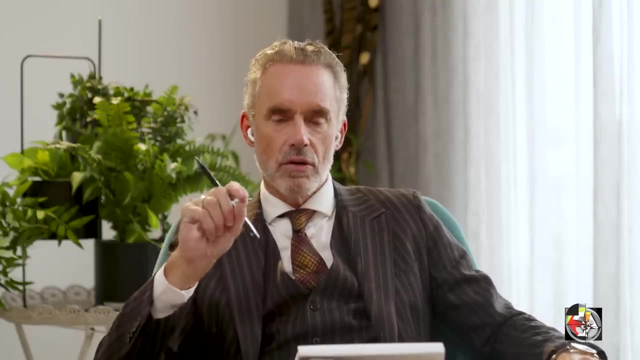 want to talk about it wanted to paint them in a photorealistic manner, you'd find that the surface of one goblet is very much unlike the surface of another, and you'd have to render that at high resolution in order to represent it accurately on a canvas. And then they differ in weight and they differ in the. 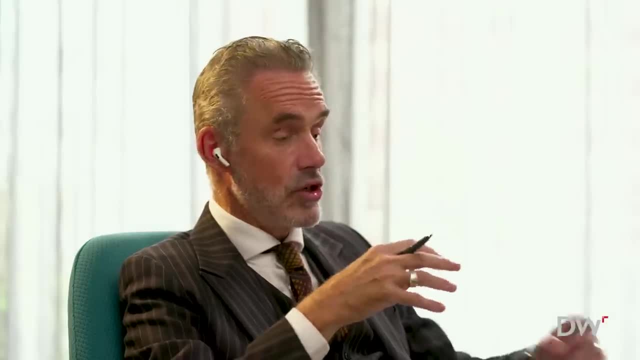 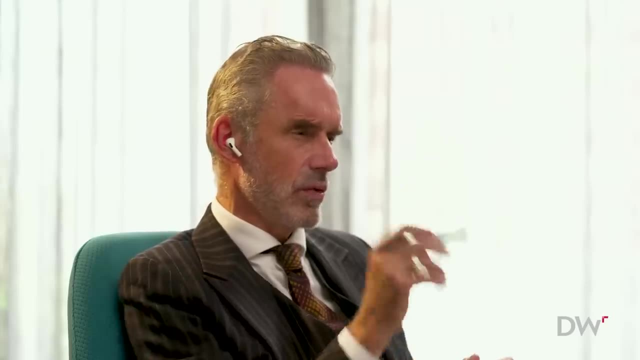 regularity of the surface, and they might differ in age. There's all sorts of differences between them that you might not think are germane or relevant, but that's really the issue is: why do you regard some similarities as crucial and some differences as irrelevant And so? 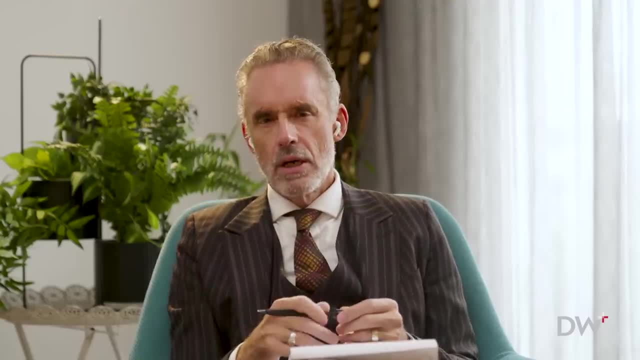 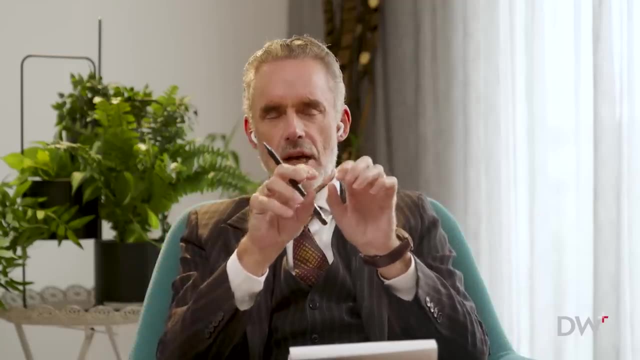 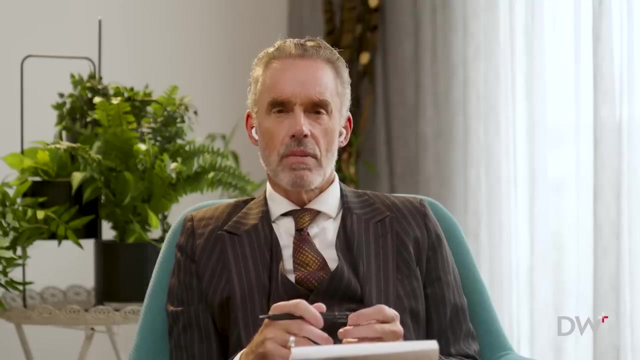 here's something I'd like to run by you. So would it be reasonable to say? imagine a hierarchy of perception and conception. so the idea is: well, two goblets are identical if I can drink out of either of them using the same pattern of perception and action. So 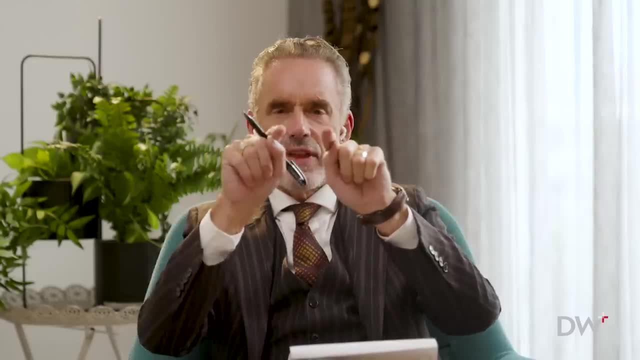 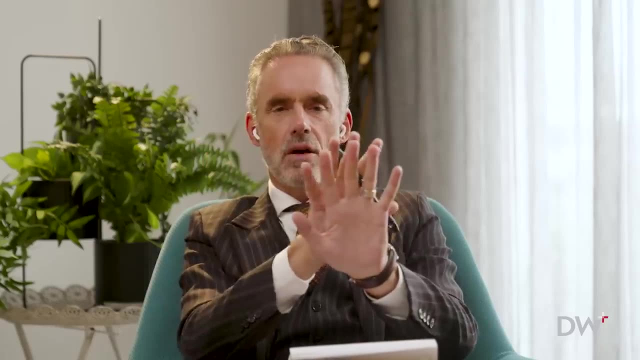 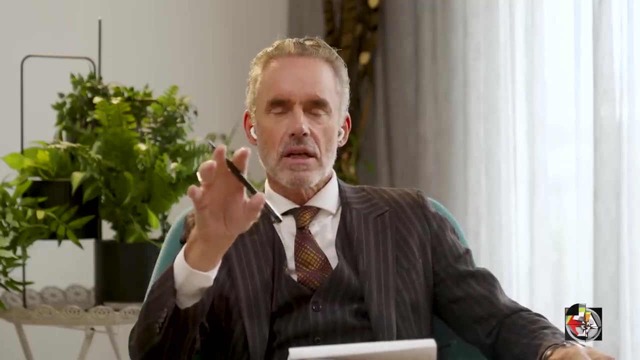 it. so that's kind of an indication of the entropy constrained by the notion of wishing to drink. Any two things are substitutable as long as they leave me with the ability to drink as an axiom of my current action set, And that's something like maybe a computational definition of resemblance. 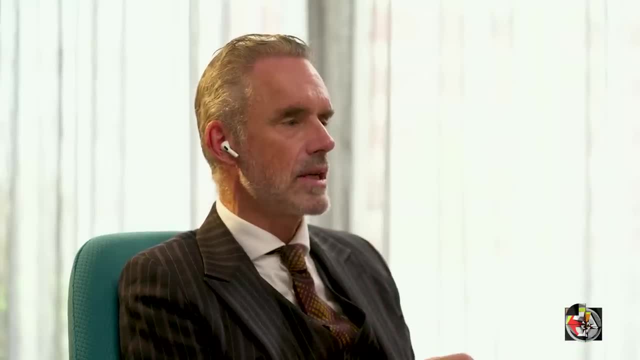 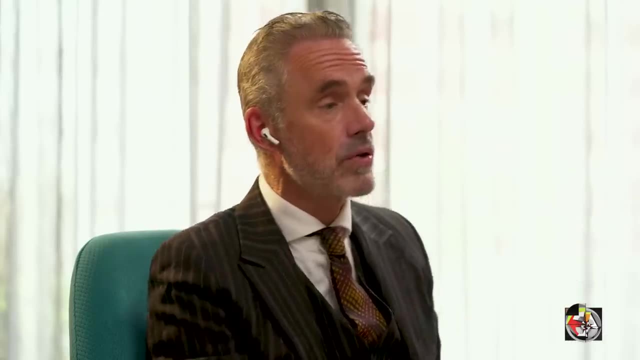 Because I can't understand how you can bind resemblance otherwise. if any two things differ in a near infinite number of ways, They differ in terms of the microstates that they might be composed of. That would be a way of thinking about it from the perspective of entropy theory. 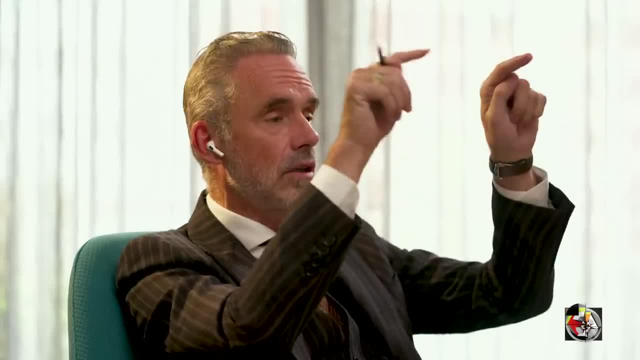 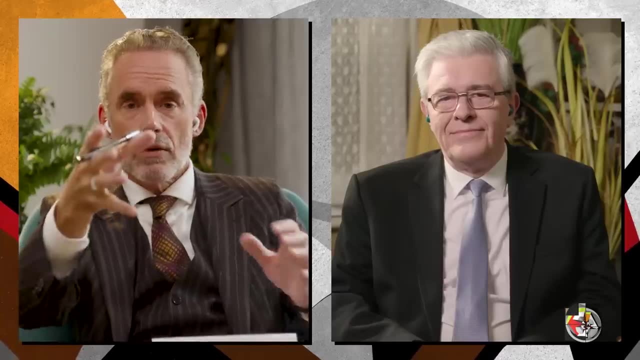 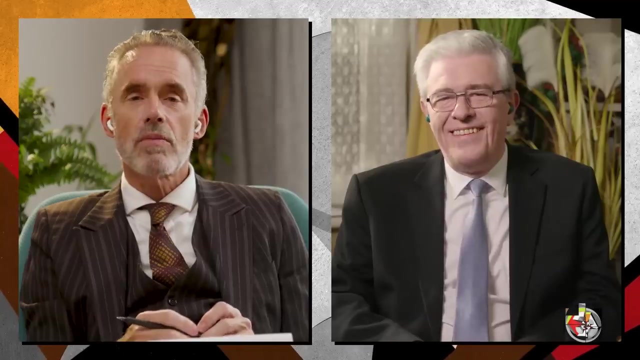 So if they're substitutable within a higher hierarchical conception, then they're identical perceptually and conceptually. So do you know the change blindness experiments that was Dan Simon managed at Harvard? Yeah well, that's a good example, right? So I'll just run. 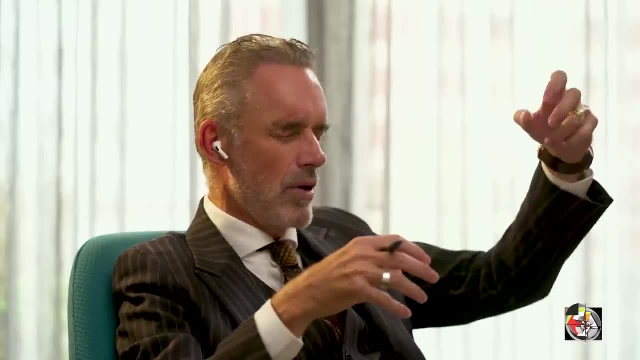 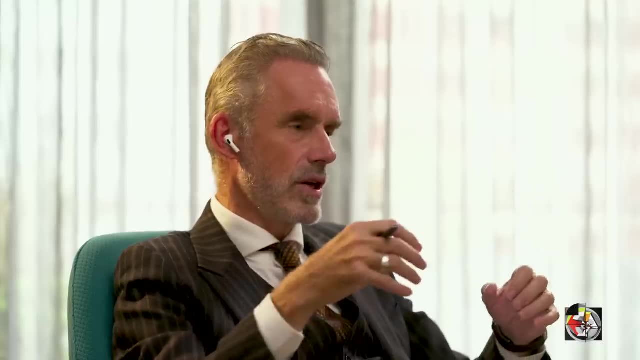 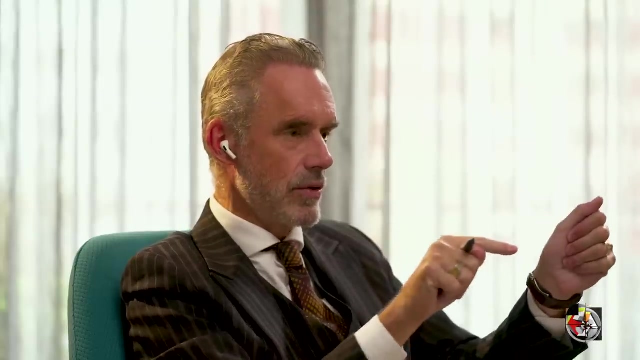 through one of those experiments For the people listening. So imagine you put a camera on a two-story building and it's looking down over a university yard. And now imagine that you have tourists walking through the yard and an undergraduate research associate comes up to a tourist with a map and asks the tourist: 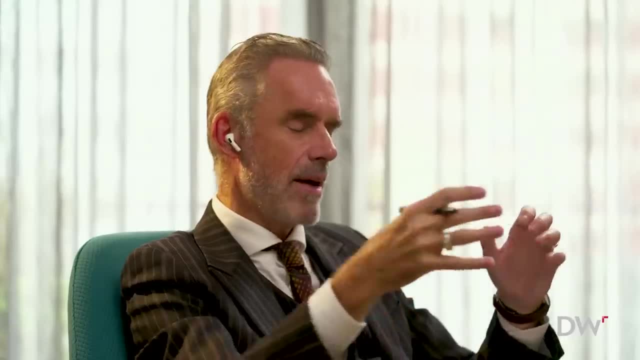 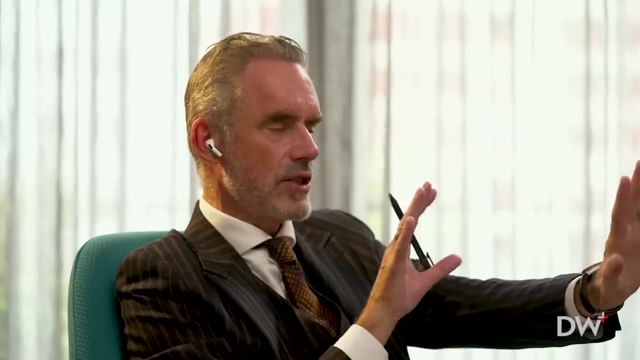 to help him find his way. And while that's happening, some other experimental compatriots walk between the person who's asking for directions and the tourist carrying a door to a university yard. And they're walking between the person who's asking for directions and the 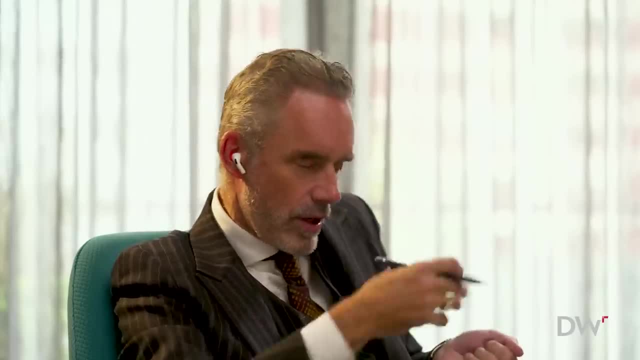 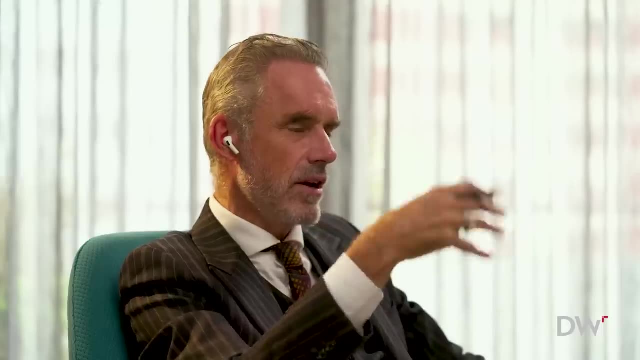 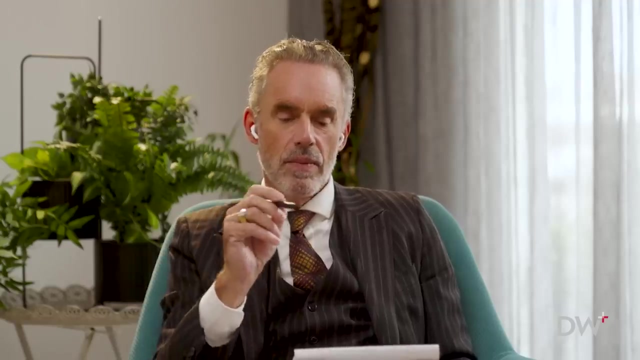 two of them, And the person asking the question grabs the door, hidden from the tourist, and continues walking with the door, And the person who is carrying the door stands there and continues asking the question with the map, And what Simon found was that the largest percentage of people. 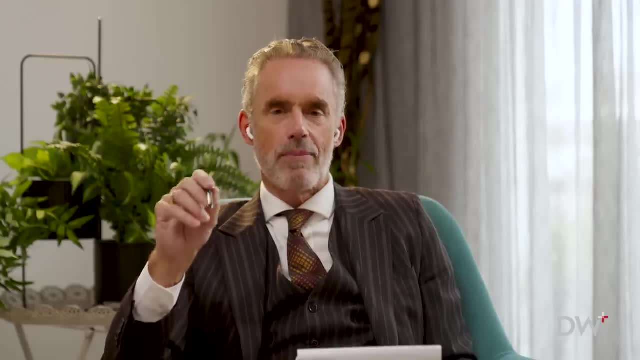 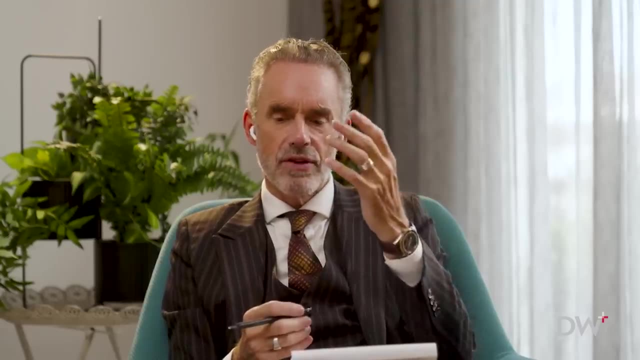 the majority of people do not notice that the student has been swapped in the middle of the conversation, And the reason for that has to be that the percentage of people who are walking in the middle of the conversation is the majority. So the perception of the student by the tourist is: 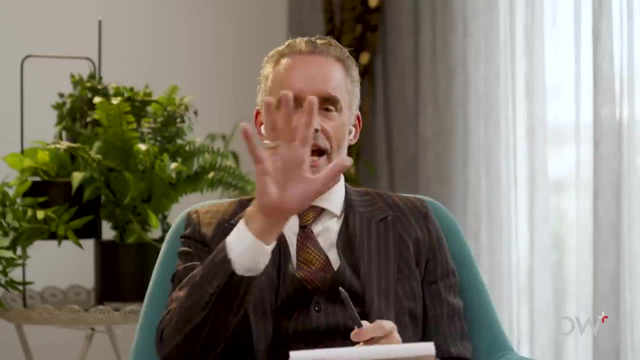 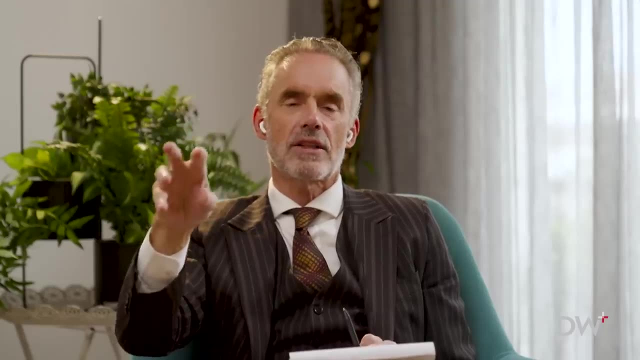 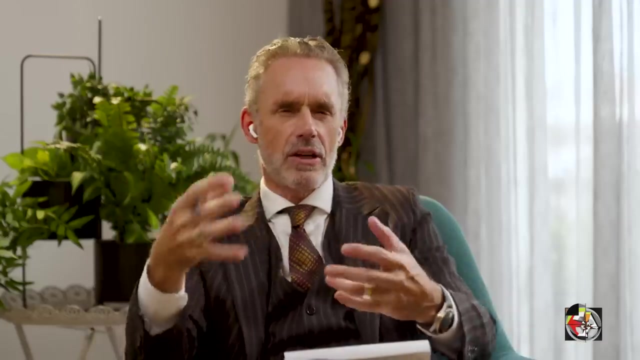 something like generic student asking for directions, And any student who's asking for directions at that point will fulfill that function or act as a player in that story, And so there's no reason to be surprised by the transformation, even though- quote- it's a different person, And that seems to add credence to this notion of a theory of. 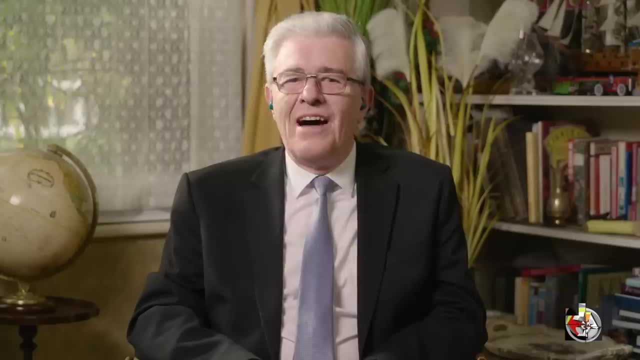 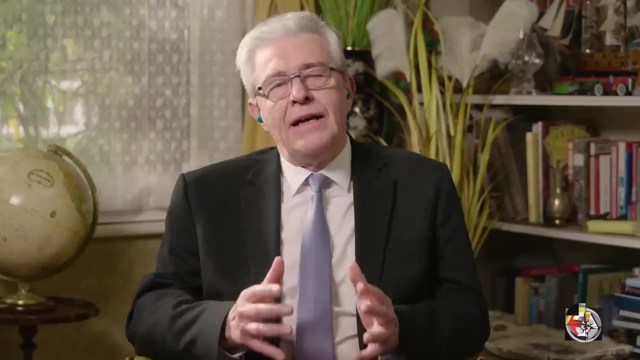 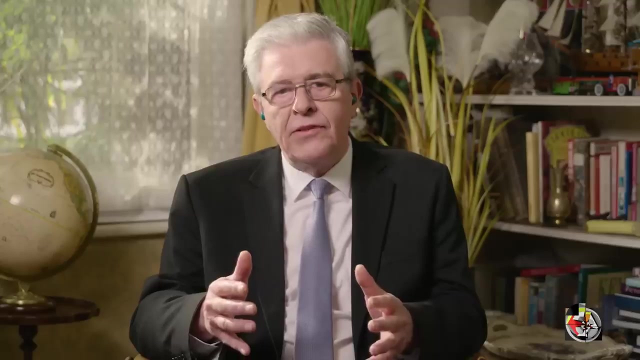 identity or resemblance. Does that seem reasonable to you? It seems very reasonable. So mathematically, I think you could. you would describe that exactly in terms of finding those latent states or categories or structures or resemblance that are conserved over different contexts And that 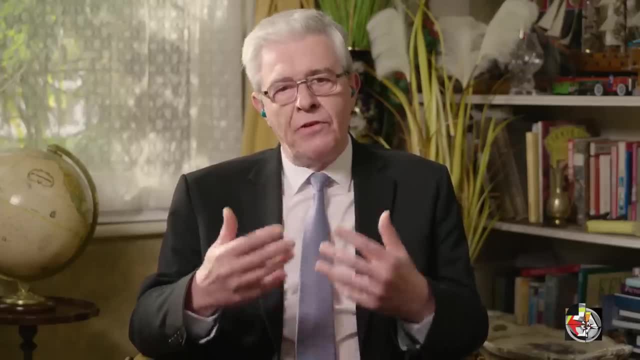 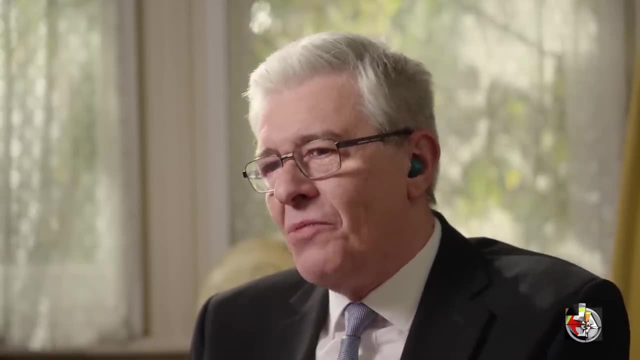 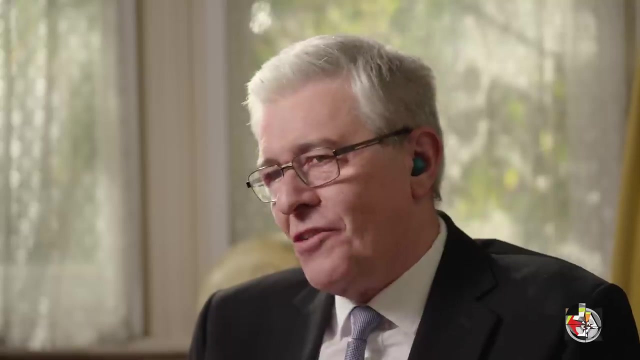 enables you to have a simple but apt for purpose model of your world. So if you can find the causal structure that is as simple as possible, that provides an adequate explanation of your sensorium, then you know that is the good model. I mean literally. 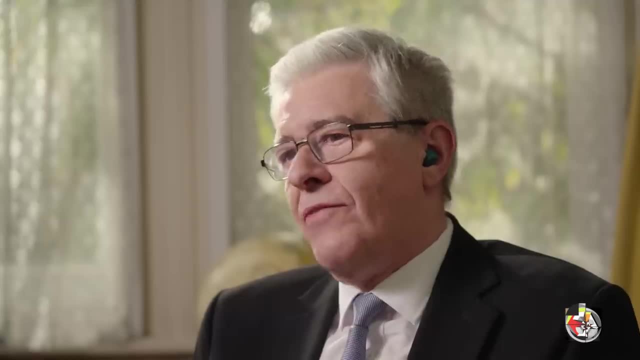 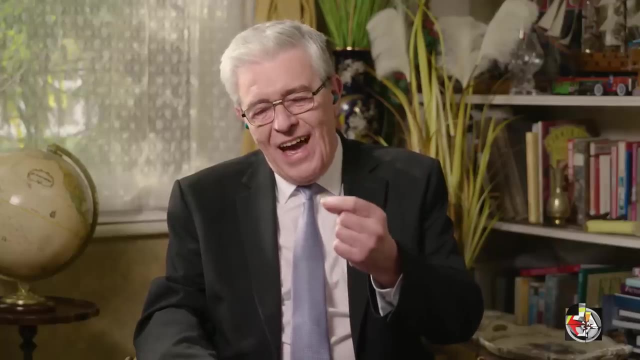 as a statistician, I think it's a good model. I think it's a good model. I think it's a good model, But as a statistician, that would be the model with the greatest evidence, the accuracy minus the complexity. You also brought something interesting into the conversation again, which was what I 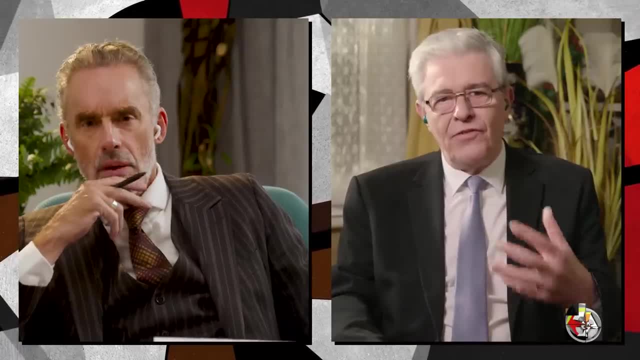 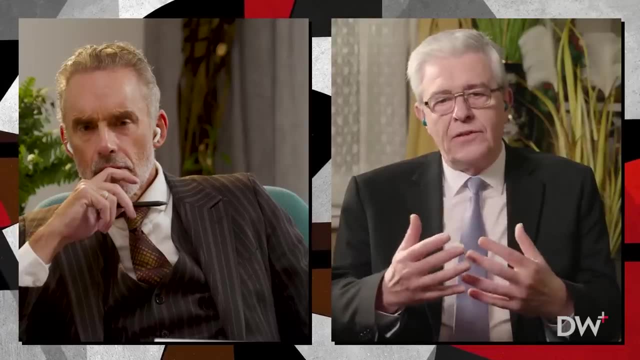 would read as affordance. Do you like sort of Gibsonian notions of affordance? Yeah, So you were saying that? this, you know, this ability to extract the latent structure, the essence, the resemblances that are conserved over different contexts, you know they have. 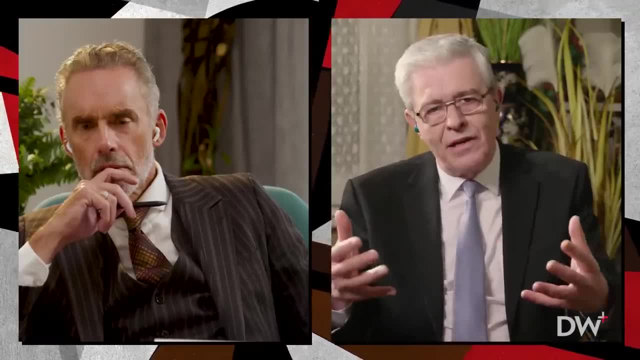 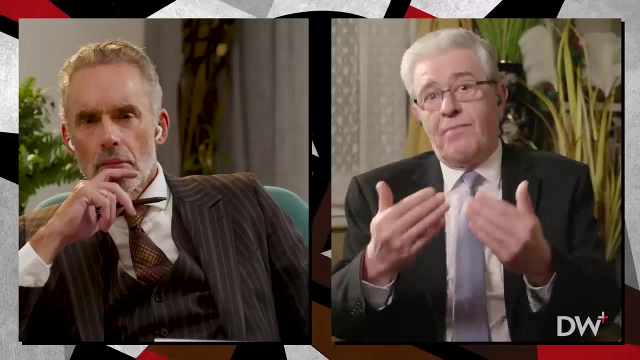 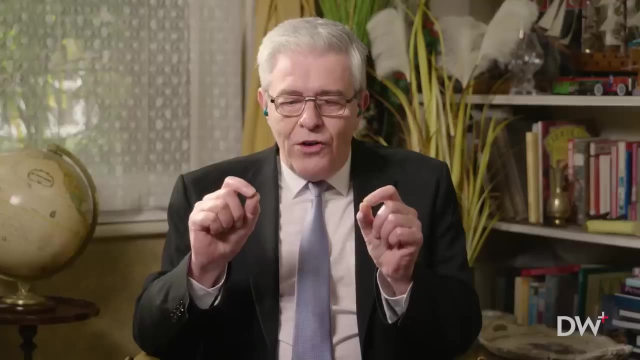 at very low levels of the hierarchy, these microscopic or detailed differences, but at higher levels of the hierarchy they are the same kind of thing. They have the same affordance. I sit on this, I drink this. I love that. I don't like that. What you've done, though. 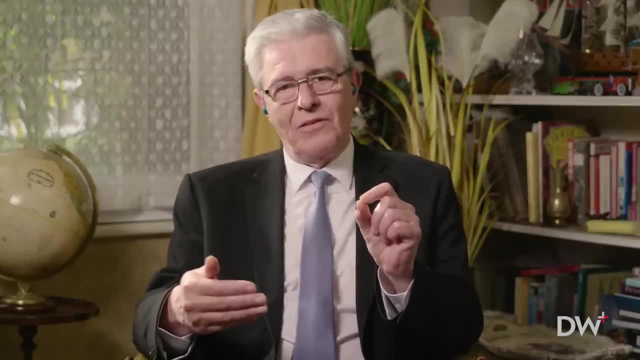 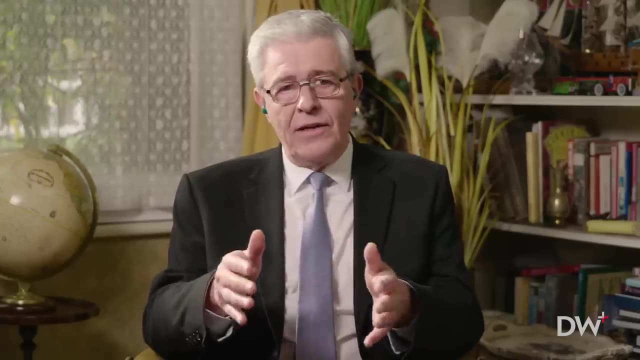 again in terms of talking about affordance, is: bring action, you know, to the fore. You know I can perceive lots of inferences in my world. You know there are categories and there are, you know, exemplars of particular categories and I can unpack that hierarchically, And many 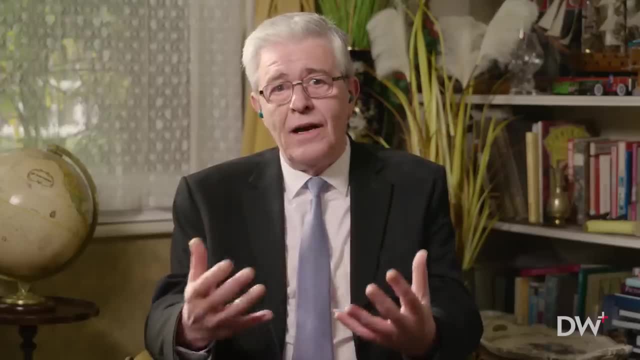 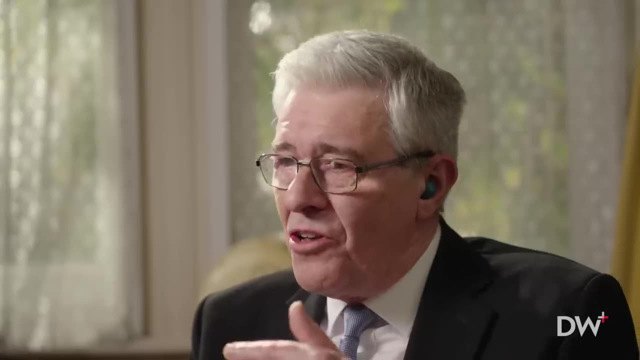 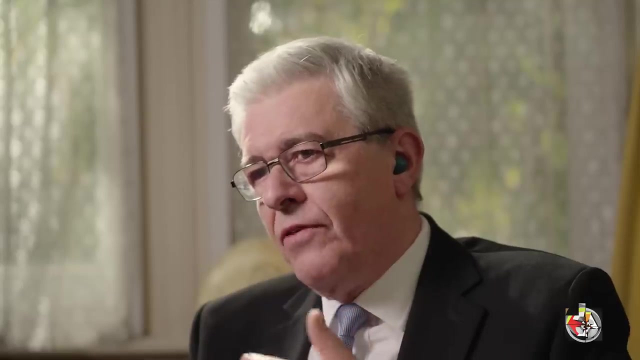 people think that's how the visual hierarchy, the cortical hierarchy that subtends or subserves visual perception and visual synthesis, is organized. But what you're saying is this also holds true in the way that I plan to act and the outcomes of those actions and all of these. 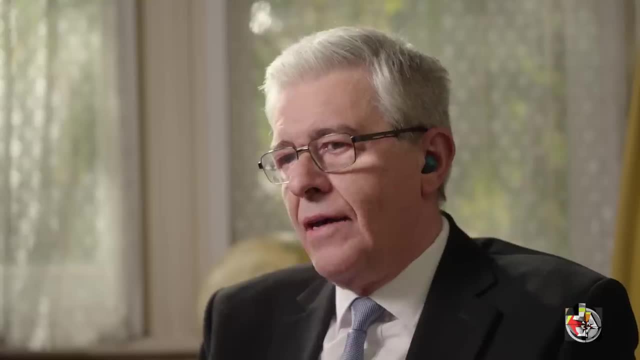 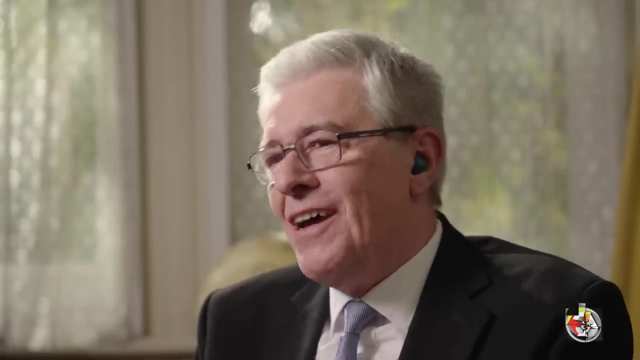 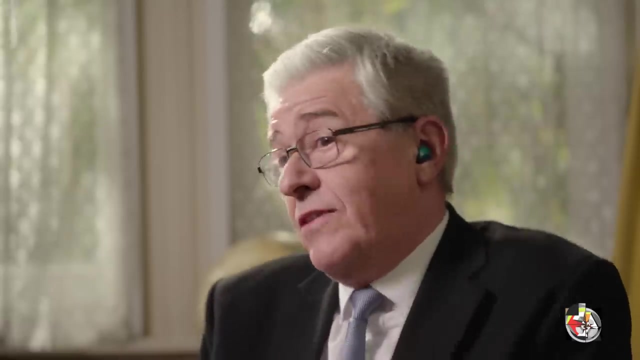 if I get those inferences out, then they are the right kinds of affordances that speak to my model of the way I'm going to behave in the situation, putting center stage the self-model. You know what kind of thing am I and what will I do in this situation, And is my model good enough? 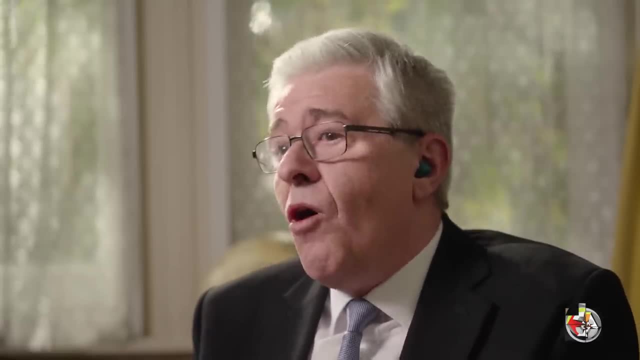 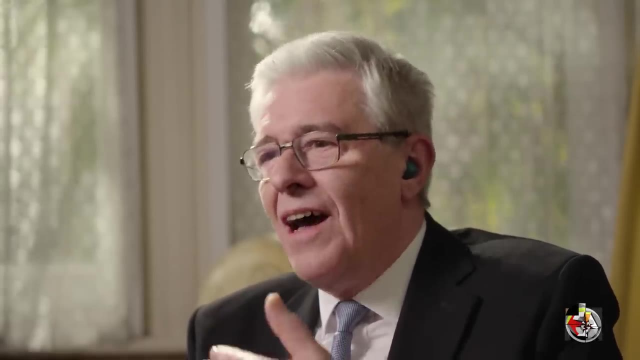 Is it too rigid? Is it, you know? should it be more flexible? All these are crucial questions in terms of updating not just your beliefs about what you're doing and the context in which you're operating, but the kind of thing you are and whether you've got the right simple explanations. 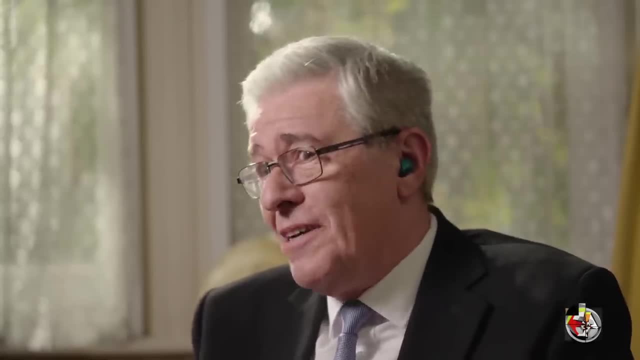 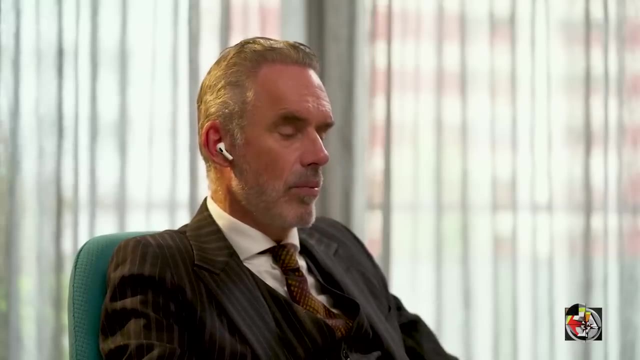 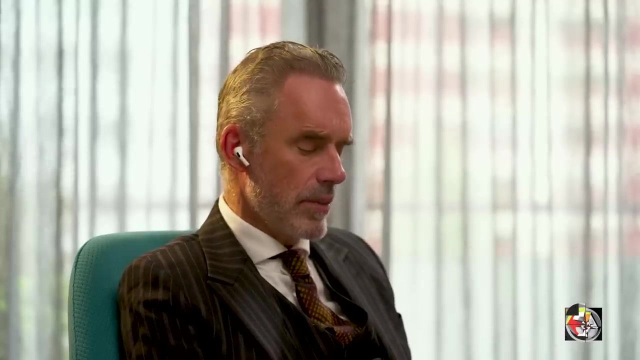 whether they should be more complex or or simpler, Right. And so the optimal simple explanation is the least complex affordance necessary for the operation at hand. And so then we could, we could talk about affordances a little bit, So people who are watching and listening might think that you see the object and infer the meaning. 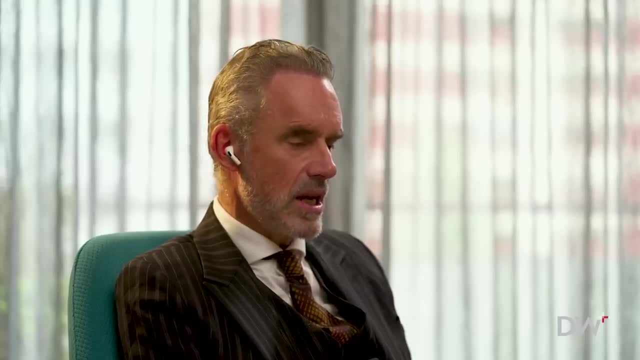 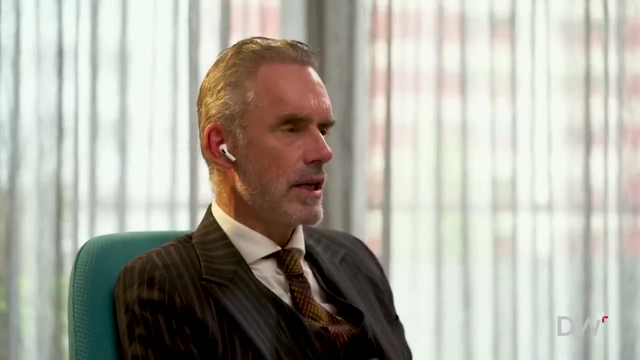 but the theory of affordances would suggest that you see the meaning and infer the object or something like that It reverses it And that what you see first is the meaning of the object. What you see first is something like functional utility, But I think you can bring both those. 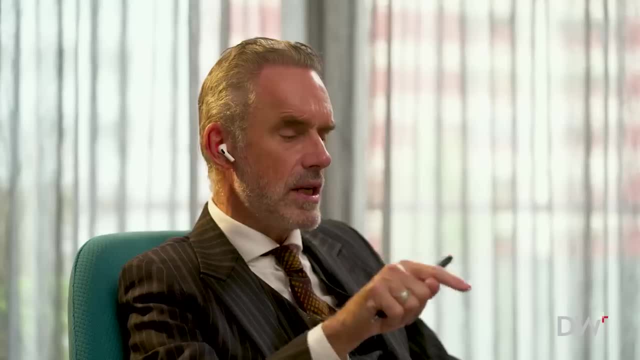 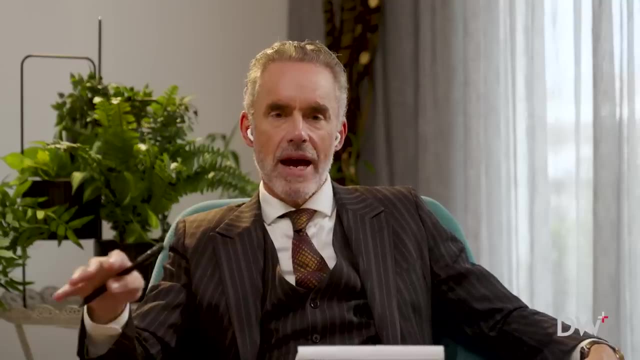 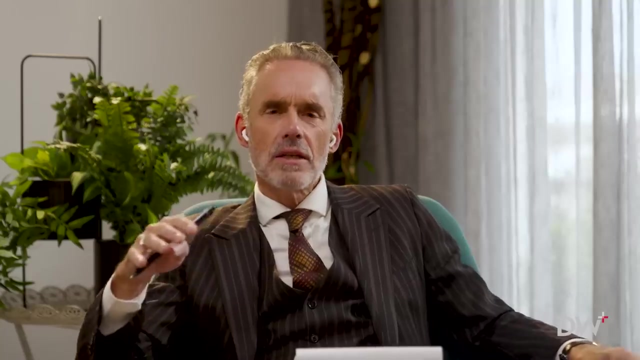 positions together. if you think that what we see in the world are patterns that have functional utility. Now, there's all sorts of patterns that don't have functional utility or that only have potential functional utility, And that might be. you might consider patterns that don't have. 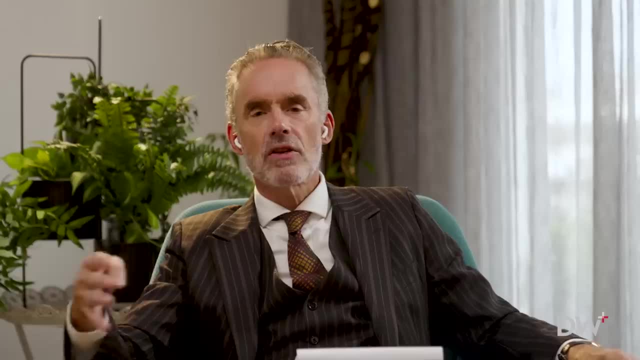 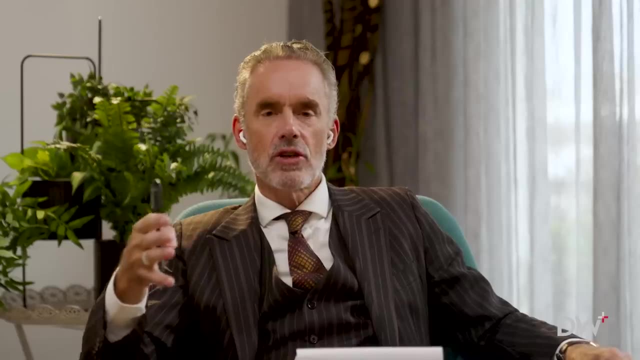 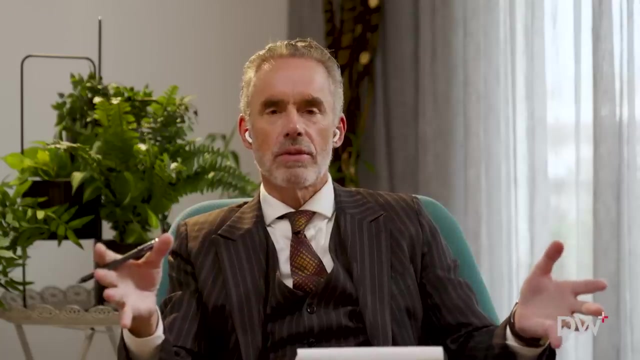 specified functional utility as something like the infinite domain of potential empirical facts. If a fact is something like the accurate identification of a pattern that exists, stably across contexts, But then we can't see all the set of all possible facts because it's way too. 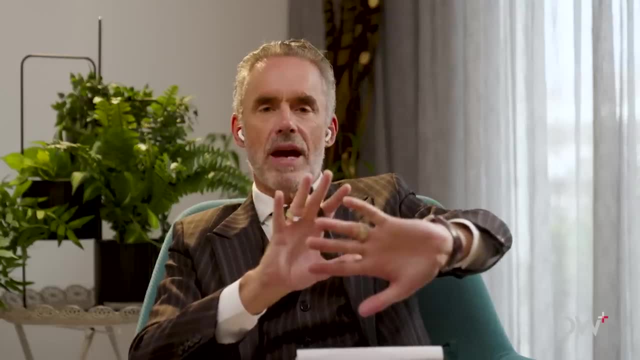 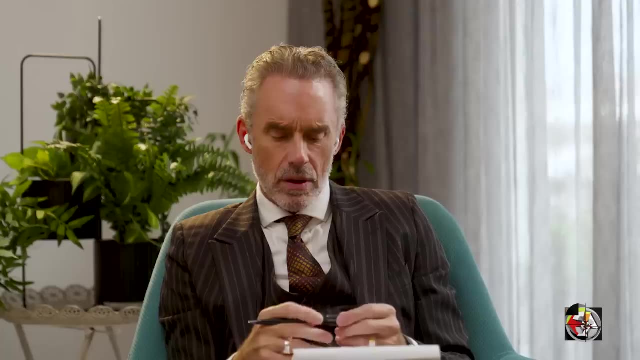 large, And so we want to reduce that further to that set of patterns that offer us a grip on the world. And Gibson, who wrote An Ecological Approach to Visual Perception, talked a lot about affordances, tools and obstacles in particular, If I remember correctly. 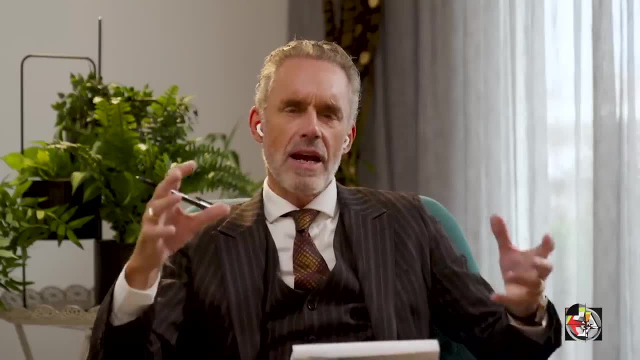 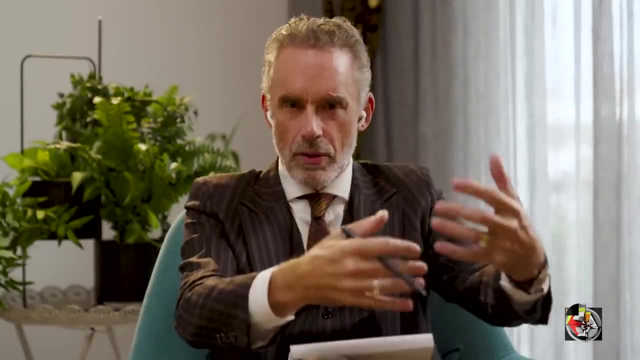 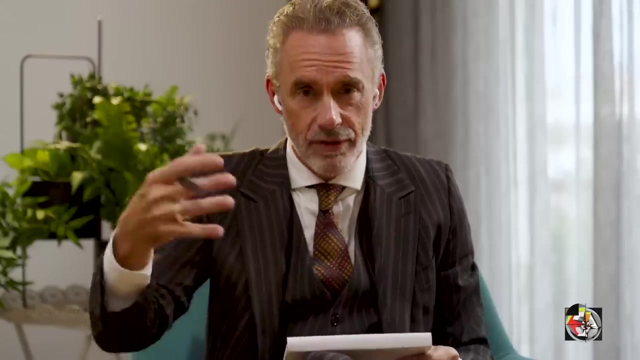 but I'm wondering as well, is it is the domain of affordance? here's a way of conceptualizing the domain of affordance. It's tool, those things that you can get a grip on the world with and move forward towards a desired goal. Obstacles, so things that get in your way, of different size. 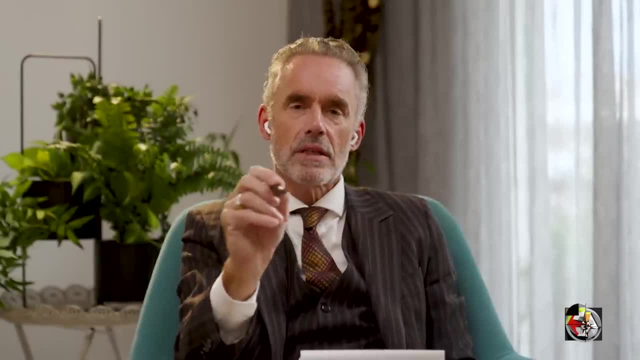 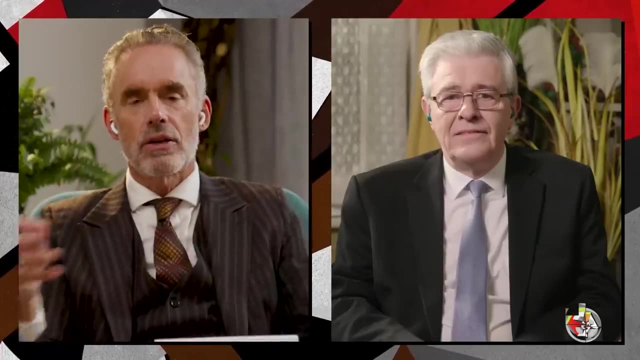 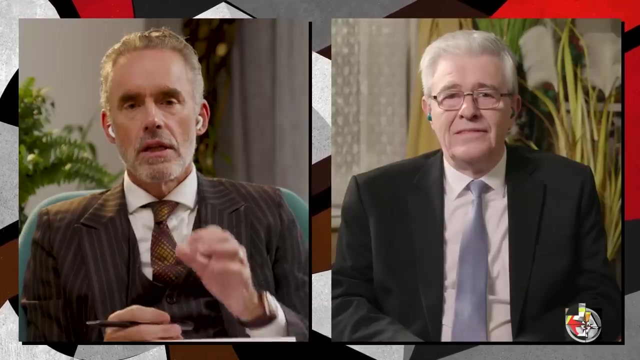 And then pathways And the pathways. in some, so I would say, the pathways are littered with tools and obstacles, And the description of a pathway that's littered with tools and obstacles, that's a story. And so these, these, it looks to me like those hierarchical conceptual 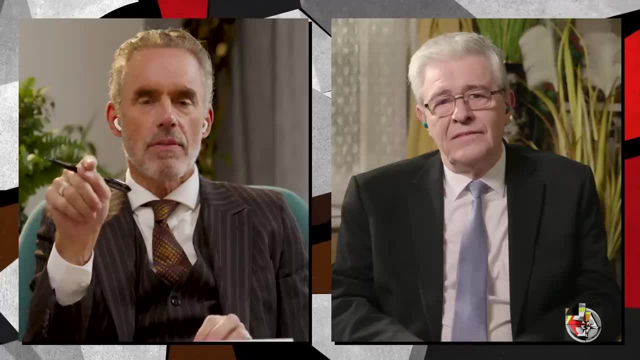 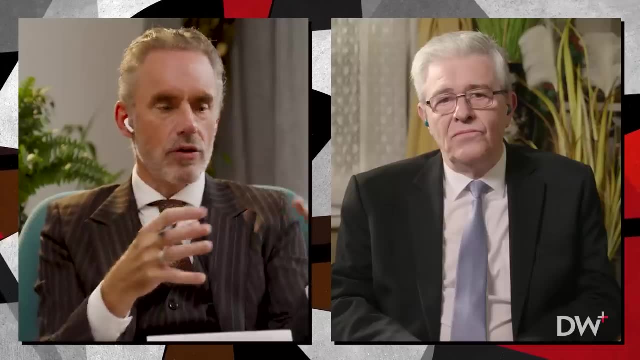 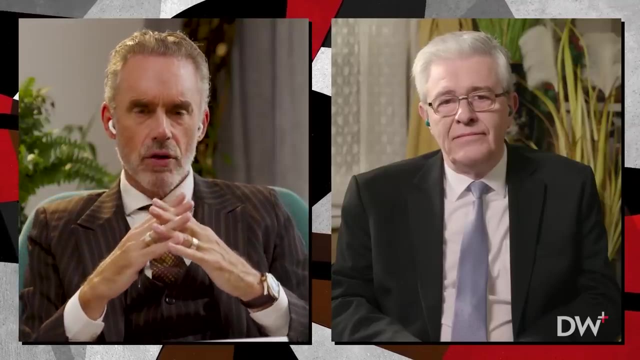 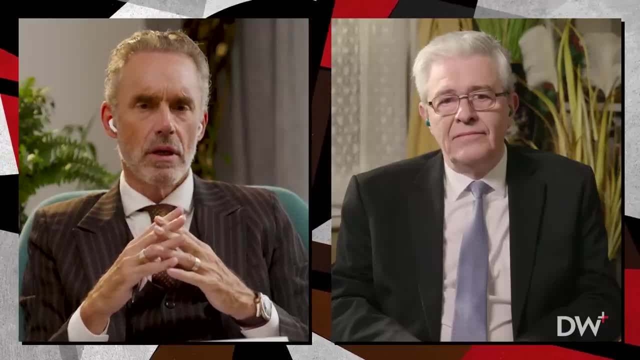 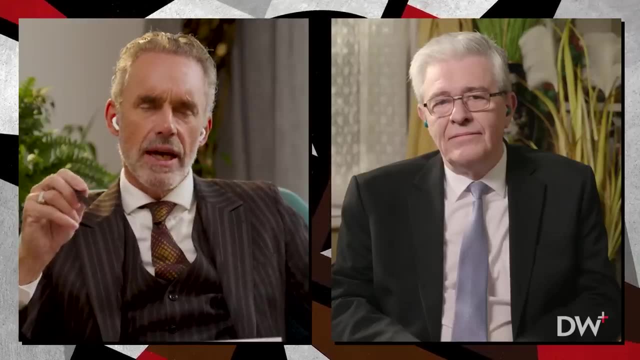 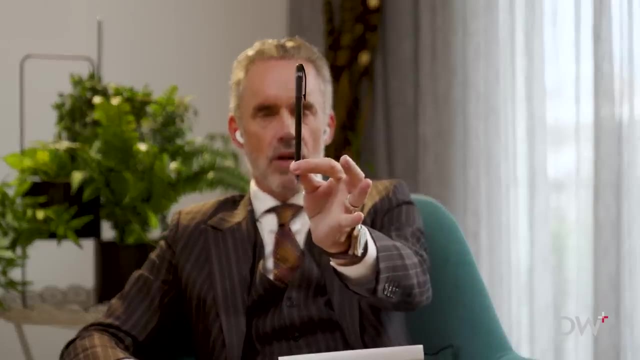 the purpose meet. That's a, that's a way of thinking about it. Yeah, And I would think, maybe even when you perceive a tool, it seems to me that what you're perceiving is something like a micro story. You know, like if I perceive this pen, say well, that's obviously, it's an. 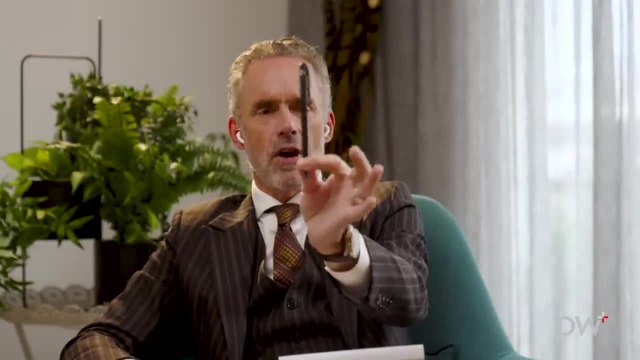 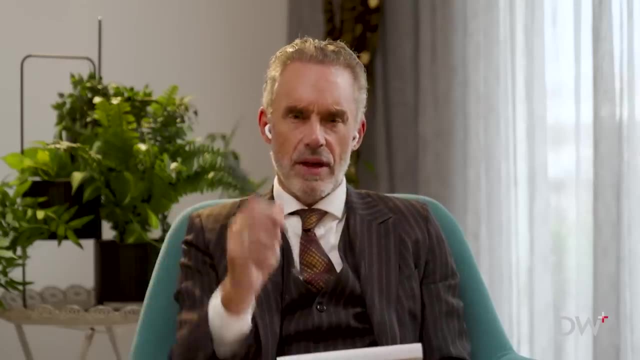 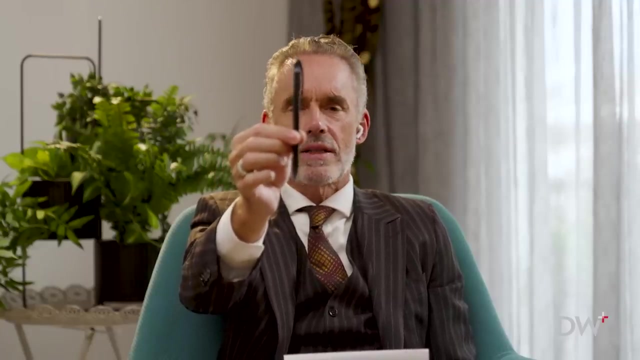 objective fact that this pen exists, And it is insofar as the pen is a stable pattern in time and space. but it's the function of the pen that makes it a pen and gives the unity that. it gives the unity to the perception, because you might ask: well, why is the pen a pen? 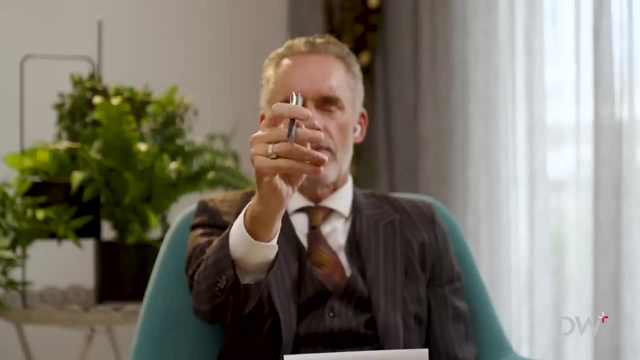 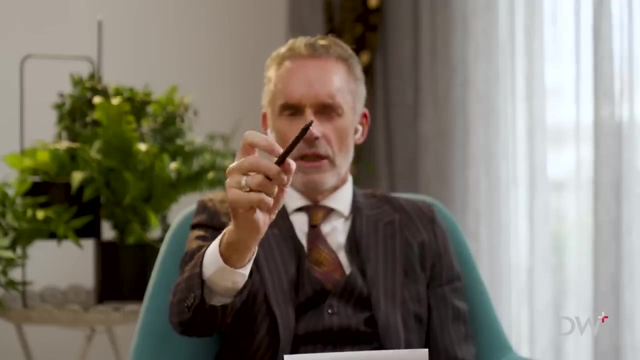 this way and a pen this way, and also a pen this way, and speak well, because, because it's, it's objective characteristics transform tremendously when it's moved or when it's illuminated differently, but its function remains constant, And so, I think, even an 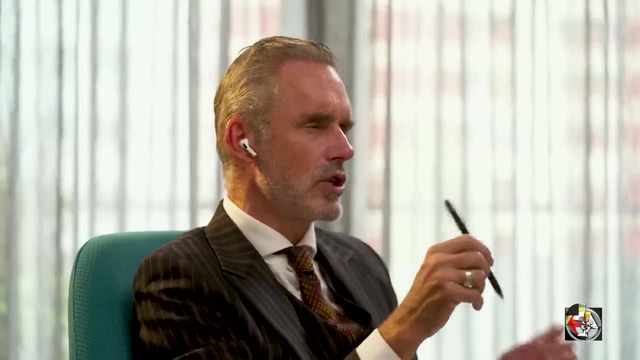 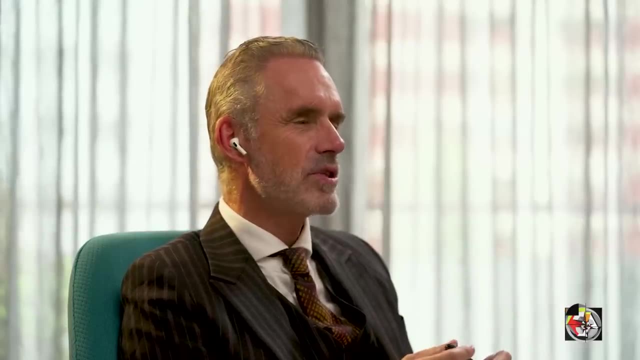 affordance is a micro story, And so a tool is a positive, it's a comedy, That's a way of thinking about it, And so I think even an affordance is a micro story, And so a tool is a positive thinking about it. A tool is a comedy and an obstacle is a tragedy, And- and we lay out the 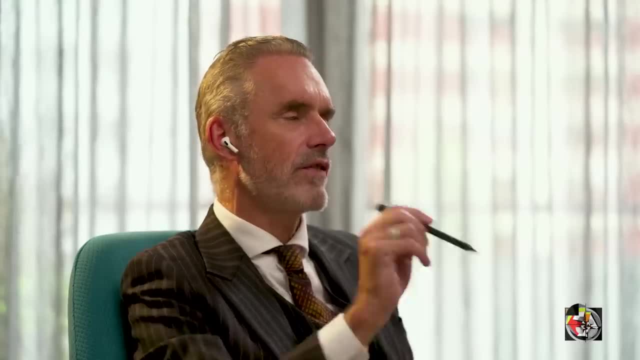 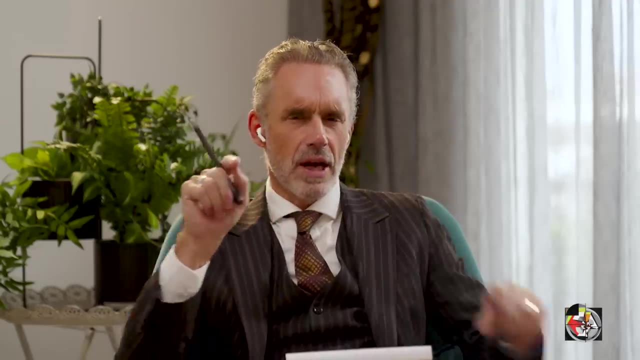 world like that, even at the levels of our fundamental, even at the level of our fundamental perceptions, Is there any? what do you think of the idea of a concept or a percept as a, as a story? Because you see, the reason I like that, the reason I think this is so important, is that there's an 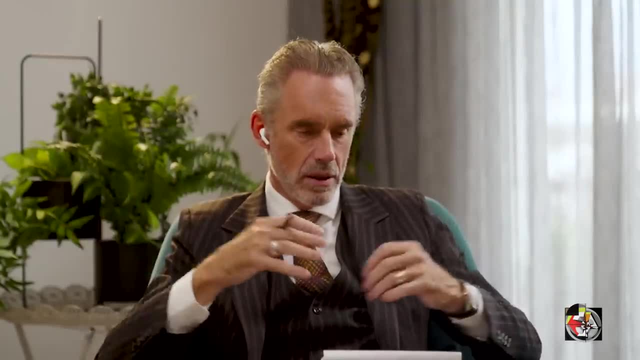 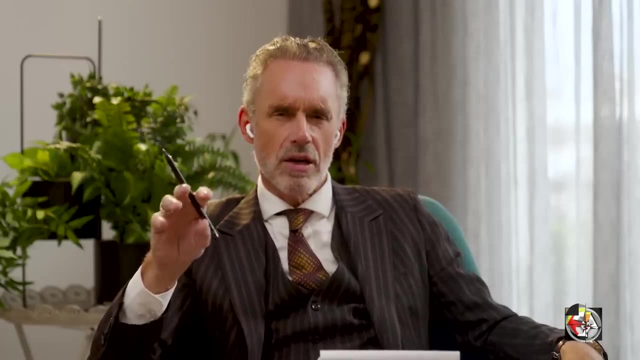 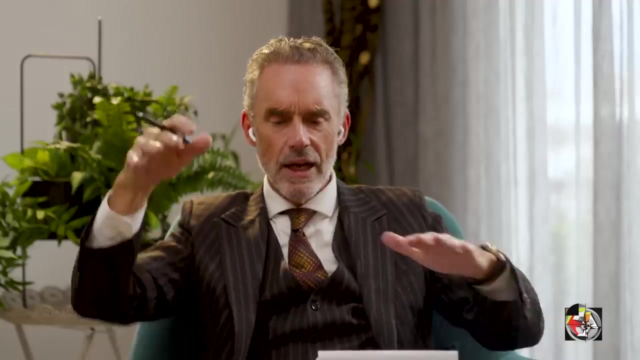 entire literature on narrative. Of course, the entire literature on literature is about narrative, And if it is the case that our fundamental concepts are narrative in, in their, in their, in their origin and their nature, then that allows us to lay the narrative world on top. 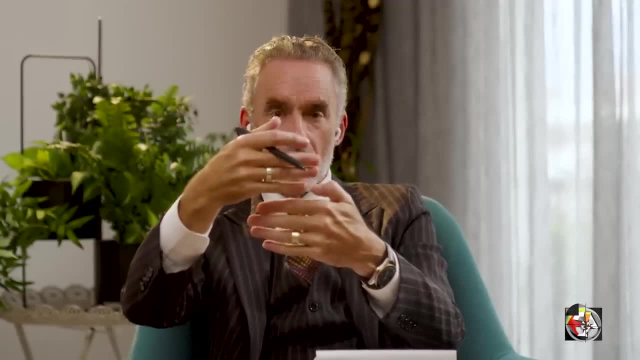 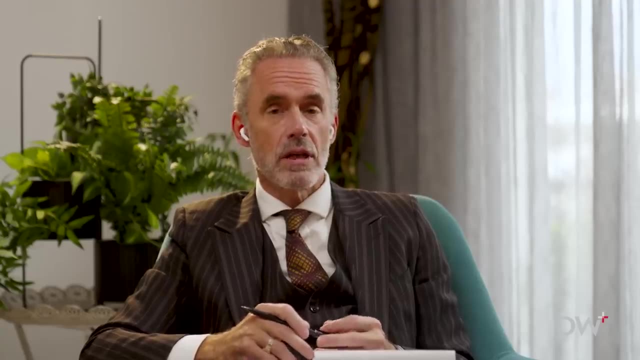 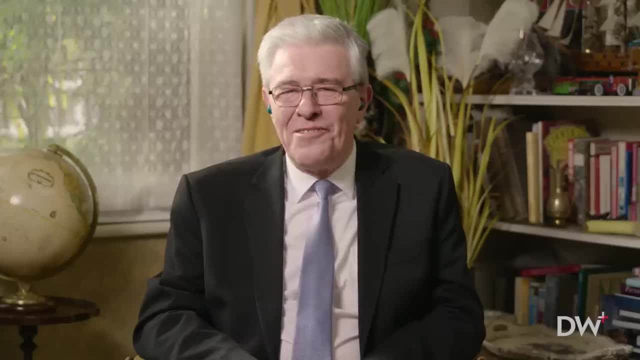 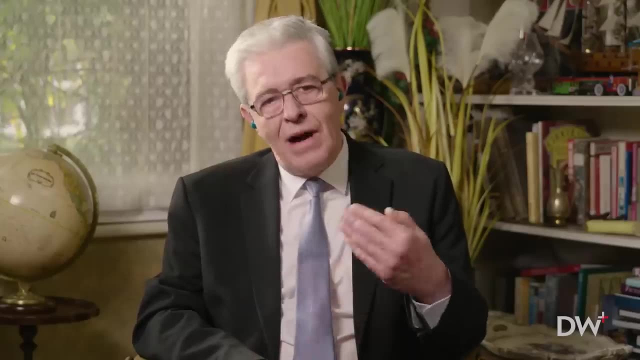 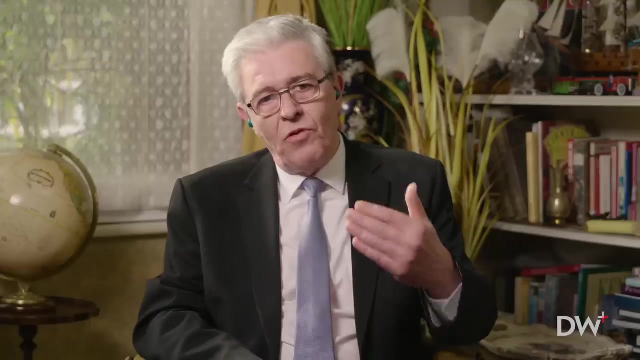 in terms of hierarchical processing. Yeah, I think there's some deep truths there. Um a number of ways I could sort of paraphrase what you've just said. So this notion of micro-stories and narratives, I think that is exactly the plans into the future that we were talking about before. that, you know. 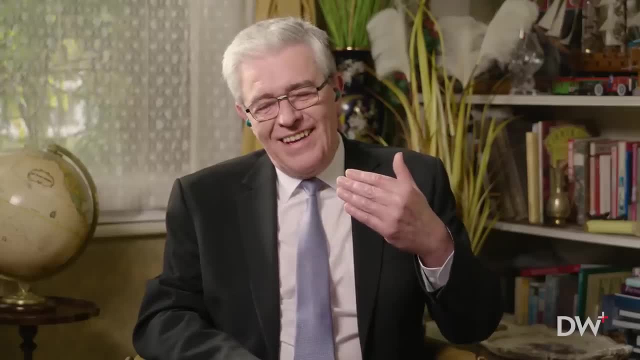 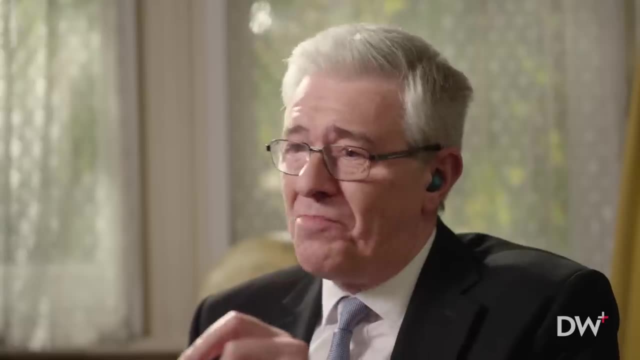 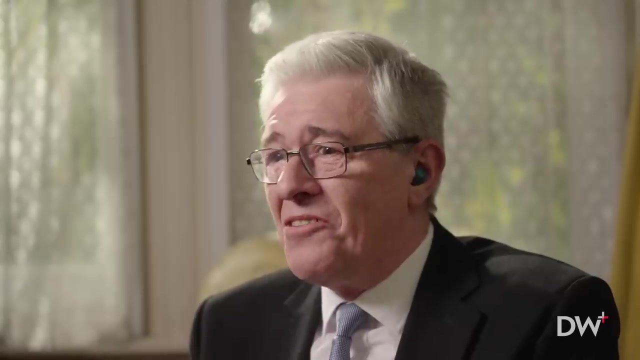 choosing the right ones, Um, and mathematically you can think of that exactly as you articulated, as as a path Um. one perspective on that is that of Richard Feynman in terms of the pathological formulation of quantum electrodynamics. 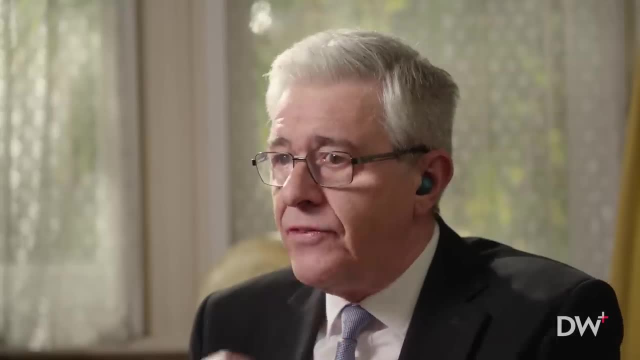 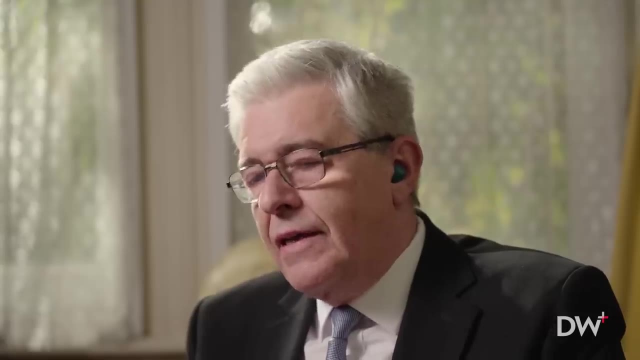 where he was playing exactly the same game: finding the path of least action, the path with the least obstacles, the path that is the most fluent, the most egocentronic, leading to exactly what we talked about before: either the information gain. 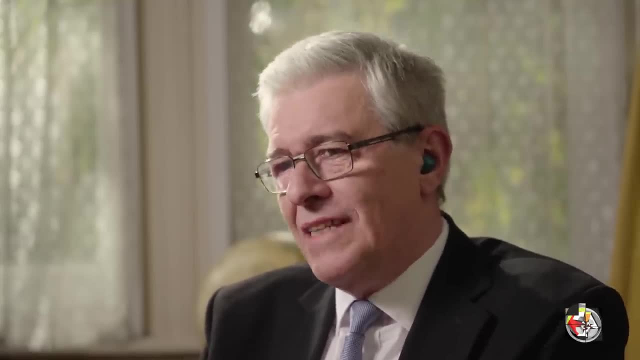 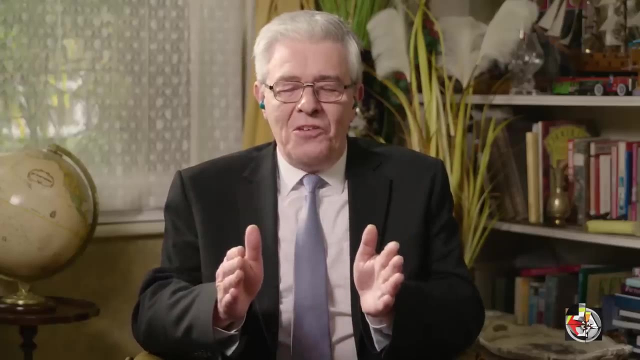 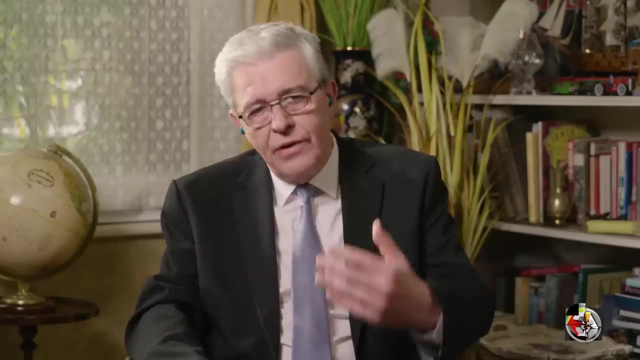 or avoiding surprising outcomes, which I would read as the obstacles. I don't go there. That's not the kind of thing that I'm in. So if you read our active engagement with the world, our active inference, just as a process of committing to the right paths, 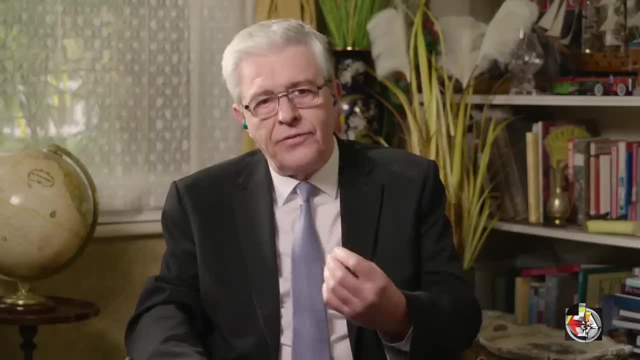 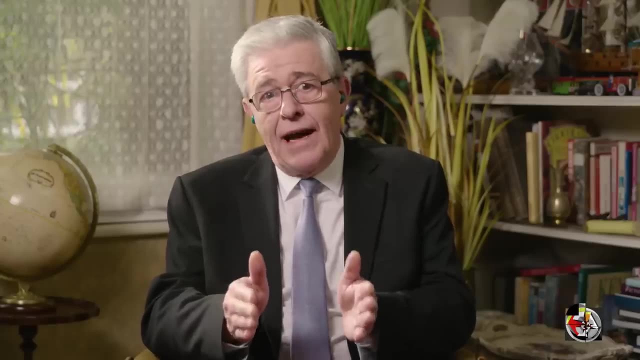 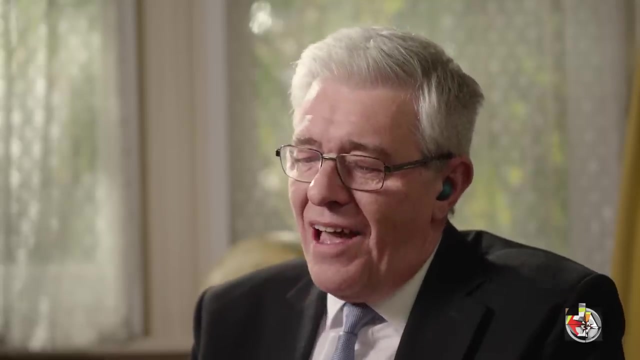 the right plans, the right narratives, the right micro-stories. I think that is the essence of, one could argue, sort of sentient behavior and existence. So I would put myself very much, or I would certainly find it very easy to commit to that kind of formulation. 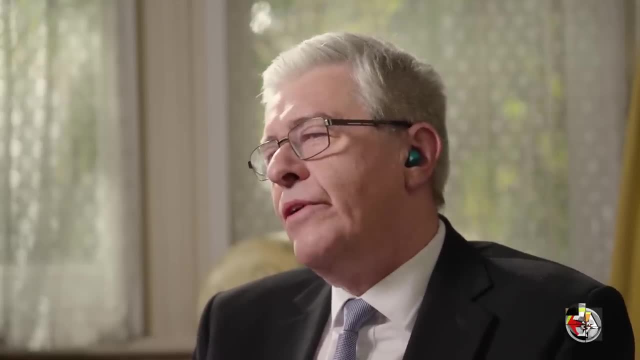 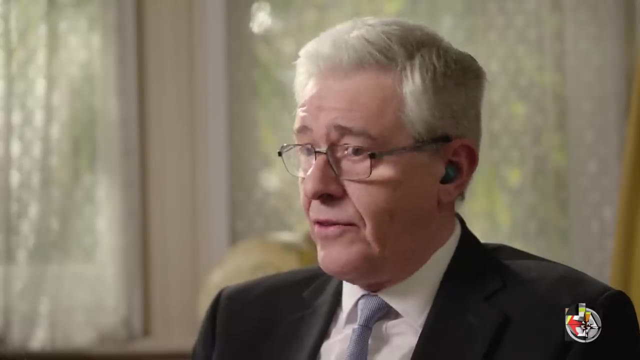 I think a lot of other people would as well, in different fields. So what you're talking about- you mentioned before about you know all the facts that are knowable and yet we only register and recognize those that matter, essential variables, for example. 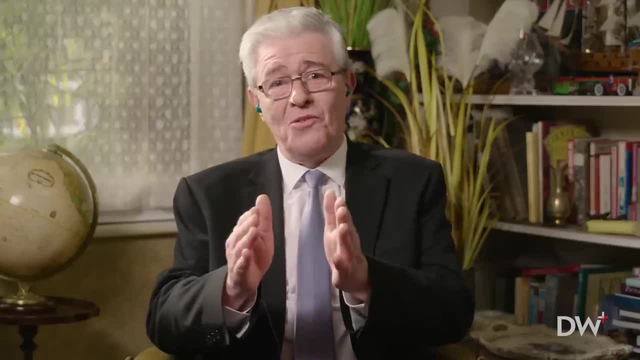 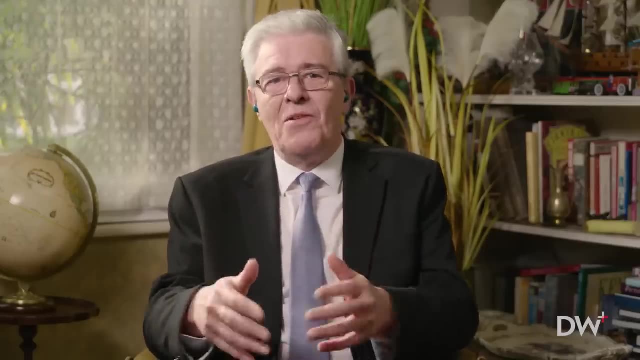 Change. blindness is a nice example of that. You don't see student of a particular identity, personal identity change. It's just a student. You only see and you only model and rehearse and sample the world using the level, the simple level of explanation. 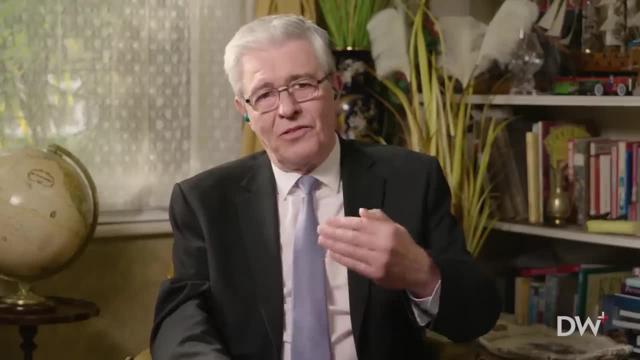 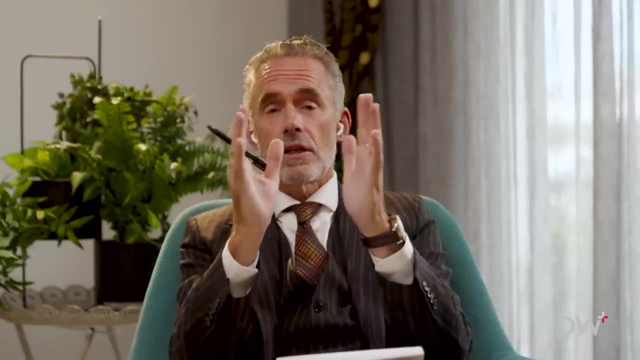 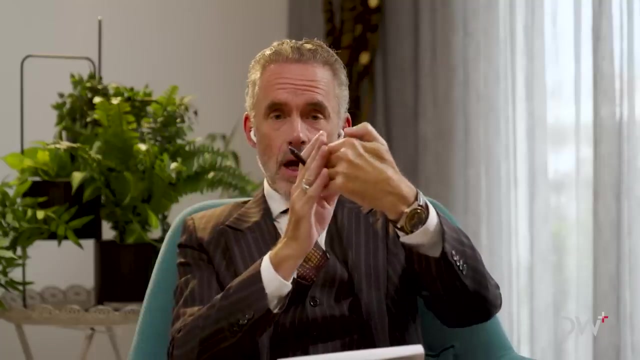 that is apt for getting those right paths forward. Yes, well, and it would be lovely if your hierarchical conceptualization consisted of micro-stories, let's say, that were flexible enough so that they would apply across a very wide range of microstate transformations. 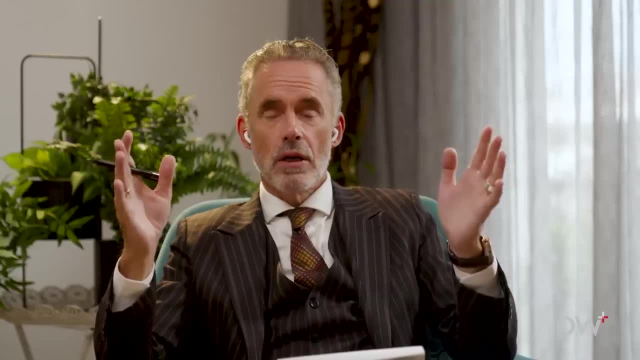 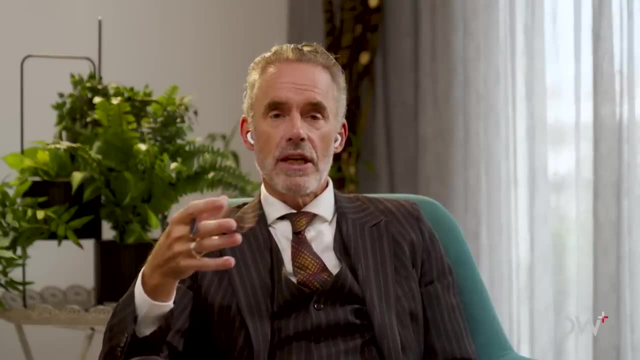 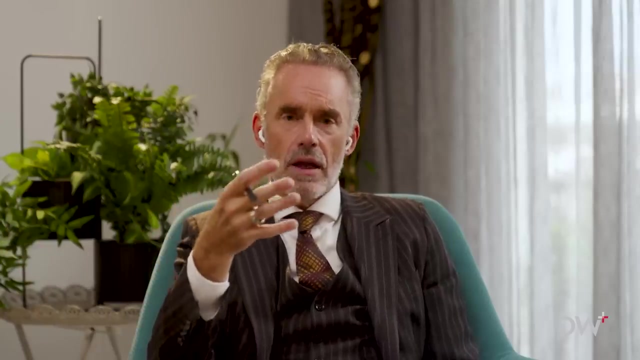 because then you can use the same simple model in all sorts of different situations. So you might say: well, if you could extract out a universal ethic for dealing with people, then you could apply that ethic to everyone that you met And then- and that idea might help us triangulate in- 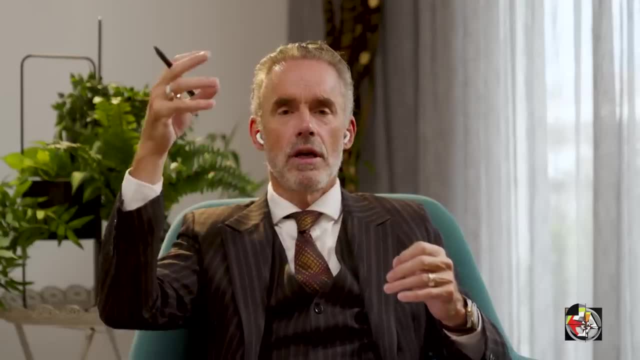 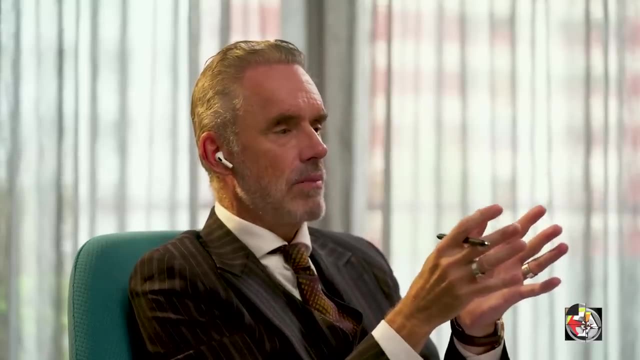 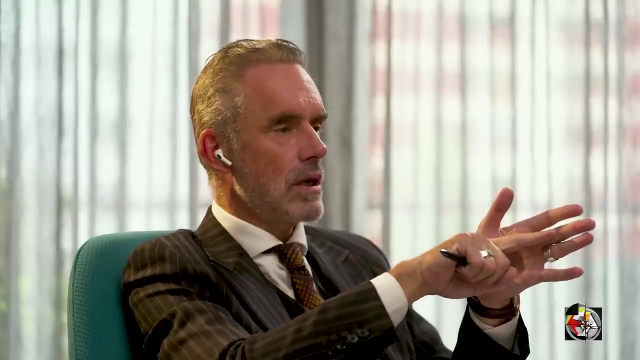 on what might constitute a universal higher order ethical narrative. And if you imagine that interactions with people are generally constrained by the necessity of iterating the interactions across time, And then you might say by the additional constraint of iterating the interactions across time so that they increase in their utility. 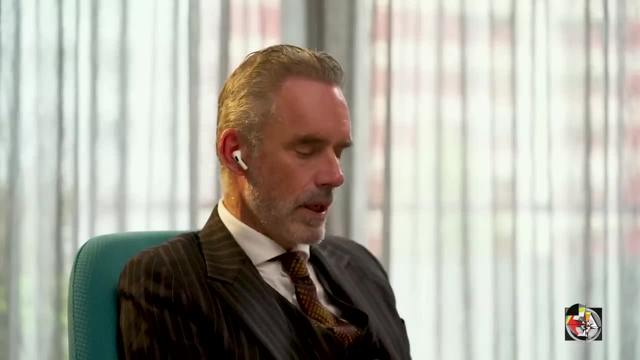 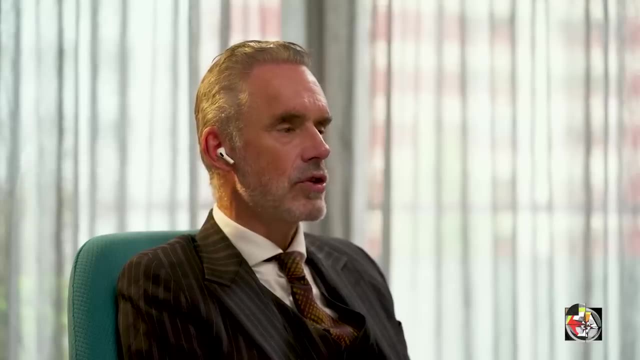 And so then you might say: well, how do you have to treat someone- or everyone for that matter- so that that reality makes itself manifest as you move forward into the future? And I would say, well, that looks like something like genuine altruism. 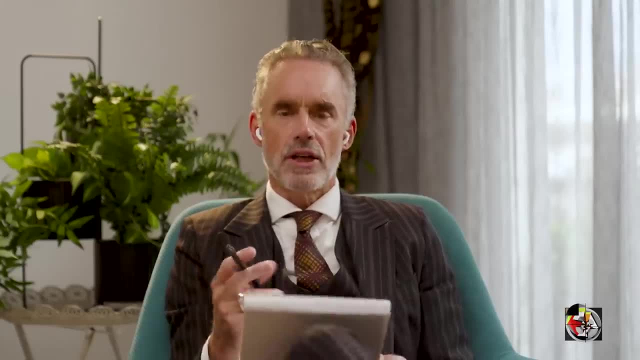 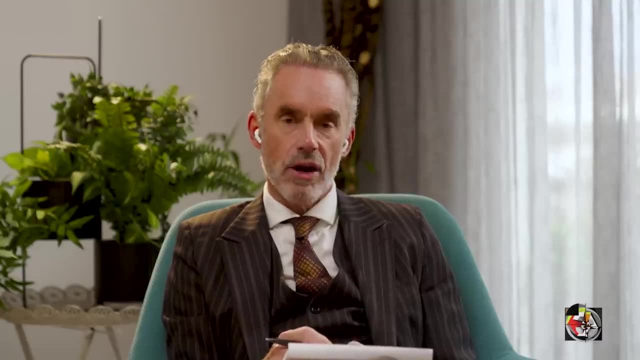 It's like genuine altruistic reciprocity. Now, Franz de Waal. I had a chance to talk to Franz de Waal about his work with chimpanzees. You know, when chimpanzee alpha males are often parodied as dominant, in a sort of Marxist sense, power-driven. 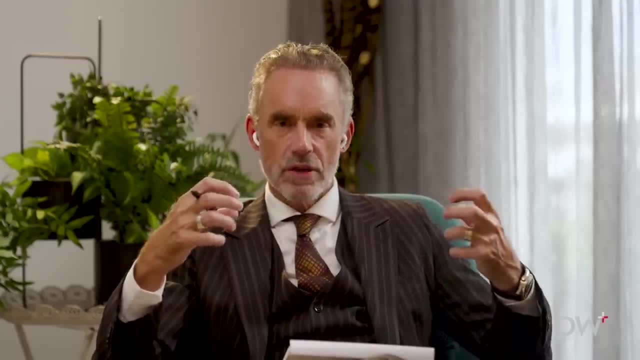 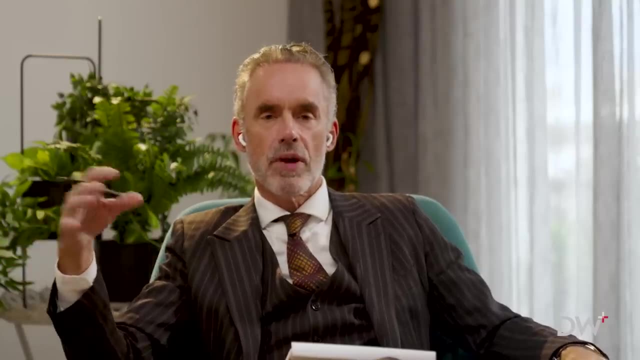 And it's the most dominant male chimps, so the one with the most physical prowess, the biggest tyrant in some sense, who gets to dominate all the other chimps and who, in consequence, has preferential reproductive access. And so it's a theory. 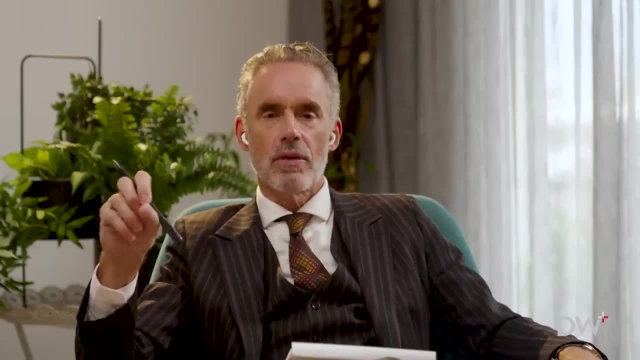 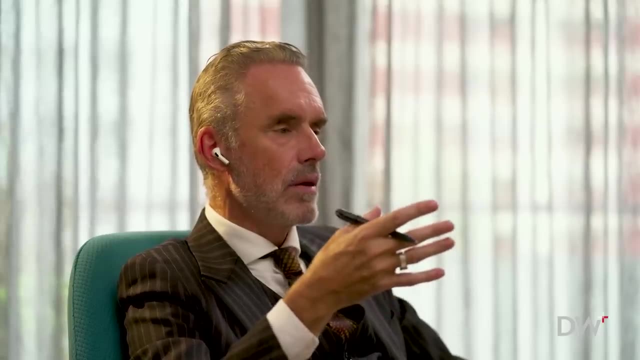 it's a theory of power and social structure and reproduction all tangled up into one. But the problem with that is: it's not true. So de Waal has shown very, very clearly that first of all, sometimes the alpha chimps, so to speak. 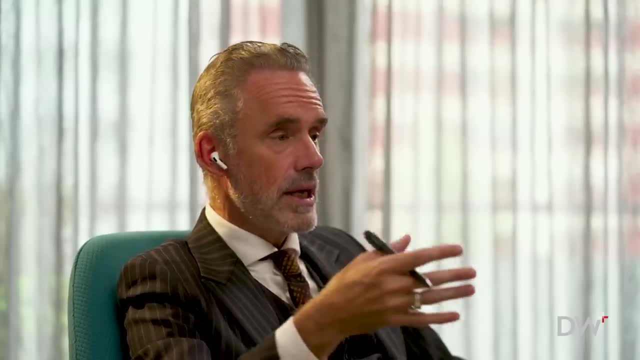 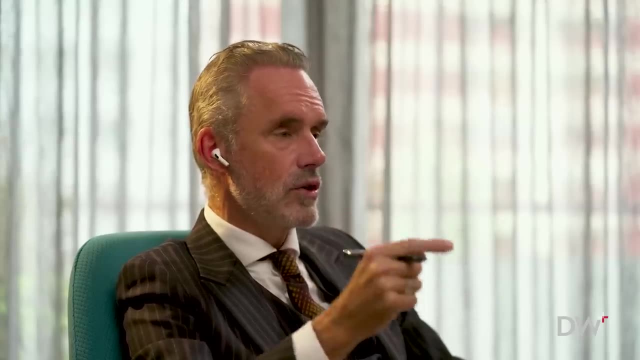 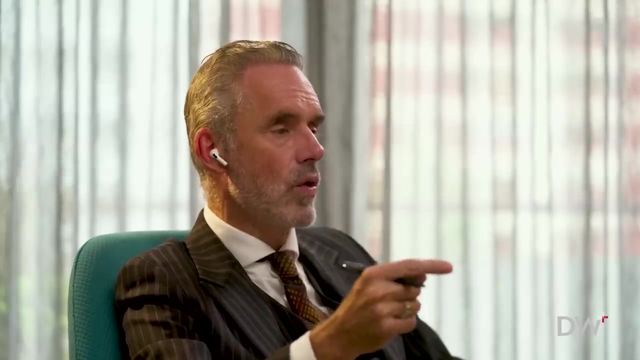 can be the smallest male in the troop. Frequently he's allied with a powerful female and he is generally the most reciprocal individual in the troop, very concerned with the long-term maintenance of social relations and very good at maintaining social relations. He's very good at making peace, not war. 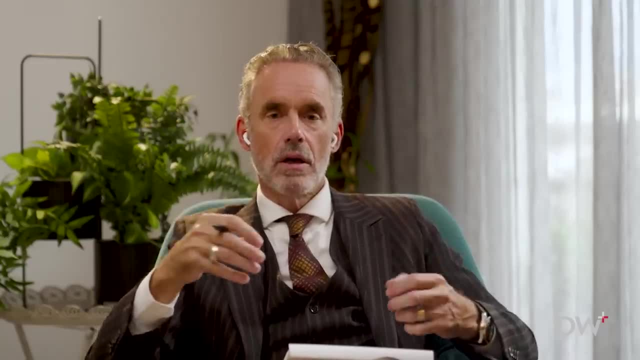 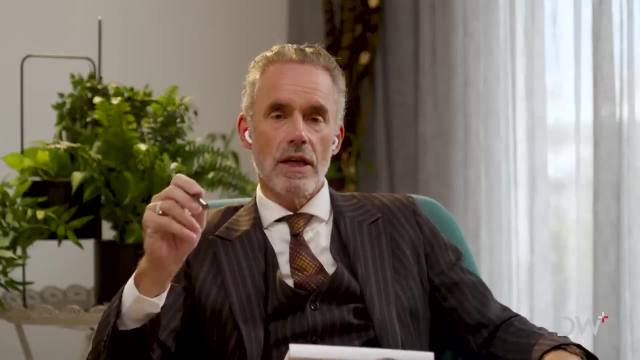 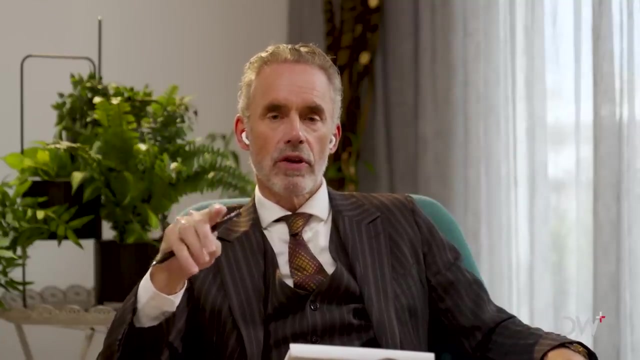 Now that doesn't mean he doesn't have- let's call it- power at his disposal, especially in coalitions, if necessary. But de Waal has shown very clearly that the alpha chimps who rely on power and force are very likely to rule over an unstable polity. 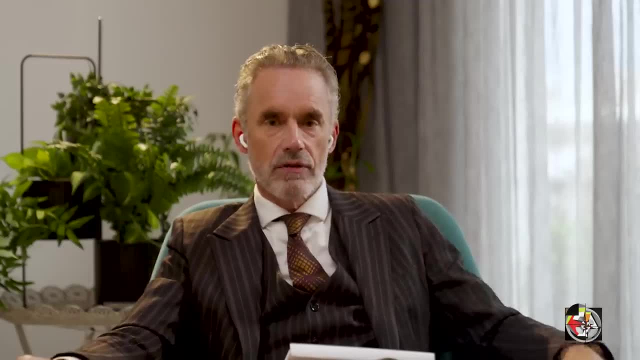 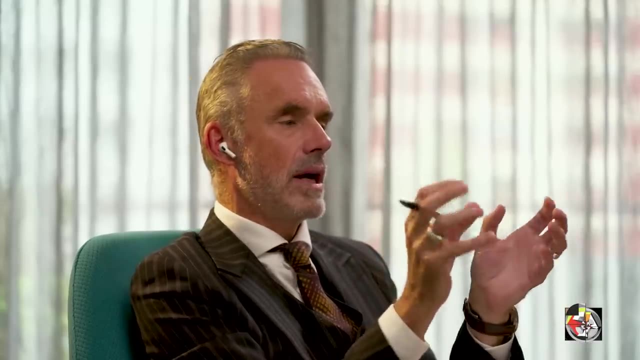 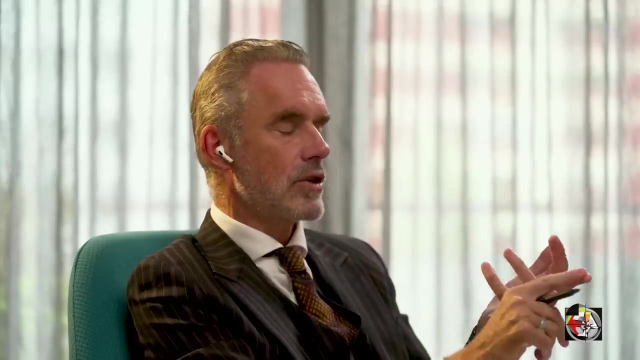 and to meet an extremely violent end in the relatively short term. And so if your fantasy about the future, let's say, is motivated by an underlying motivational state, it could be hunger, it could be thirst, it could be sexual need, it could be rage. 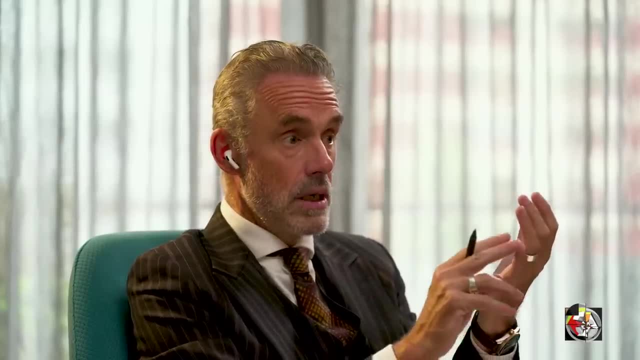 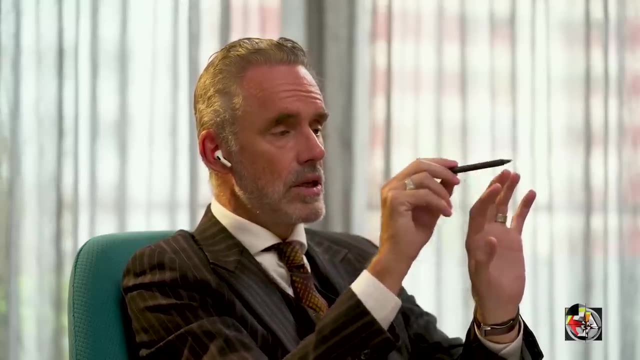 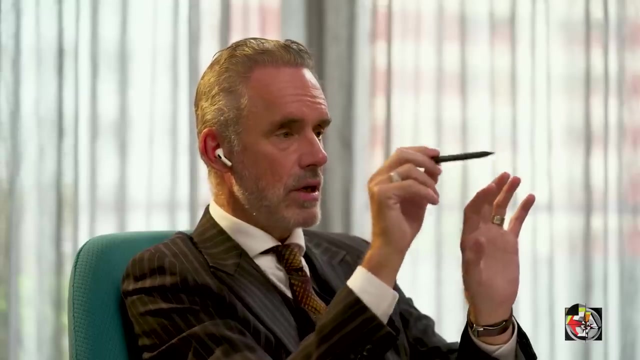 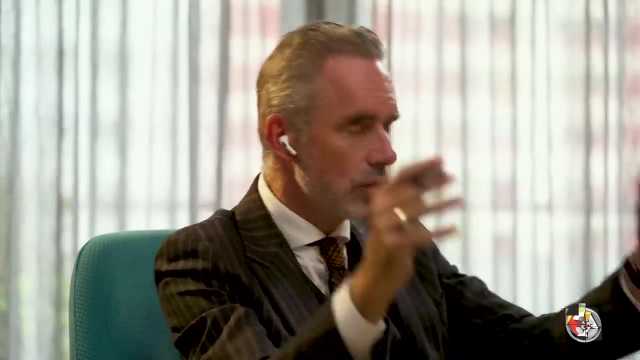 it could be the desire to make anxiety decrease. then you could imagine that there are ways of interacting in the world that satisfy multiple motivational states simultaneously, And then you could imagine that those modes of being satisfy multiple states of motivation simultaneously in a social context. 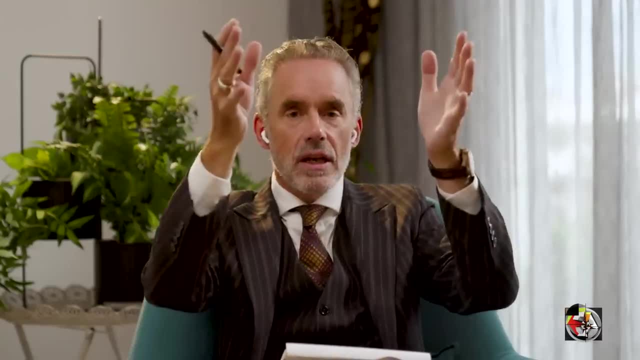 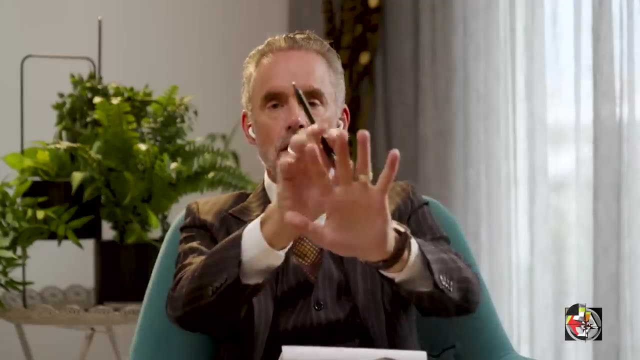 so also for other people. And then you could say: and that make that occur as it iterates forward into the future. And then you could say: well, you want to extract out a representation that allows you all those advantages simultaneously. And it looks to me like something. 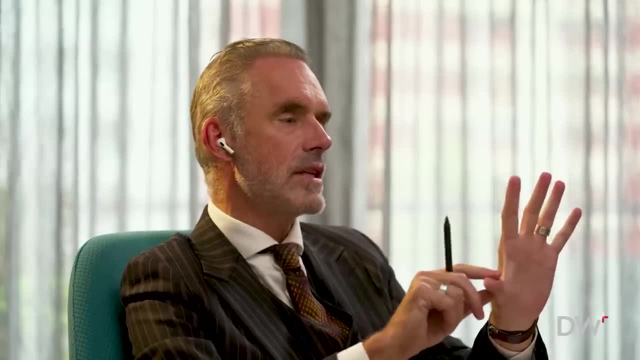 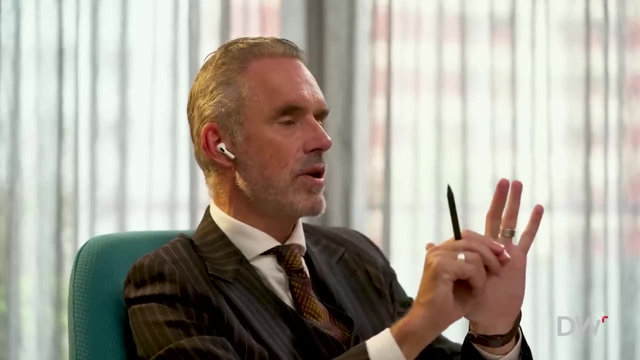 maybe that's marked. here's some hypotheses. It's marked by the sense of active engagement that you might have in a good conversation. It's marked by the sense of the emergence of the spirit of play, And Jaak Panksepp has detailed out. 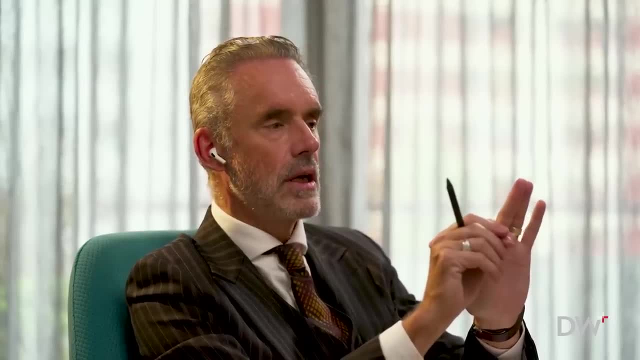 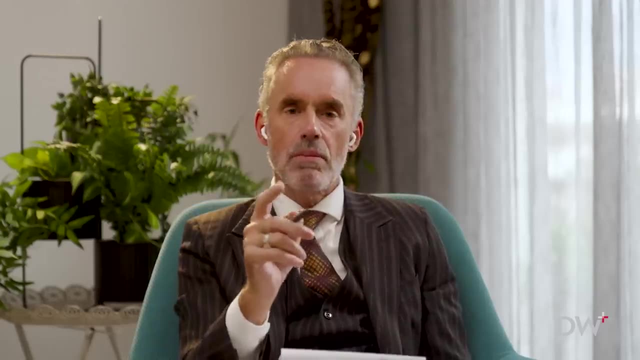 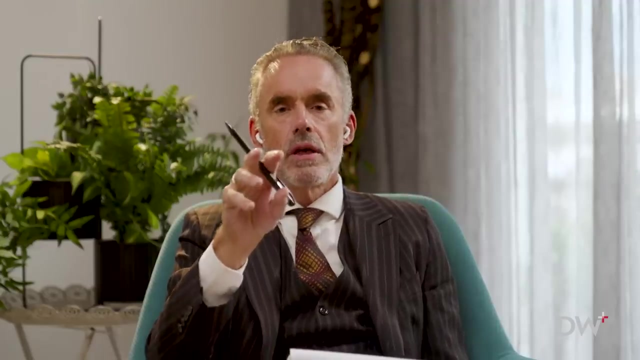 the psychophysiological structures underlying the play circuit. It would underlie something like maximal- no optimized- stress. So you talked about minimizing predictive error. but here's a variant: What if you optimize predictive error so that you lay out a fantasy on the future? 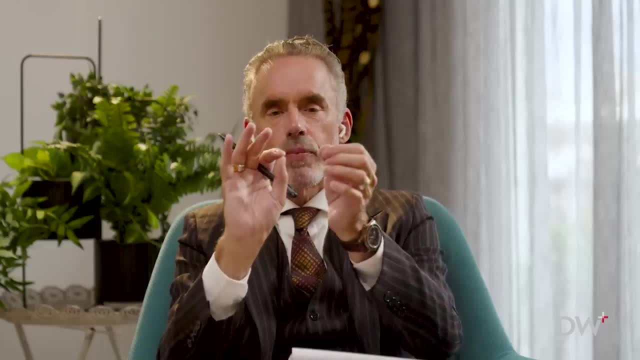 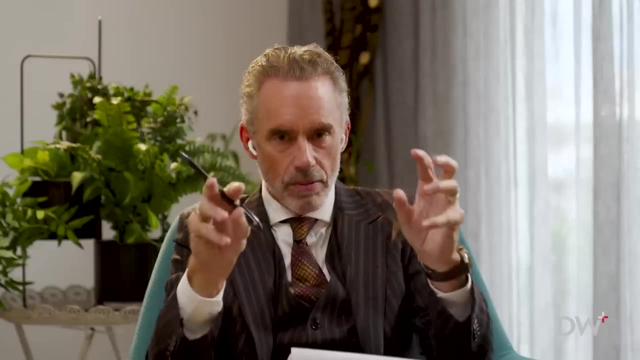 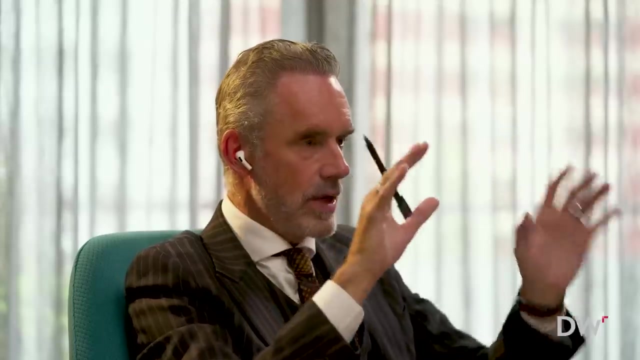 and then work so that there's just enough predictive error so that you encounter something you don't expect at a micro level, small enough that you can manage it, but large enough so that it expands the confines of your hierarchical presuppositions. And maybe you do that. 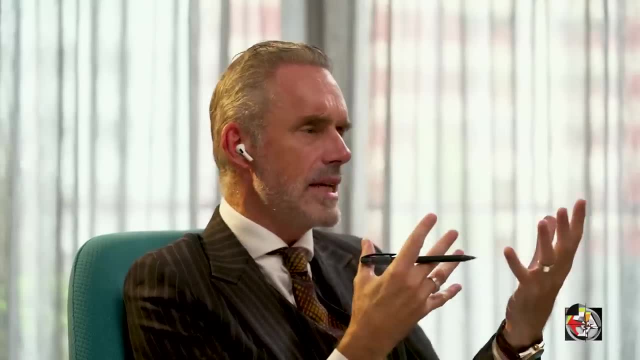 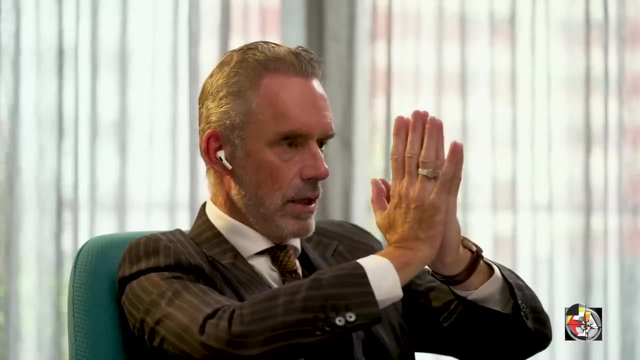 See, I was thinking about that relationship to play, because if you're on a team and you're playing against a well-matched opponent, the opponent pushes you right to the limit of your skill, not past it, so it's not too stressful. 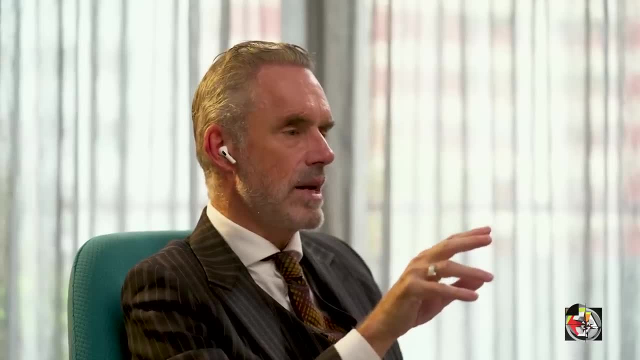 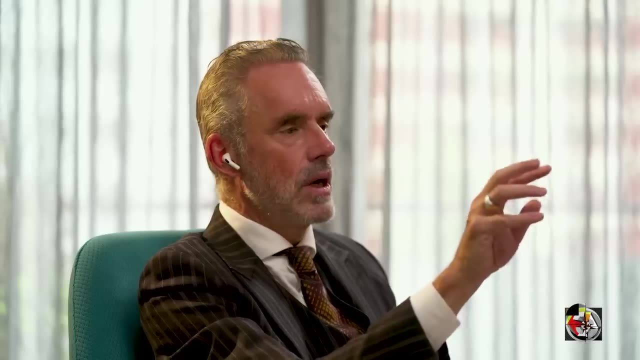 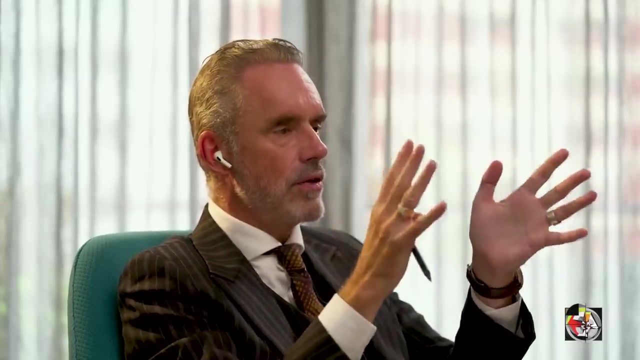 but it isn't exactly in that situation that surprise is minimized. It's more like a little entropy is allowed to enter the system at just enough rate and intensity so that you can push your development in a manner that doesn't stress you too badly physiologically. 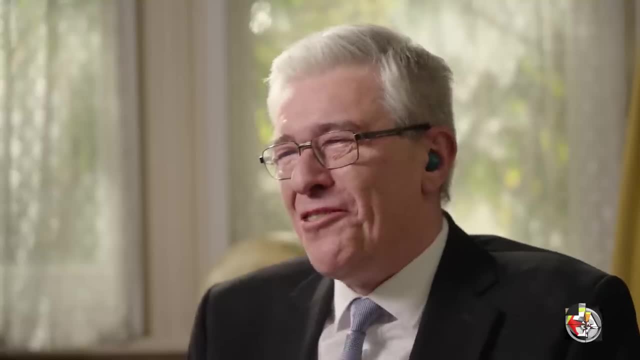 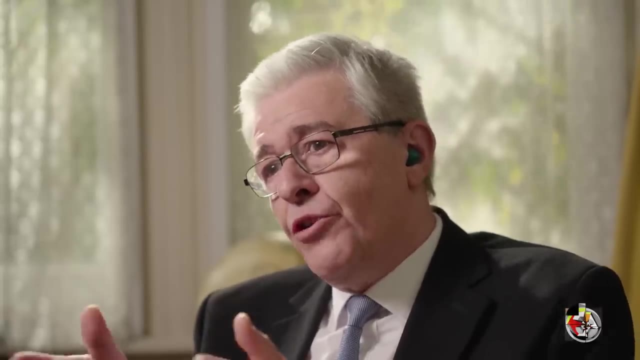 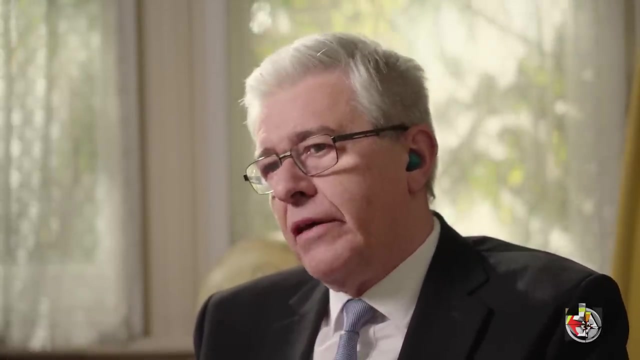 Yeah, So you brought it about sort of four really important themes here. The two key things that you've brought to the table there were sort of putting sentient creatures together. So you're talking about social interactions now and social hierarchism and sense-making. 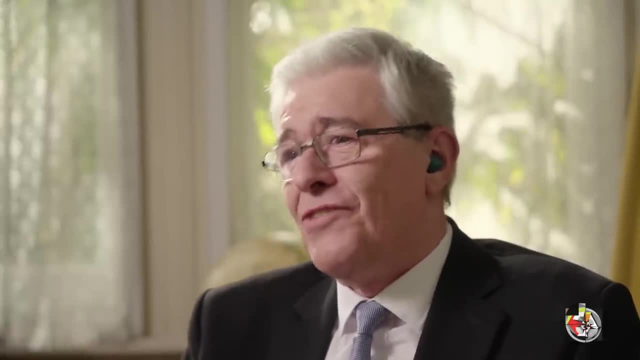 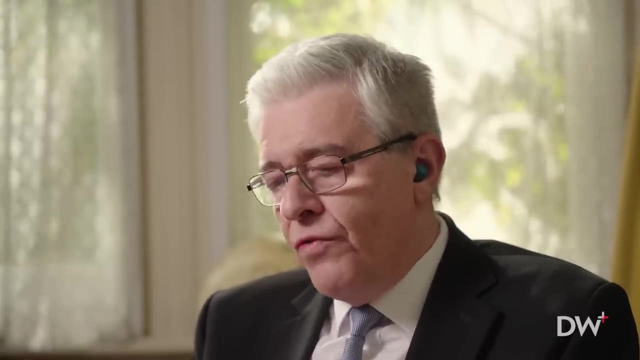 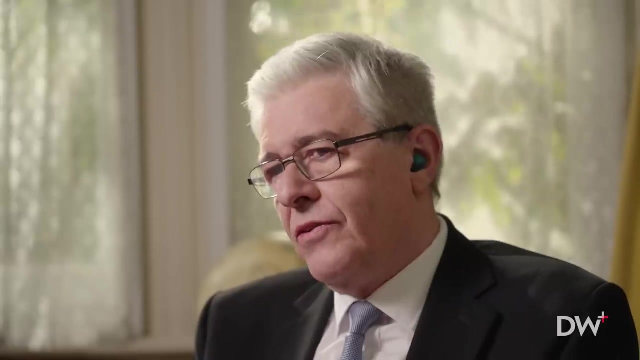 when the other- the thing I'm making sense about- is also trying to make sense of me. I think that's a really important sort of and challenging sort of move there. You've also brought to this sort of highlighted, this paradox that you know. 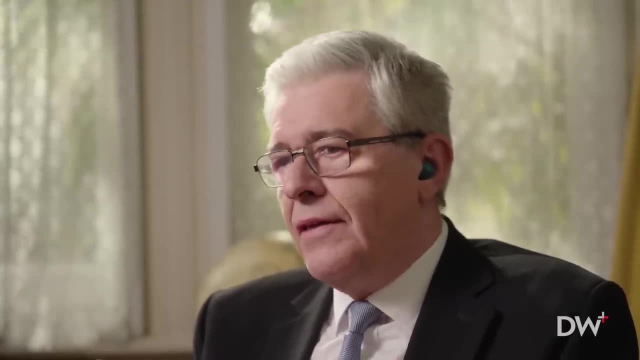 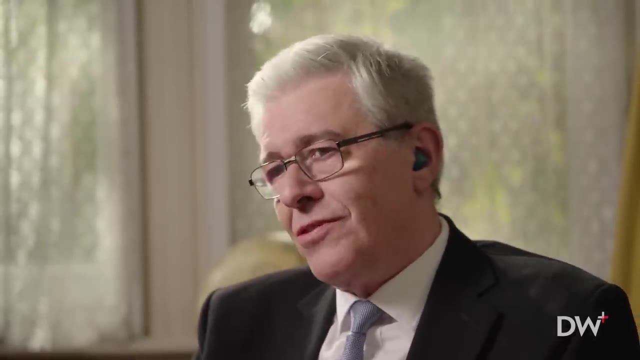 we might be in the game, or we might be seen as in the game- of trying to minimize our surprise, minimize our prediction errors, and yet we seek out novelty. So I think there's a fundamental paradox there that needs resolving. I think you've 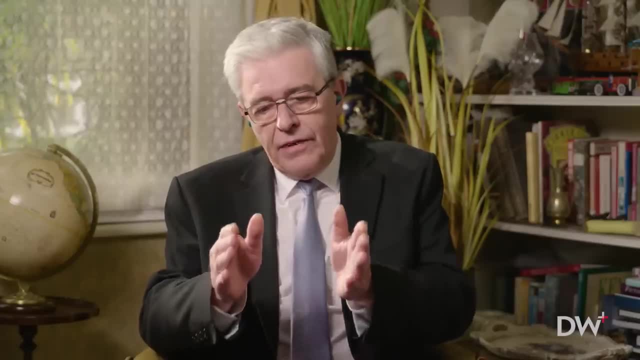 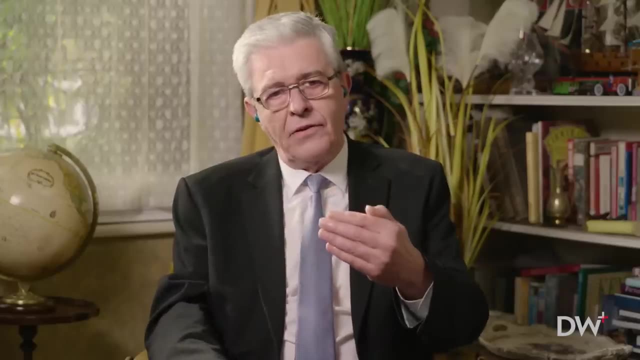 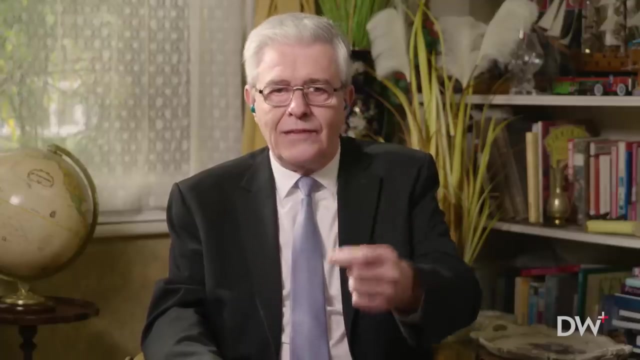 in your setting up of the issue, I think you've implicitly resolved it. There is, I think, a very simple way of resolving that, And it comes back to this sort of isomorphism between expected surprise and uncertainty. And I notice you also use the word angst and anxiety. 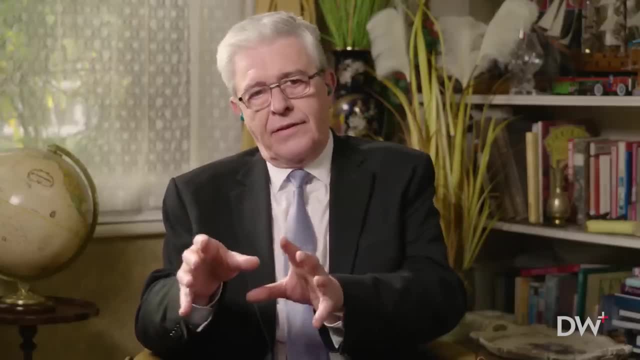 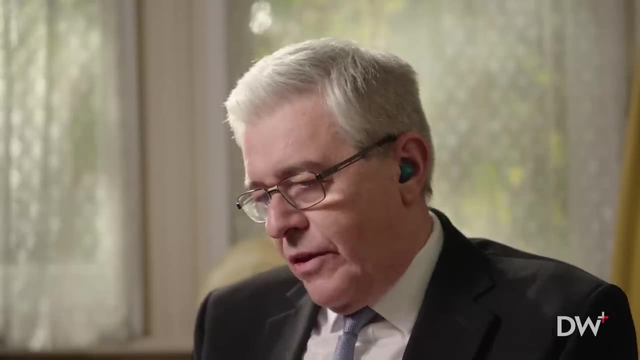 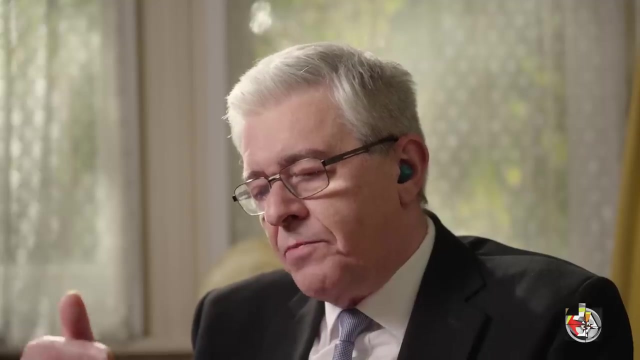 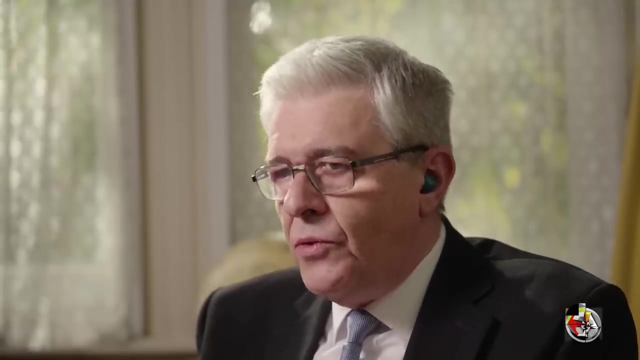 To my mind, uncertainty just is a state of, or recognized as a state of, angst or anxiety. So you know, that sort of imperative to minimize expected surprise just is choosing, or can be complied with by choosing, those plans that minimize uncertainty. And what would that look like? 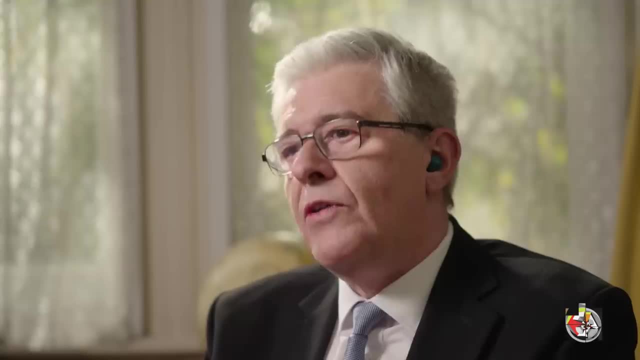 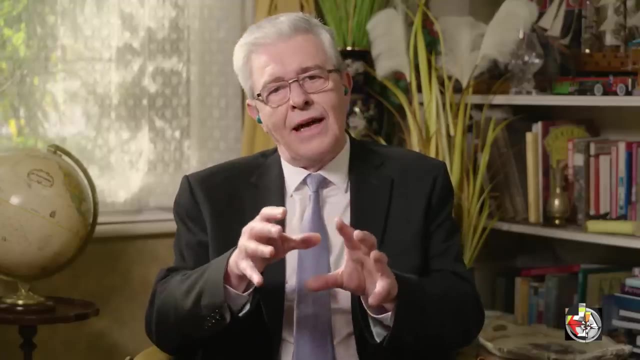 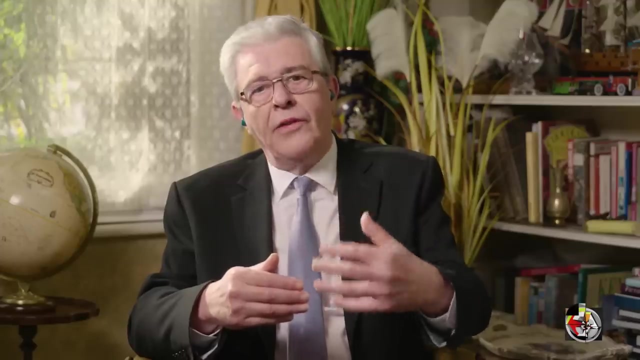 It would basically look like responding to epistemic affordances that resolve that uncertainty. So I think that's the kind of surprise that we aspire to. It's the novelty that affords the opportunity to resolve uncertainty and thereby resolve angst. And if that's true, 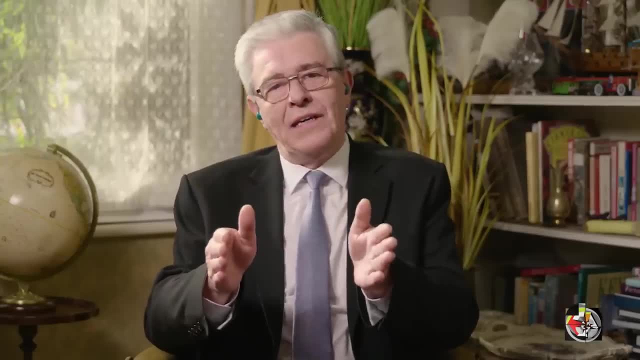 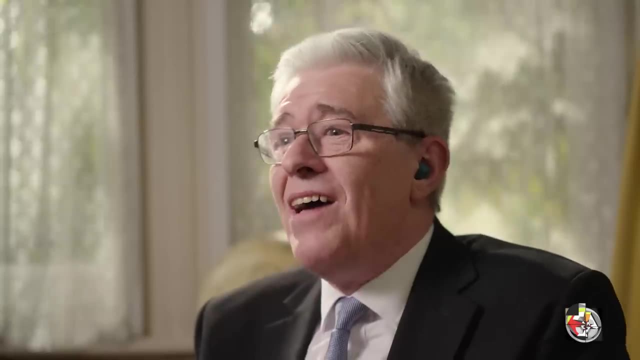 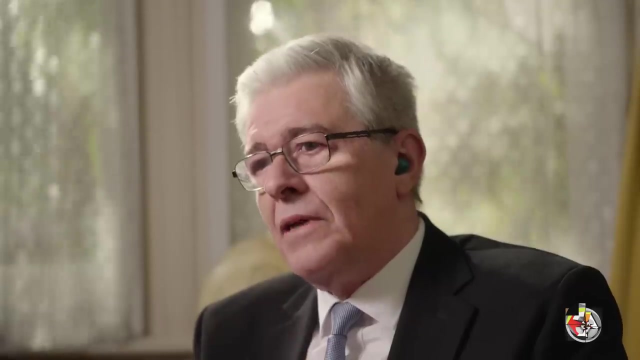 then taking it to your context, how would I do that If I was in a social hierarchy of chimpanzees or I was in any social setting? In one sense, the simplest way to resolve my surprise and make the world as predictable as possible. 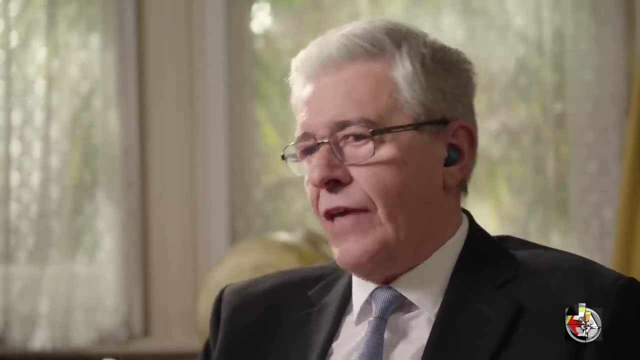 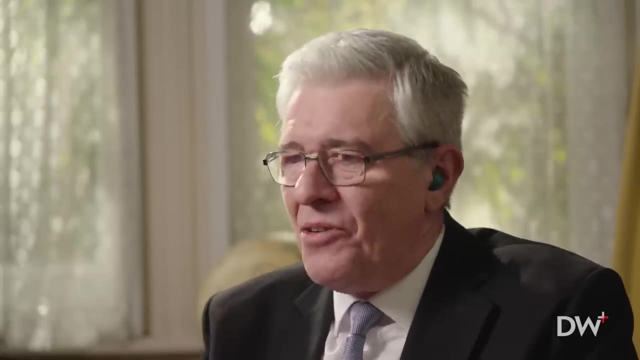 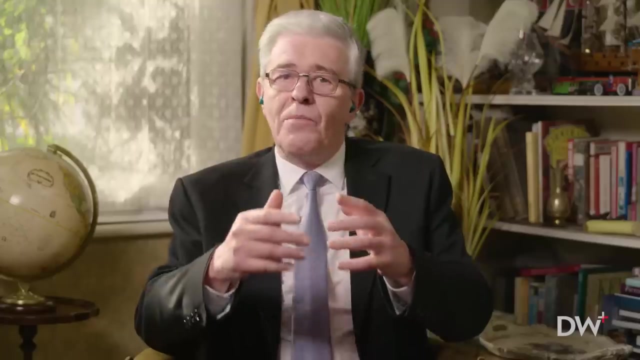 would initially be to resolve my uncertainty about you by asking you the right kinds of questions. that allows me to sort of put you in a particular category in one of my narratives, in one of my narratives, my pro-social narratives about the kinds of people that I can talk about. 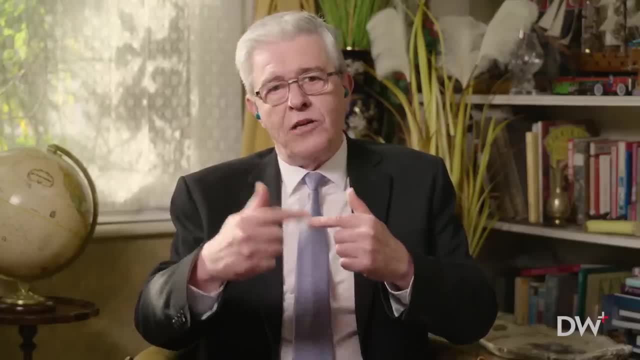 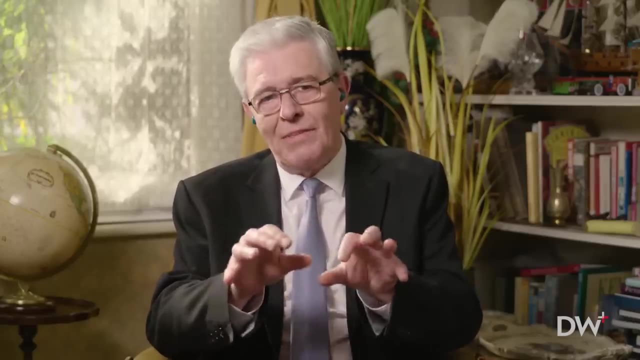 But also, ultimately, I'm going to try and make you like me, or make me like you, Because the closer we are if we can share the same narratives and the same language, then together we're mutually predictable. So that mathematically would be. 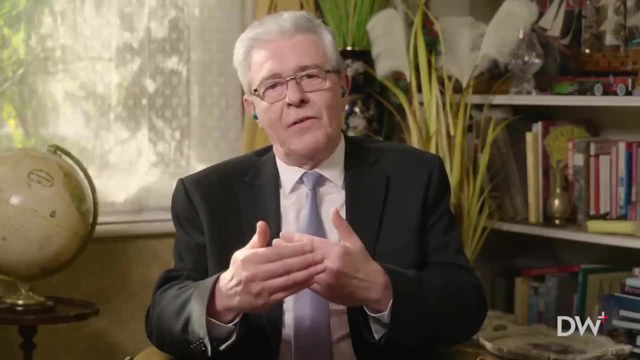 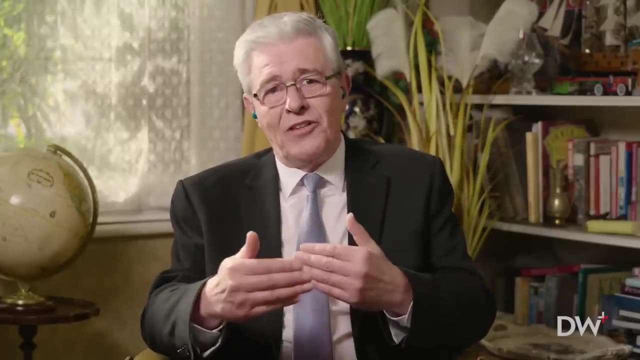 sort of like a generalized synchrony, but from a social neuroscience perspective on dynamic interactions, it's basically aligning ourselves. It's basically aligning ourselves So that we come to know each other and that we can dance and synchronize and exchange. And after a while, 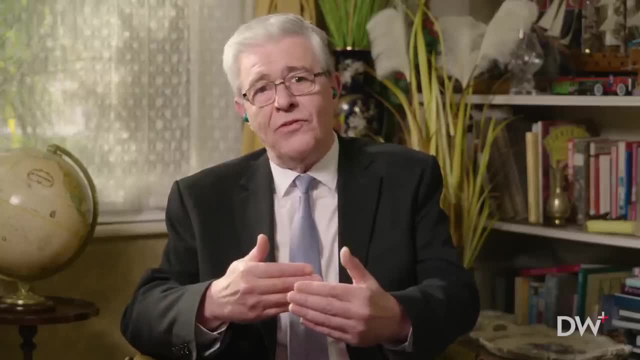 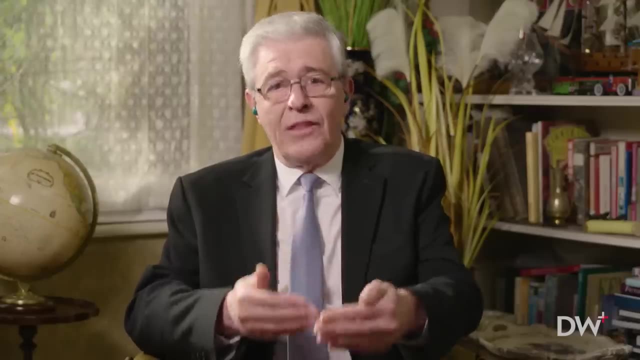 I don't need to ask you any more questions, and you don't need to ask me any more questions. We are now on the same page, singing from the same hymn sheet, the same generative model, the same world model, the same kinds of narratives. 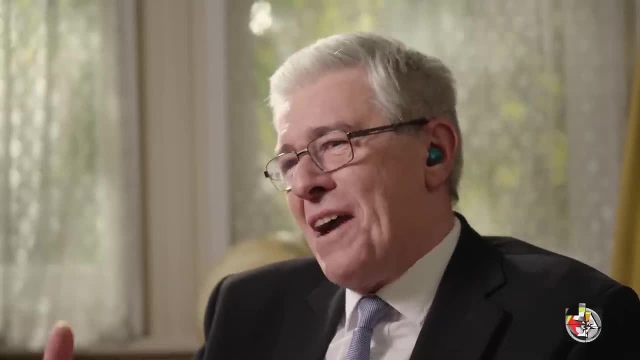 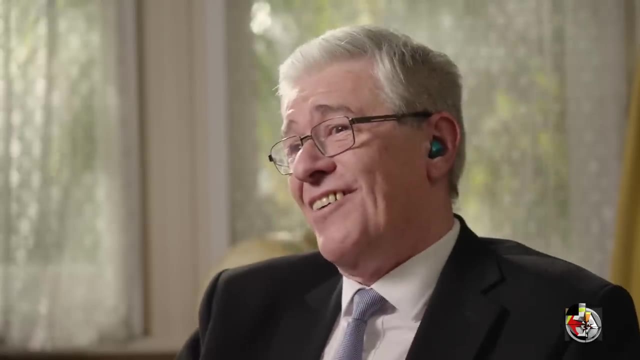 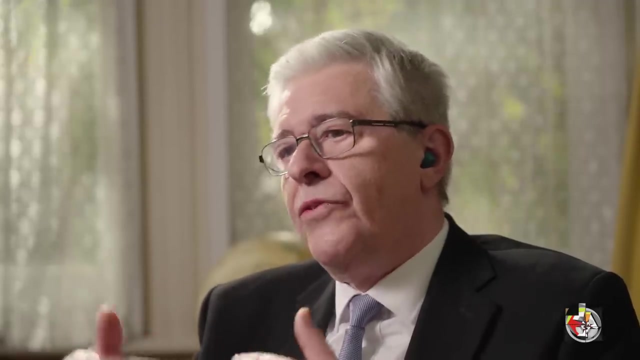 Having said that, of course, there's also, in the background, the putative or potential novelty of finding out what somebody's not like me like you know. So you know, I think, asking questions about the right kinds of narrative that resolve uncertainty. 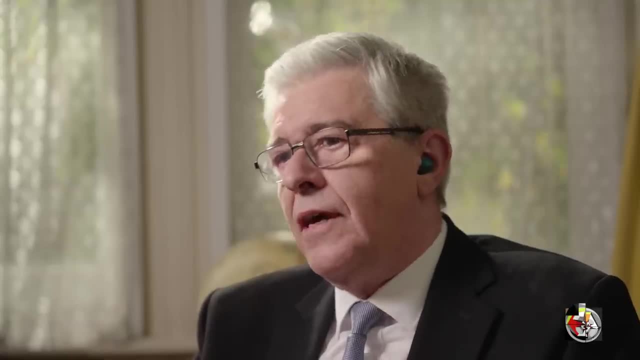 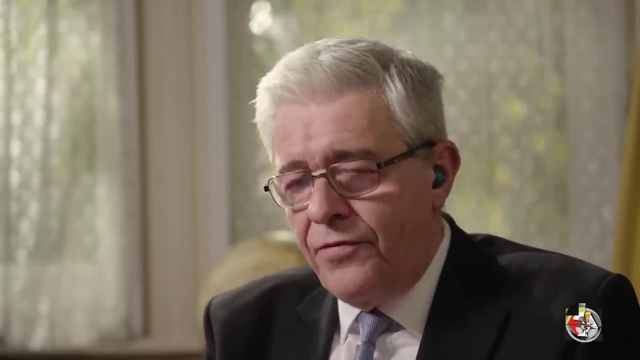 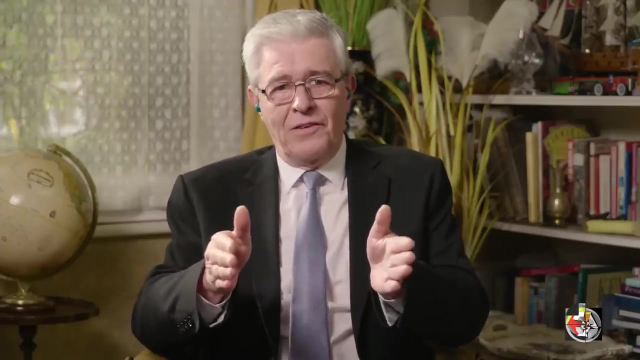 responding to epistemic affordance, novelty seeking, information seeking, whilst at the same time still avoiding those surprising states of loss or physiological extremists. put that into a social context And I think you've got some really, really good answers. 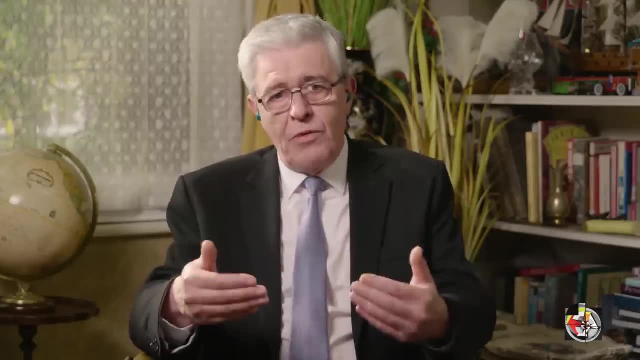 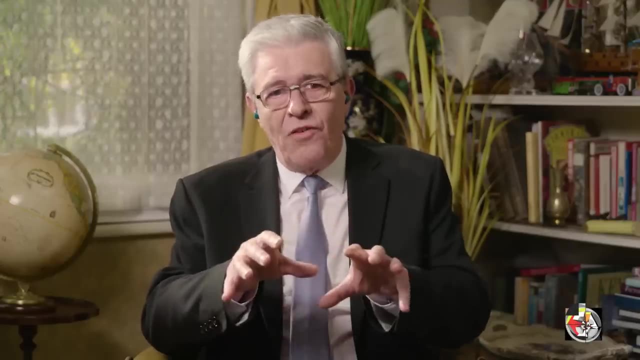 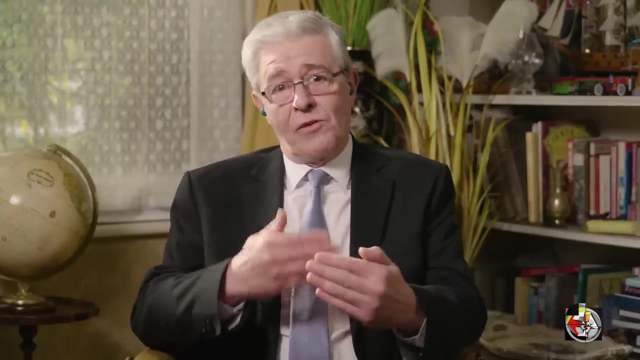 I think you've got some really interesting questions and possibly a structure and a framework to understand social organization and sort of information exchange and self-organization, not at the level of just the individual negotiating with his or her body but negotiating with another individual with a very similar kind of body. 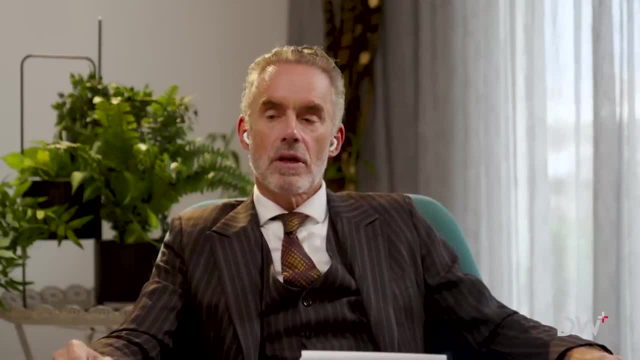 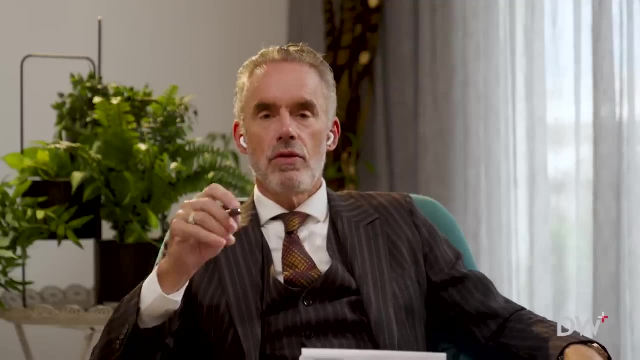 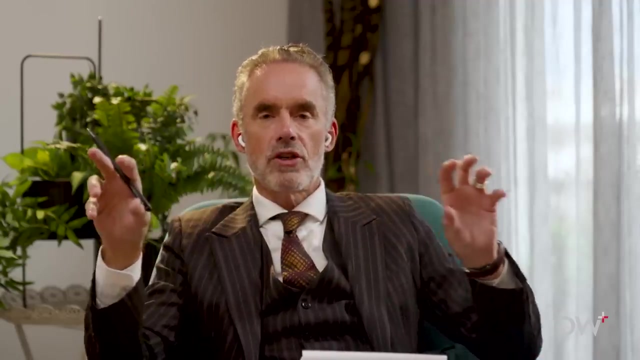 I spent a lot of time studying Jean Piaget and his description of how people organize themselves across time, And you might imagine a two-year-old as a collection of micro narratives, each of which are driven by a somewhat independent motivational state, And so two-year-olds will cycle. 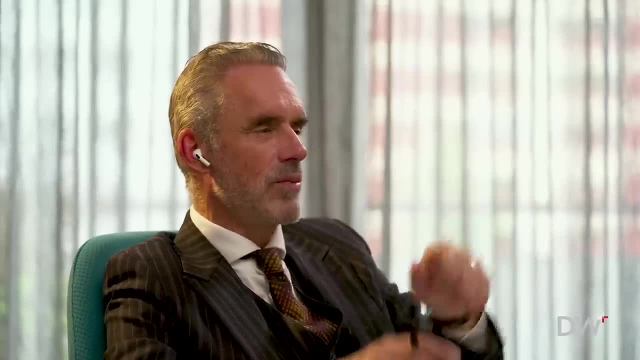 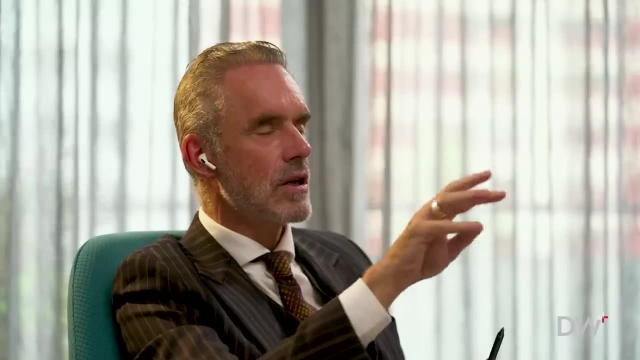 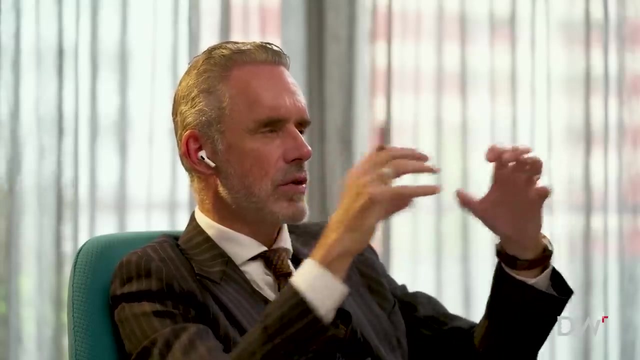 between being too hot and too cold and too tired and too playful and too enthusiastic and too anxious, without any real overarching integration. And they start to manifest that ability to integrate those already integrated motivational states which are probably in large part hypothalamically controlled. 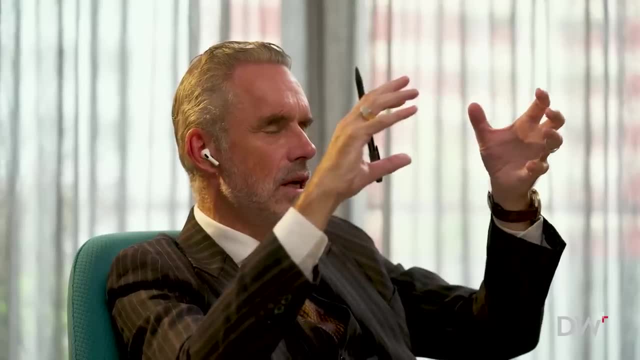 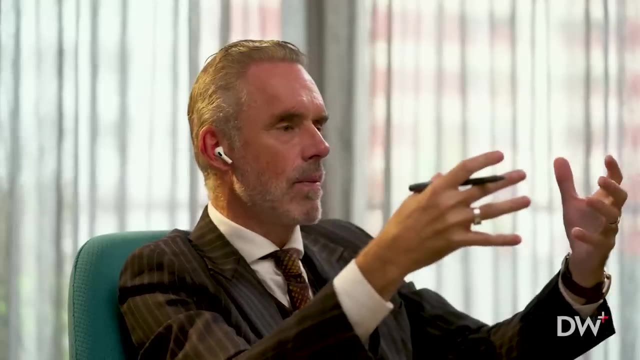 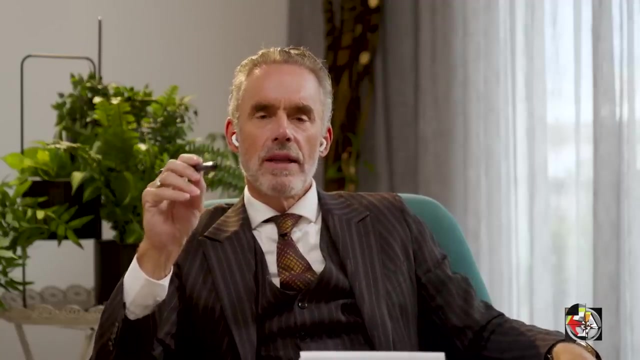 They start to be able to integrate those into a continuous narrative through time and in different locales, at two And so then they start to be able to play by themselves And so, but it's at three or thereabouts when they can adopt a shared narrative with someone else. 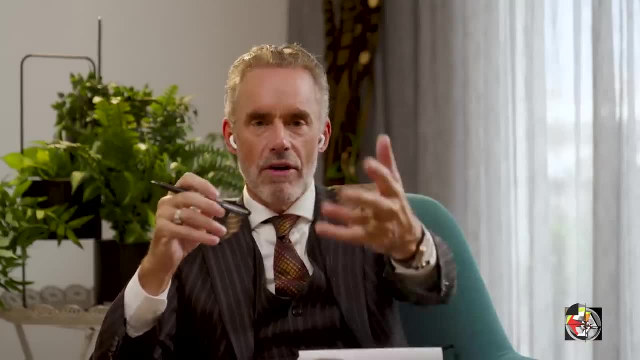 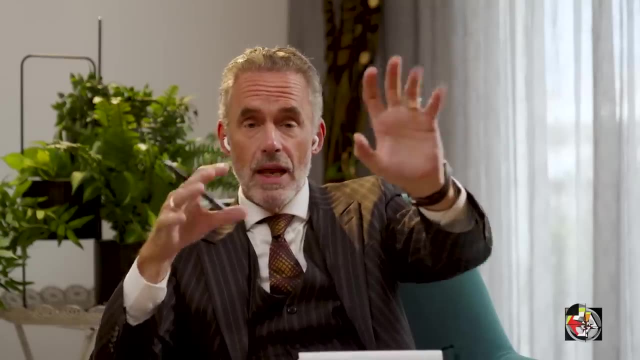 So a little boy and a little girl might get together and the little boy will offer to play, or the little girl and say, would you like to play house? And so that specifies the goal, And then the little girl has to say yes. 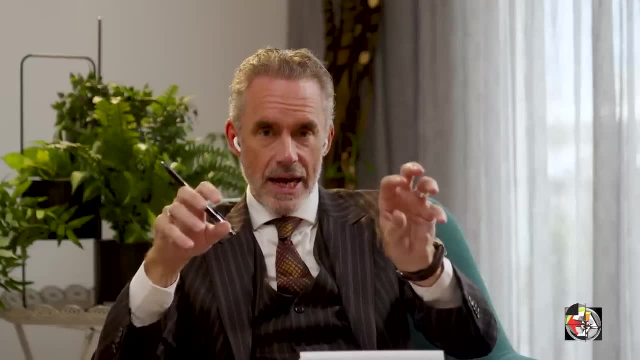 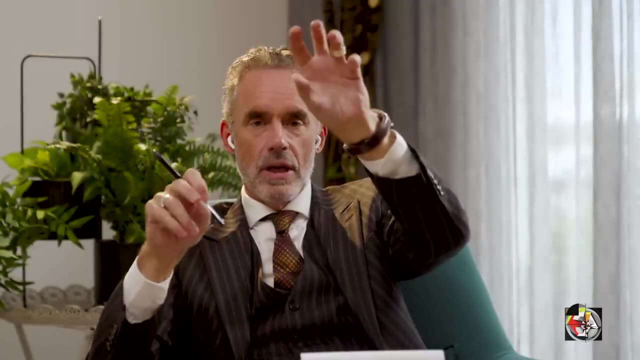 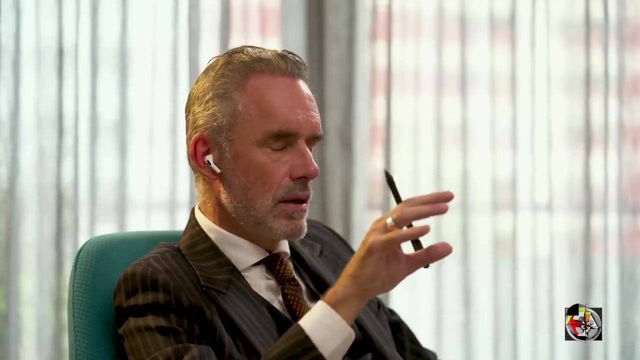 it has to be voluntary. And then the little boy might say: well, I'll be the dad and you be the mom, And then they can integrate their two identities within that overarching concept And so they can develop mutual understanding that way, And it's partly because you said earlier, 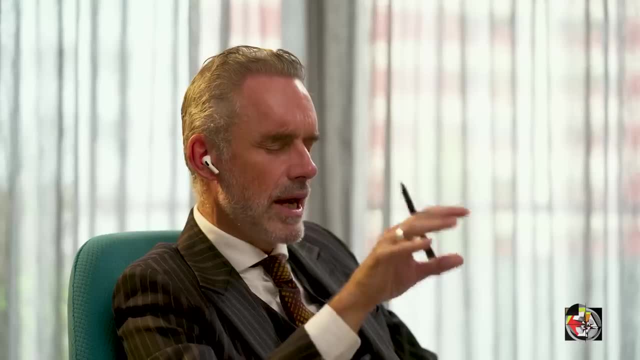 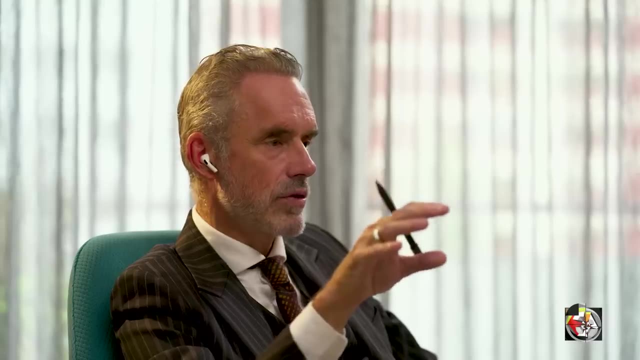 that the best way to make someone else happy, someone else predictable, and you to them, which is also equally useful in some sense- is to be inhabited by the same conceptual structure, And that's sort of what we do when we decide to play a game together. 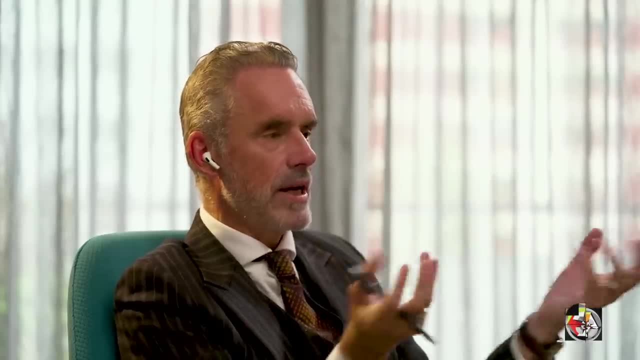 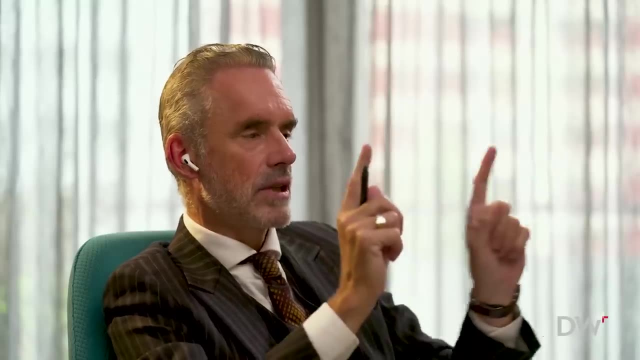 It's like: here's the game, Here are the principles by which we're going to operate, Those are the rules of the game, And if you're operating by those principles and I'm operating by those principles simultaneously, then we're going to share a perceptual reality, because that's 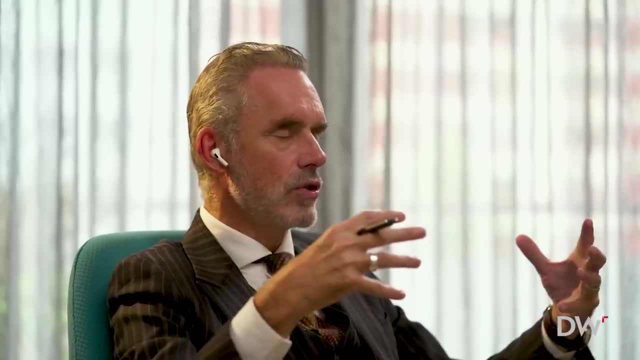 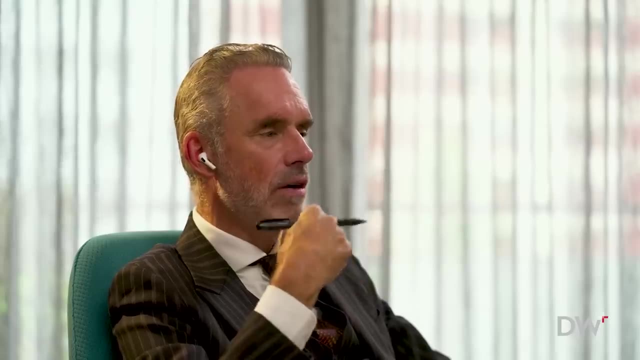 instantiated in relationship to the game And we're going to share emotional response, And so I can now predict you if you're playing the same game, merely by reading off of me, because the same thing, And I think this is what we do when we go to a movie. 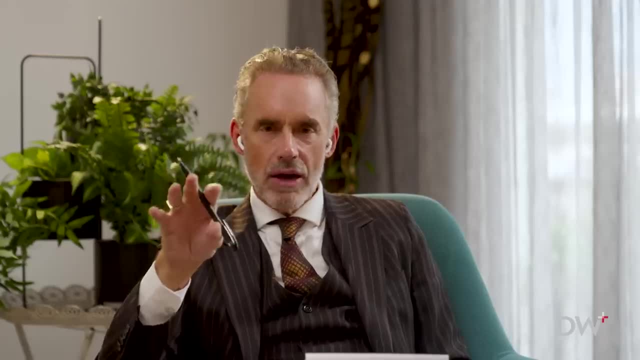 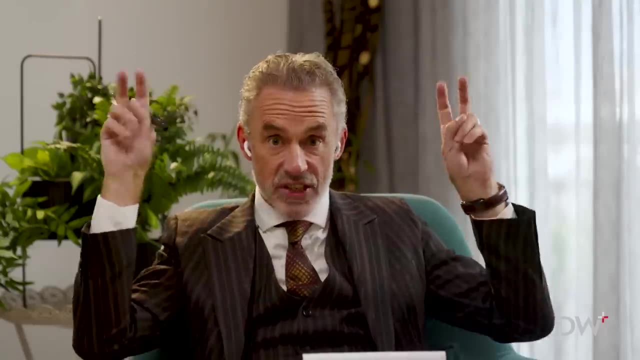 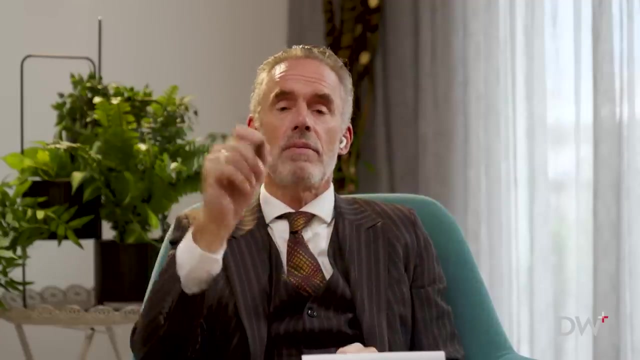 and we watch the hero, We adopt his hierarchy of attentional prioritization And then we can feel the same emotions because we're in the same state and we really are like. neurophysiologically We're in an analogous state, And then the understanding comes- not from me deriving inferences- 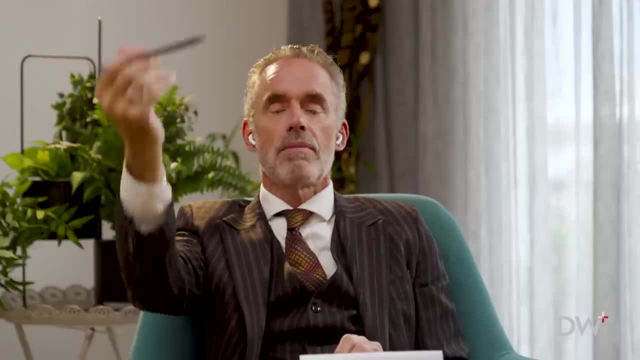 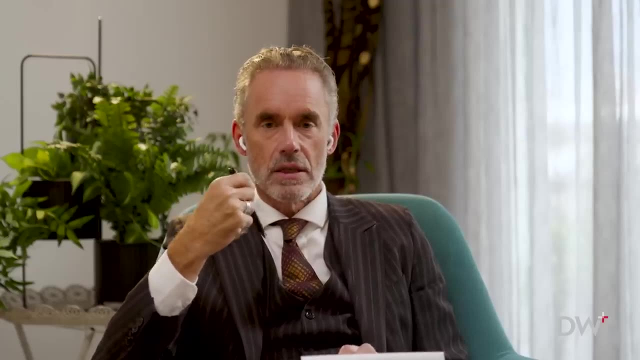 about the character's motivations because of his actions, but by me adopting his goal or his story and then reading off the emotions I have, which are now isomorphic with his, And I think children are doing the same thing when they play a game. 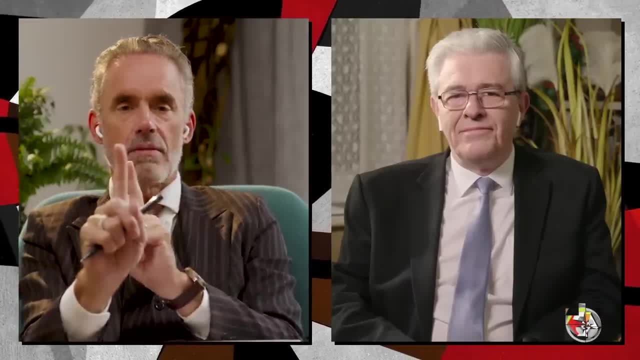 And I would say that you and I- insofar as we're playing the same game in this conversation- are very likely to remain predictable to one another, And I think that's what we're going to do, And I think that's what we're going to do. 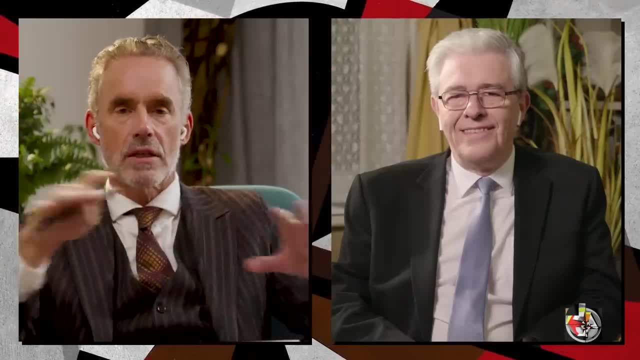 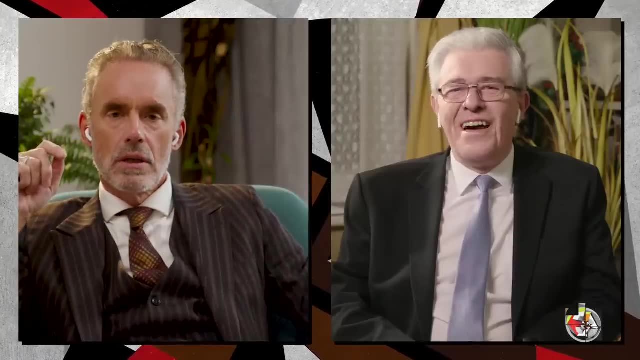 And I think that's what we're going to do- And also to occupy the same emotional states simultaneously, similar, at least Similar enough, so we're not jarring and off-putting to each other. Yes, I wanted to say that. 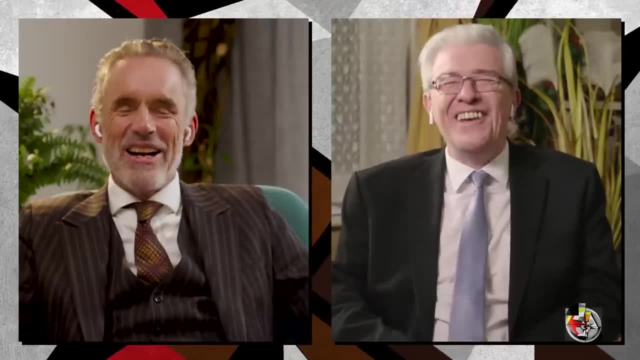 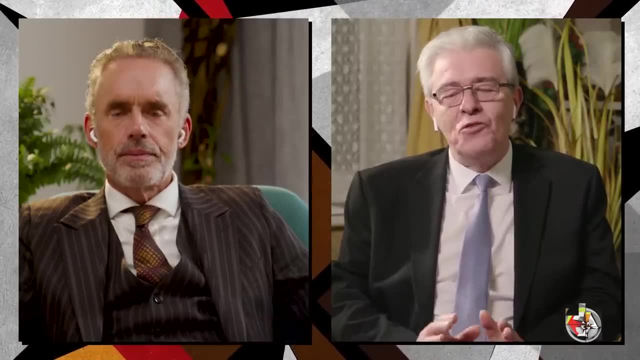 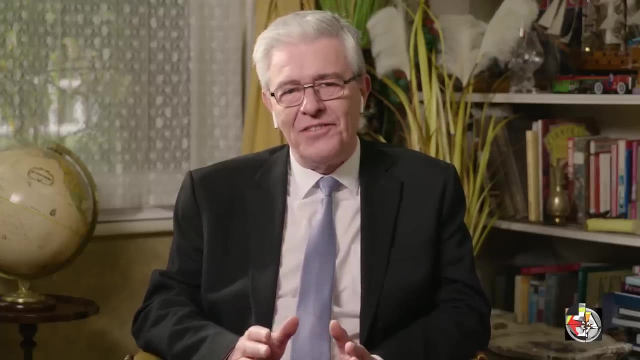 So the shared narrative is. I think that's a perfect example of a shared narrative, And you crucially point out that you're talking about theory of mind, And one of the easiest ways to get to theory of mind is It's just to commit to the hypothesis that you are very much like me. 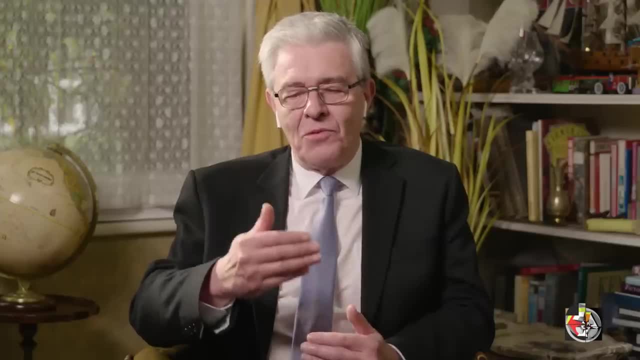 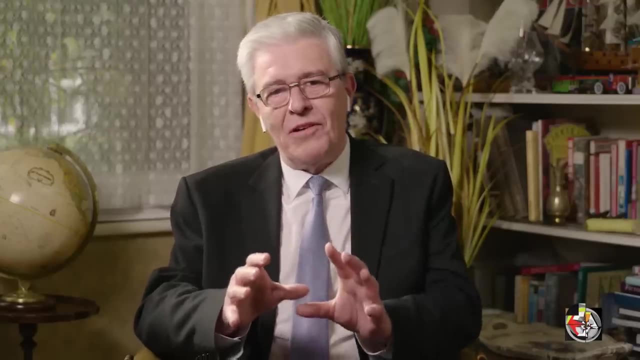 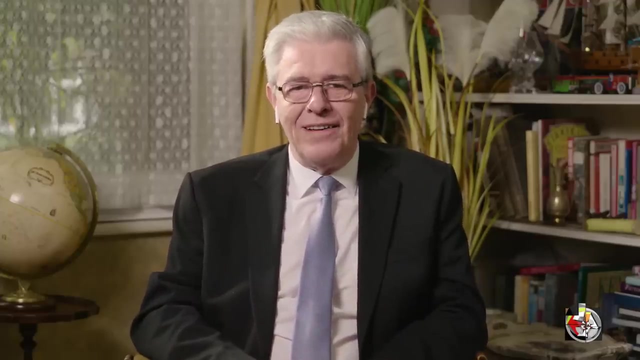 So what I would feel if I sensed what you sensed is going to be a very good proxy for my inference about your feelings, And, of course, making inferences about you just is theory of mind. I also wonder whether you were going to develop that argument. 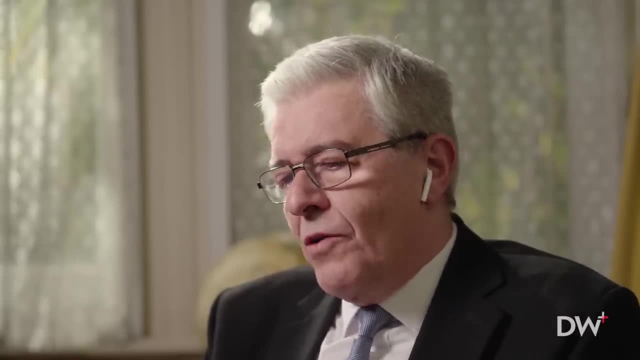 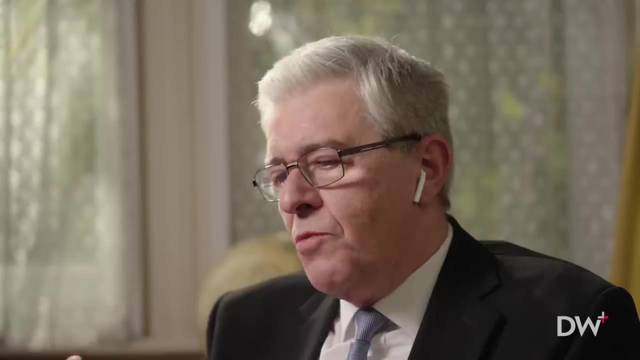 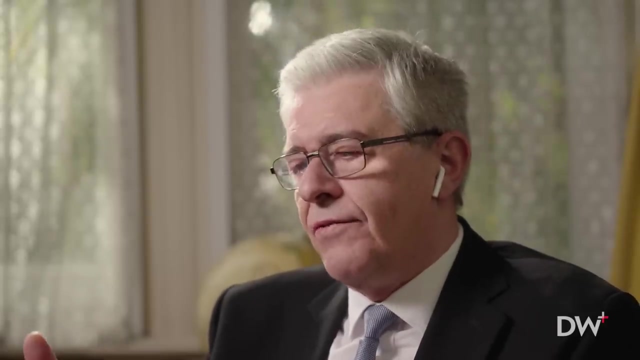 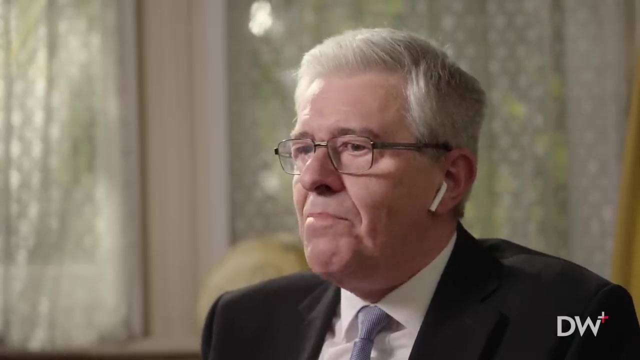 almost pre-stages of Piangetian development, just to how a newborn infant starts to make sense of its world and the very emergence of selfhood. that self is distinct from mum or the rest of the world. Getting into notions of motor babbling. 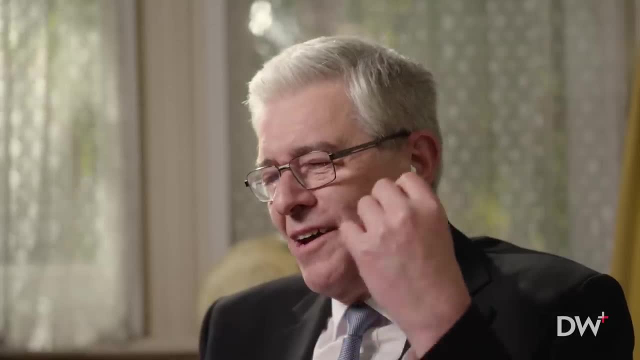 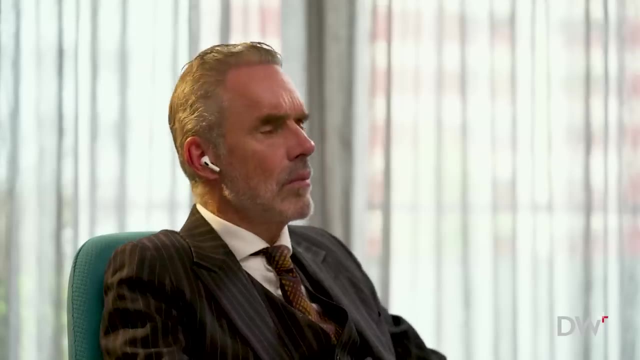 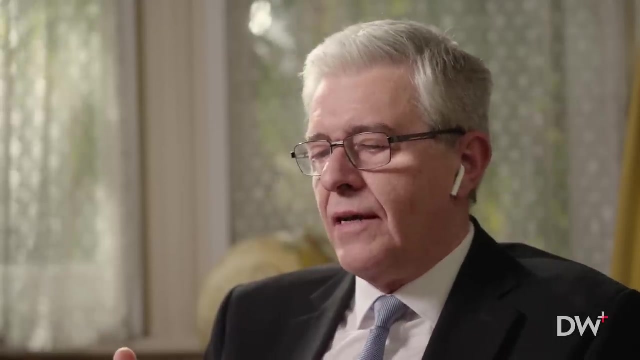 you know, babies that will rattle their children, toys to say yes, I caused that, as opposed to mum causing that. So you know, I think that what you're talking about the Newmont being the ability to actually recognise. 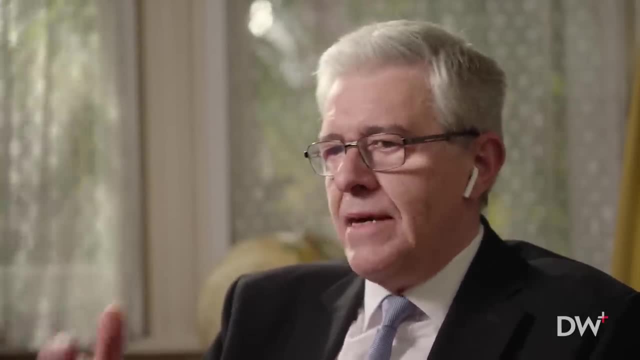 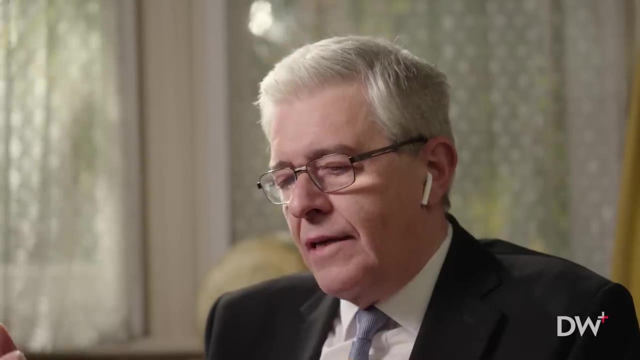 oh, you are another that is like me, And if we can share the same narrative, then there is not only a deep connection and a communication, but also a very sophisticated theory of mind. That would be the Newmont, But en route. 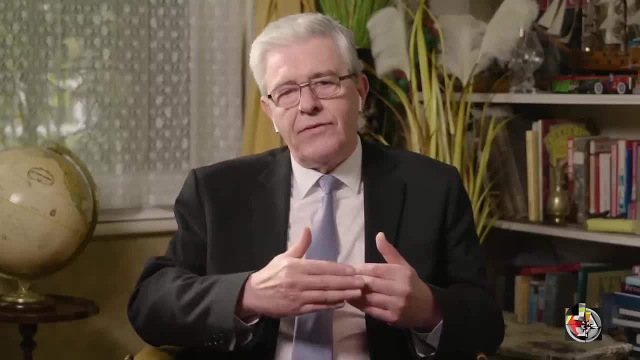 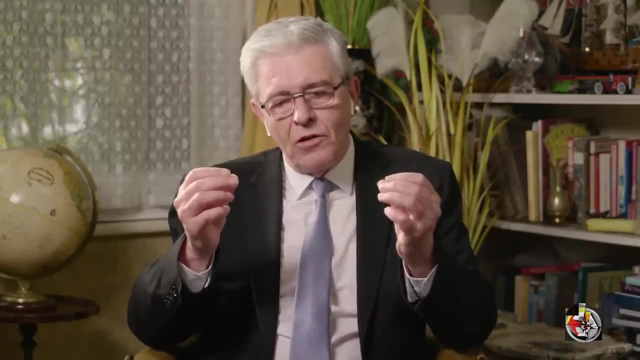 You've actually described a mechanism, let's say a structure, learning, learning the structure of this hierarchical world model or self model that entails the emergence of selfhood in and of itself. You know, in order for me, for us to take turns, 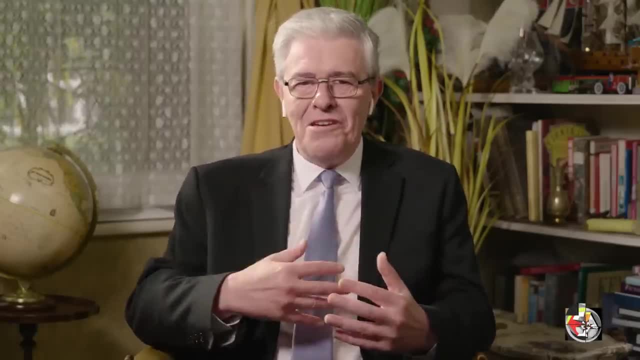 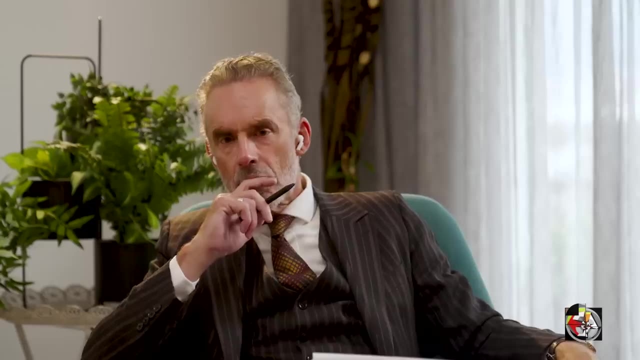 we both have to have this fantasy that I am me and you are you, And I have to recognise I am me and you are you, And we have to take turns. So now it's your turn, Right? So those are the, the axiomatic preconditions of that game and the axiomatic preconditions. 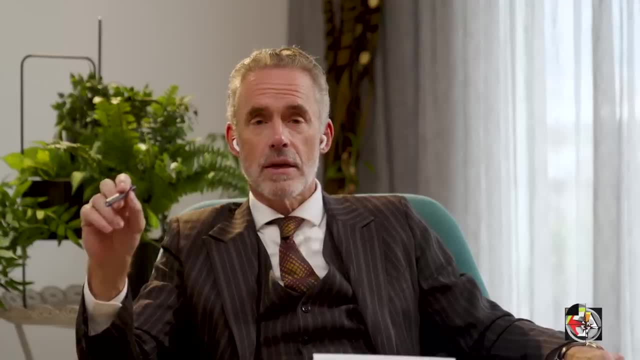 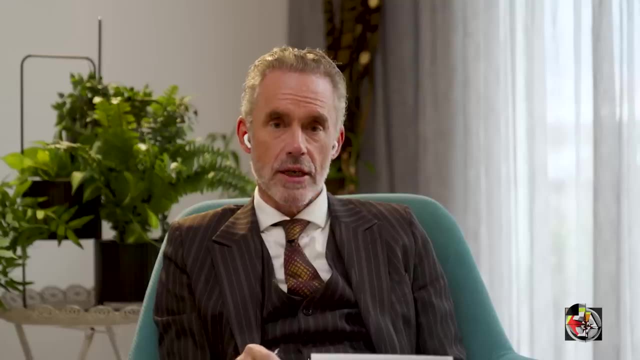 Some of them are: you exist as a separate entity and I exist as a separate entity, but we can be joined together in a shared vision, And one of the just for those of you who are watching and listening to understand is: well, if this is true and we establish a shared. 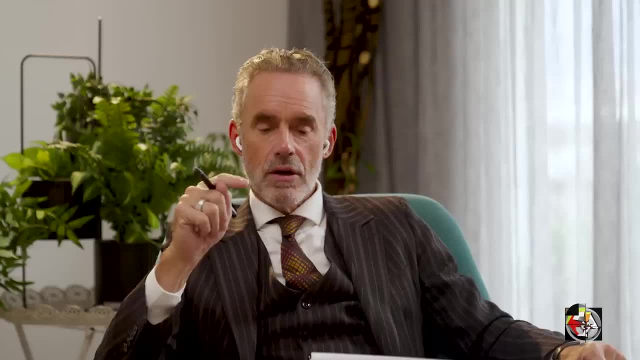 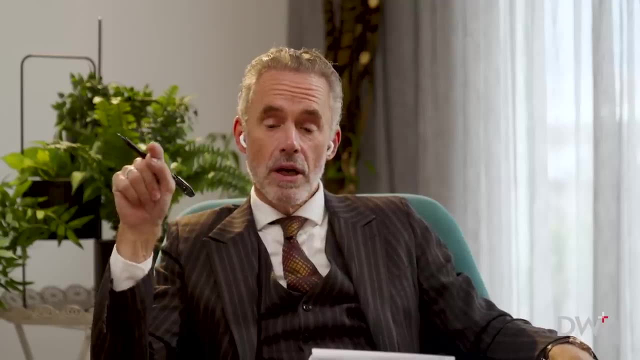 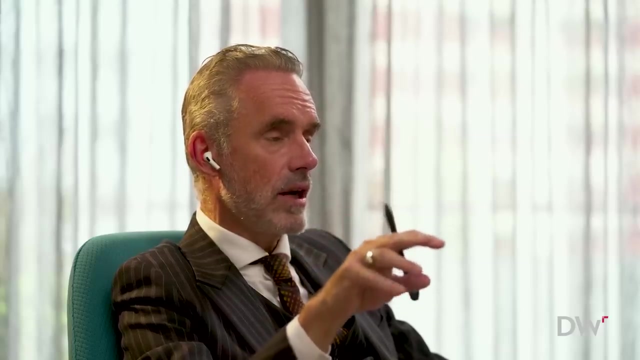 two people establish a shared narrative, and that shared narrative simplifies the world, and that simplification constrains entropy, then that shared narrative constrains terror. And so you might say: well, why is it possible to be calm in the presence of someone else? 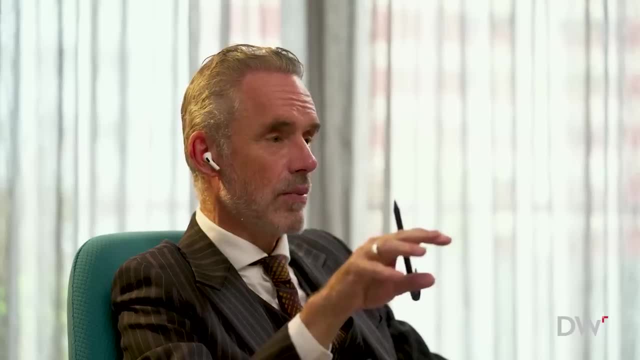 given their infinite complexity and also their almost infinite capacity for mayhem. And the answer? well, it is well. insofar as the two of you establish and inhabit a shared narrative, then all that entropic complexity is constrained by the desire. 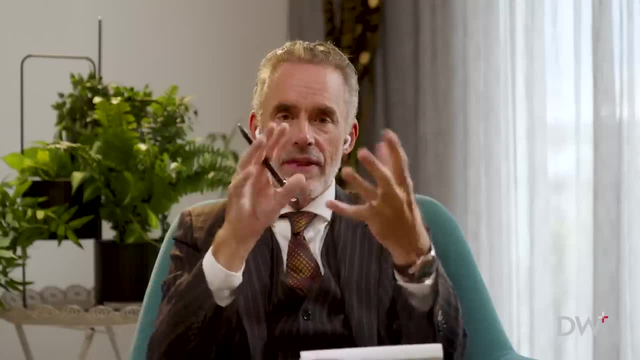 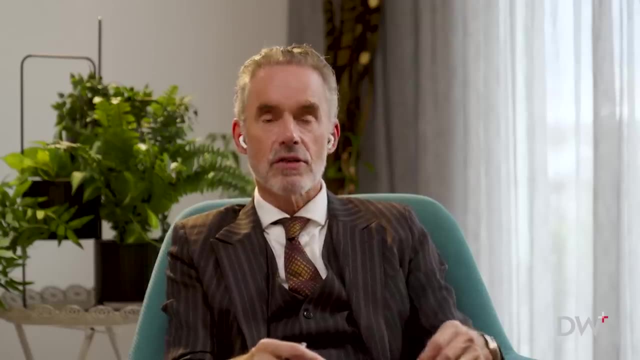 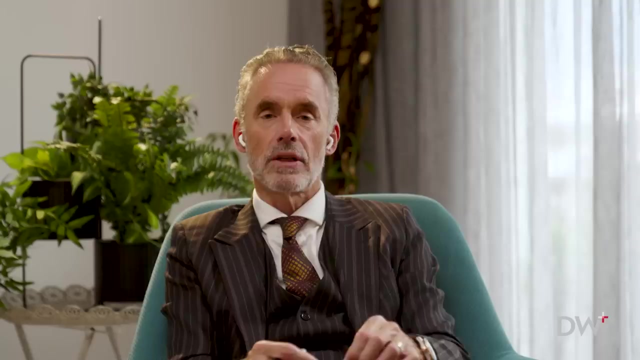 let's say, to keep the shared narrative intact. And then you might also point out that if you and I, our shared narrative might be, it would be worthwhile to have an interesting conversation, because both of us might learn something and we might have the opportunity to bring a bunch of other people along for the ride. 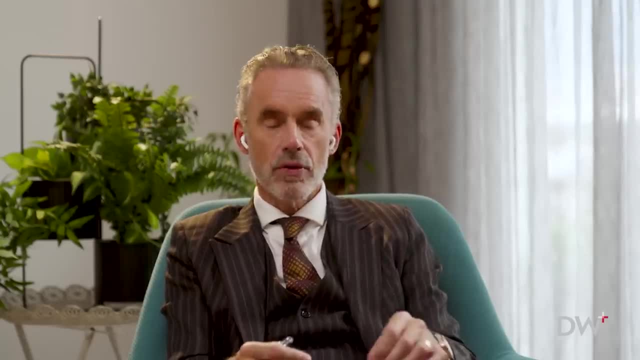 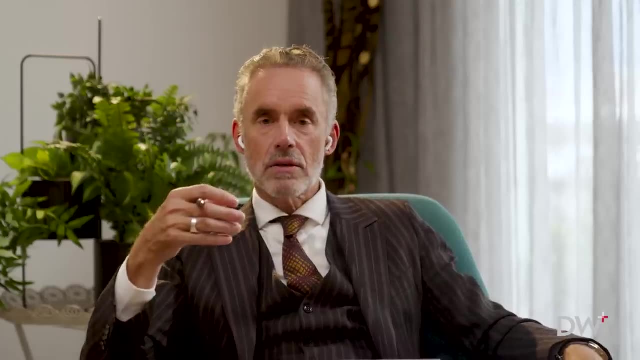 which seems like a good additional bonus, And so we both come to this conversation with that story in mind, and then we can play the game as a consequence, And even though we don't know each other, because we assume goodwill on each other's part. 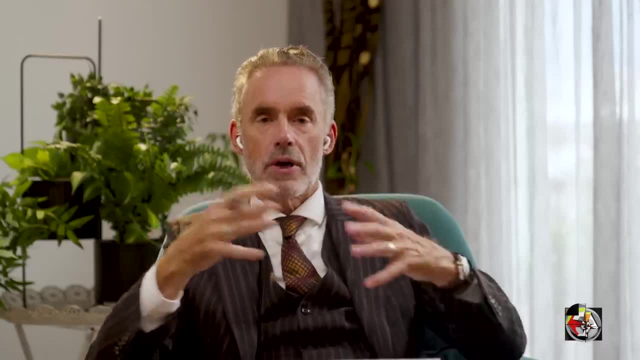 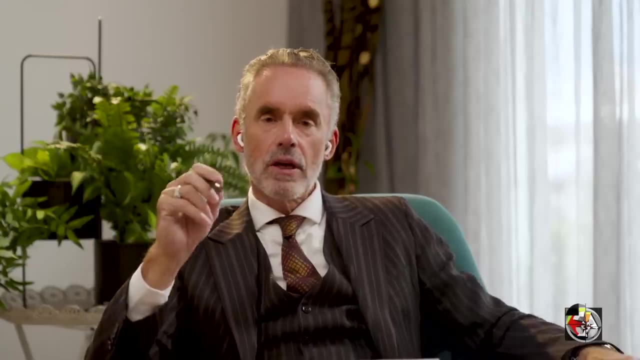 not only are we not anxious in each other's presence, apart from whatever additional relevant features might have to do with being on a podcast, but we can also take some pleasure in joint movement towards the shared goal, because the dopamine system to me 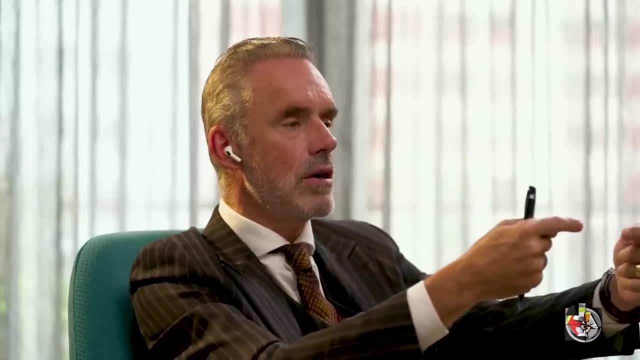 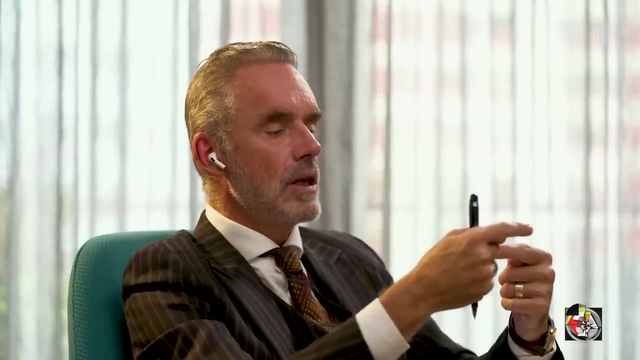 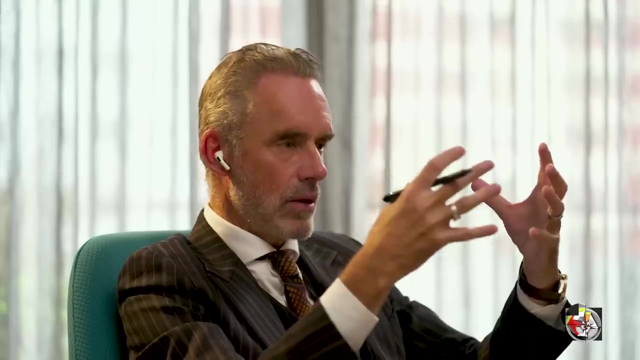 seems to indicate progress towards a shared to the instantiation of a vision. It's something like that. And then if you're acting in a manner that makes the vision appear to be making itself manifest, then that's rewarding, And that reward has an existential element. 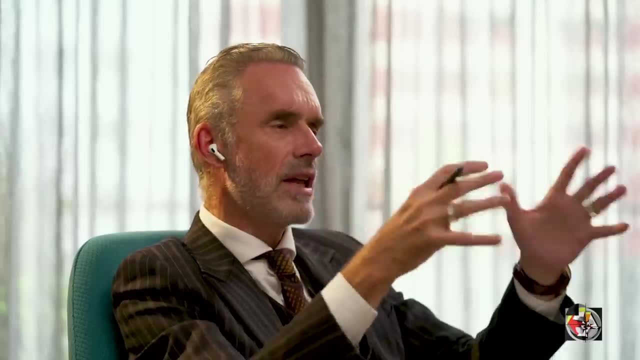 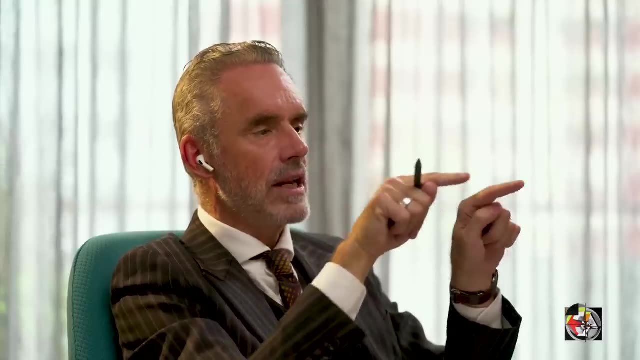 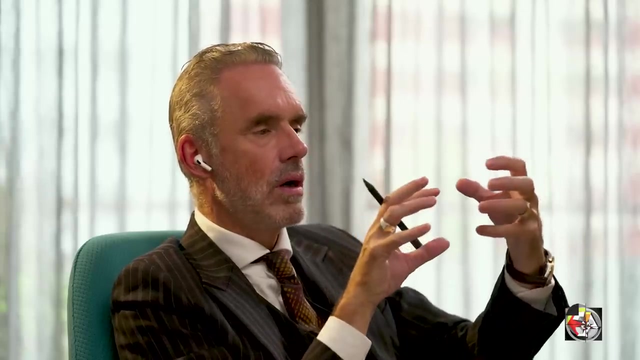 a phenomenological element. you can feel. It feels good. But then the dopamine. what it does neurochemically seems to be to track the neural systems that were activated just prior to the manifestation of the success and make them grow. And so, once you establish a shared narrative, 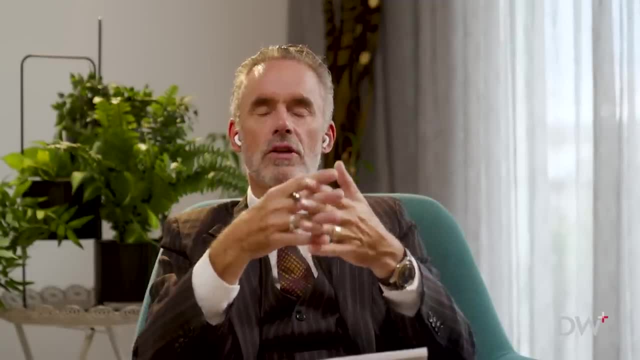 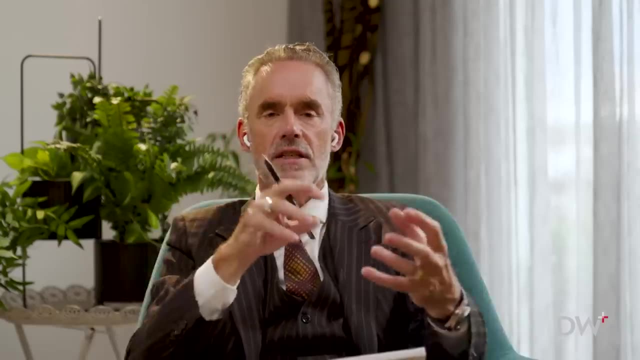 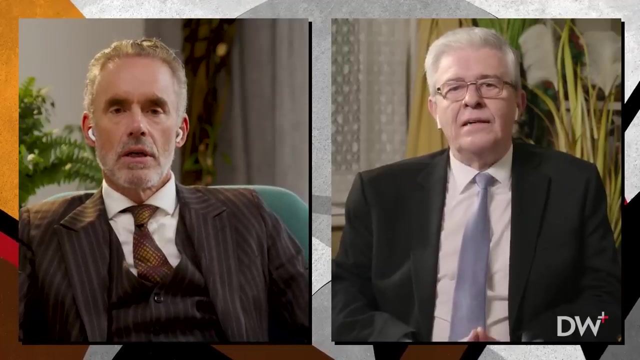 if you negotiate it successfully, you also increase the probability that the neural architecture manifesting that vision, making that vision manifest in skill and apprehension, is more likely to dominate in the future, more likely to take priority in the future. Yeah, No, no, go ahead. 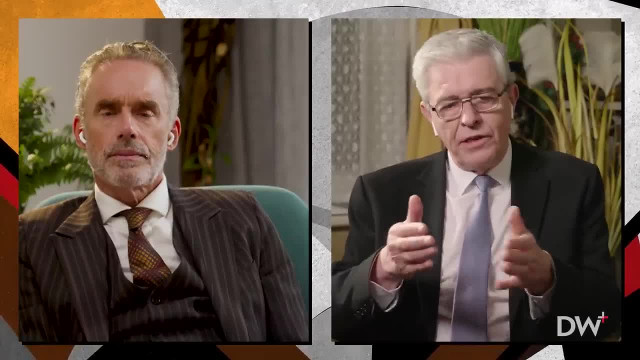 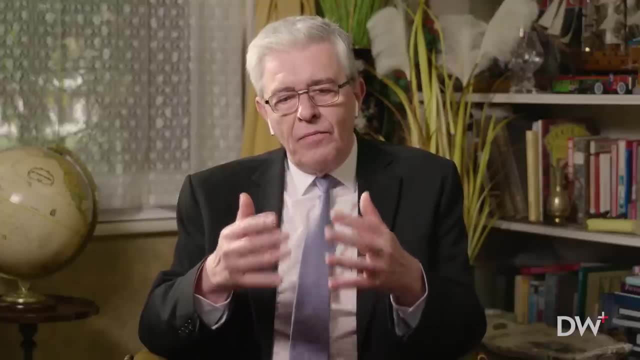 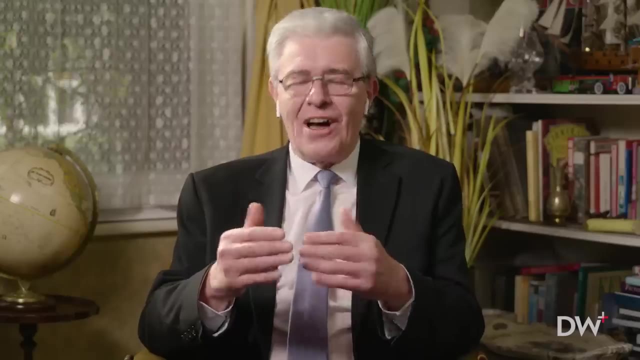 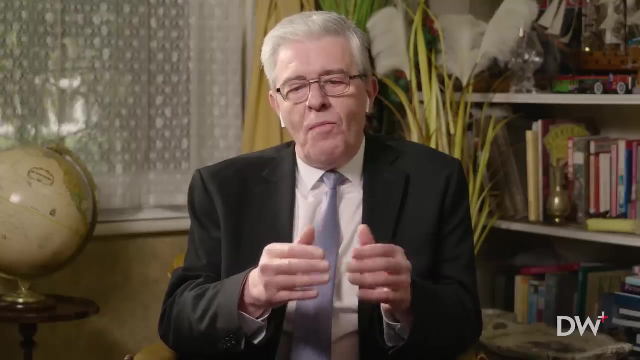 Well, no, I'm just noting you've now sort of brought in dopamine as an important neurochemical part of the anatomy of sense-making and exchange. So I just wanted to acknowledge that because in my world the way that one might describe that and interpret all the empirical evidence, 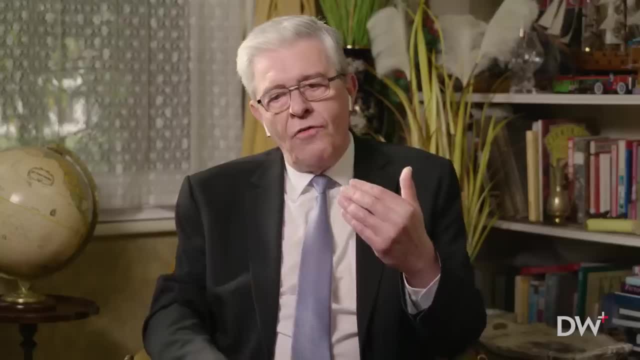 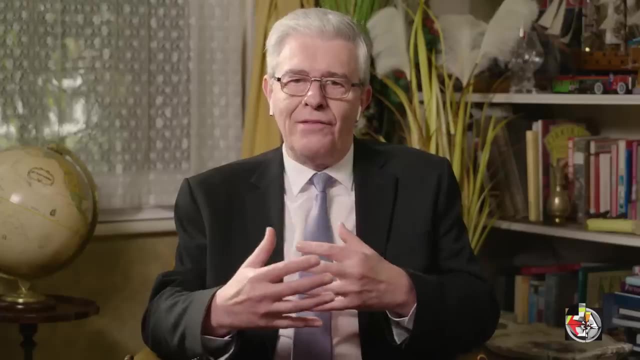 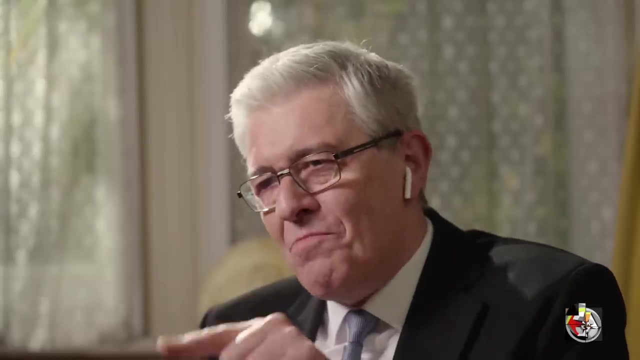 is very much along the line of this notion of pursuing a narrative and in this instance, a dyadic narrative, or a narrative about how I should behave in a dyadic context And if I resolve my uncertainty and just to open brackets. 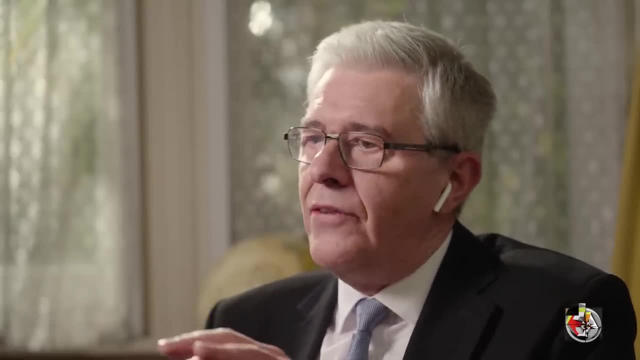 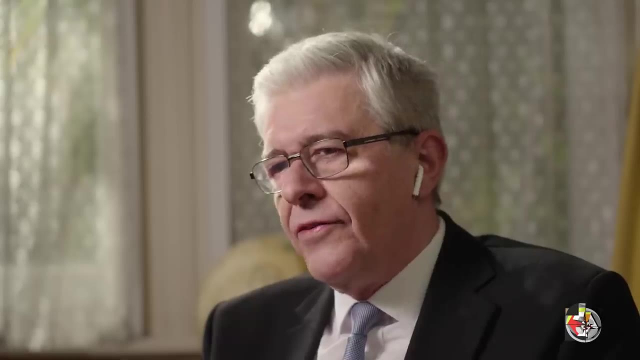 just to come back to your nice observation about we might learn something from this exchange, I think that speaks to that novelty bonus. you were talking about a bonus and certainly in machine learning, this information gain, this epistemic affordance. 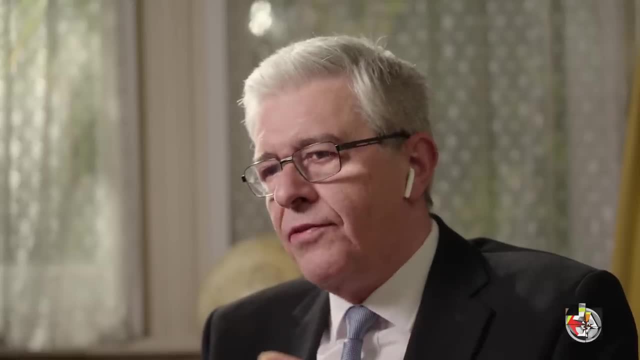 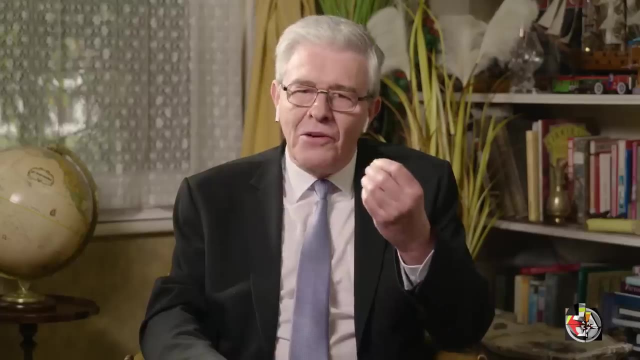 which is part of the good narratives and the good paths into the future, would be seen exactly as this sort of novelty bonus. So that is part of the reward. So if, in this exchange, we are both realizing, you use the word instantiating, 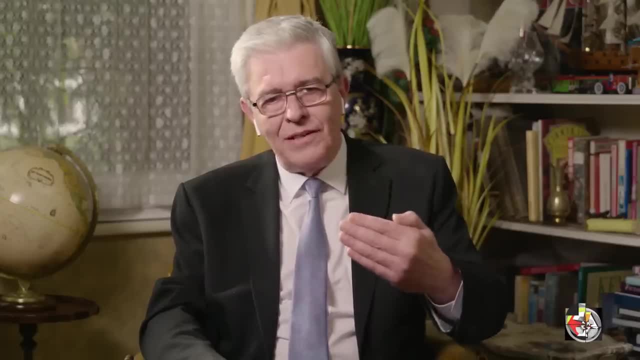 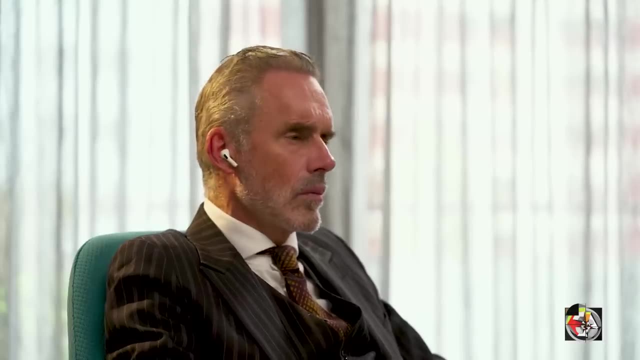 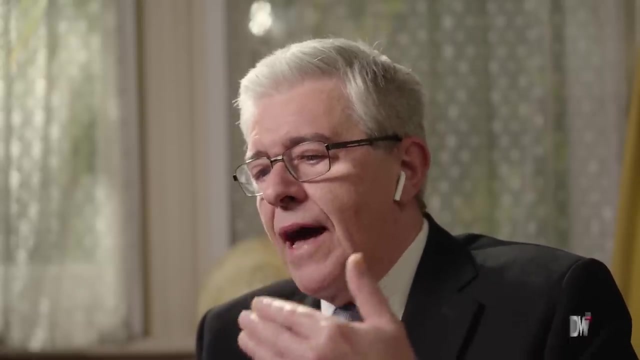 instantiating or realizing through committing to the right narratives literally a narrative of verbal exchange or linguistic exchange here, and that secures a resolution of uncertainty about what you think, or indeed about what I think, then that will be rewarding in the sense that it's minimizing uncertainty. 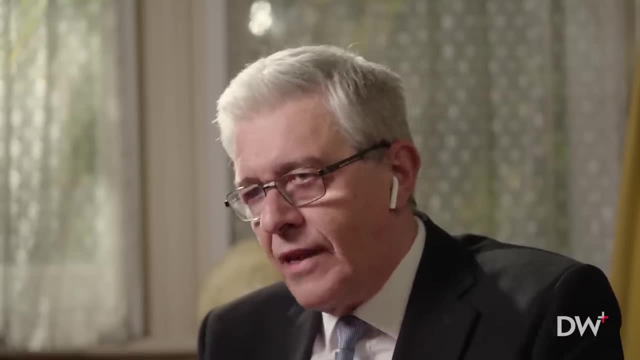 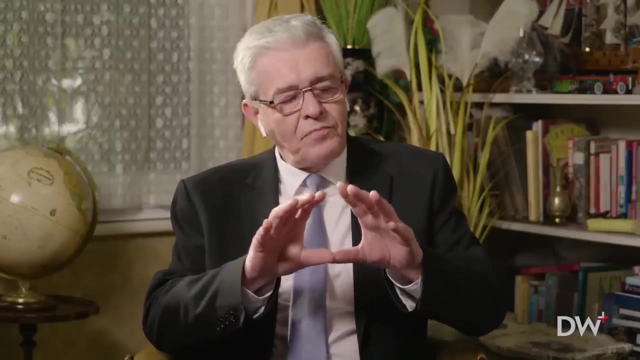 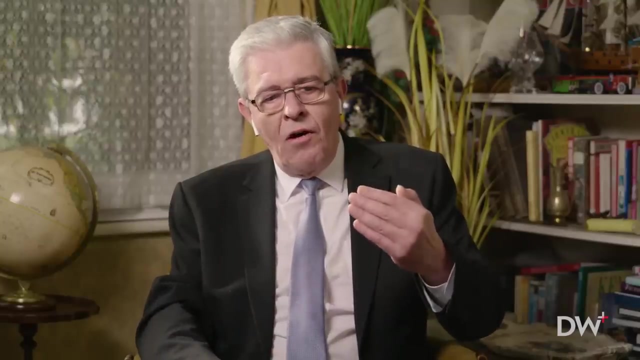 minimizing expected surprise, minimizing, if you like, entropy in the sense that you originally introduced it. So I think that's an important, if you like, generic thing, concept that you bring to the table here, that all these ways of looking at good narratives and good engagement with the world. 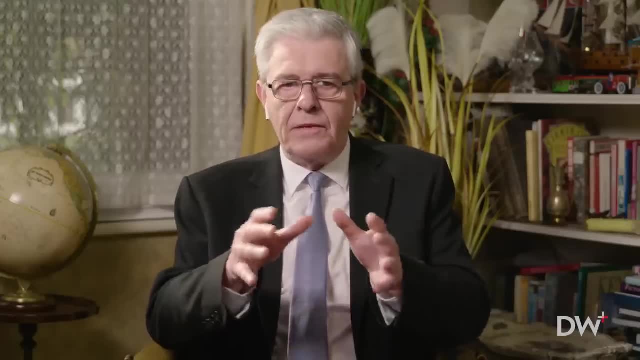 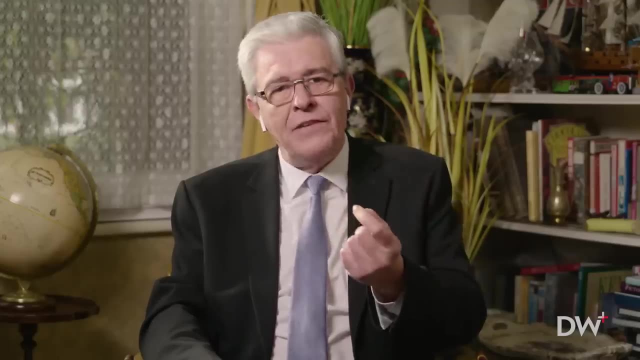 I think are all very internally consistent, especially when placed in terms of interpersonal interactions, and they also actually have biophysical correlates in our brains, And you've identified a really important one, which is dopamine, And we could talk about and I suspect you would want to talk about. 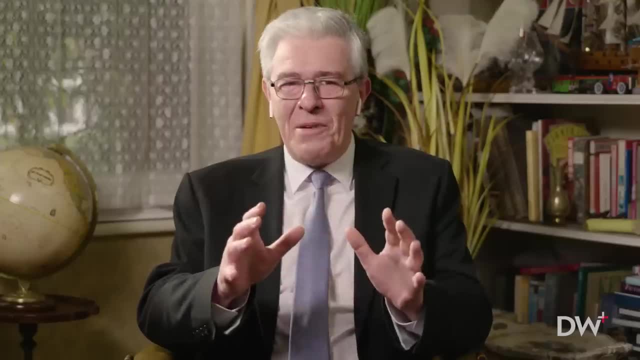 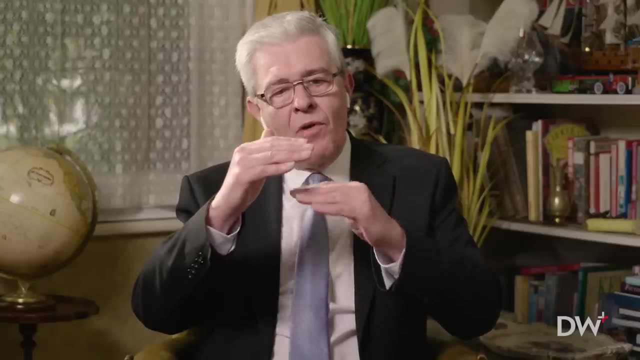 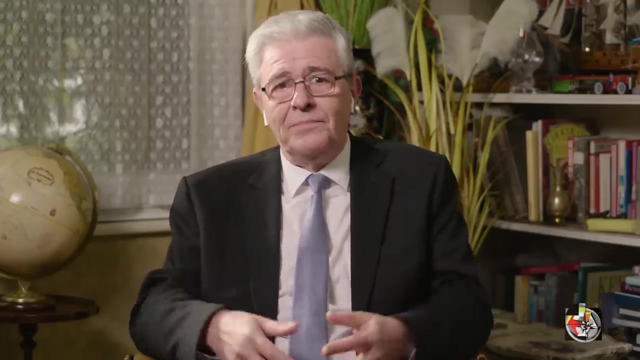 what's special about dopamine relative to all the other chemicals that are responsible for message passing and belief propagation and sort of getting the hierarchical fantasies aligned in order to explain what I'm sensing, what I'm hearing and indeed, what I'm saying? So do you want to elaborate on the role of dopamine? 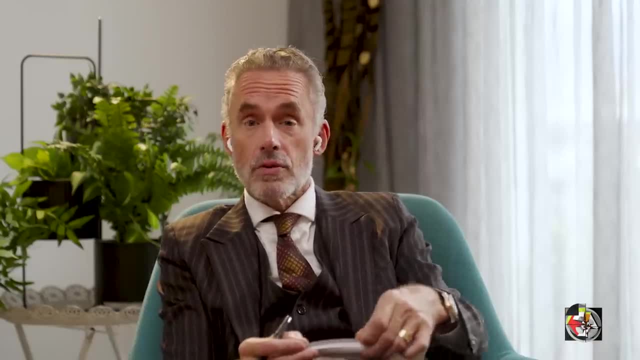 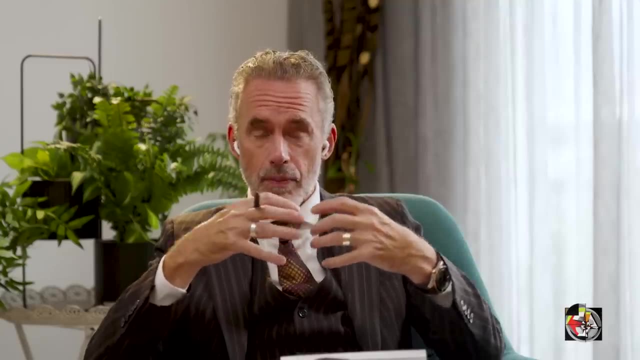 I'd be more than happy to hear what you have to say about that. So, because we talked about surprise minimization, but this is reward and reinforcement and the propagation of growth, and that can happen artificially, I mean if you dose yourself with cocaine. 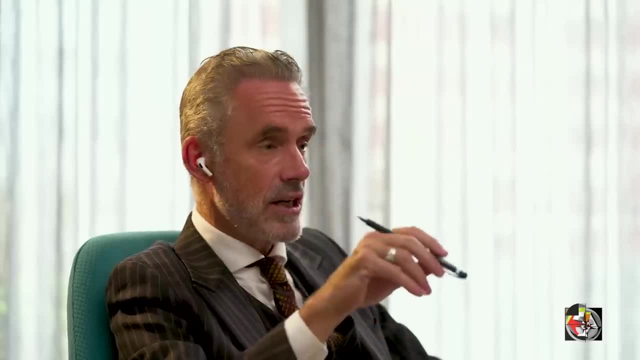 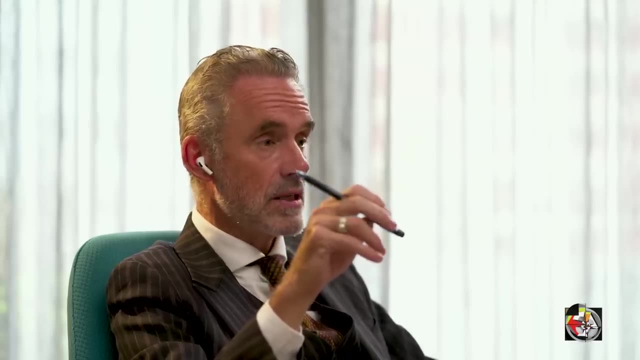 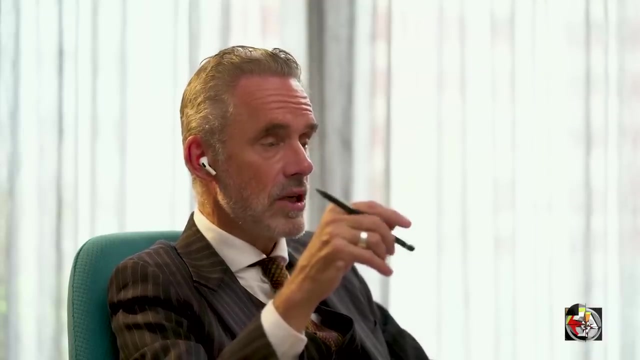 you can produce a cocaine-seeking narrative that's instantiated in your brain and that's actually what constitutes the addiction. in some sense, It's a cocaine-seeking personality. that's a unidimensional monster that now comes to dominate your neurophysiology in conditions of deprivation. 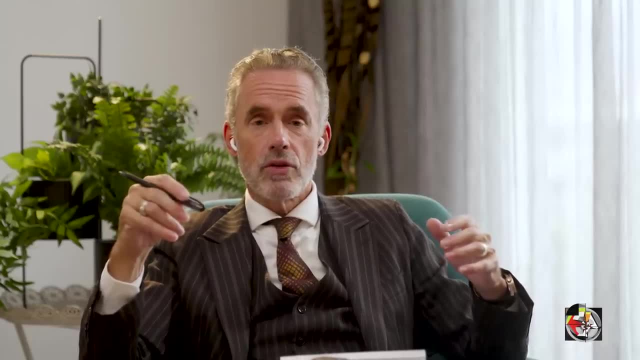 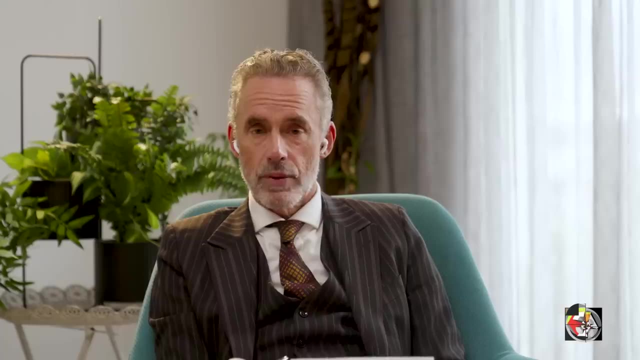 That's a very bad idea. You've generated an internal parasite that's fed on this externally applied chemical, But so if you could elaborate on the role of dopamine, I'd be more than happy to hear what you have to say about that. Yeah, absolutely. 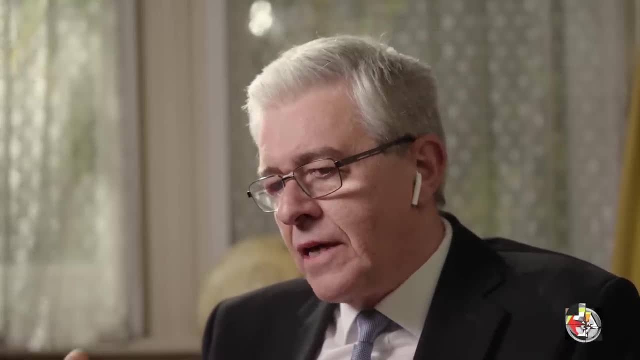 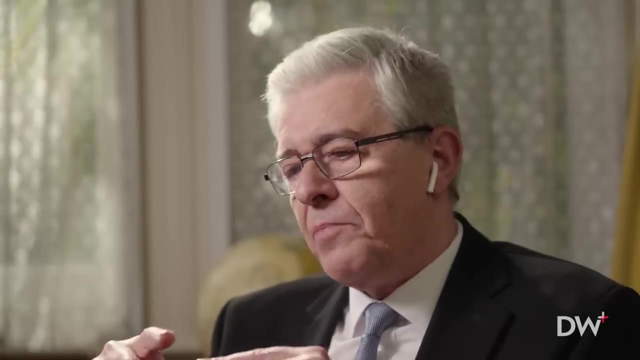 Just picking up on that nice notion of a cocaine addiction. it's sort of parasitic. I think that's absolutely right. It's sort of almost as if there's been a short circuit, a hijacking of the normal mechanisms that we would. 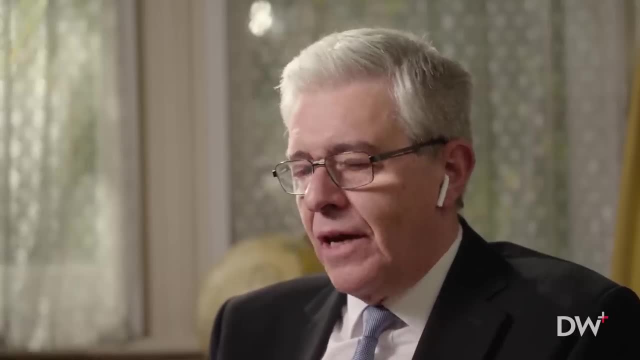 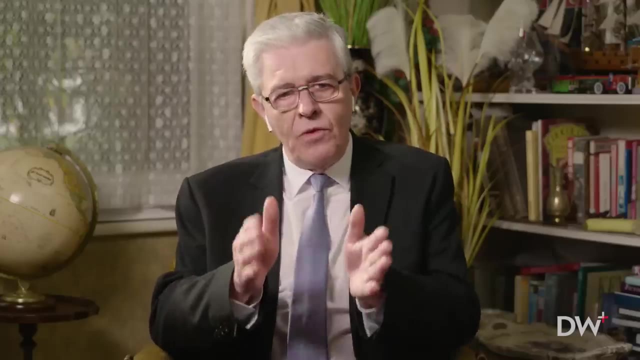 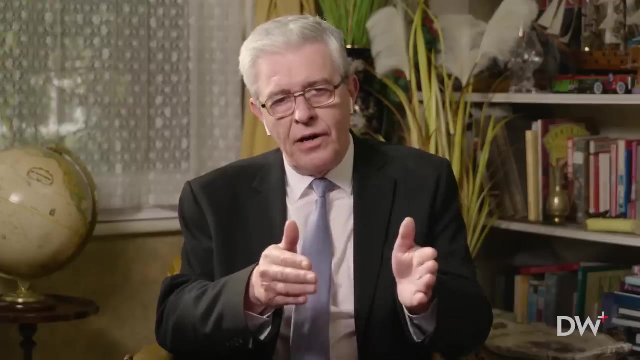 you know our brains would certainly bring to the fore to actually choose and register the choice of the right paths forward. So for me, reward just is that minimization or realization, minimization of expected surprise or uncertainty. So it is intrinsic, It is intrinsically rewarding to resolve uncertainty. 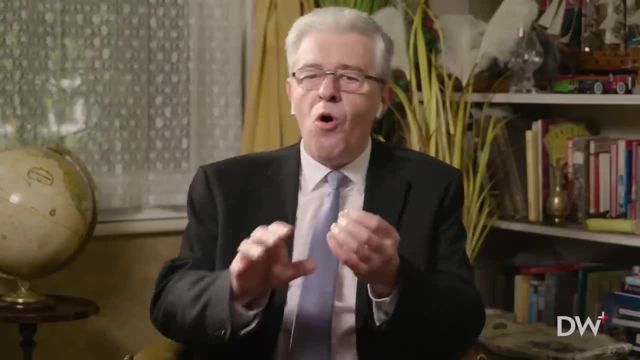 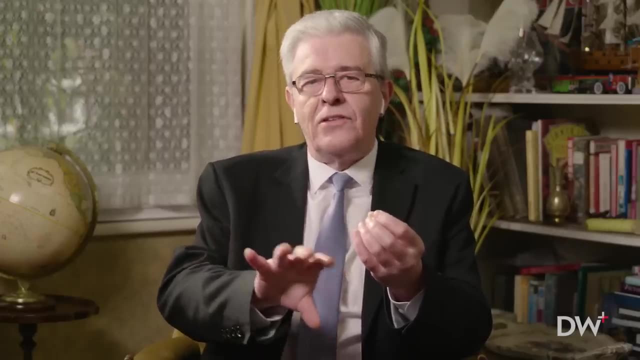 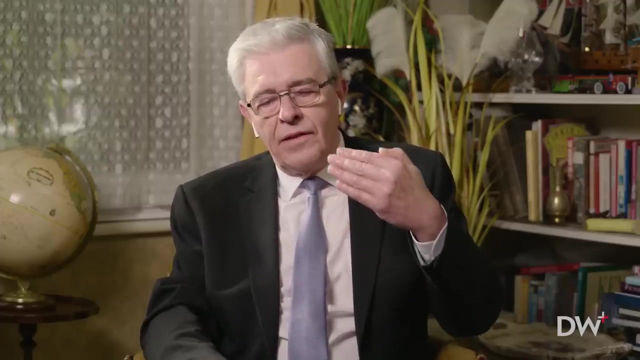 and to secure and seek out those novel things or avoid those unfamiliar, uncharacteristic, obstacle-like states that you know, states that do not characterize me. So you know, dopamine, I think, read like that- just is the fact you have resolved uncertainty. 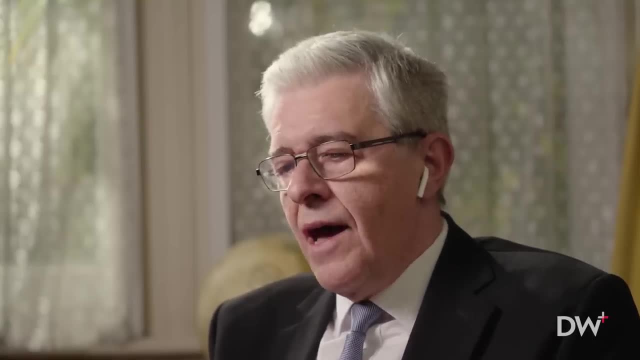 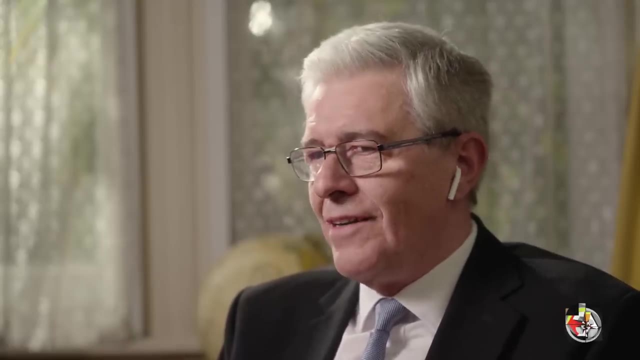 So if I get a cue in the world, say a conditioned stimulus, that tells me, oh, I now know exactly what I'm going to do next, I'm going to- if I'm a little monkey in an experimental paradigm- I'm going to receive a drop of juice and I'm going to drink that. 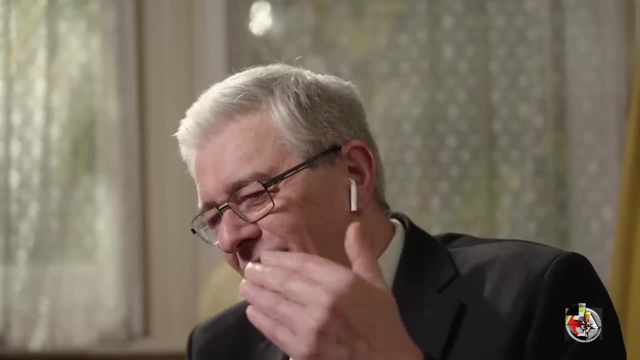 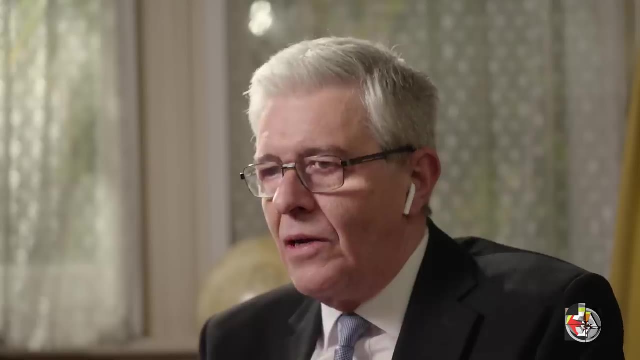 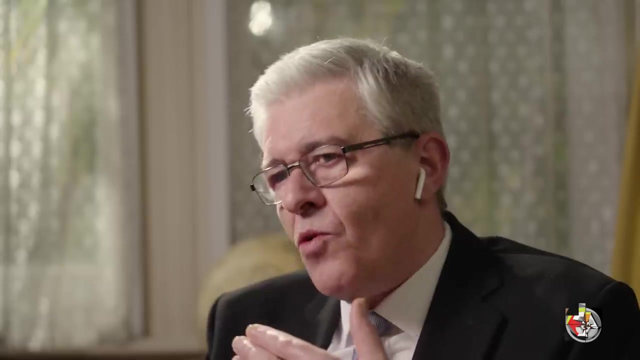 If I am somebody engaging in a social conversation, then I know exactly where this conversation is going. That's great, I know exactly what I want to say. So I think that's when you get the dopamine blush, that resolution of uncertainty: Suddenly you see the path forward clearly and it is exactly. 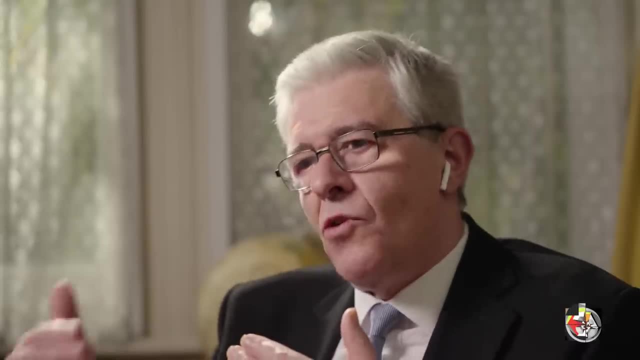 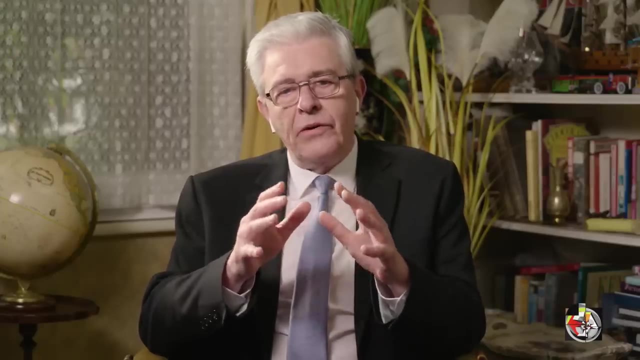 and I'm I'm using path, in your sense of the micro story, the micro story that's responding to the affordances. What's special about dopamine, though? Well, it's a neuromodulator, So it plays the role in the brain as not- of sending information. 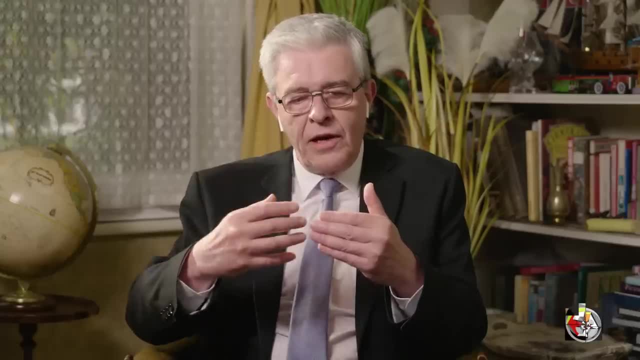 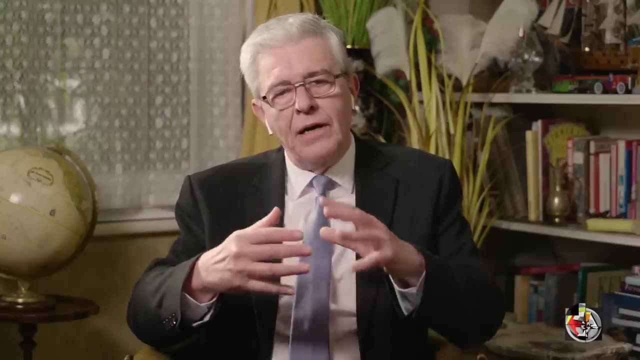 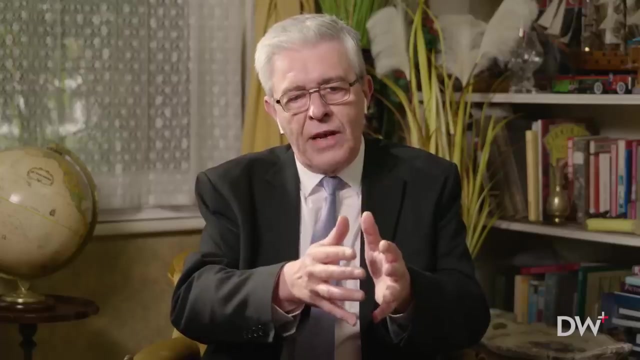 from this neuronal structure to this neural structure or this set of neurons to this set of neurons, but greasing the pathway by setting the excitability or the game, by being the, the chemical mechanism by which you will switch on this set of messages or that method set of messages. 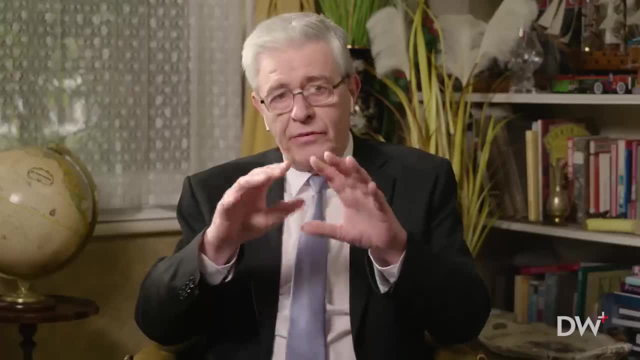 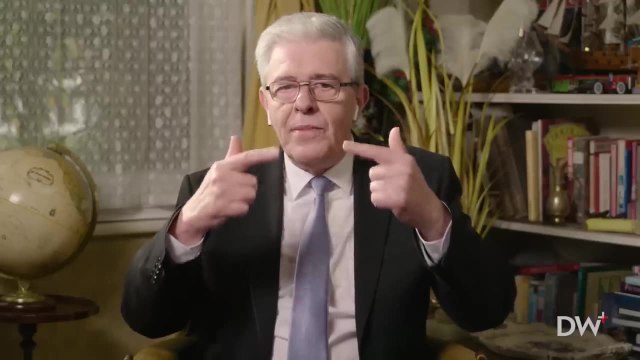 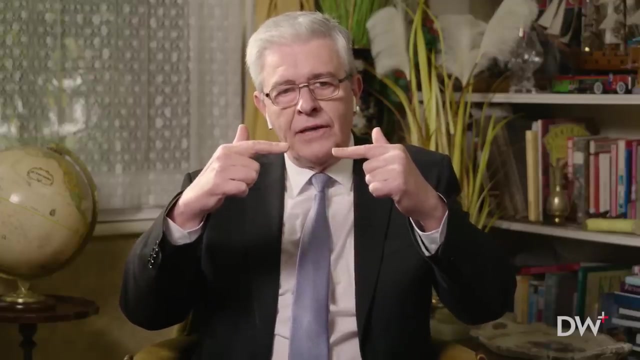 Another way of saying that is: it sensitizes. for example, let's come back to your sort of hierarchical structure that the, the micro stories are informing, or perhaps the mismatch at the lowest level- The prediction is at the lowest level- are inducing belief. updates at a higher level. 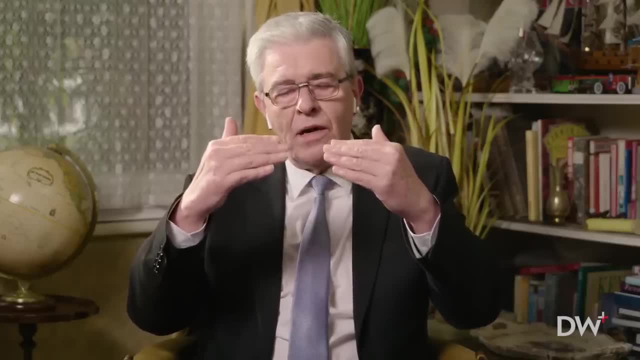 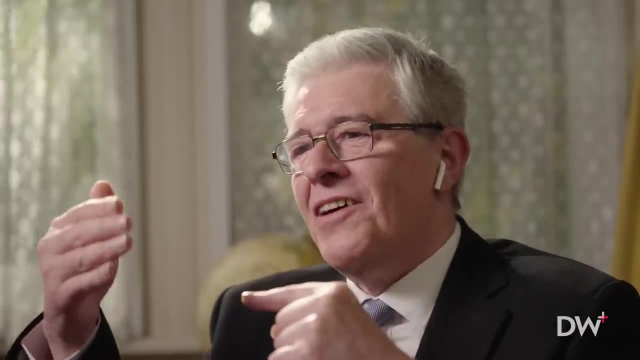 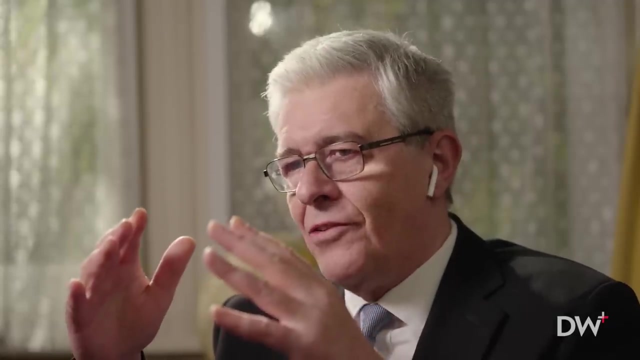 to get to these simpler, more abstracted inferences you were talking about before. but how much does the high level listen to the low level and how much does a low level inherit or respond to top-down constraints afforded by your simple high-level abstractions? your- which could of course be be the narrative? 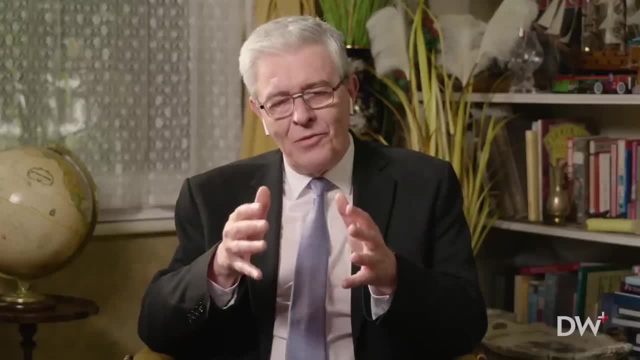 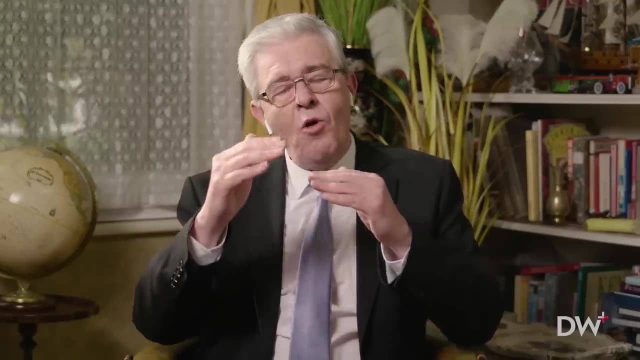 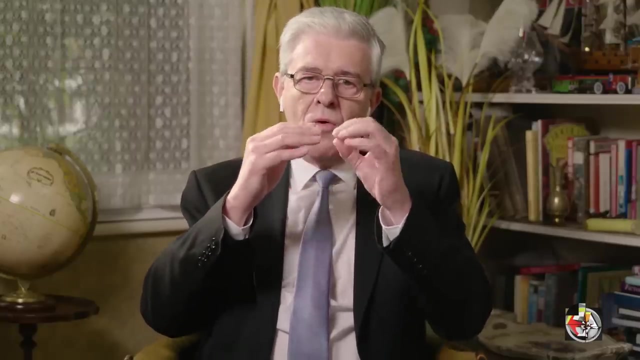 So chemicals like dopamine and I- and I wonder whether you also want to talk about things like serotonin in relation to things such as depression and learn helplessness- All of these neurochemicals Have one thing in common: their role in the brain is just to sensitize one set of 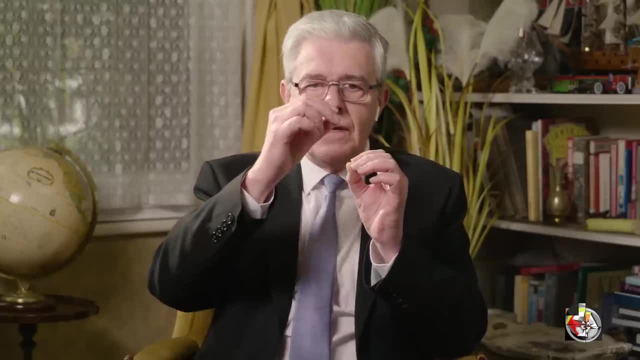 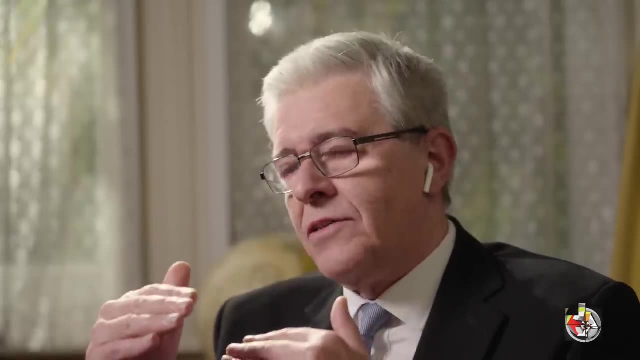 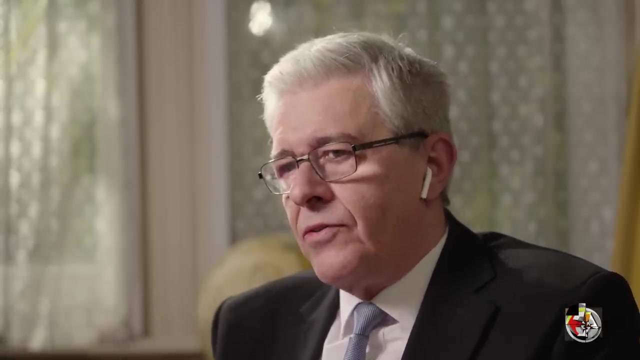 neuronal representations to messages from another set of neural neural representations. when placed in your hierarchical context, that can have a profound effect on the balance between how much you're attending to what's going on out there. So you're the micro, the microstructure, the low-level sensory and constructions. 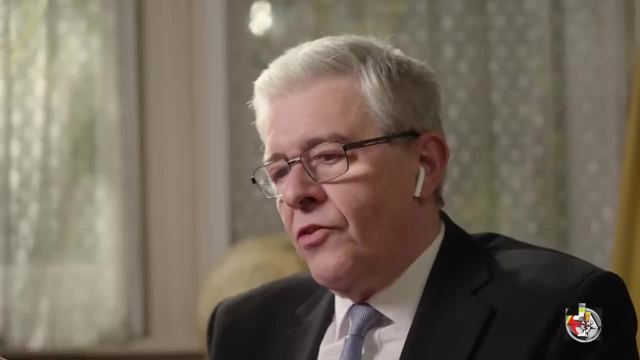 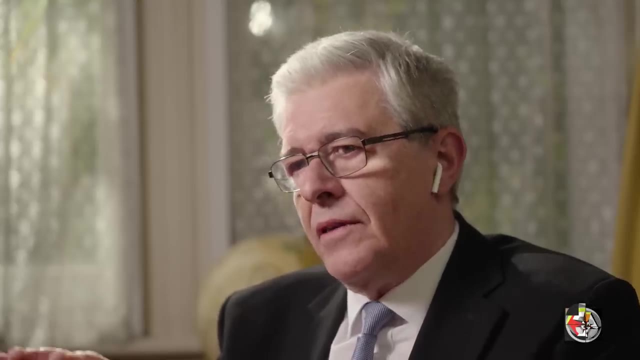 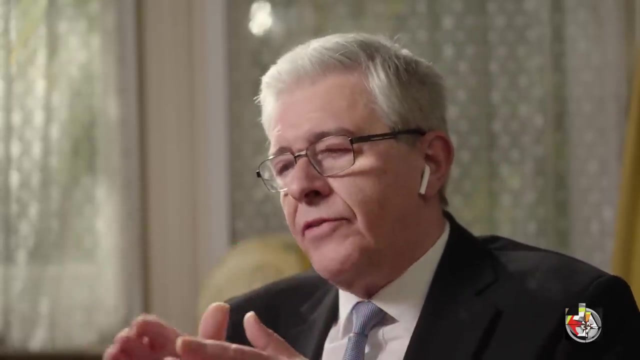 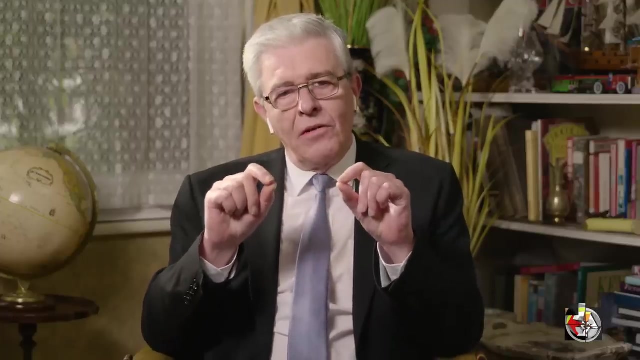 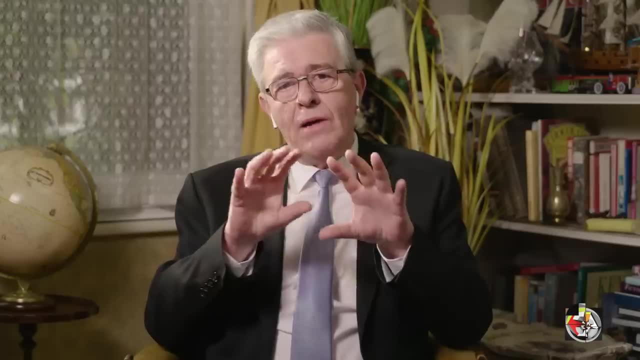 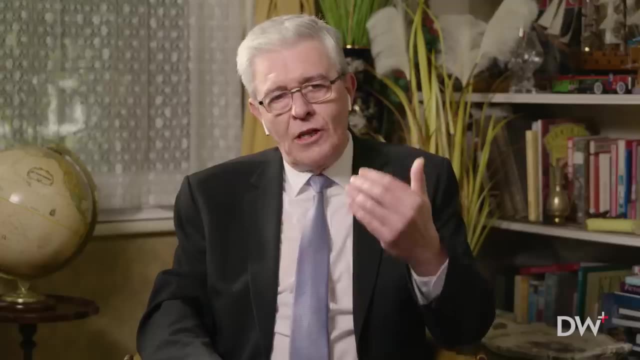 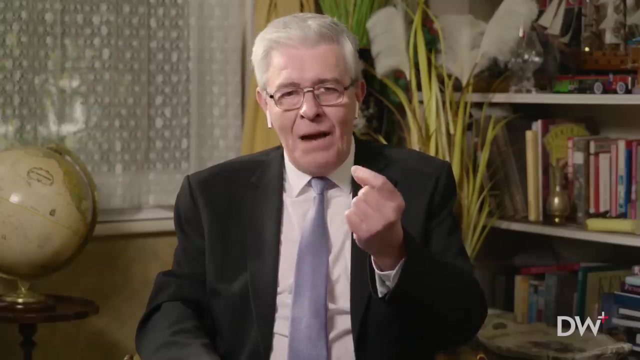 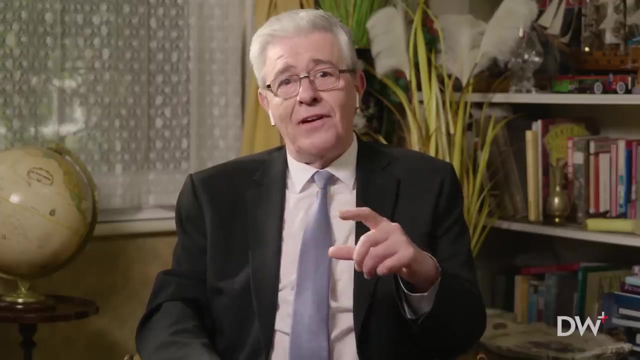 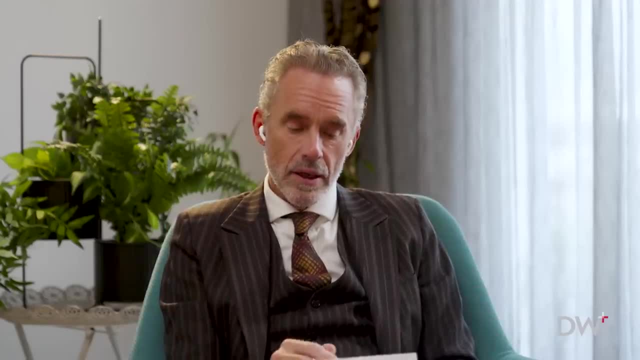 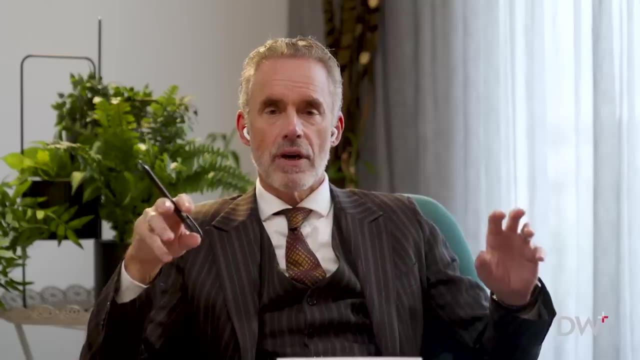 And it does that neurologically, On the serotonin front. so here's a pattern of depressive cognition And you can think about it as the collapse of a hierarchy. So let's say you have. You have a tiff with your wife. 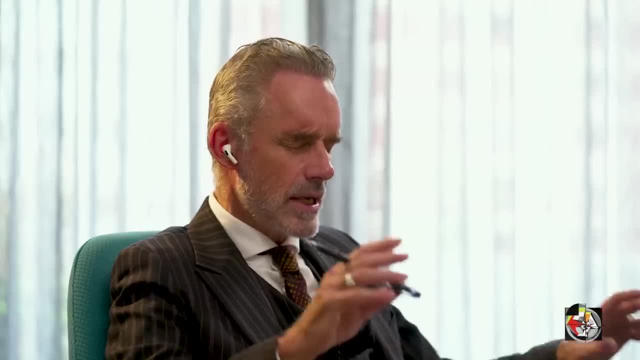 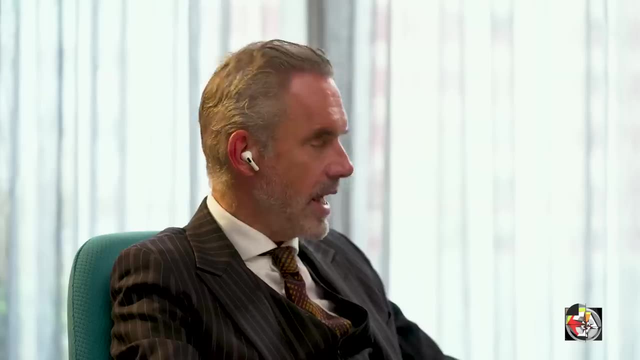 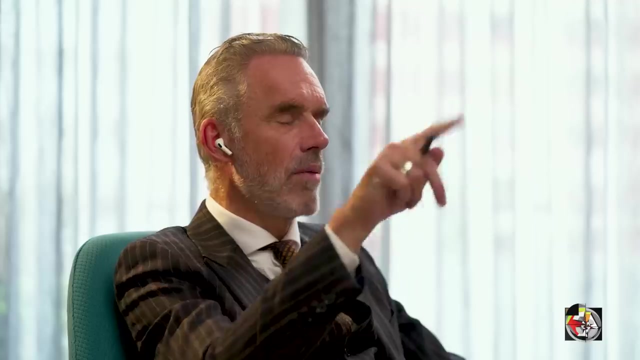 And if you're operating, let's say, normally in terms of your neurological hierarchy, you might say: well, you know, I'm just having an off day or I'm having an off hour, and it's only one little upset, it's only one little anomaly, it's only one little surprise. 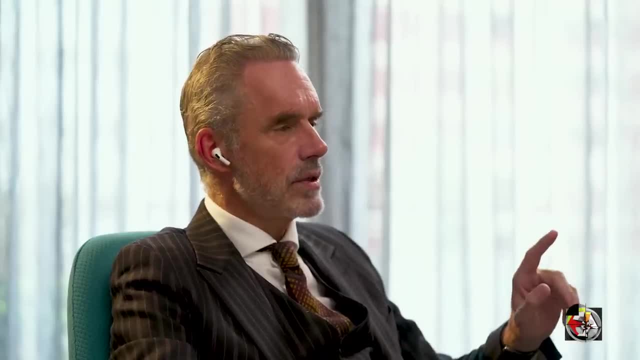 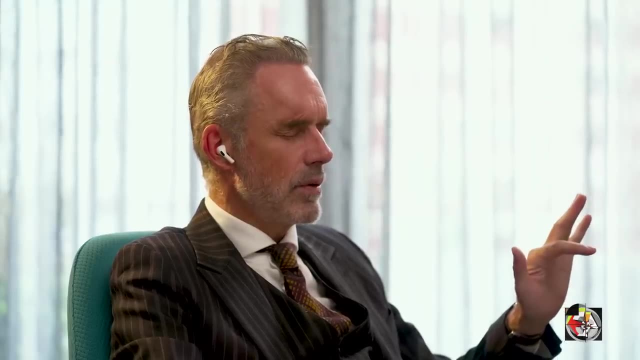 I can safely ignore it. But that isn't what a depressive person will think. A depressive person will think: oh my God, I just had another fight with my wife. I'm doing nothing but fighting with my wife. lately My marriage isn't going very well. 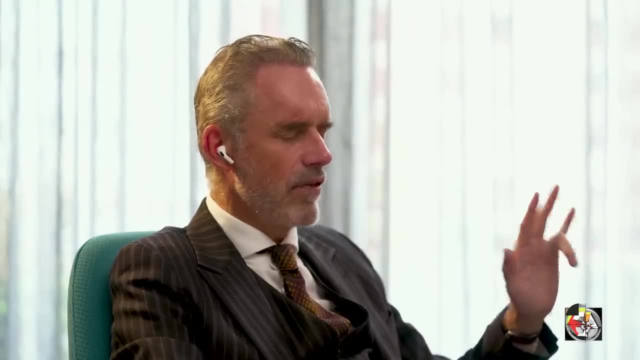 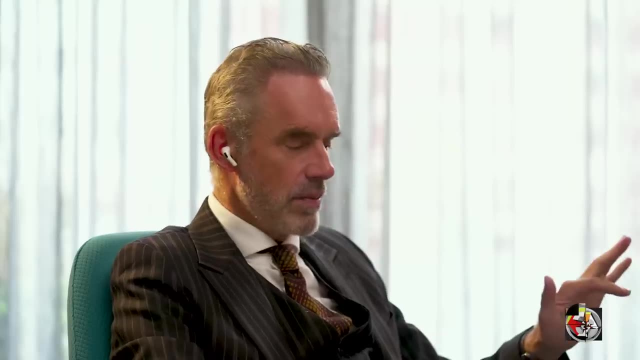 I've always fought with my wife too much in the past and I'm fighting a lot with my friends. I'm not a really good person to get along with. I mess up everything I do. I've always messed up everything I do. 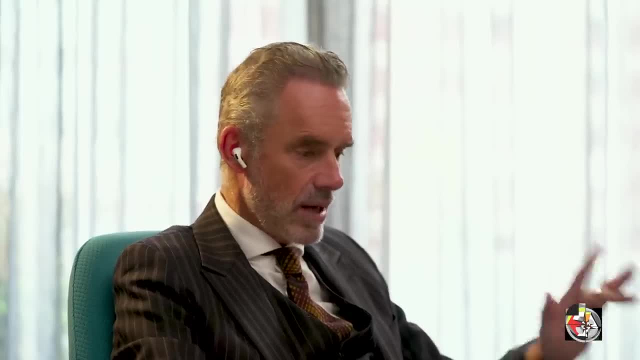 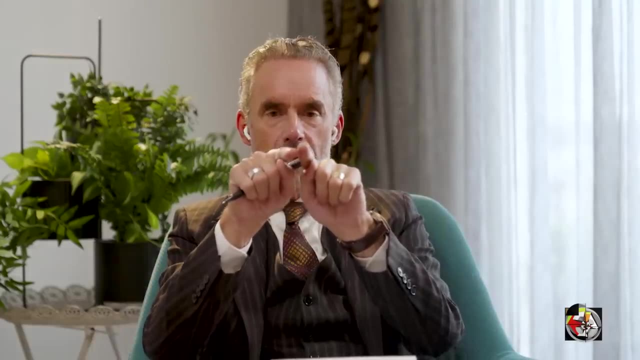 I'm going to keep messing up everything I do in the present because that's what I'm like and there's no hope at all for me to change in the future. And you can see that An error that could have been bounded at a low level. 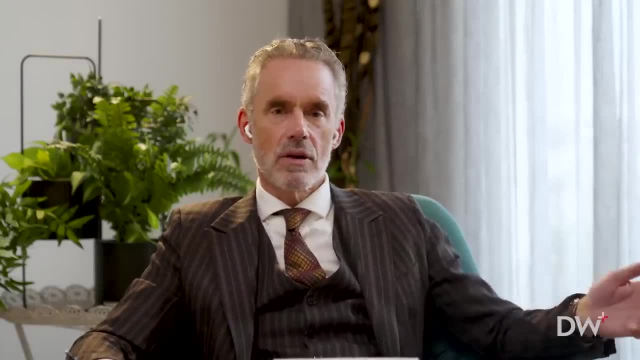 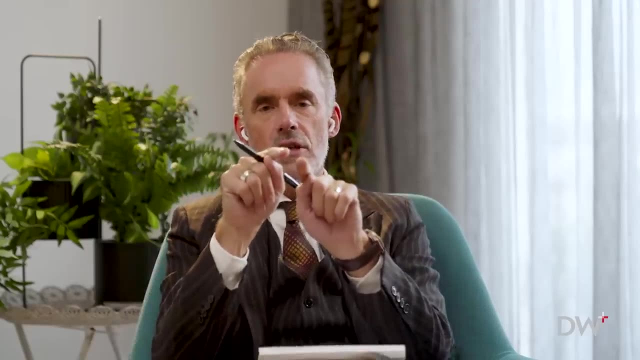 which is well- maybe I didn't have enough to eat in the last two hours and so I'm a little irritable- has cascaded through the entire hierarchy of self-conceptualization, And so imagine that each level of the hierarchy 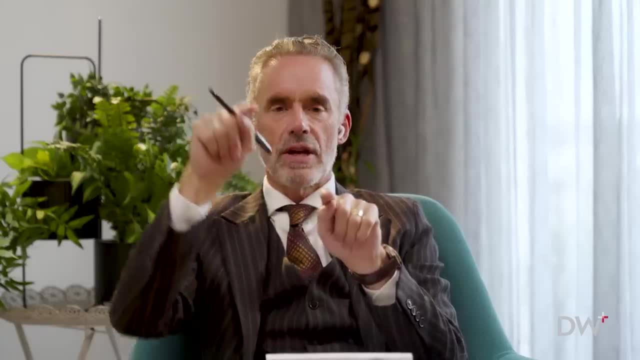 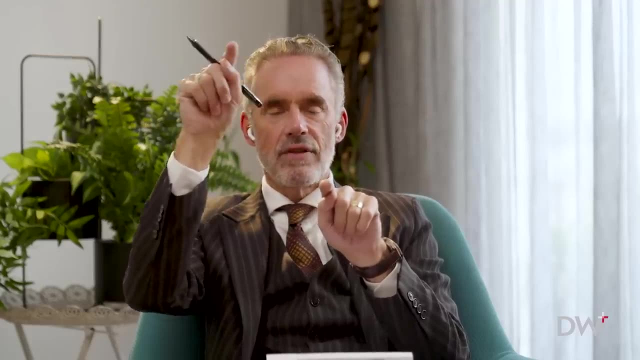 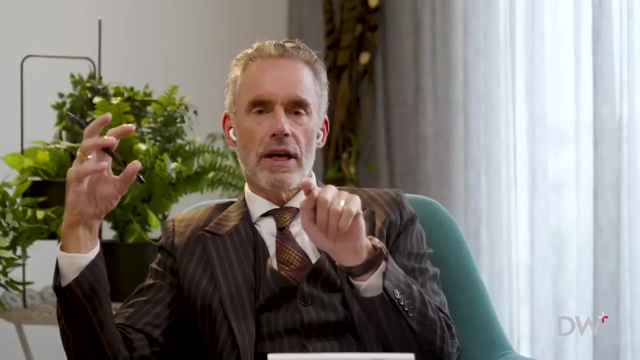 has to be protected against the propagation of error messages from a lower level. And then imagine: each level of the hierarchy has a resistance level that's set by something like the taunting, which is the taunting level of serotonin, And so the higher the serotonin level. 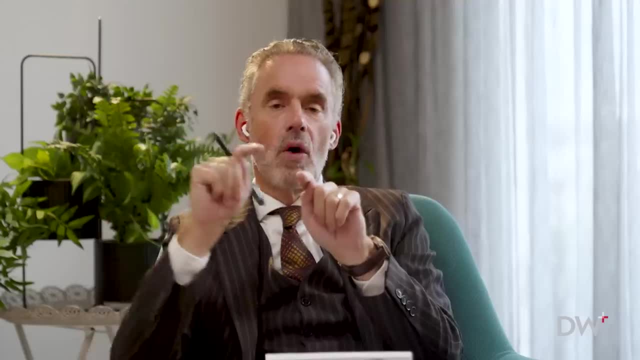 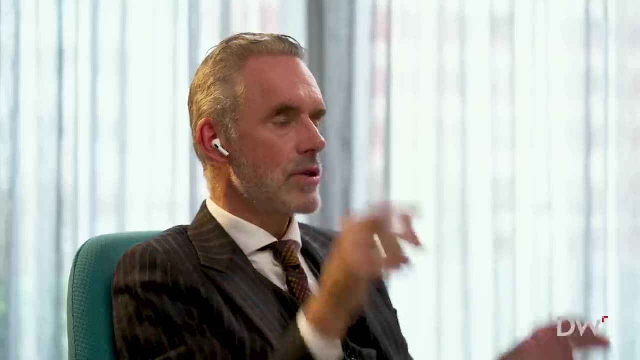 corresponding to higher social status. by the way, the more error has to accrue at a given level of analysis before a message will propagate up the hierarchical system, And so one of the things my wife and I have worked out in terms of modulating our reactivity to each other. 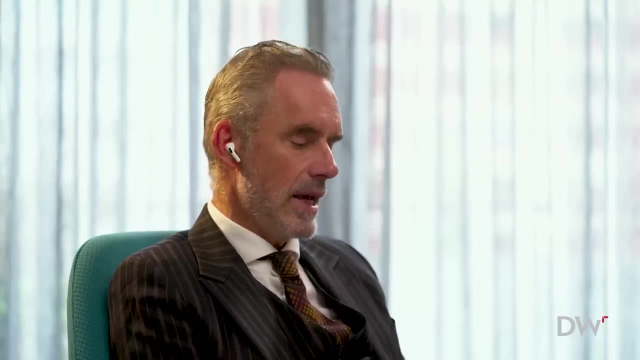 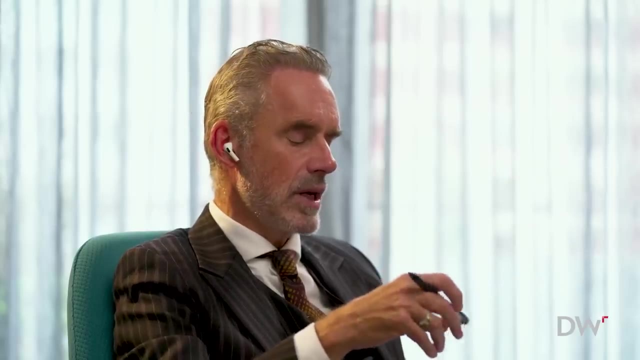 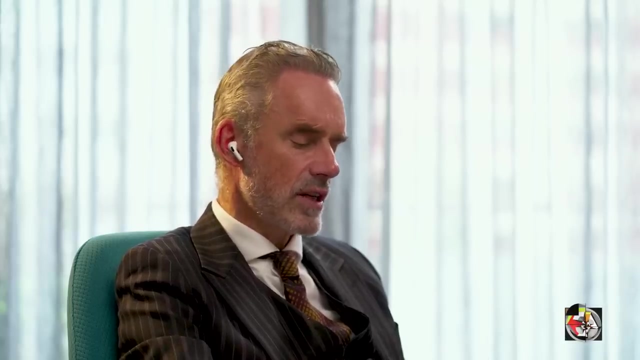 and to other people is: well, when should you respond to a disruption in social communication? When should you call someone on it? And our answer has been something like the rule of three. that's fairly typical of narrative descriptions of such things. If it happens once, you can ignore it. 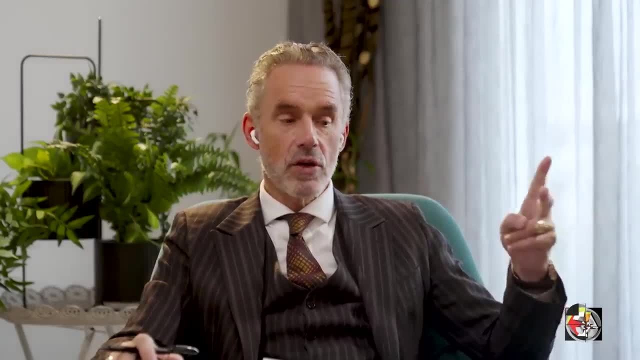 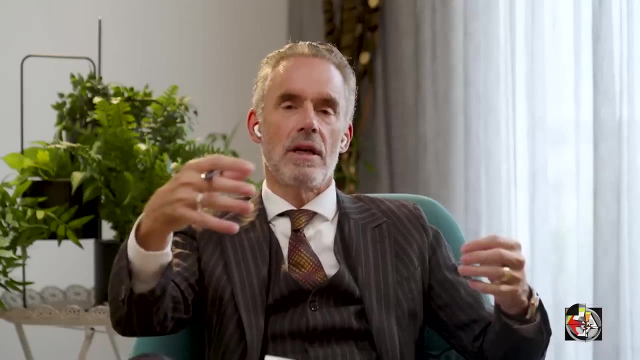 It's just random fluctuation. If it happens twice, you could mark it but still discount it. But if it happens three times, it establishes a pattern and then something has to be called into question. So I might say: if I'm interacting with my wife, 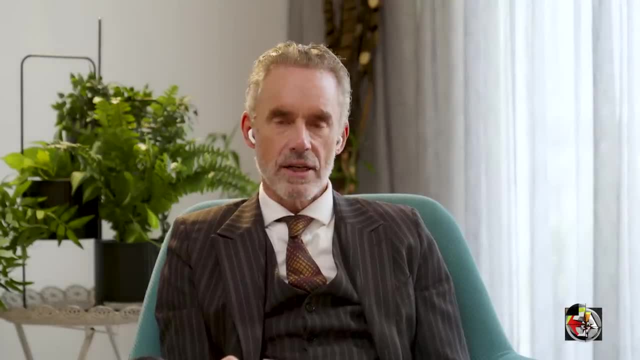 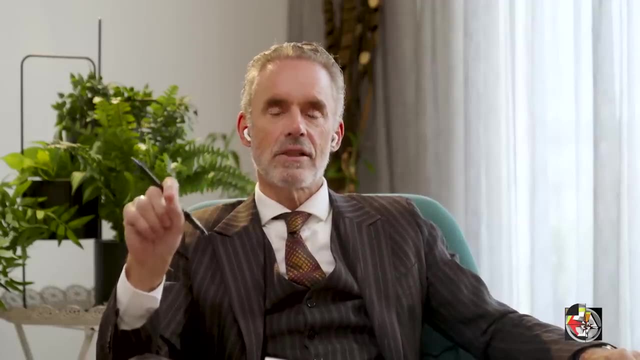 and it doesn't go well three times in a row. I might say to her: I tried to be friendly three times in a row and I've been rebuffed. What that indicates to me is something else is going on here. That's like a Freudian slip in some sense. 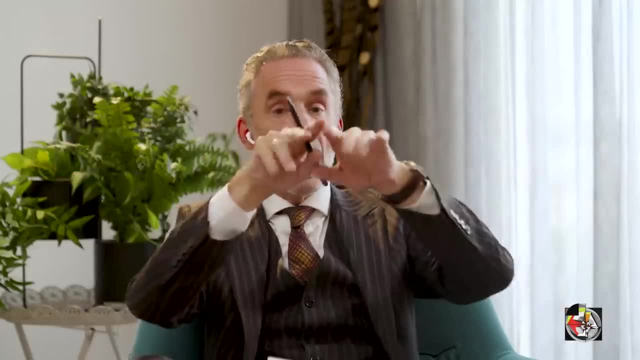 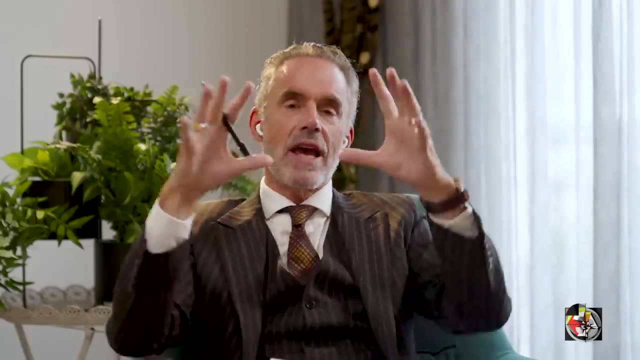 It's like I think this is what's happening. I want this to be happening, but it's not happening. Here's the evidence: three instances. Thus, we have to reconfigure the narrative that we're using to structure the space, and we have to say: well, 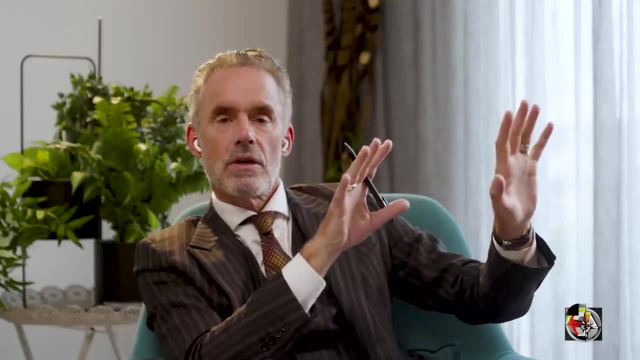 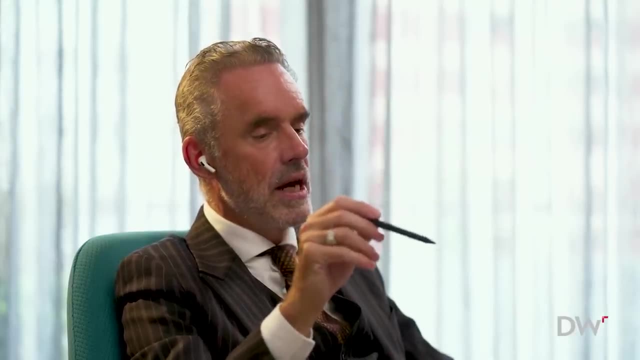 what actually happened, What actually is happening here, What needs to be resolved? And you don't say well, we were rude to each other three times. today, therefore, our marriage is over and we're both terrible people, because that would be leaping too far up in the hierarchy. 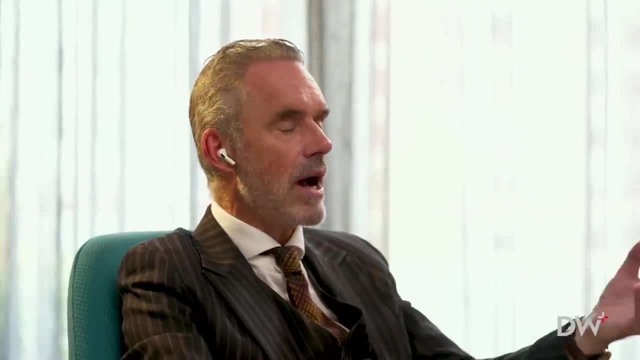 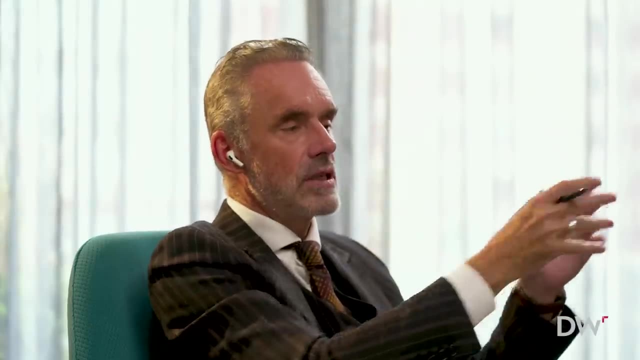 You might say: well, is there something else going on in the background that's disturbing you, so that you're more irritable in relationship to me? that's part of a different conceptual structure, And maybe the other person will say: well, you know. 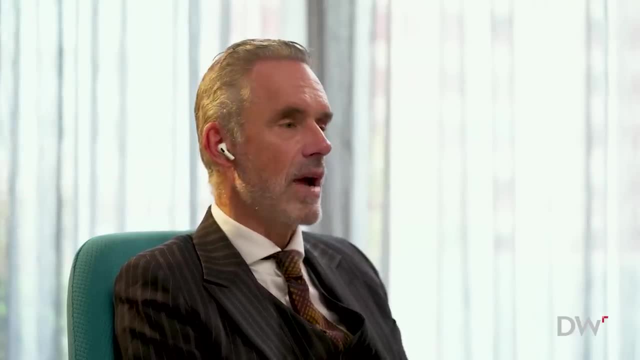 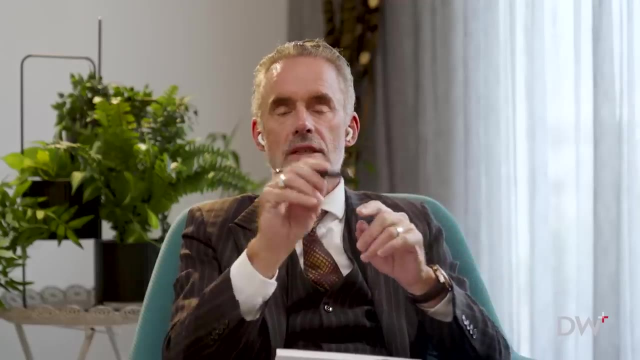 I didn't have a very good day at work. I was arguing with my boss. He's a bit tyrannical. Then you can go off on that narrative and try to resolve it, But you can see depression as the collapse of that resistance. 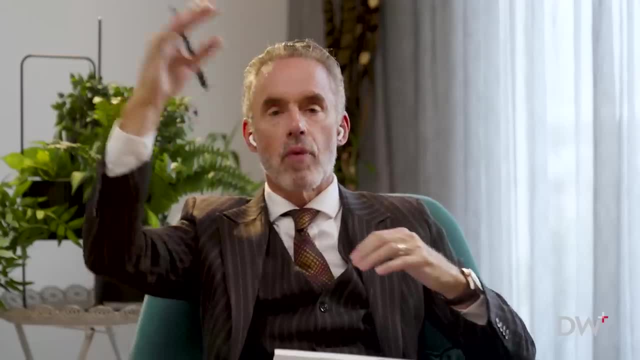 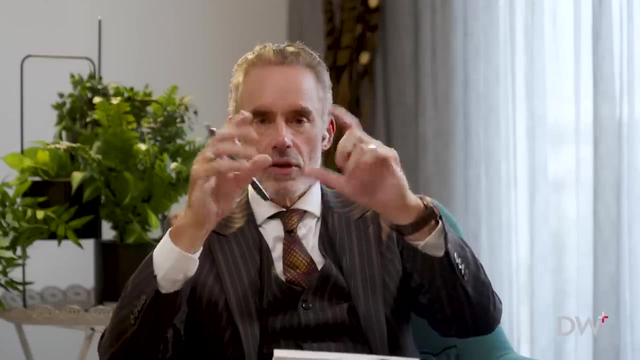 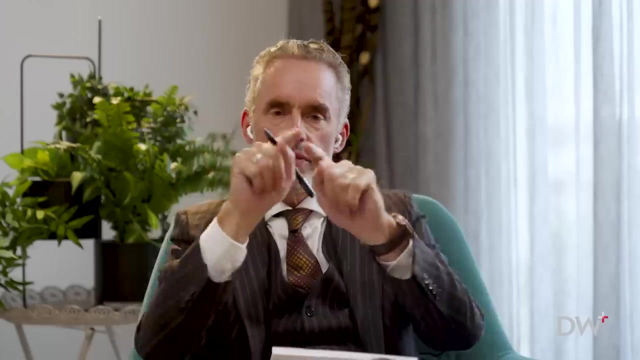 of the hierarchy to the propagation of errors upward. And so when you give people serotonergic reuptake inhibitors, what they seem to do, arguably, is make each level of the hierarchy more resistant to the propagation of upward error. And the reason I tied that into social status is because we know 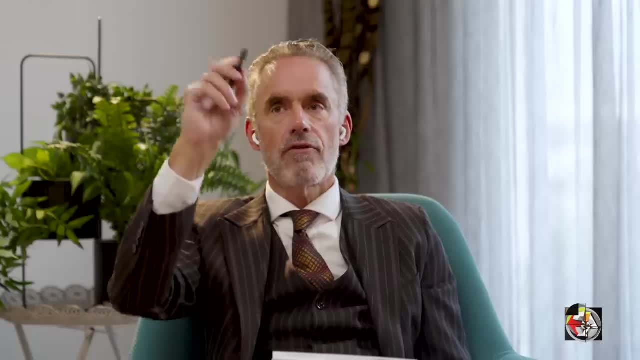 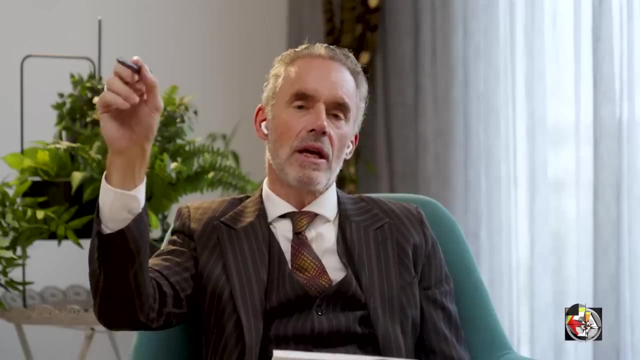 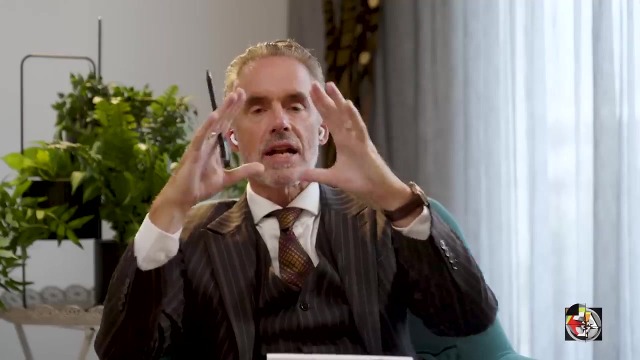 that animals that have higher social status and therefore occupy a more secure position in the social and environmental hierarchy, are more resistant to anomaly, partly because they can rest comfortable in the supposition that their superordinate status actually means that they're globally safer, They have better social relations, they have better access to necessary 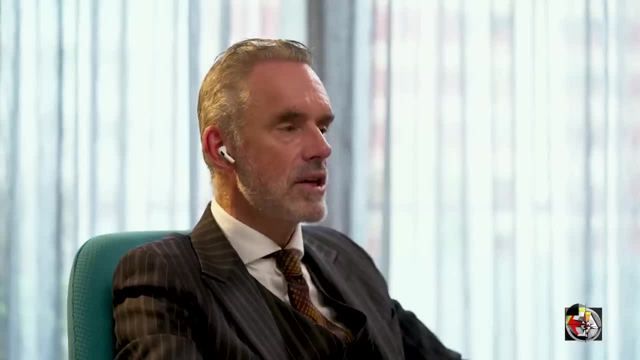 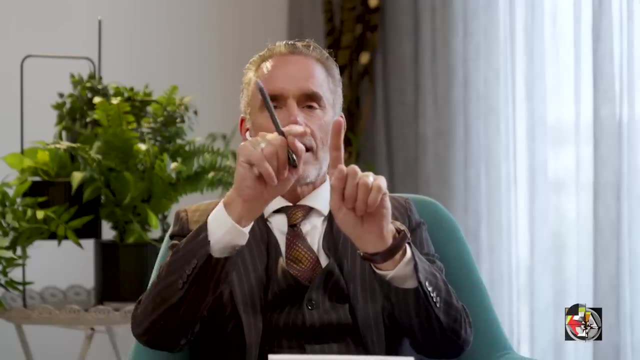 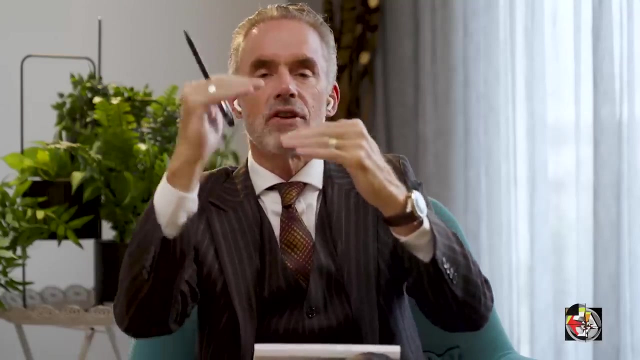 environmental resources. The world isn't as dangerous a place, And so you can imagine that your brain computes how likely an error message is to propagate upward, partly by looking at your social status, which would be the value that other people have attributed to you. 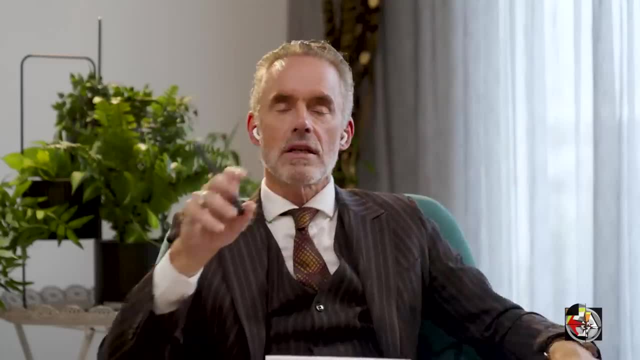 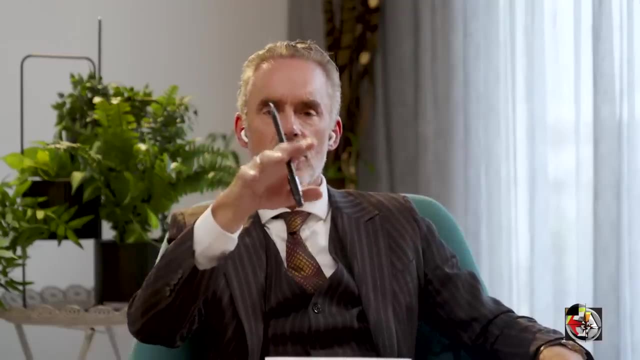 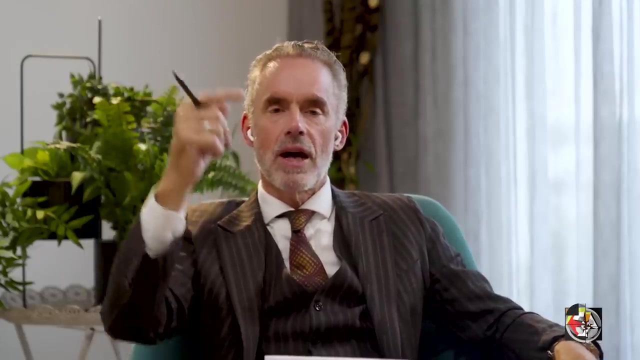 by their distributed computation. And it does that with trait neuroticism which is your own, genetically mediated- mostly partially at least genetically mediated- initial propensity for those error messages to propagate up the hierarchy. You might say they're more likely to propagate up the hierarchy. 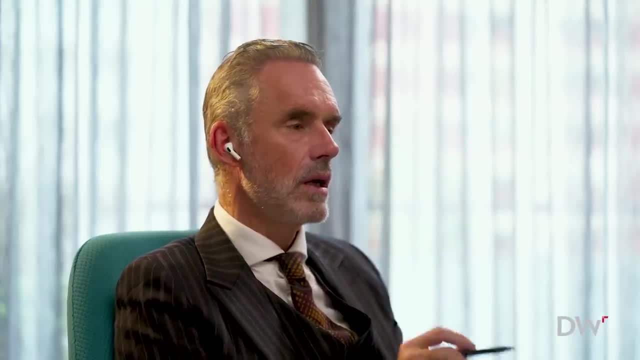 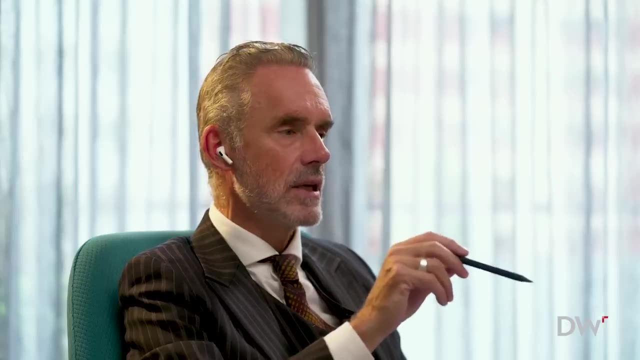 the internal representational hierarchy of women, And women are more sensitive to negative emotion than men, And I think the reason for that is because they have to take care of infants. it makes sense for them to be more sensitive to smaller errors of prediction. 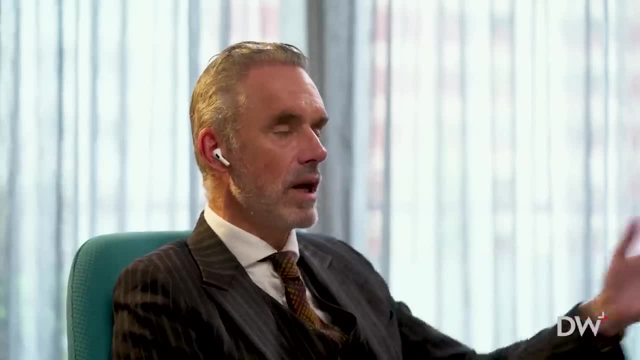 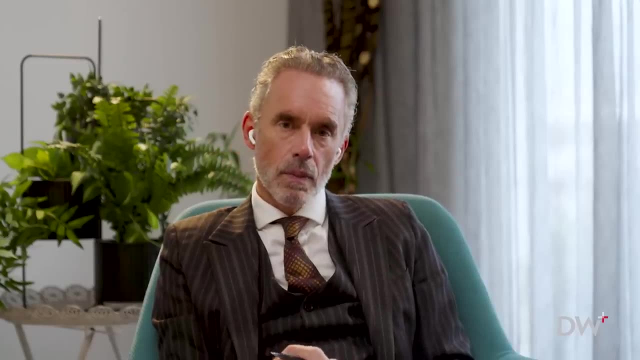 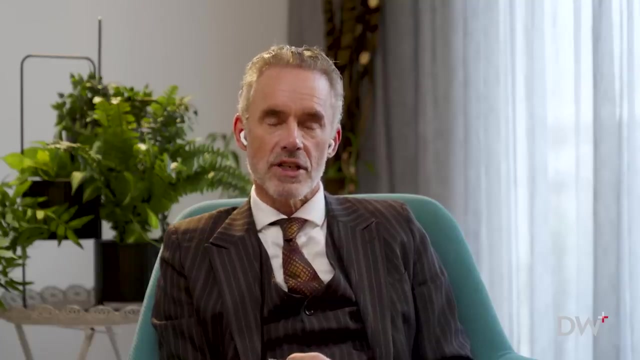 Because the consequences for someone who's truly vulnerable, an infant, can be cataclysmic, And so, anyways, there's a lot in that, But that's a theory of the relationship between hierarchical processing of entropy and the proclivity for depression. 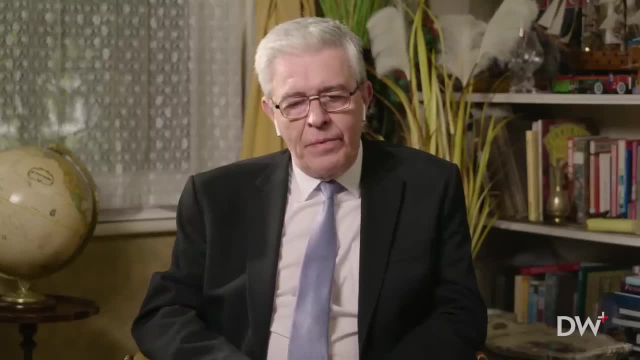 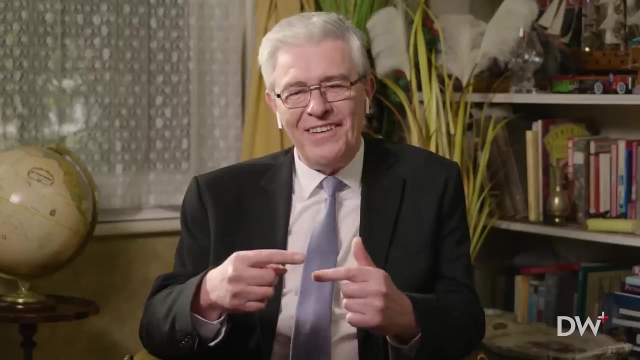 Yeah, There is a lot there, But it all makes perfect sense from the point of view of hierarchical inference in the brain, particularly hierarchical predictive coding. So, if you'll indulge me, I'm just going to say exactly what you said, but using slightly different words. 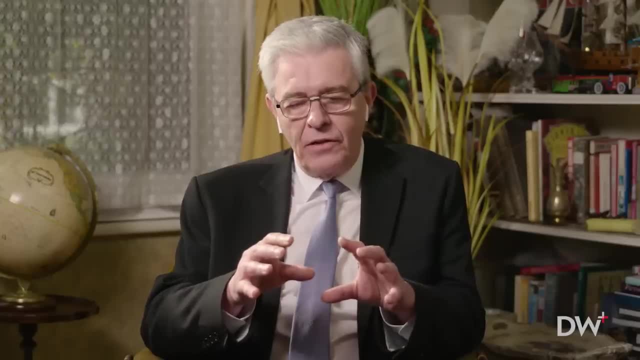 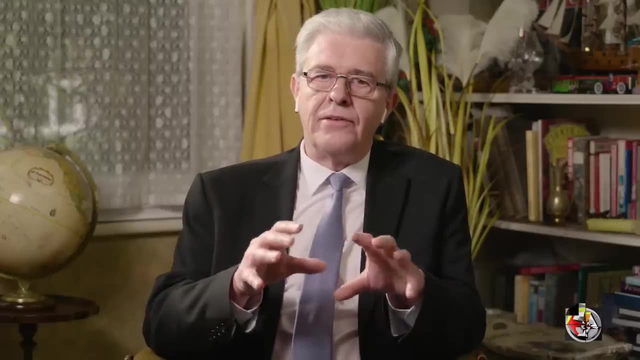 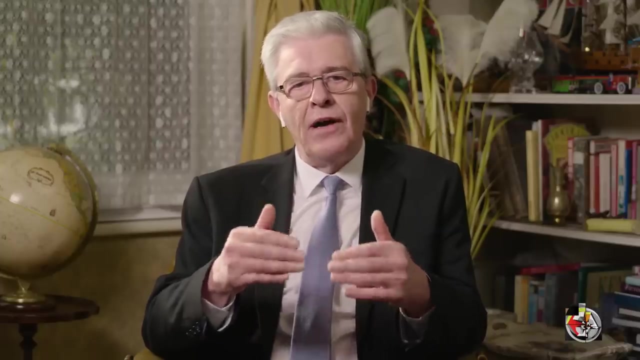 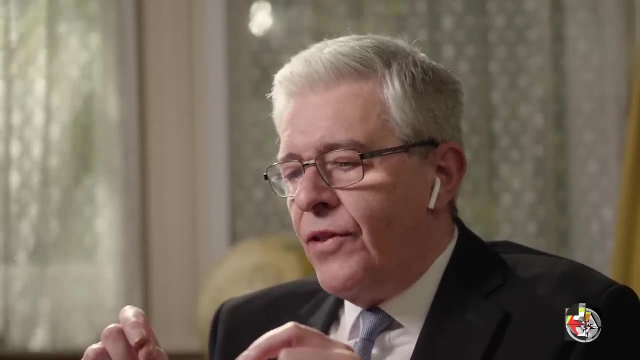 Because I think that that notion that you've just described, and its implications for things like depression, has a lot of construct validity in relation to sort of more machine learning, artificial intelligence, formulations of this hierarchical processing. So one way of articulating that insight is to think of 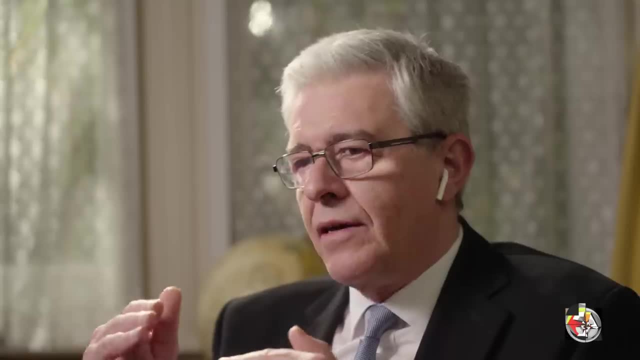 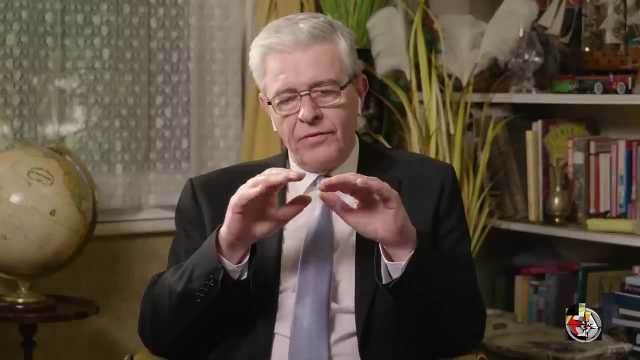 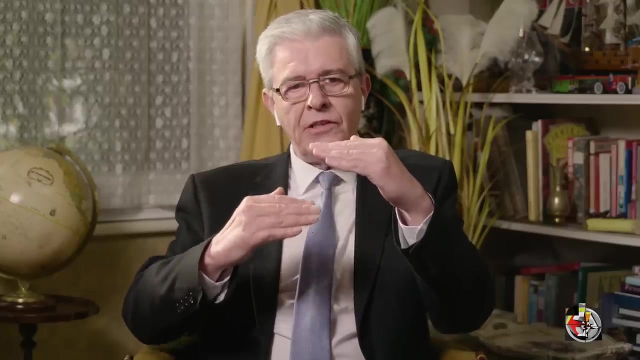 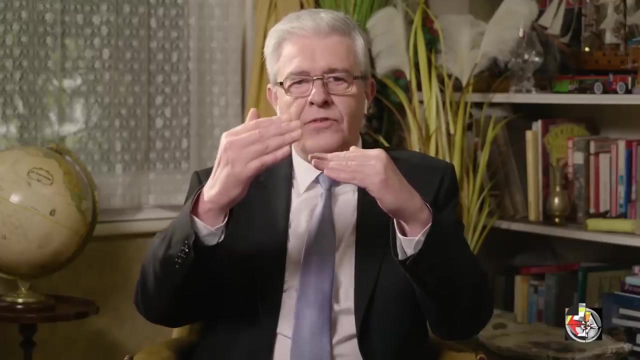 the message passing in a hierarchy that literally is our brain, under the rubric of predictive coding. So in this sort of framework or scheme, the idea is that each level of the hierarchy receives information from below and it tries to explain away the information based upon top-down predictions. 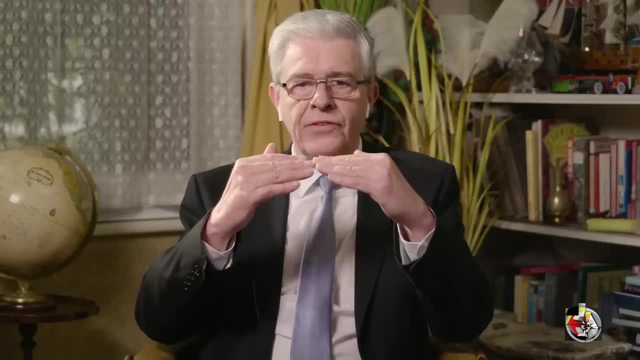 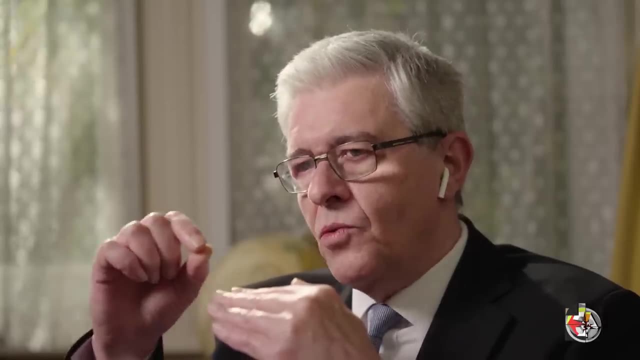 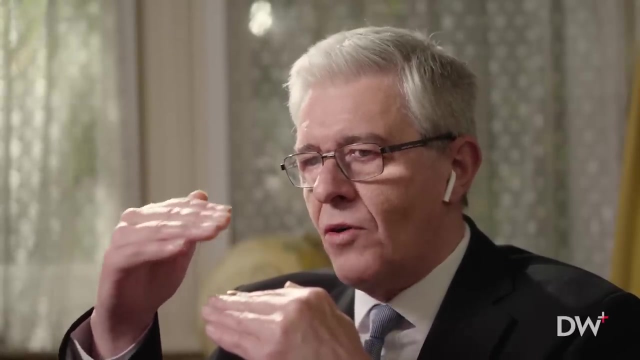 And that which cannot be explained is ensuing, and that is the top-down prediction error. So these are the mismatches you were referring to before, And then these prediction errors are used to revise beliefs or representations, sub-personal beliefs or representations at the higher level. 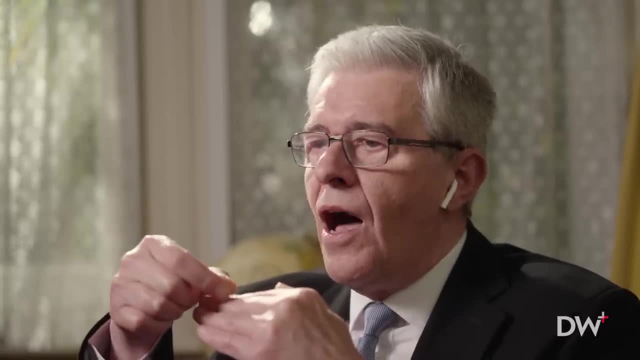 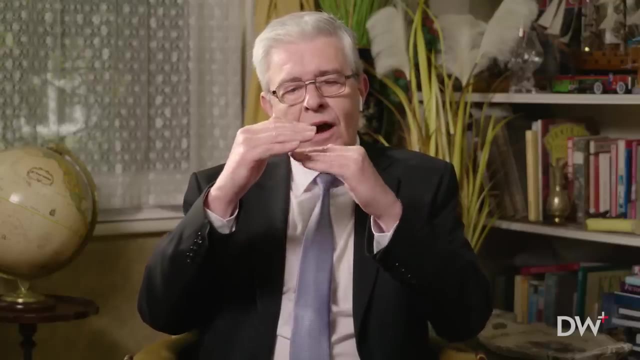 at the more abstract level until the top-down predictions are more apt to explain away what's going on below. Now, the key thing about this architecture? well, there are a number of key things, and we've spoken in depth about a number of them. 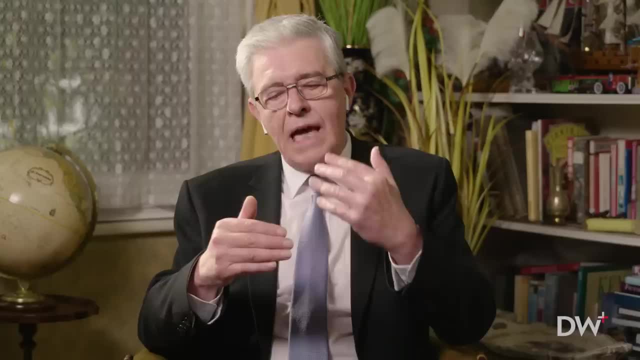 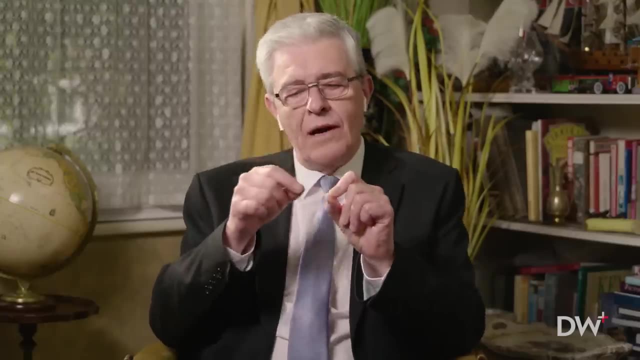 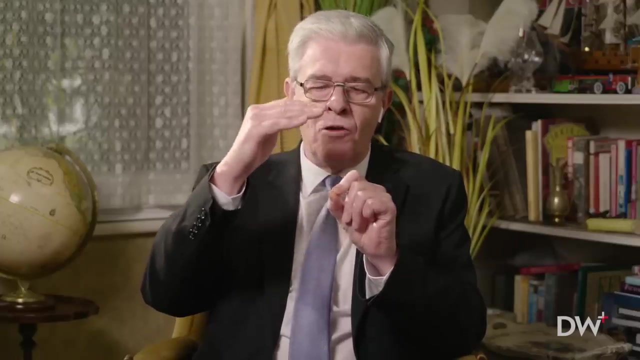 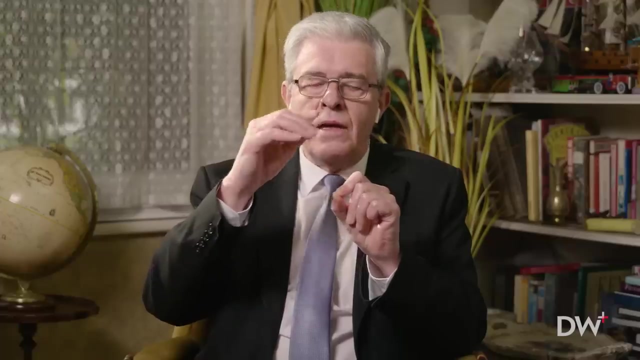 but if you're framing like this, then the game of minimizing surprise is just the game of minimizing prediction errors. But how are you doing that? Well, you're explaining away what's going on down there, based upon higher-level hypotheses or belief structures or expectations or representations in your hierarchy. 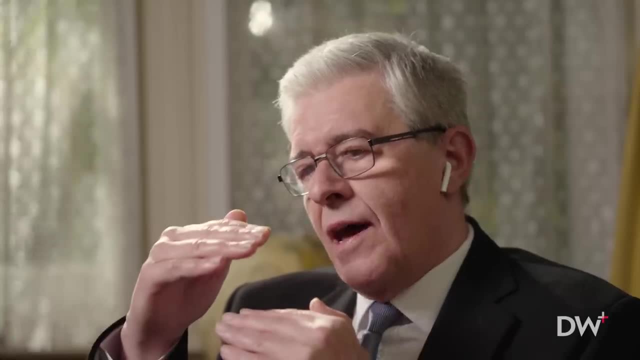 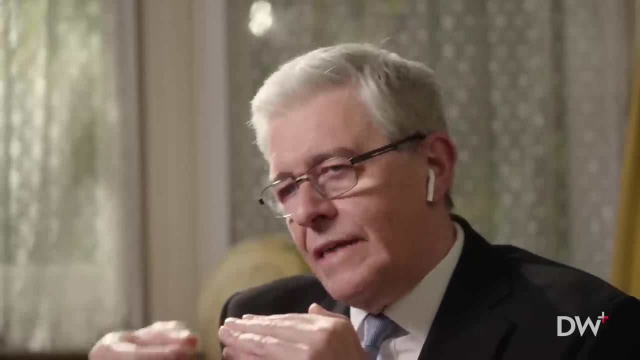 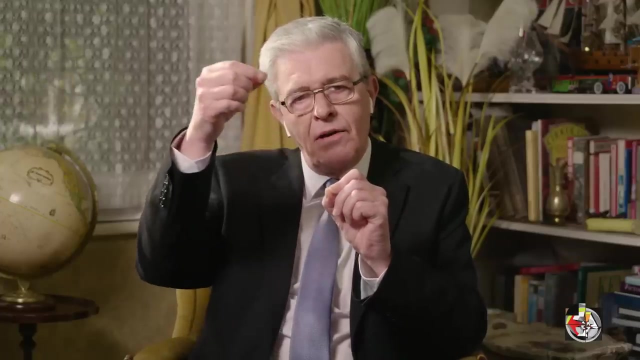 The key aspect of this sort of message-passing scheme, this predictive coding scheme, is that it really matters how much weight you afford to the prediction errors that are passed and ascend the hierarchy- You use the word sort of cascading up the hierarchy. 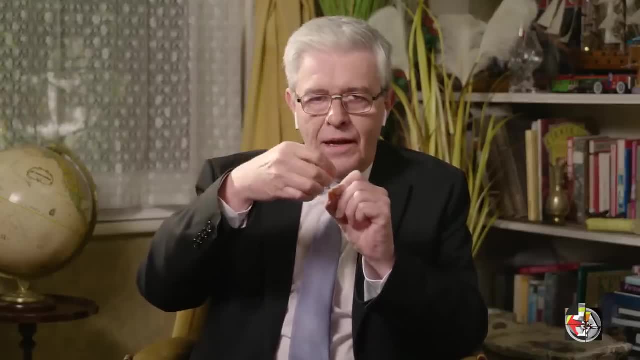 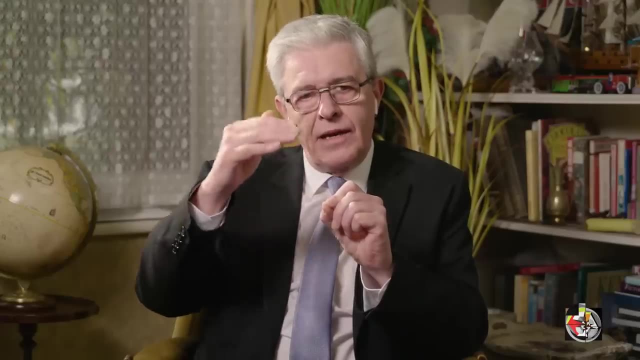 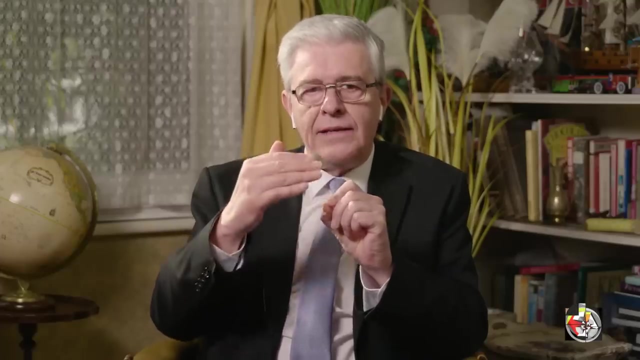 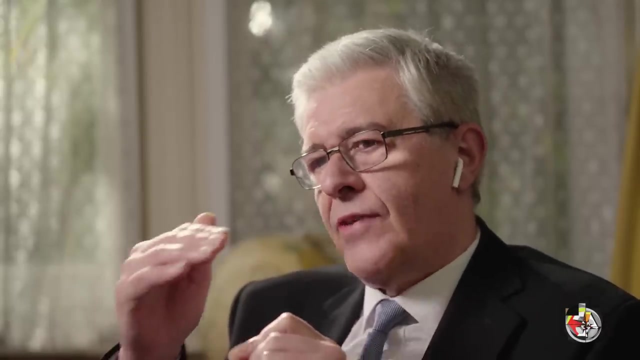 And this is exactly the image that an engineer would have when building a predictive coding machine. And the degree to which they cascade up is exactly proportional to the gain or the sensitivity that is set by the neuromodulators, in this instance serotonin. So the resistance now is set by having entrenched 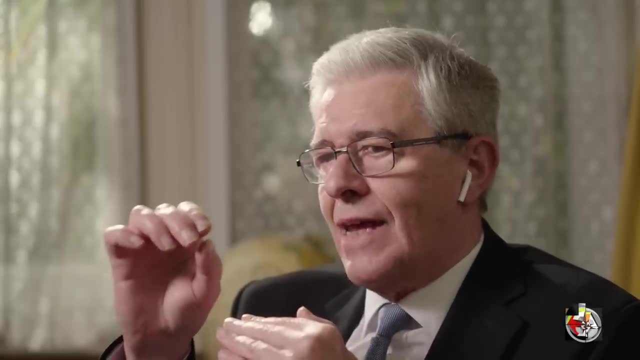 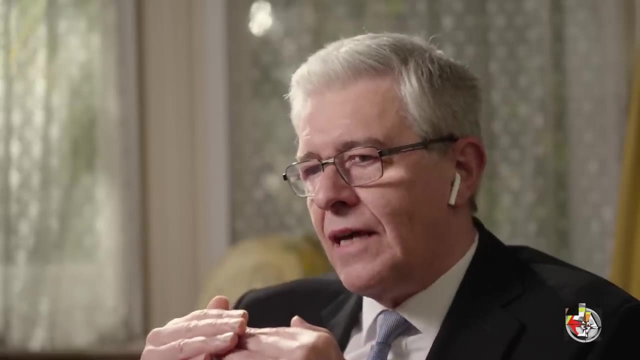 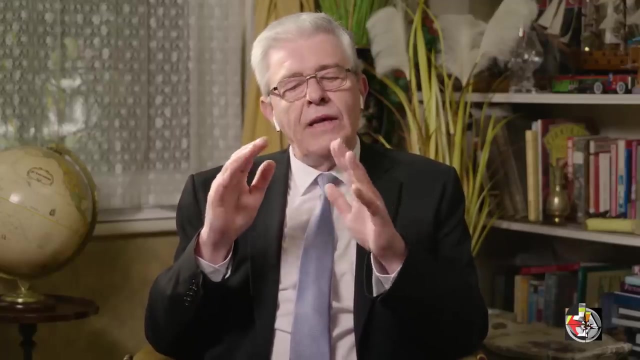 if you like, beliefs about this level of the hierarchy. relative to this level of the hierarchy, that is mediated by decreasing your sensitivity to the ascending prediction errors. So, if I read your Well, let's take depression, And I'd also like to talk about psychedelics. 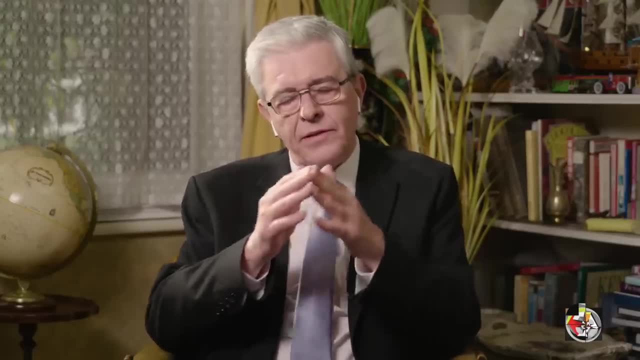 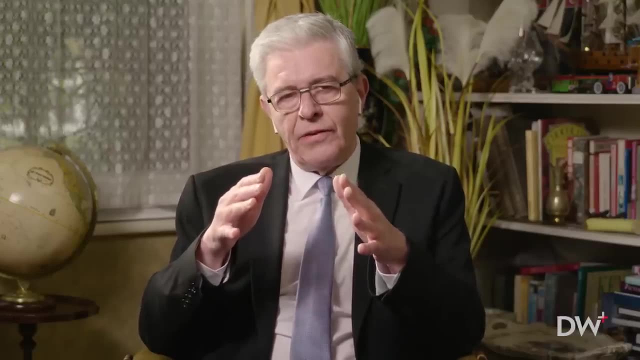 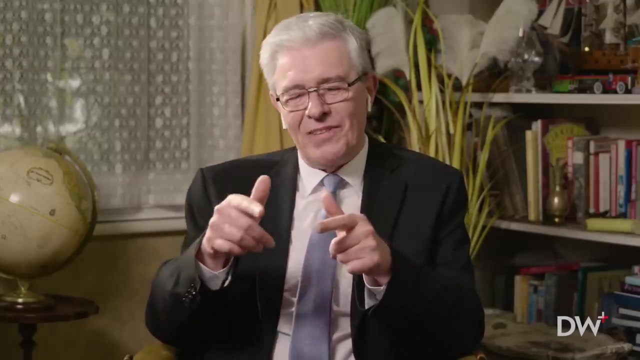 because they act upon exactly the same neurotransmitter systems. But let's just take depression, which is a particularly pernicious, I think, sort of set of narratives to find yourself in, because I'll just cut to the denouement of this argument. 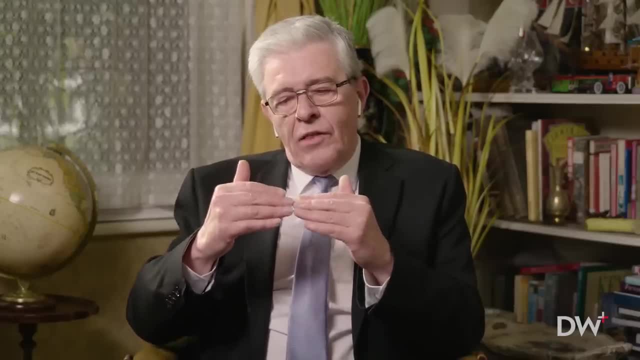 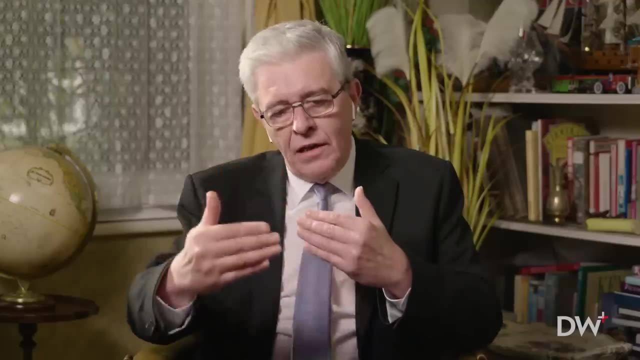 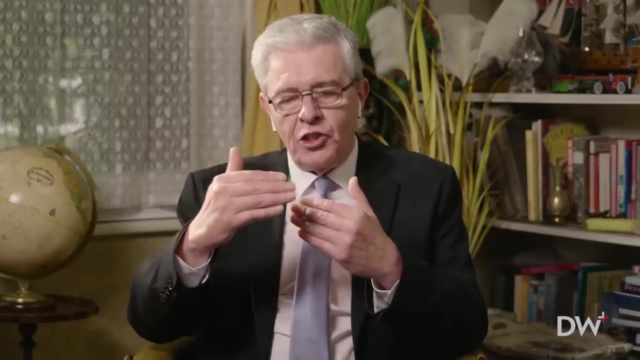 In many senses, this predictive coding formulation, when put in the context of predictive coding, it's not just about me discovering and learning and optimising my models of the world. It's all about accumulating evidence for my explanations that are updated in a way that minimise the prediction errors. 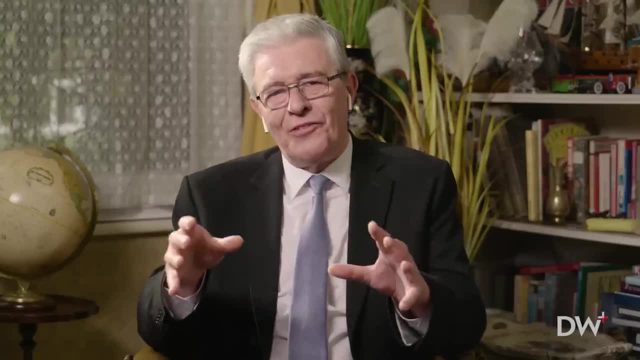 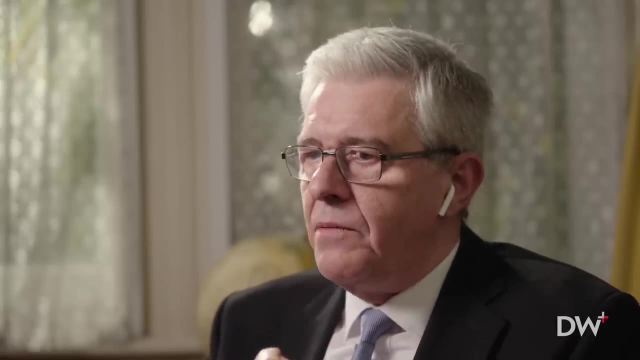 But in accumulating evidence I have to choose to expose myself to the world. I have to actively sense and go out there. Depression is pernicious because of course a lot of the symptoms of depression prevent you going and getting evidence that you're not this kind of person. 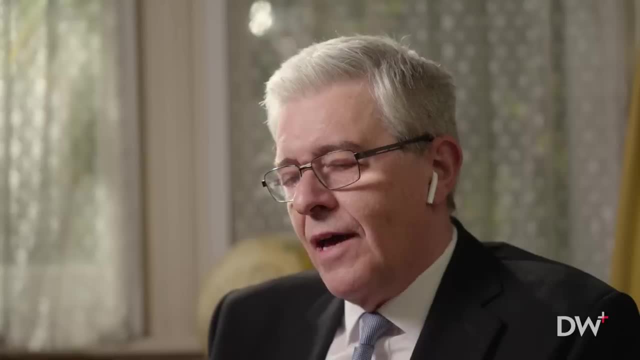 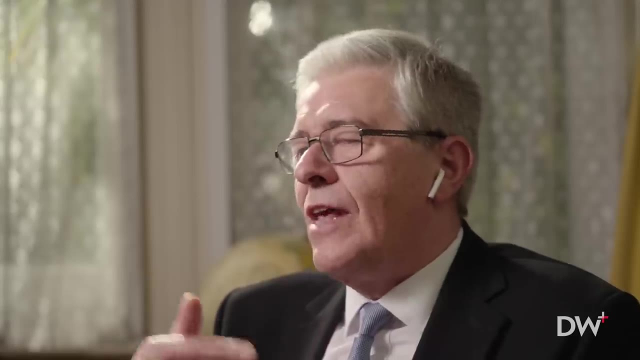 or that you could have coped with this particular scenario. So depression, I think a little bit like the cocaine using that it has a slightly self-subverting or self-maintaining aspect that sort of hijacks the normal ways that we get out of it. 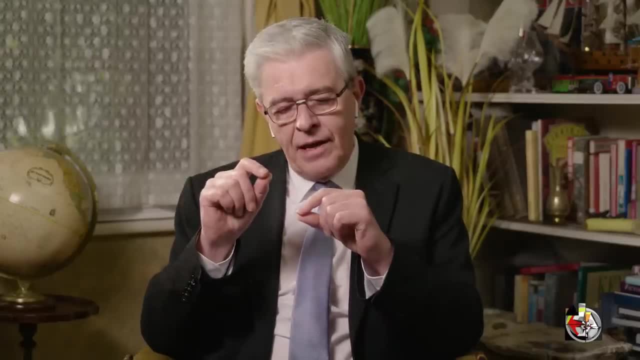 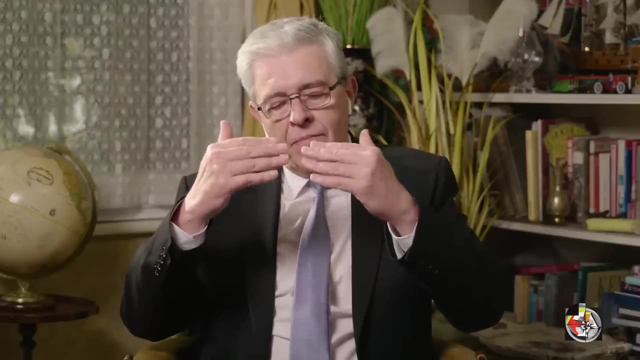 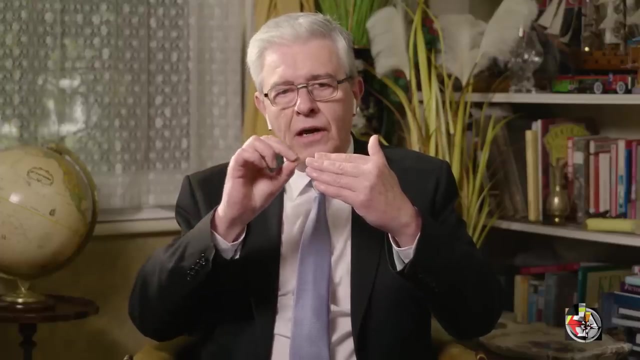 But just to come back to this sort of, I think, quite fundamental notion of sort of inducing, either through physiological setting of that resistance or that, what we call precision. So we call it the precision, It's the inverse, uncertainty, It's the reliability. 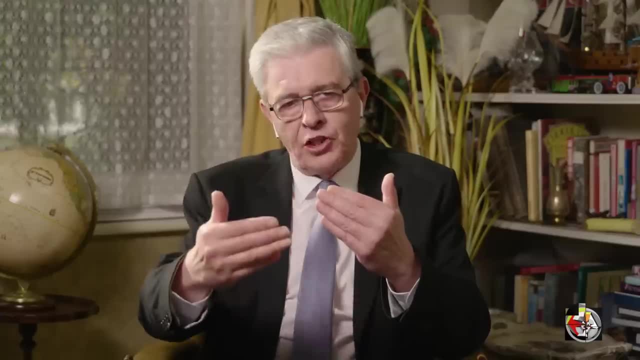 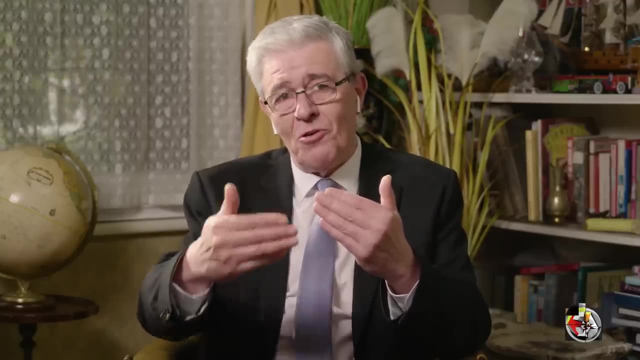 that you can afford these ascending prediction errors that tell you you've got to change your mind, You've got to find a new way of coping, either in a marital relationship or just in terms of where you're actually looking from many, many different levels. 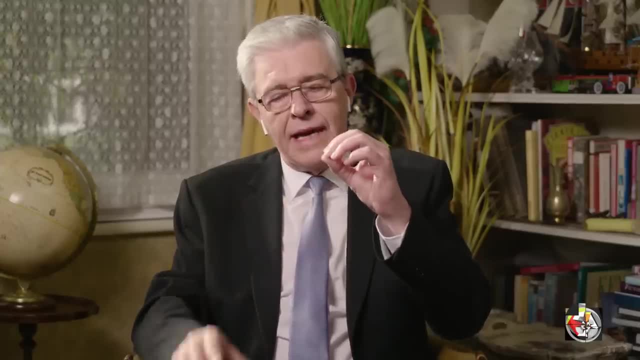 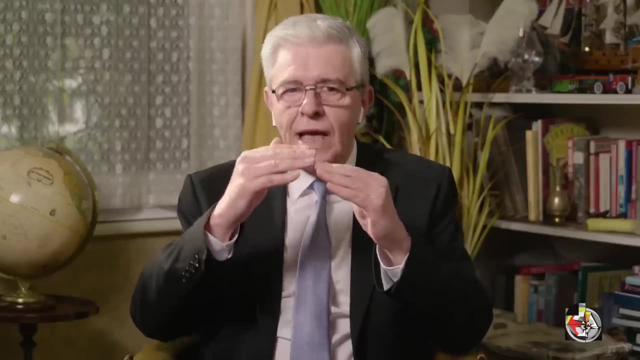 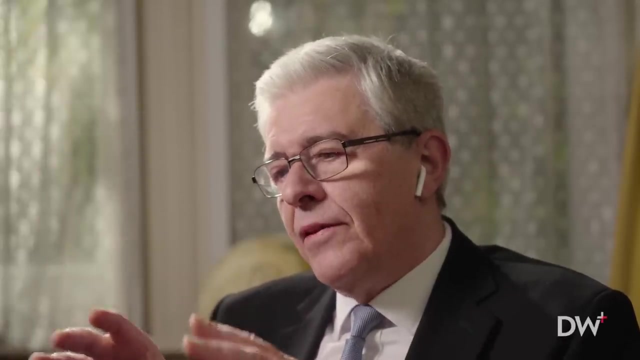 So this notion of precision translates into exactly what the neuromodulators control, which is the excitability of the neuronal cells that are broadcasting the prediction errors to the next level, And as such, that looks very much like attention. You know we were talking before. 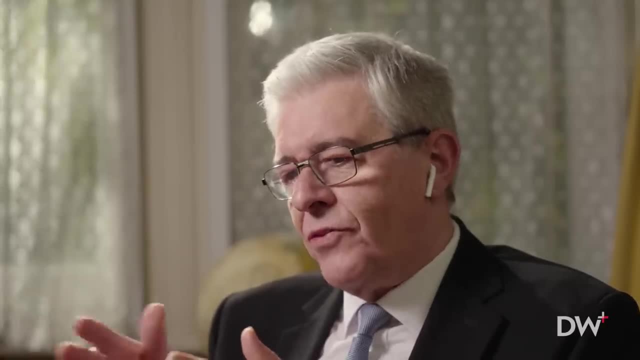 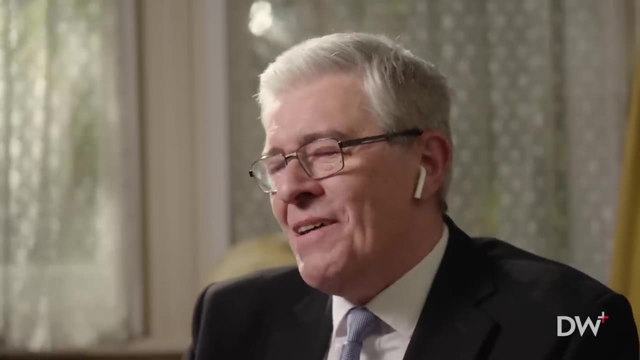 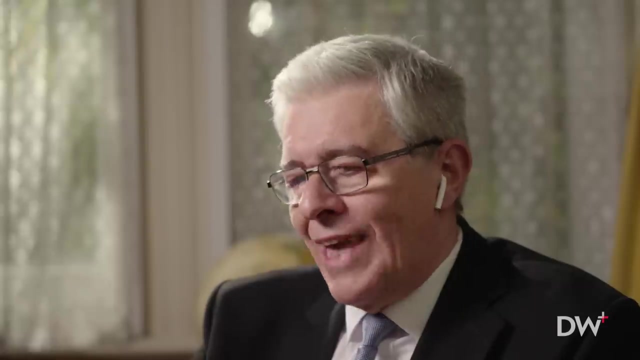 about sort of change blindness, and we just don't seem to be able to attend to things that are irrelevant, to the extent we don't even notice changes when they occur if we don't assign them the right kind of informativeness or salience or precision that is necessary to explain. 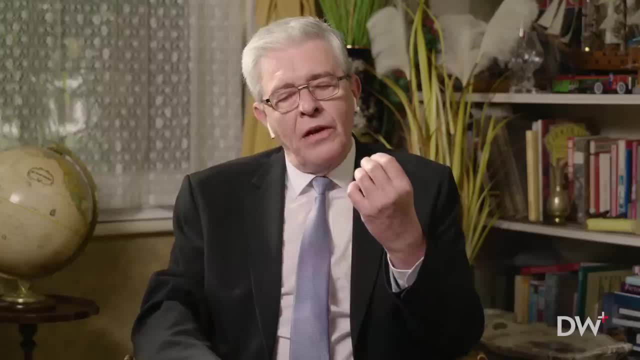 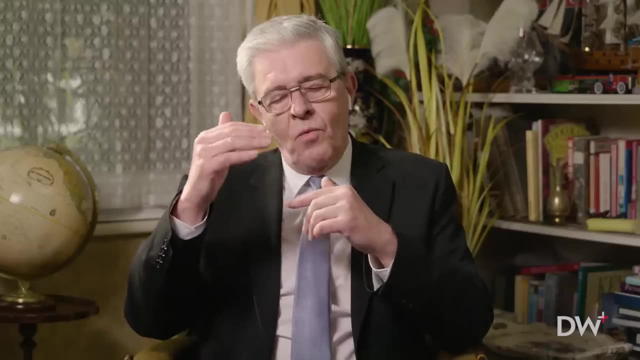 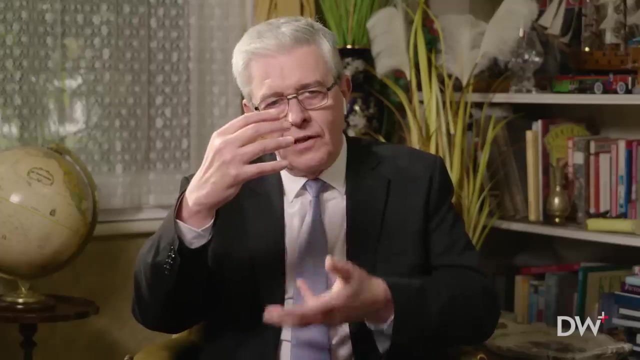 the narrative that's unfolding before us. So one way of reading this sort of state, this serotonergic state or continuum where these high-level, hierarchically higher-level beliefs are recalcitrant or insensitive to the lower-level, information is the remarkable and important capacity. 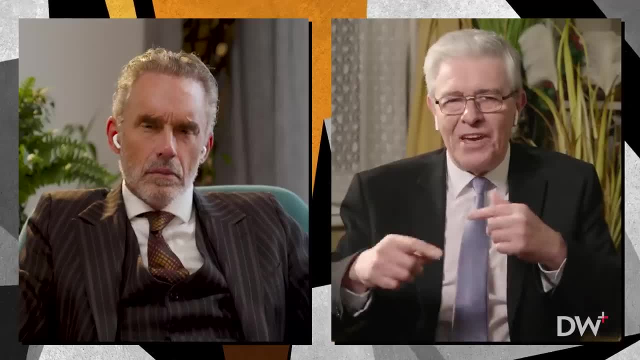 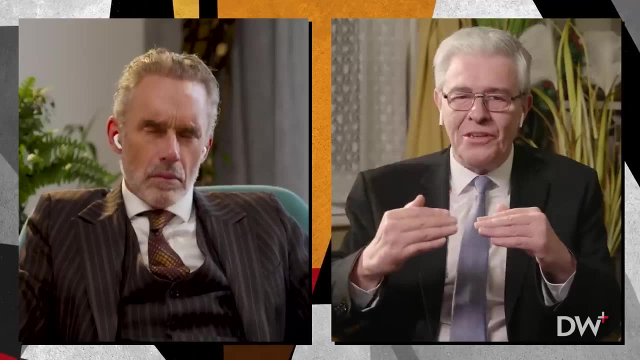 to ignore stuff that is irrelevant, And what you're saying is when it happens three times. perhaps I shouldn't be ignoring it anymore and I now have to redeploy the precision, refocus my neuromodulator systems, perhaps away from serotonin at the top. 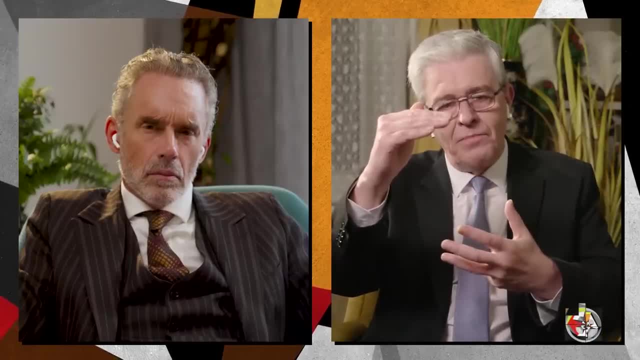 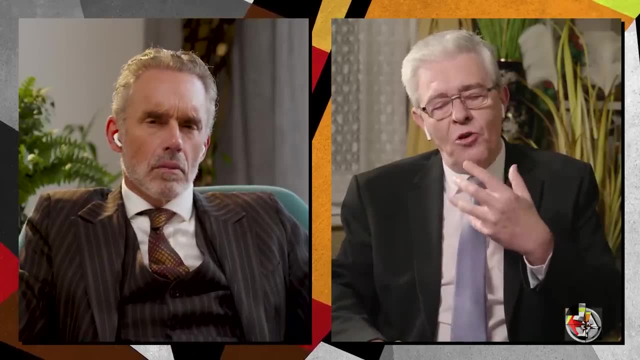 and perhaps, more to say, acetylcholine at the bottom. just given the anatomy of these neurotransmitter systems, that would indeed render me in a state where I'm now much more attentive to what's actually going on out there. and what is actually going on out there. 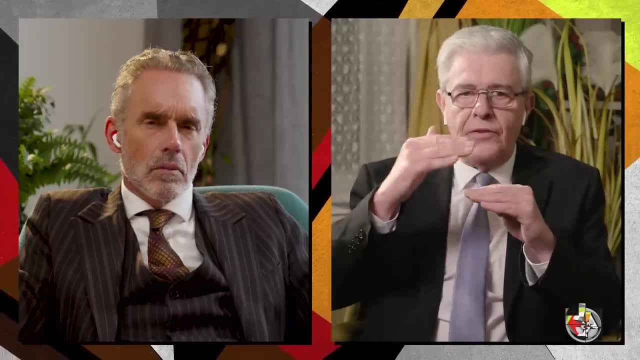 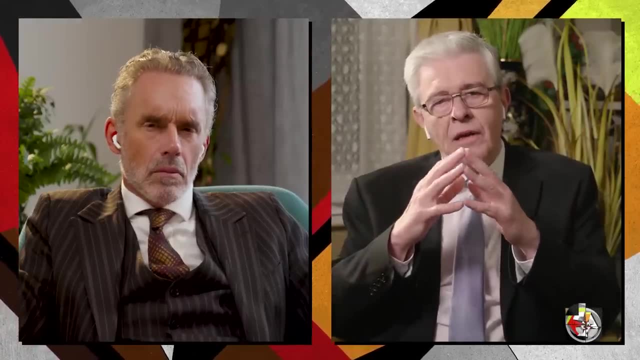 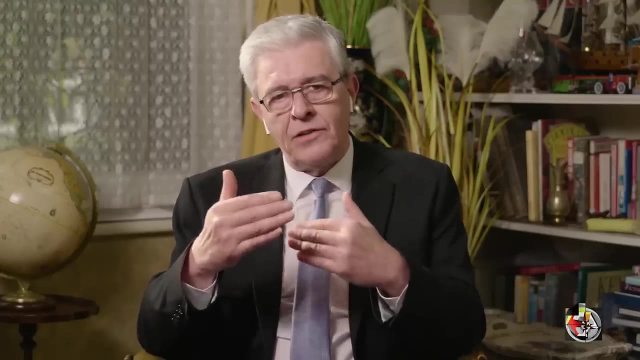 will engender prediction errors that will change my mind or indeed change my generative model. that entails this hierarchical structure. So I think everything you've said makes perfect sense from the perspective of the mechanics of belief updating and structure learning in the brain, seen through the lens of an engineer. 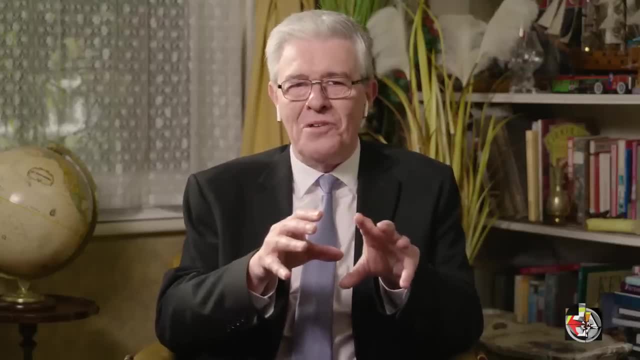 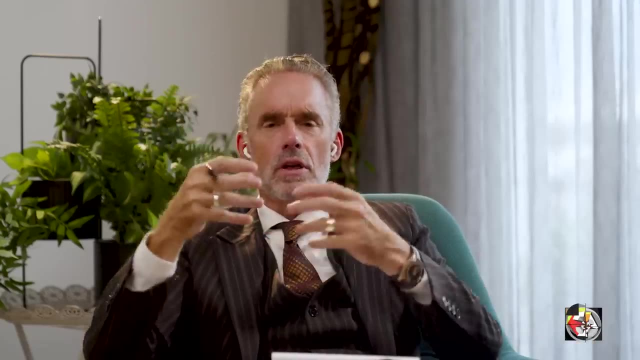 who thinks about the brain as a predictive processing or coding machine. So what does acetylcholine do? What does acetylcholine do? You contrasted acetylcholine with serotonin and you associated acetylcholine with increased precision of attention. 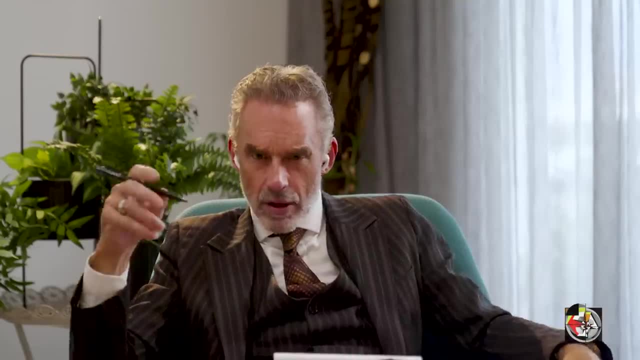 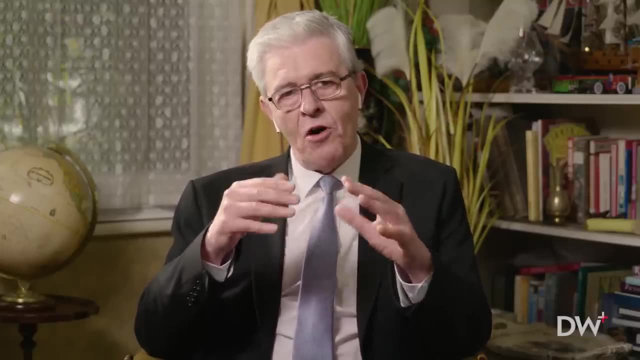 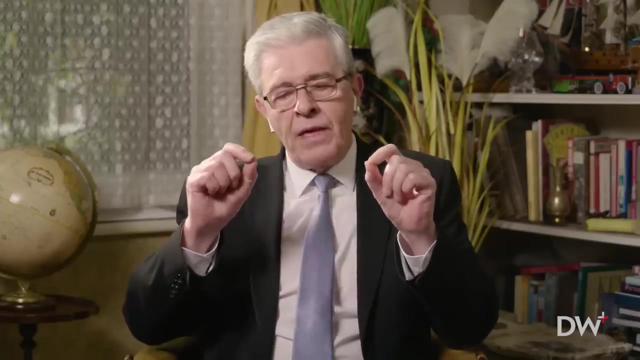 focused outward and that's at the lower levels of the hierarchy. Yeah, So this is a vast simplification, but I think it's sort of a useful mnemonic. So if you think about the hierarchy that you were describing before and you now want to discriminate, 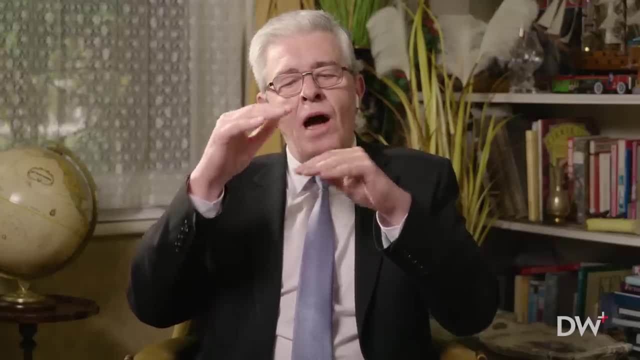 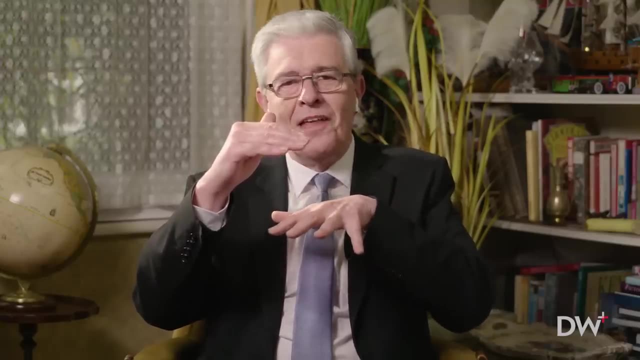 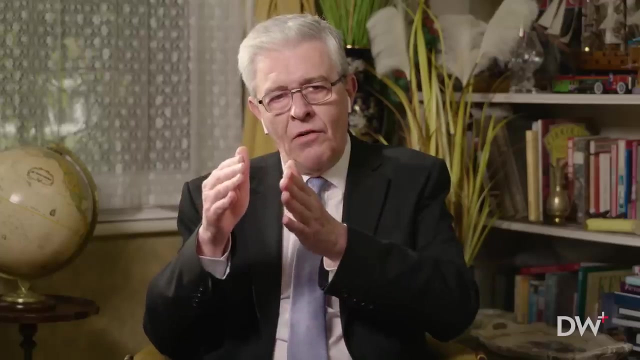 between a situation where all my high-level beliefs are insensitive to changes at the lower levels. so this would be say, the dominant alpha male, very, very self-confident, has very precise what we sometimes, in a Bayesian reading of this predictive coding scheme, called prior beliefs. 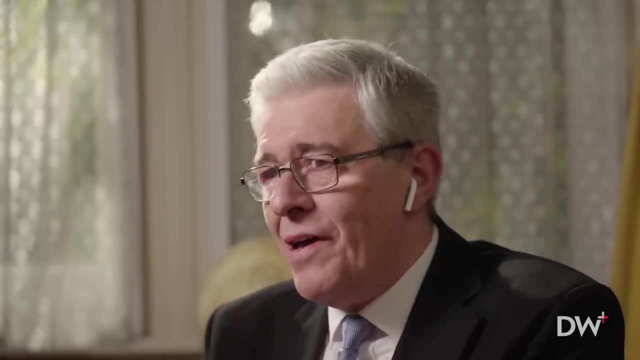 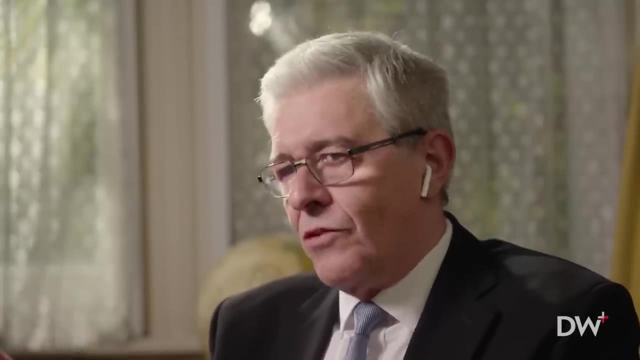 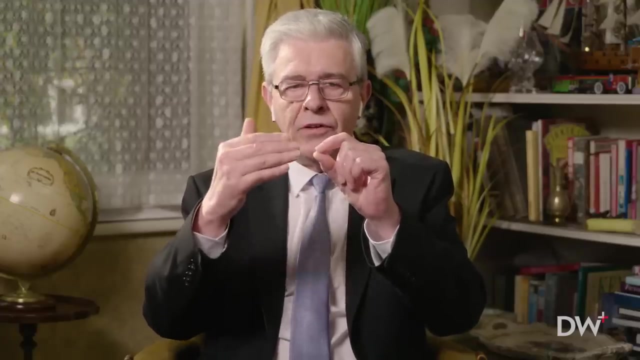 Prior beliefs. this is the way I behave, this is the way you behave, and I am going to realise, instantiate those fantasies by behaving in this way, And indeed that's what normally happens. So I'm very confident, and that translates into a high degree of prior precision. 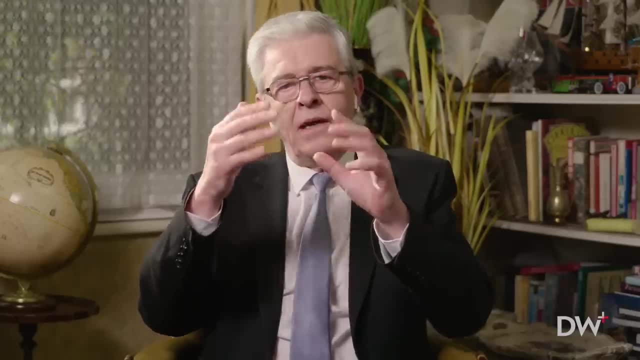 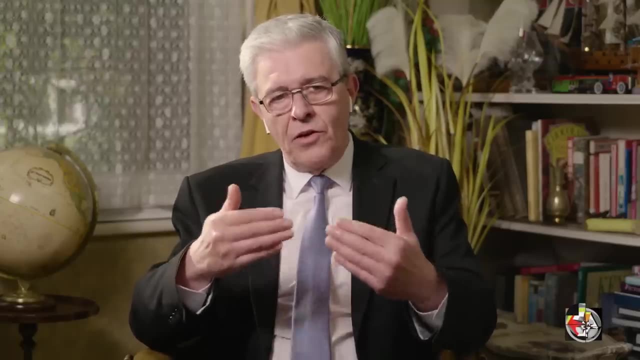 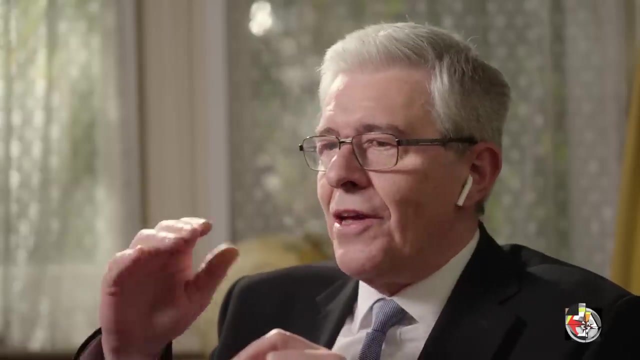 which could be mediated by things like serotonin. The equivalent neurotransmitter at the lower level is often just looking at the neuroanatomy and the neurochemistry and physiological experiments. a similar role might be played by acetylcholine. So you can think of if you like. 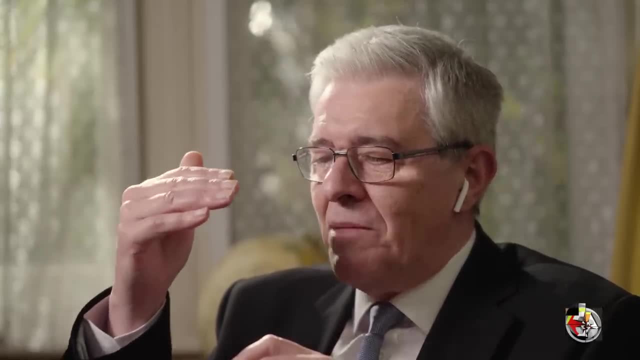 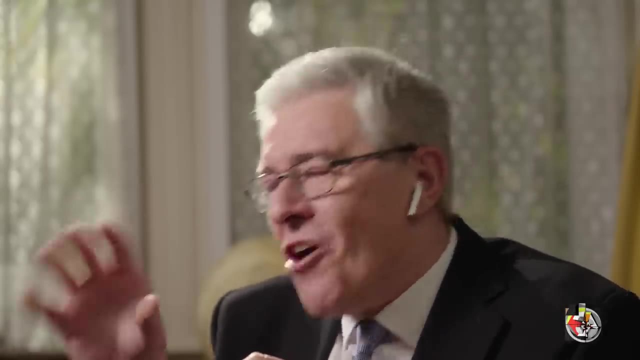 too much prior precision- as being mediated by serotonergic neurotransmission. and of course you know as well as I do that it's a very complicated game with different receptor subtypes and sort of inverted U behaviours, so I'm not saying it's more or less. 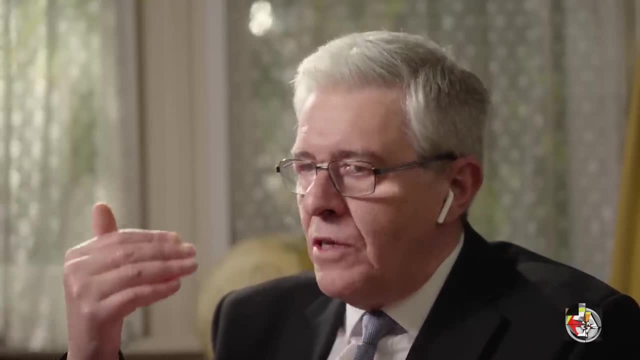 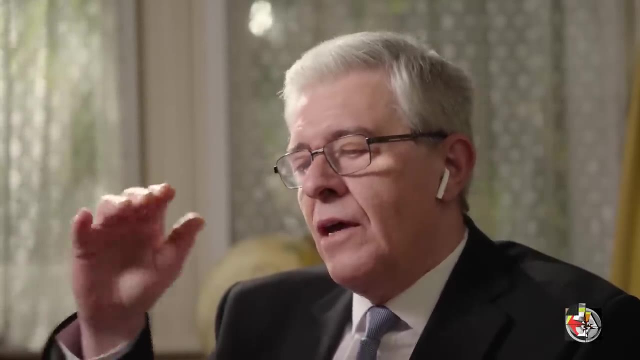 but certainly rests upon the way that you deploy your serotonergic firing. that will have a profound influence on the higher level prior beliefs. Exactly the same kind of role may be ascribed for cholinergic neurotransmitters. So you've got cholinergic neurotransmission. 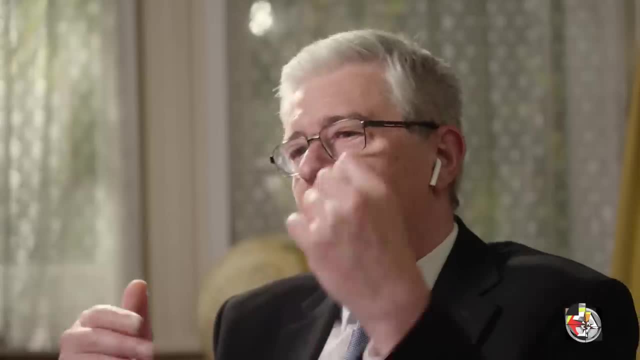 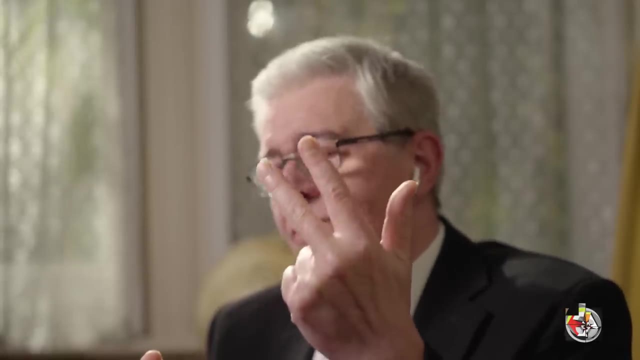 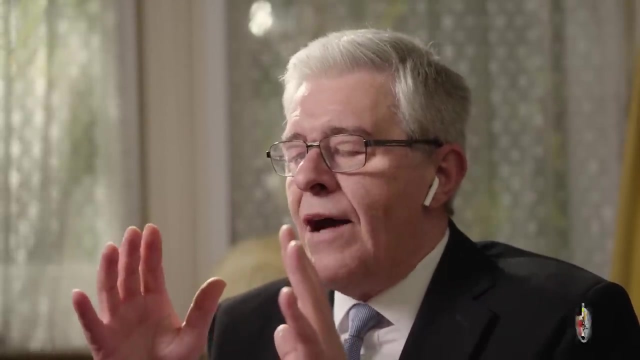 from the nucleus basilaris of my heart, which is another neuromodulator. so you've got dopamine, you've got serotonin, you've got adrenaline or norepinephrine, you have oxytocin. there are lots of them and they may all have particular roles. 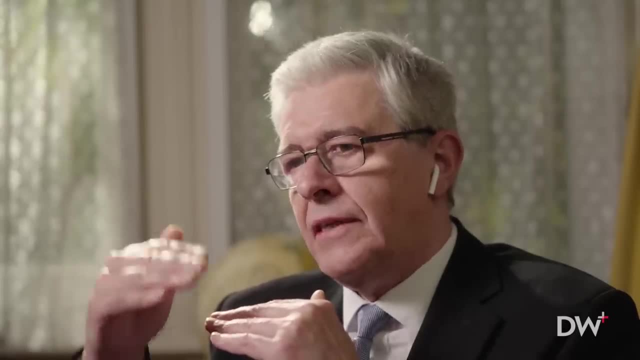 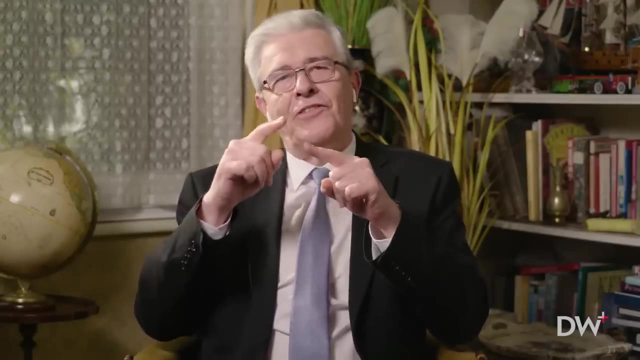 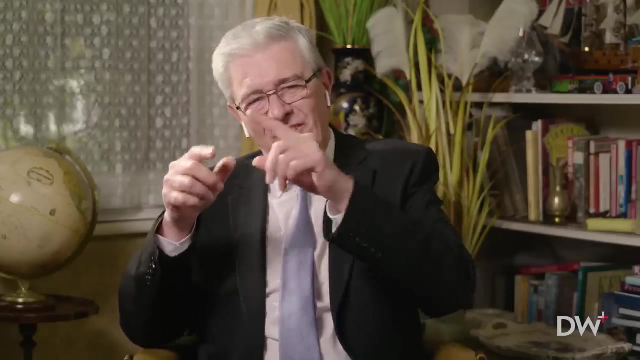 in setting the precision or the recalcitrance or the sensitivity at different hierarchical levels. So it's generally in my world. if you think of serotonin doing one thing, then the complement of that is that the acetylcholine is doing it in the inverse way. 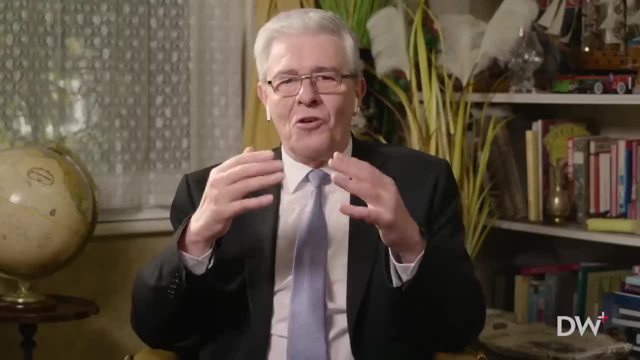 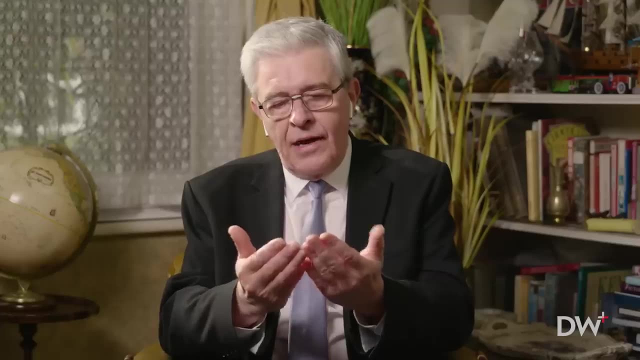 so it's sort of like a yin-yang. So when I talk about attention at the periphery, it's likely that that does sorry, at the low level of the hierarchy. it's likely that that does rely upon intact cholinergic neurotransmission with possibly aberrant serotonergic neurotransmission. that may be due to psychopathology or it could be due to taking drugs that affect, say, 5-HT2A receptors, like all the psychedelics, psilocybin, for example. Okay, so I want to go in. 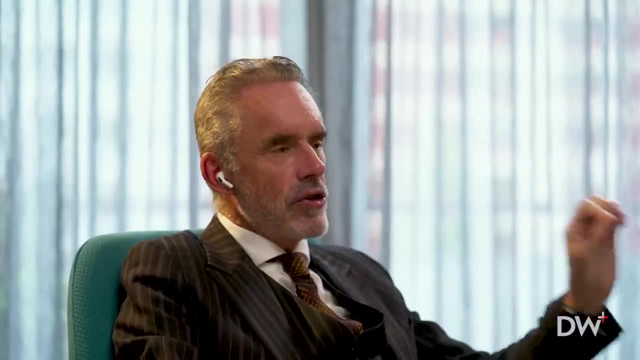 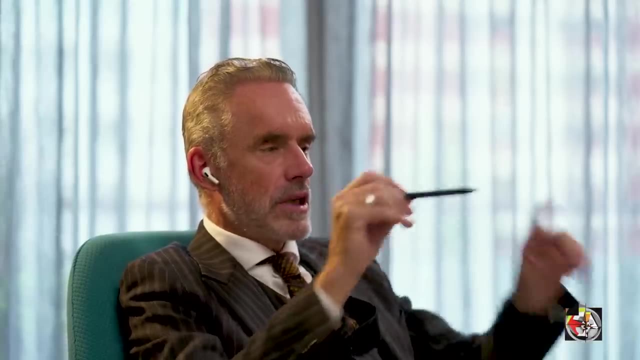 I've got three directions to go in now. The first question that's been lurking in the back of my mind for a while is: okay when you make progress towards a valued goal? let's say we inhabit a shared narrative and we're making progress towards our mutual goal. 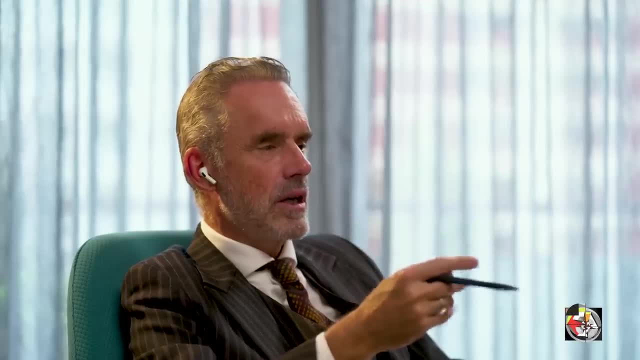 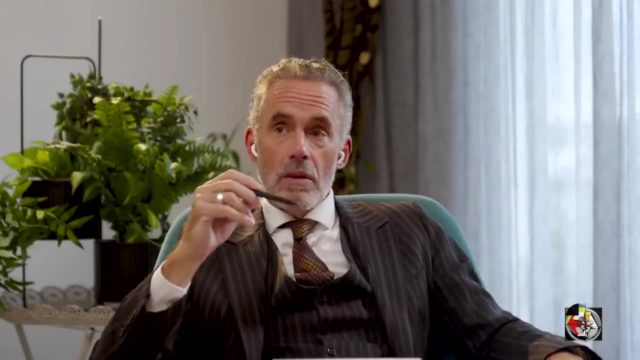 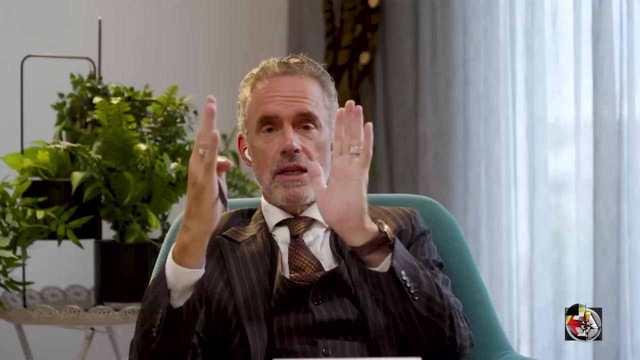 stated goal and when we see ourselves making progress we get a bit of a dopamine hit. Could you say that the fundamental reason for the positively rewarding effect of that movement forward is that as I move forward towards a goal, I decrease the entropy that still remains between me and the goal. 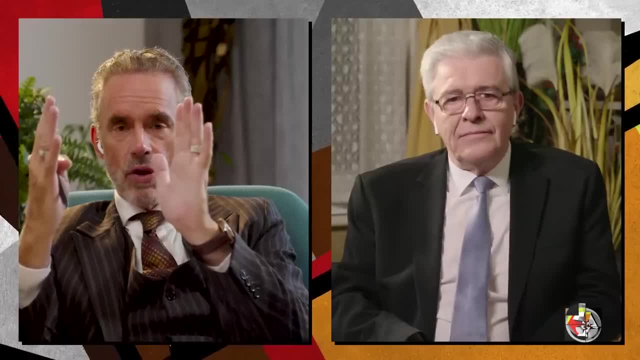 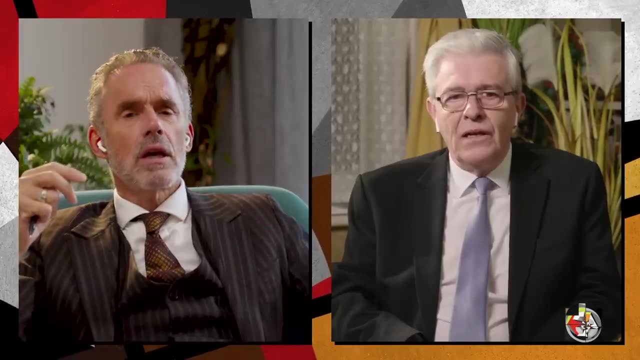 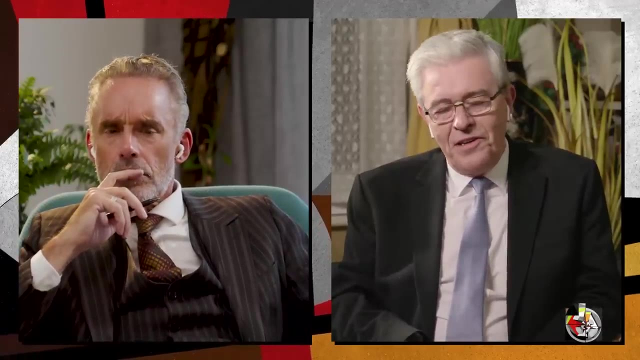 And so is even that reward. is even that movement forward readable as an entropy reduction? Yeah, absolutely, Because I'm closer now. so there's okay, okay. so I mean, see, I didn't know, I didn't understand that before. okay, okay, that I mean it's almost written into the 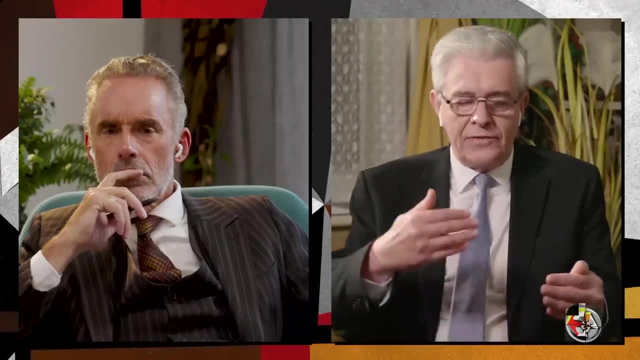 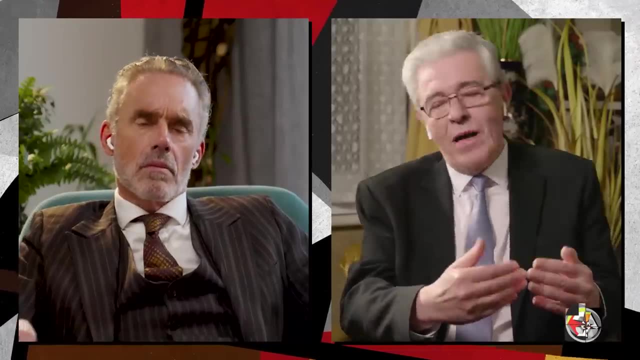 mathematical meaning of the word. so if entropy just is uncertainty- and as I get close to resolving that uncertainty- getting my fruit juice pleasing my wife or you know, being able to watch the news- you know, if it's an epistemic reward, it is just expected surprise. 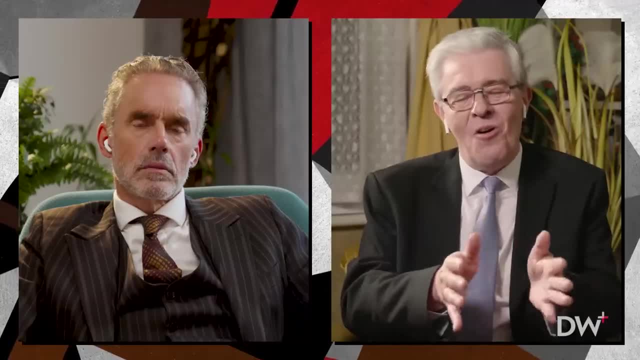 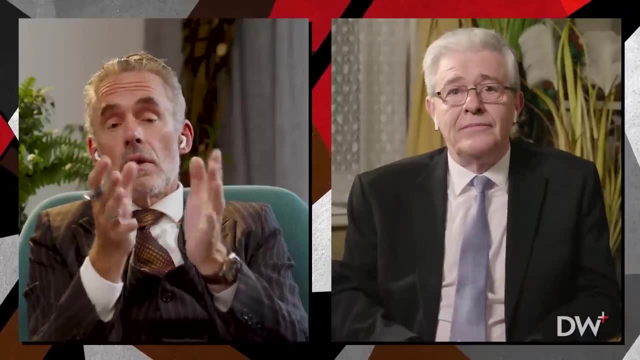 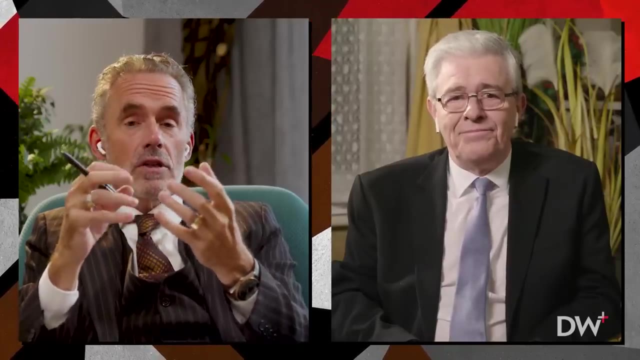 just is the uncertainty, and the closer you get, the more, the less uncertain you are. and all the evidence suggests exactly, partly because the well, the closer you get, the fewer things you have to compute in order to get there. So that's a good working definition of entropy. 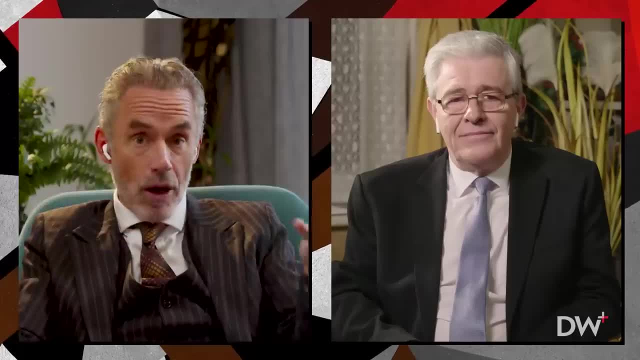 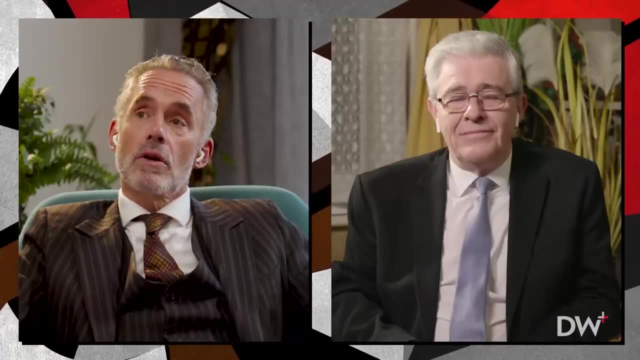 it's like I have to do less, I have to handle less doubt between me and my eventual destination. So that okay, so that's cool. so that reduces dopaminergic reward to a subset of entropy reduction- Right, and we should point out, you know living creatures. 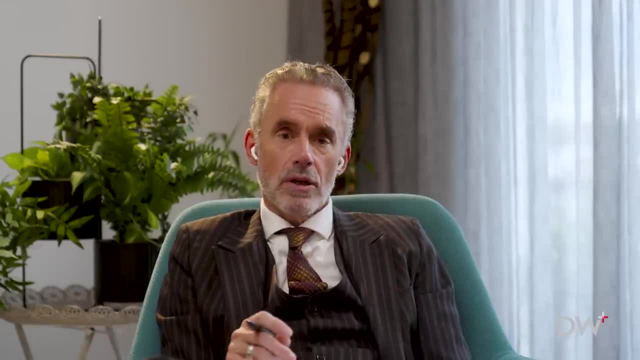 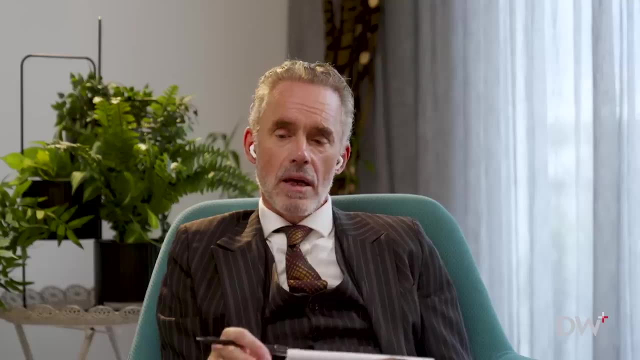 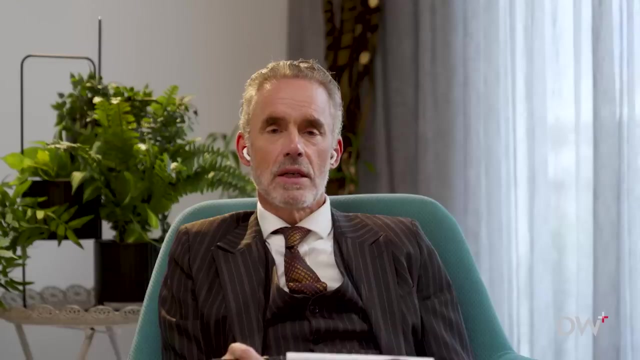 are always fighting entropy. they're trying to violate the laws of thermodynamics in some- not fundamentally, but in some- local sense, by insisting upon the maintenance of order in the face of this proclivity for things to go every which way at once. and so all right. 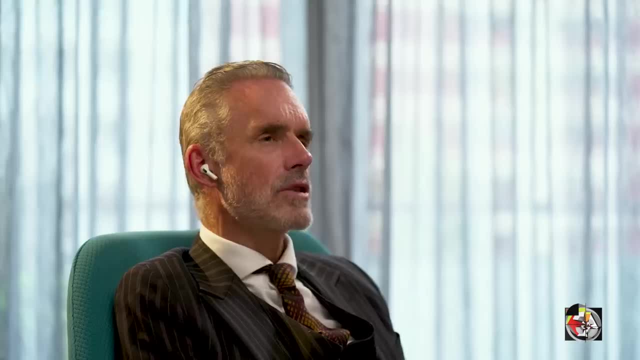 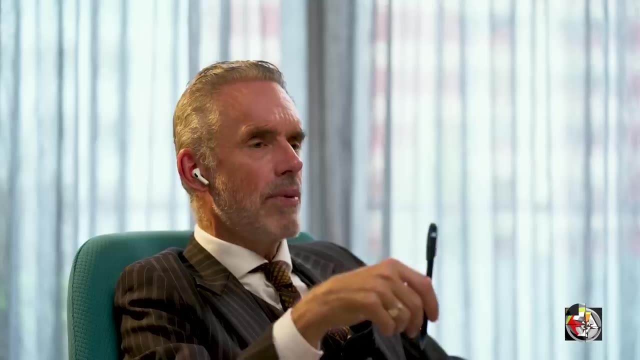 so movement towards, movement forward, towards a shared goal. that's also going to reduce the entropy between us, because it means if I can rely on you to be to accompany me as I move forward, that means I can predict you better. it also means that both of us 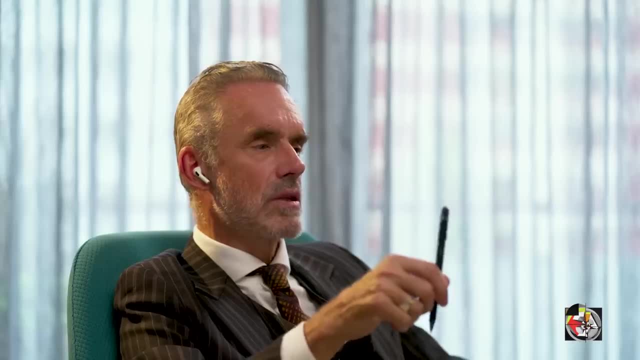 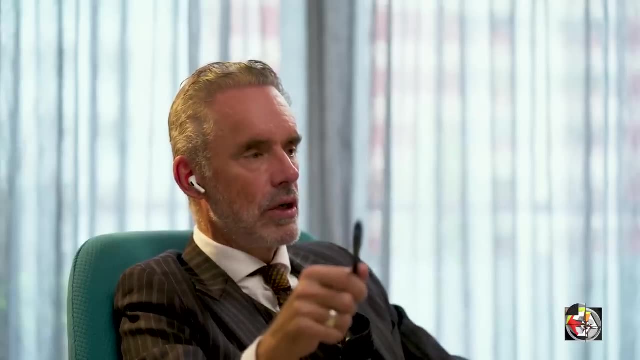 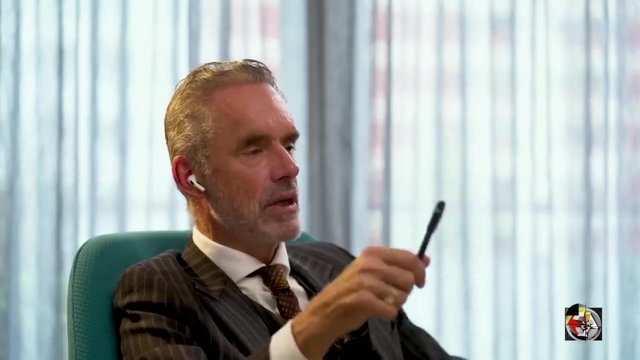 are now in a situation that's less entropic because there's less variability between you and me and the joint us and that shared goal, and so I've fortified my belief in your reliability and I've reduced my apprehension of your entropy. Yep, a physicist would love that. 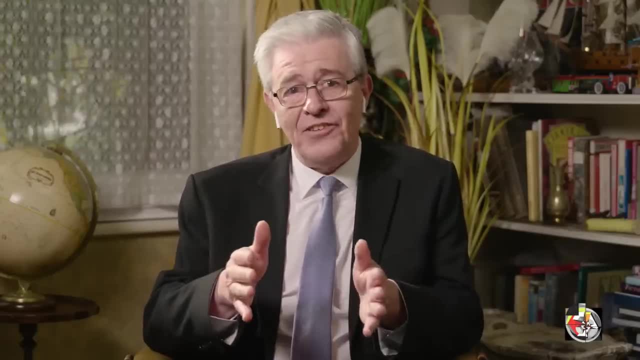 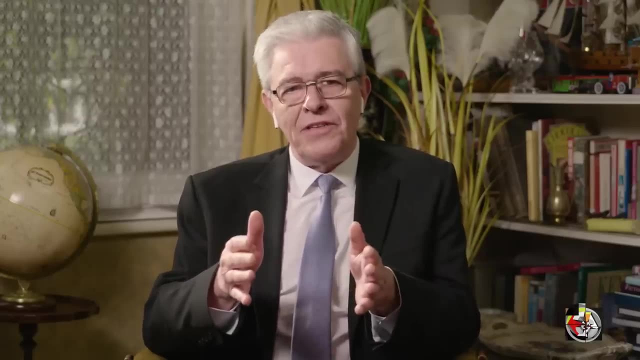 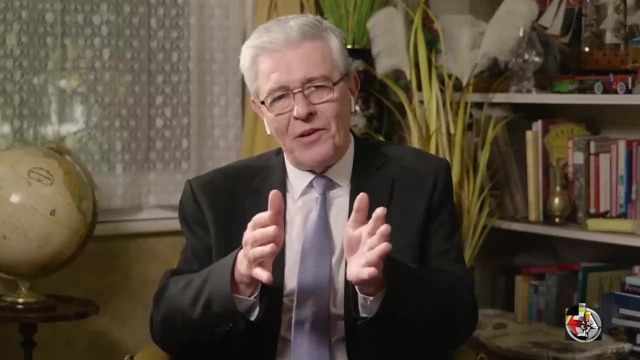 because, of course, the nice thing about entropy and free energy, which you know we're here sort of reading as surprise and prediction errors- is an extensive quantity. so your free energy and my free energy, or your entropy and my entropy, we just have to add them together because they're extensive. 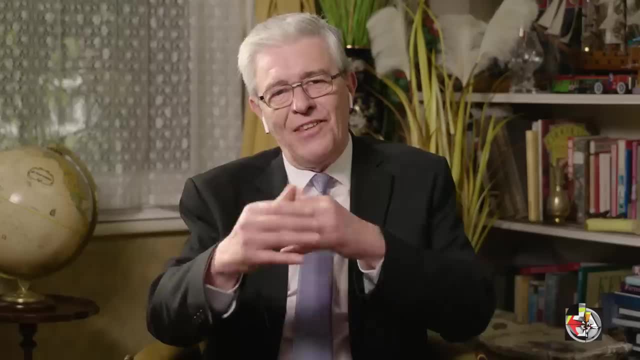 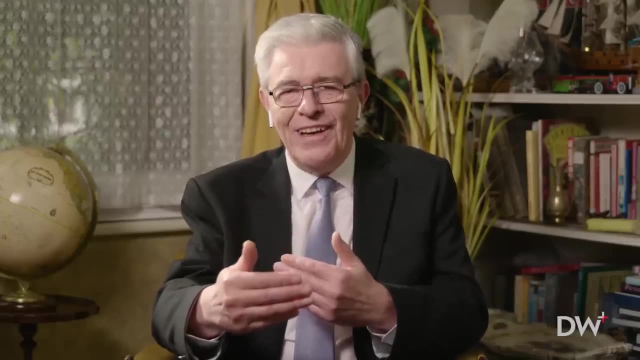 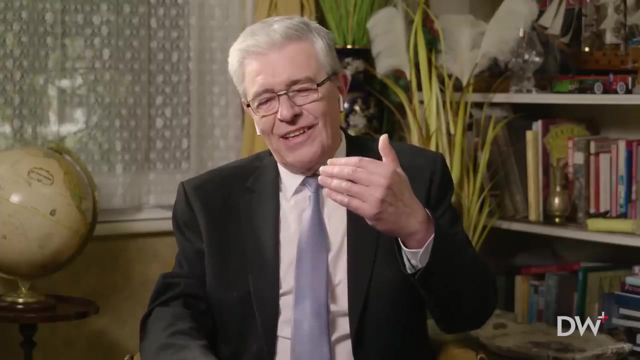 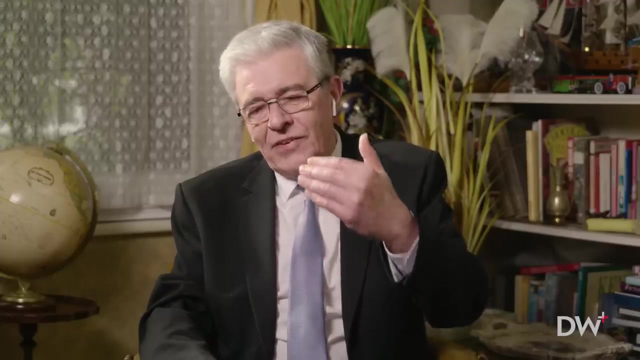 and then our free energy is exactly the sum of our free energy. so if we can both render our mutual worlds more predictable and less surprising, then our joint free energy will fall. and this, you know, this is, if you like, it could be read as a a statement of imperatives. 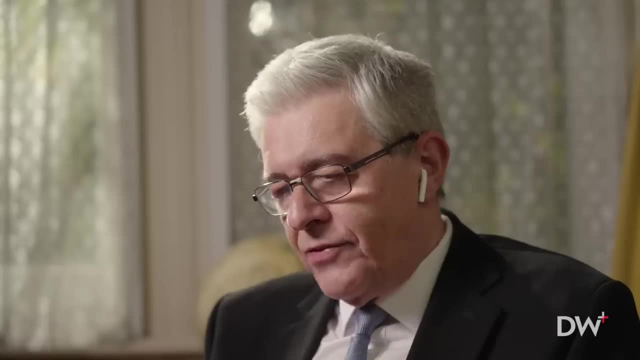 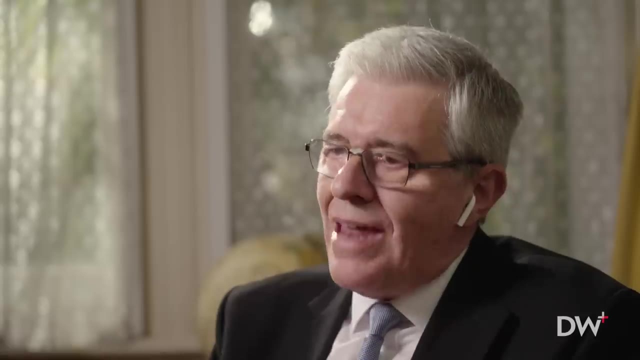 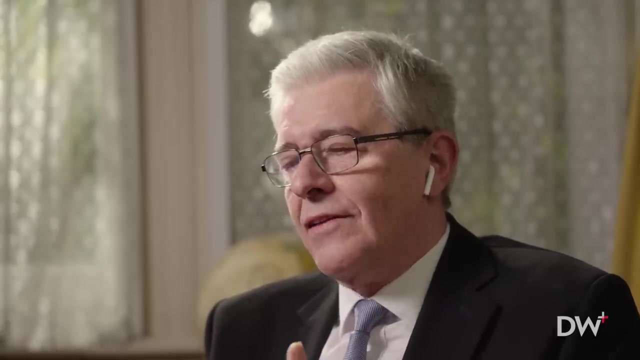 but you could also read it another way, in a much more deflationary way: that stuff societies through to cells that exist are just these free energy minimizing systems. so you know, these conversations are just the kinds of conversations that can only be there, simply because they are. 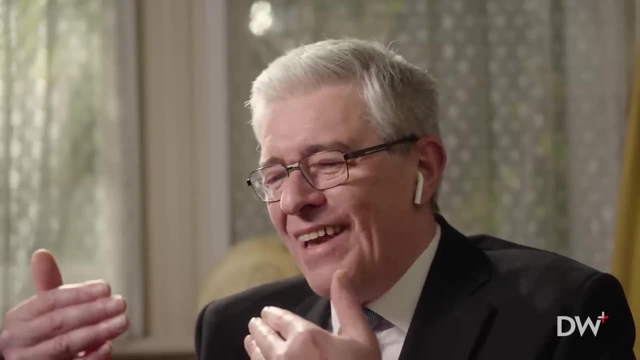 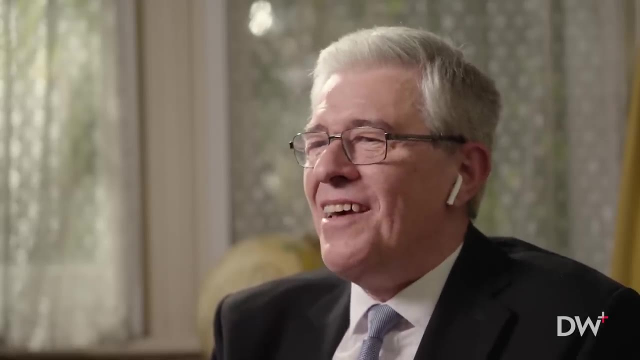 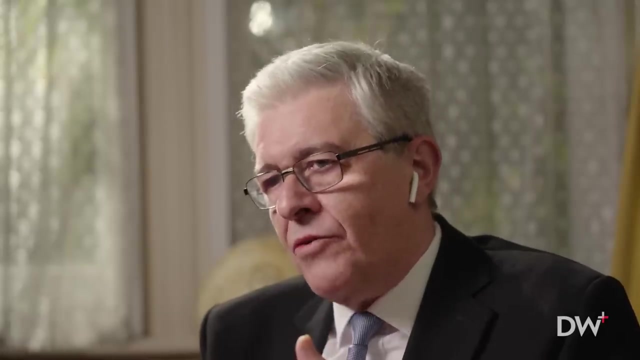 free energy, minimizing and, if you like, are what is left, when you wanted to say resisting the second law of thermodynamics. the very fact that we are here having this low free energy conversation and this exchange, rendering everything mutually predictable and resolving uncertainty about ourselves, means that this little dynamic. 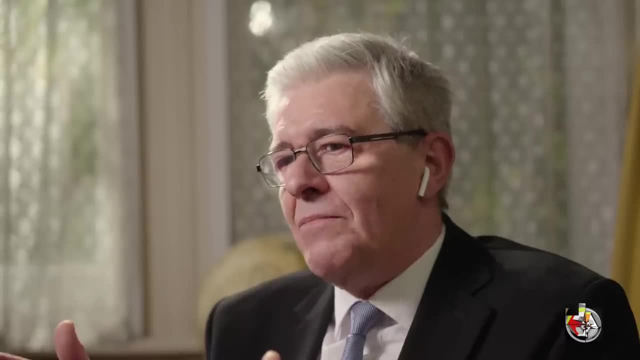 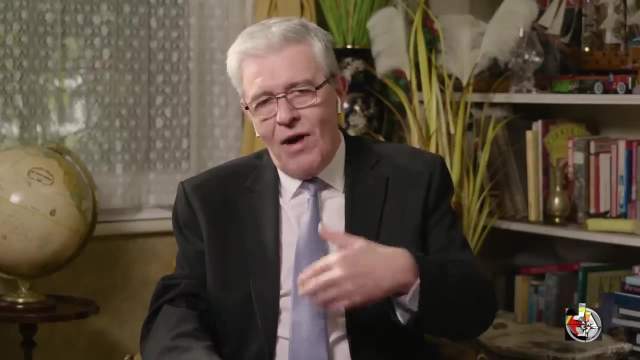 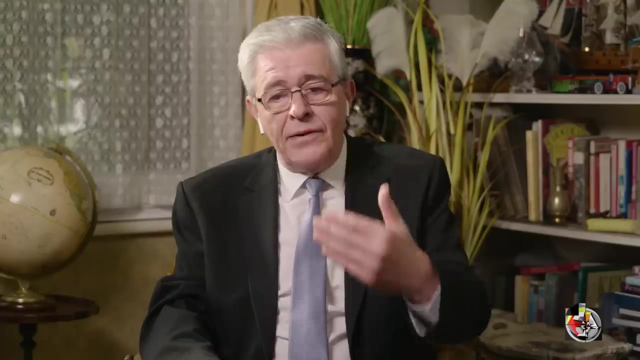 exchange is in itself a free energy minimizing. free energy minimizing system, and you know free energy. here again is this being used as a proxy for uncertainty, for unpredictability, disorder. so by minimizing free energy, by, we are implicitly going to be minimizing the disorder and the entropy and the expected surprise. 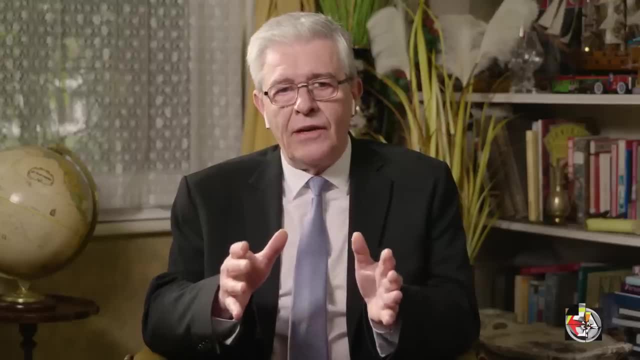 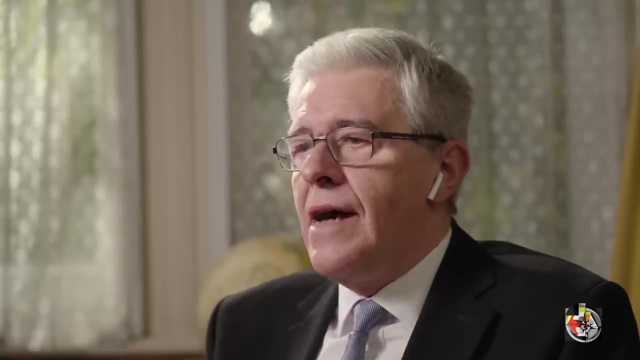 so it's all very consistent with the physics of self-organization. what you're doing, though, I think, is thinking about what would these things look like in a social context, in a dyadic context, and just to say also that one way of reading what you were saying about. 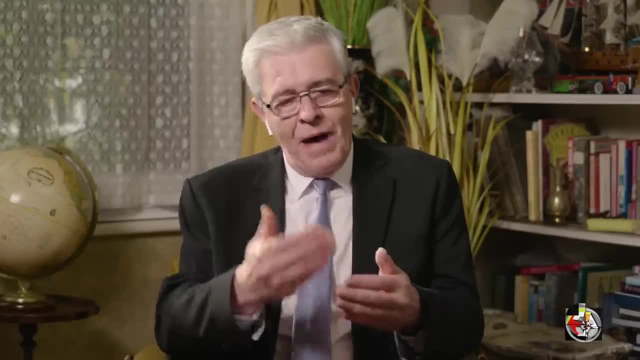 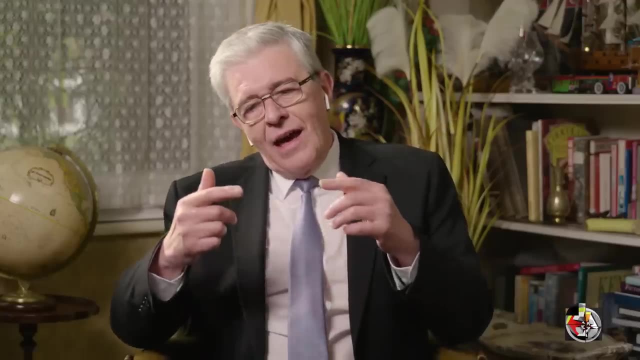 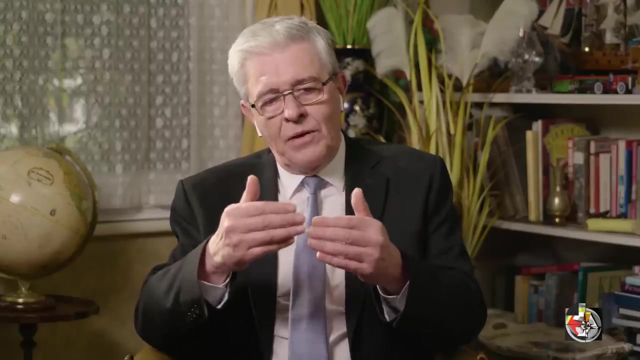 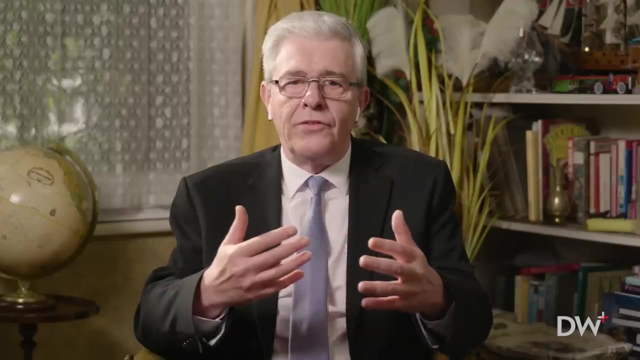 you know well, if we can both shorten the path to a state of orderly, predictiveness and uncertainty resolution, then if one thinks about that in terms of interactions either between people or between people and their environment, then you've got now a nice model for niche construction and cultural niche construction. 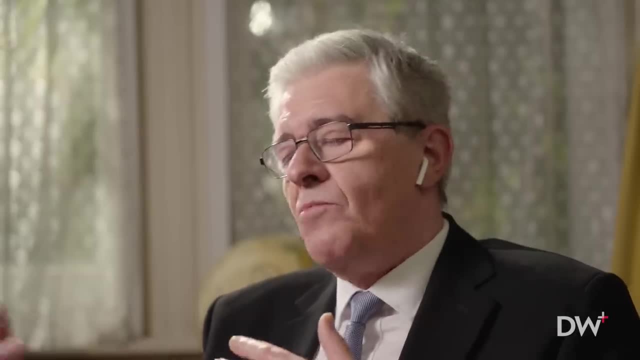 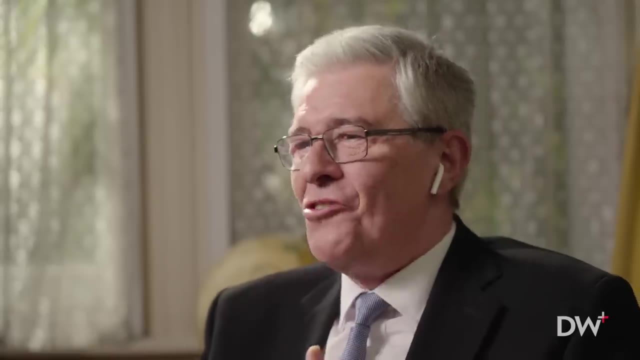 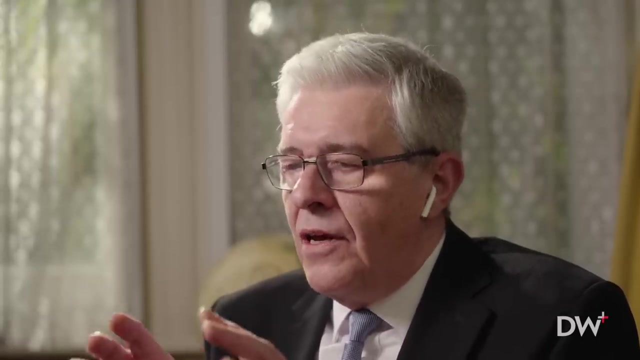 that you know, everything I do is in the service of making everything more predictable, and if that involves evolving to have a language and to teach my children language, then there's. you know, even that aspect of very, very high level niche construction or in culture, acting upon the world. 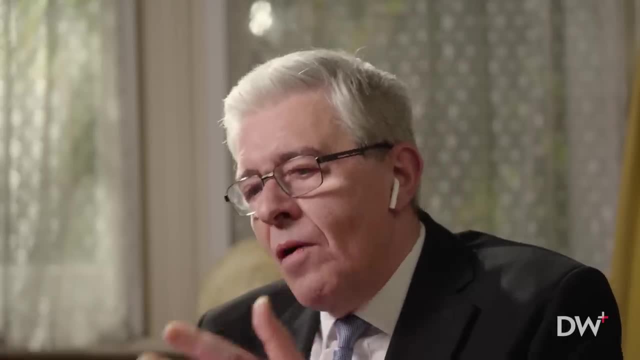 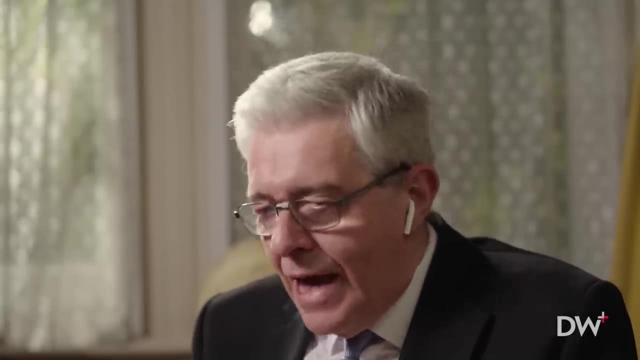 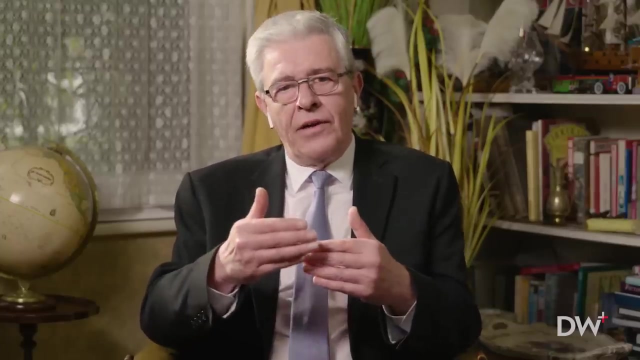 to make it, in an uncultured way, more learnable and more predictable is all in the service of minimizing this entropy, anxiety or free energy uncertainty. sorry, I slipped you an anxiety there. I shouldn't do that anxiety. I think it would be our remarkable capacity to recognize 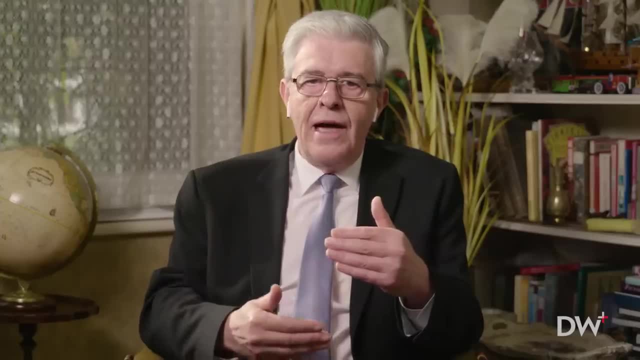 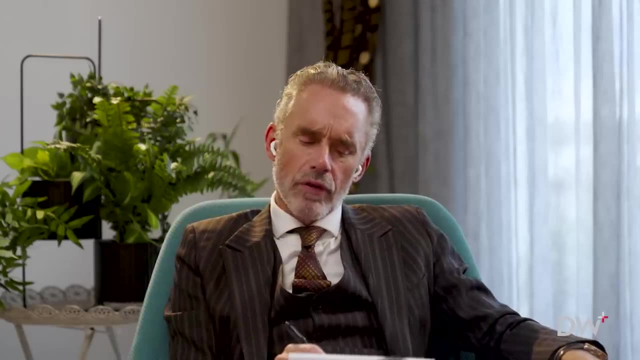 that we haven't resolved our uncertainty in the way that we normally expect to, and that would be the situation where the dopamine just goes away. So how do you view the role of GABA? and so that's one question. another question is: I've spent a fair bit of time 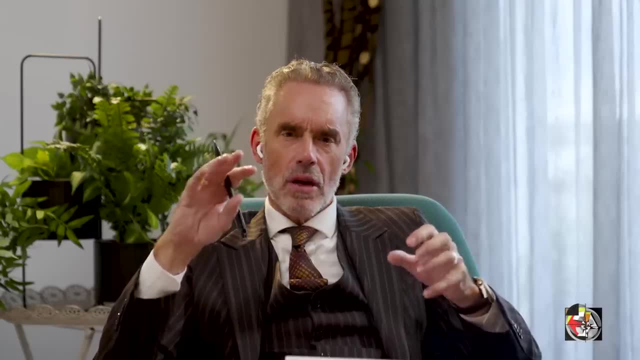 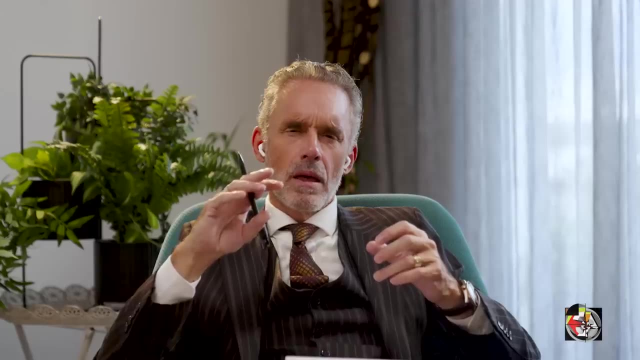 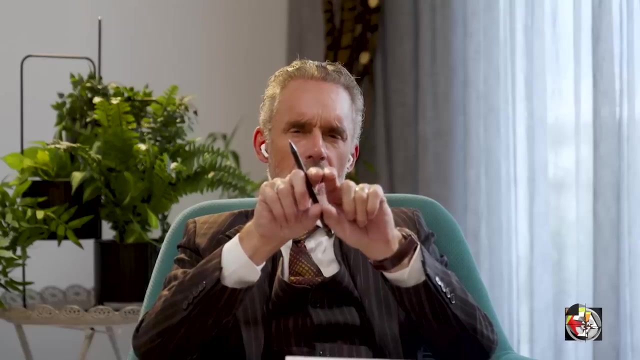 thinking about hemispheric specialization and I'm wondering if is it. is there any reason to make the assumption that does the left hemisphere specialize in some sense for precision or does it specialize for instantiating certainty at the lower levels of the hierarchy, whereas the right hemisphere 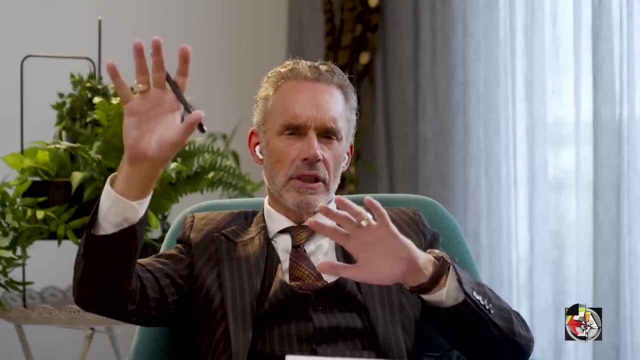 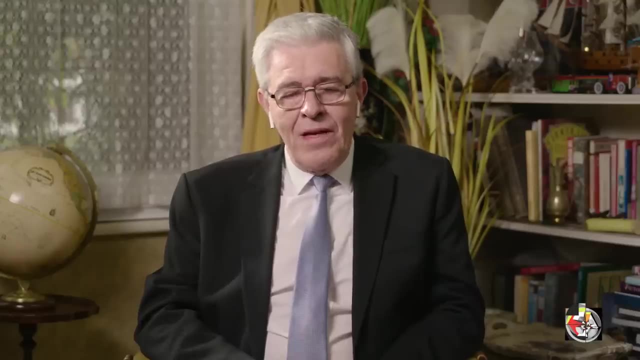 is involved in play at the hierarchy at the lower levels is that? is there anything to any of those concepts that you know of? it's a very interesting question, and now I'm sort of speaking as a sort of imaging neuroscientist about the function of anatomy. 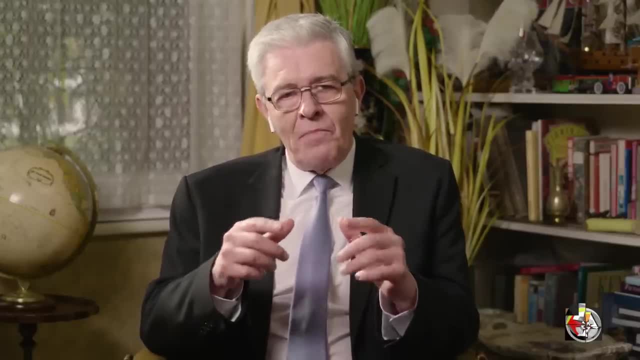 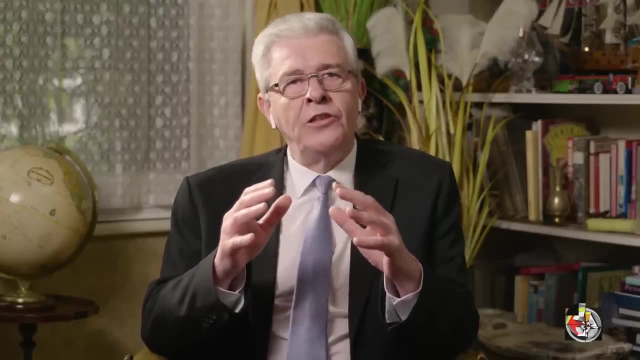 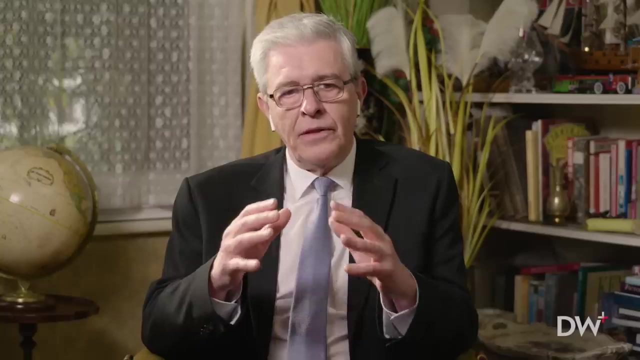 I mean, first of all, if we just go back to what we were talking about before, which is the cybernetic view and the good regulator theorem and the notion that we are, or we entail, good models of our lived world, or at least our sensed world, then having two hemispheres, 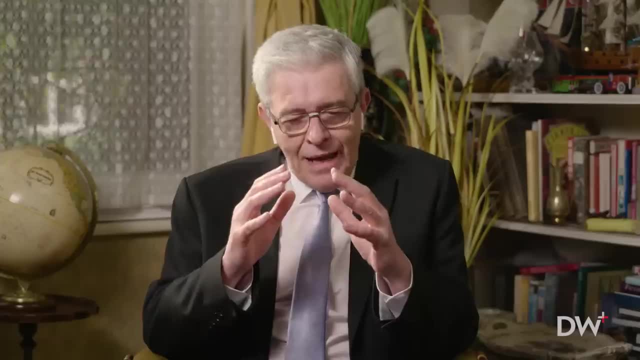 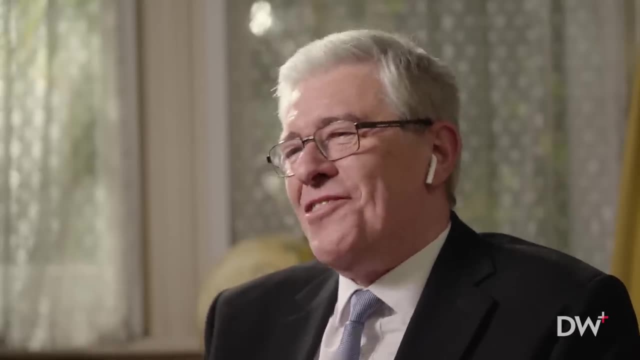 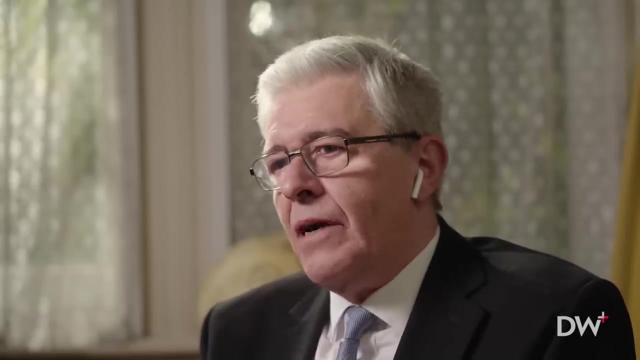 tells me immediately that there is some lateral symmetry in my lived world. and of course that tells me, of course that is true in the sense I have two arms and two legs. you know, if my world, certainly as a newborn, is basically, you know, 99% my body. 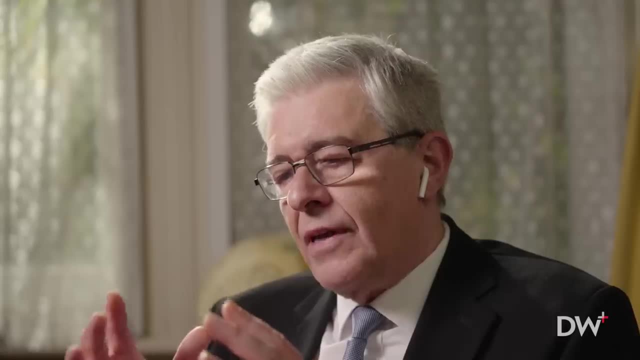 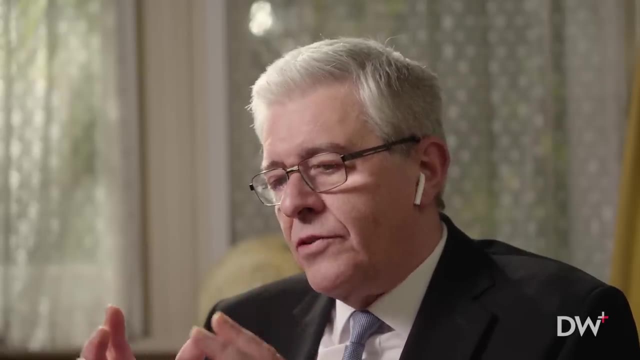 I think the sort of having two hemispheres tells you something quite fundamental about the universe into which you are, as a brain at least- introduced. just to generalize that what that means is: if you gave me the brain of a Martian, I should be able to tell you. 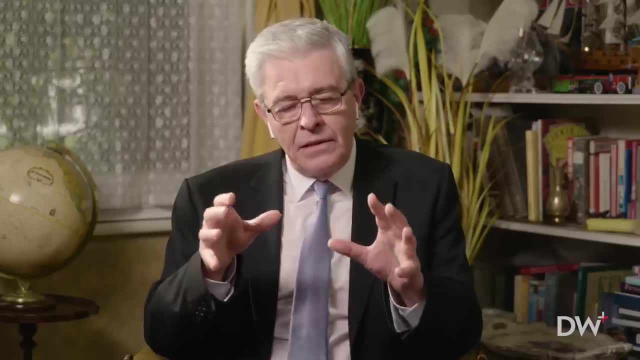 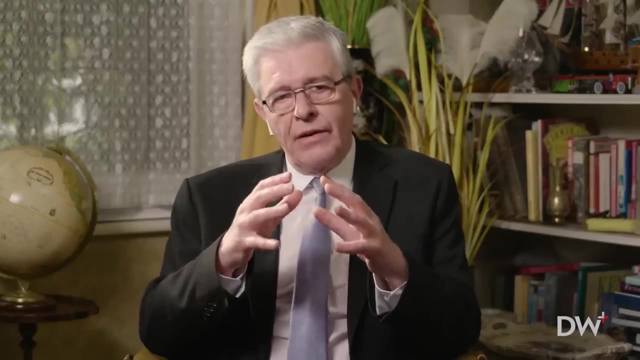 a lot about its lived world and its embodiment and its body and the kind of world that it lives in, just by looking at the structure, the anatomy of the brain. so I think that you know there's an important aspect to that sort of lateralization issue, a more 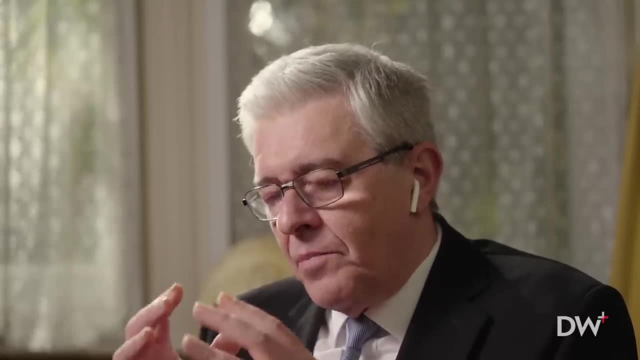 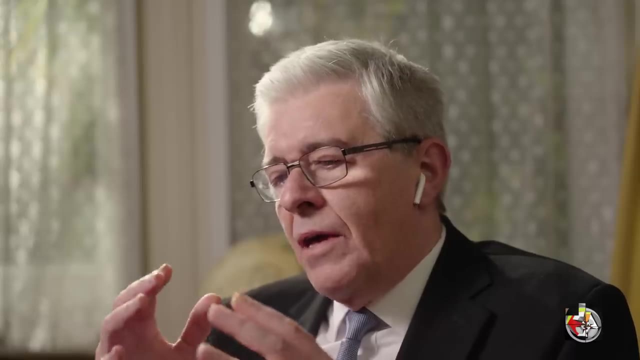 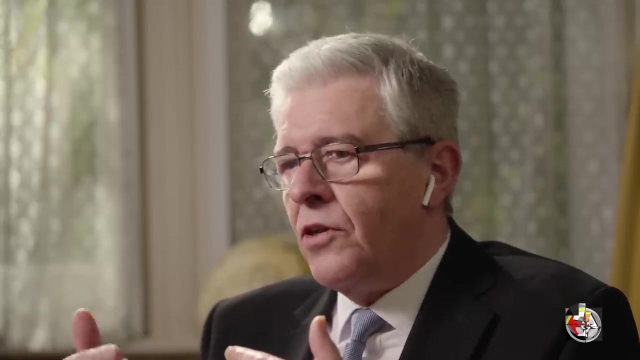 I think a sort of more scholarly and more specific answer to your question is that there is certainly in neuropsychology an asymmetry in the way we deploy attention. so if you now read the deployment of certain neuromodulators such as say serotonin or acetylcholine, 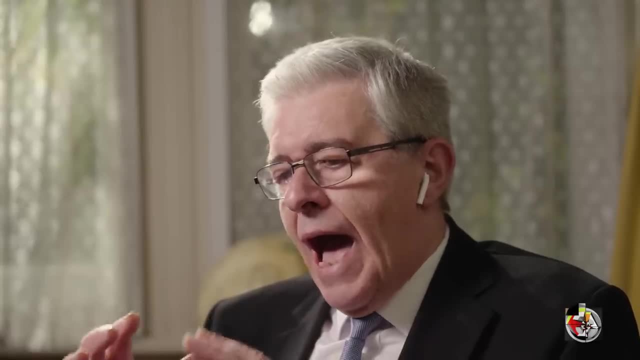 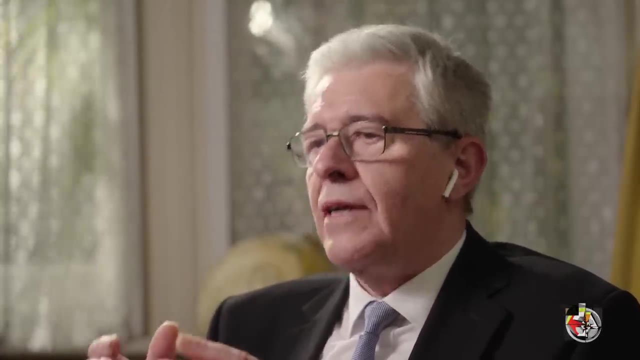 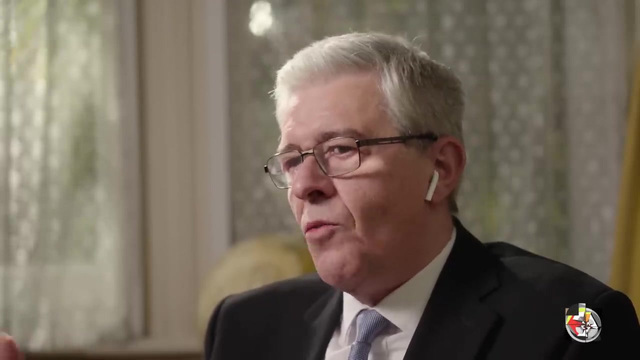 or indeed adrenaline, as instantiating endogenous attention, then its deficits will correspond to certain kinds of effects like neglect, you know, a pathological inability to attend to ie. you're always going to ignore or just not be aware of this. and of course, there's some really interesting work. 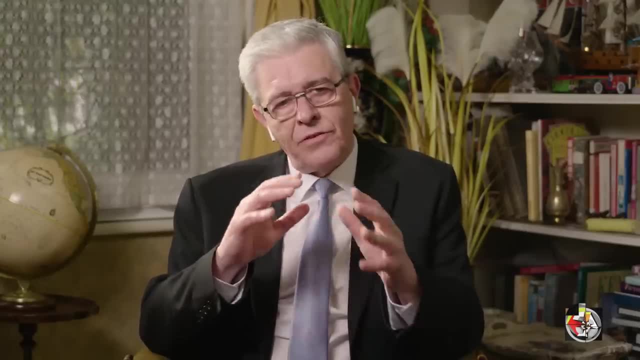 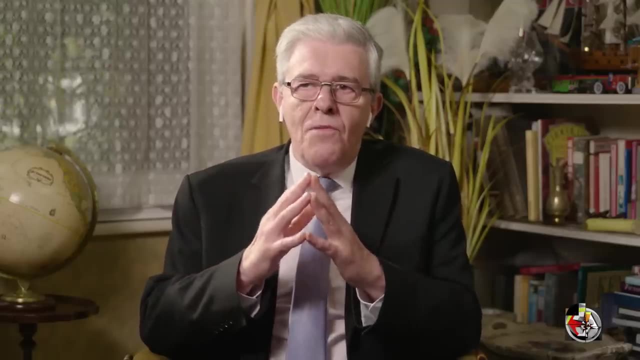 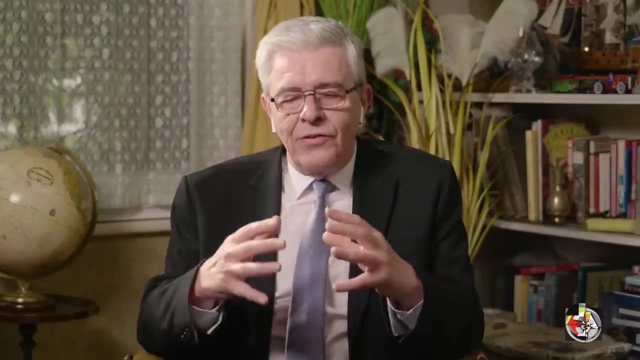 in terms of hemineglect systems and bilateral asymmetries between the right and the left parietal cortex in these syndromes. so I don't know very much beyond that, other than to be able to say that, for for reasons that must have, 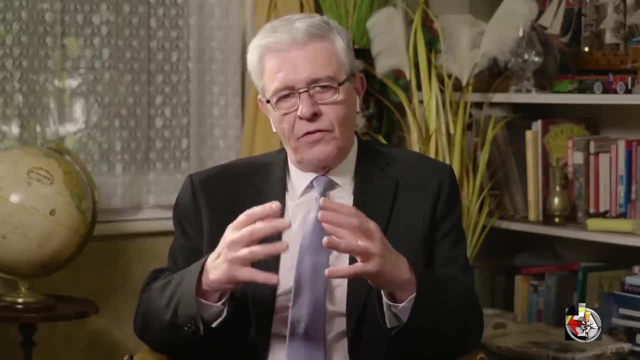 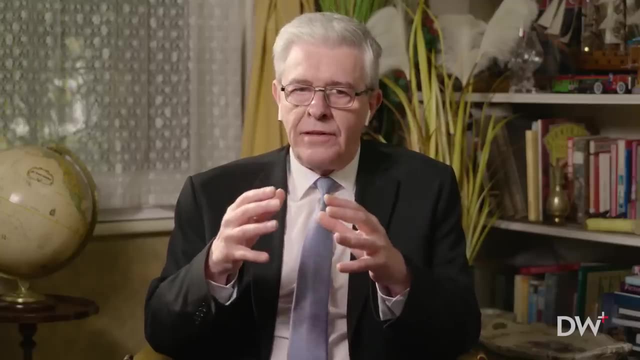 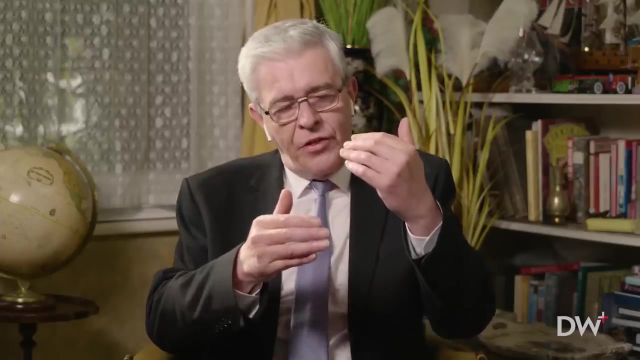 a principal explanation in terms of you know the high order causal structure of the worlds in which we operate. there certainly is some asymmetry in the way that we attend to things, or there's some benefit in terms of having that factorization that allows certain things to attend to. 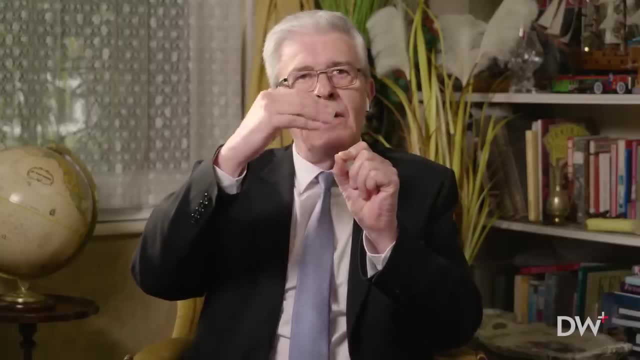 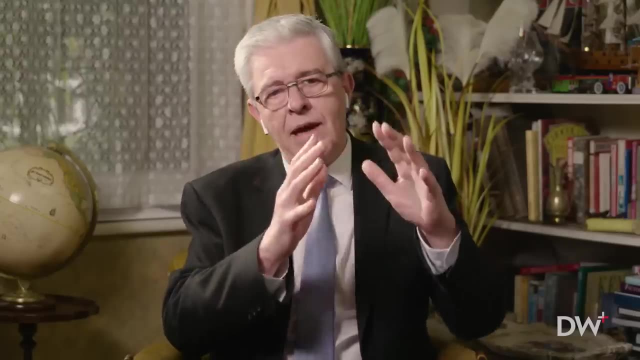 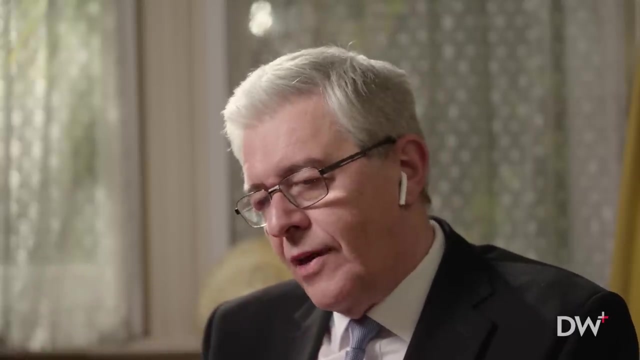 that this, you know, just set the sensitivity or the flexibility or inflexibility of a hierarchical construction. it must be the case that there's certain attributes and certain attributes that do show this, this lateralization, and just to point out also, of course, that the lateralization 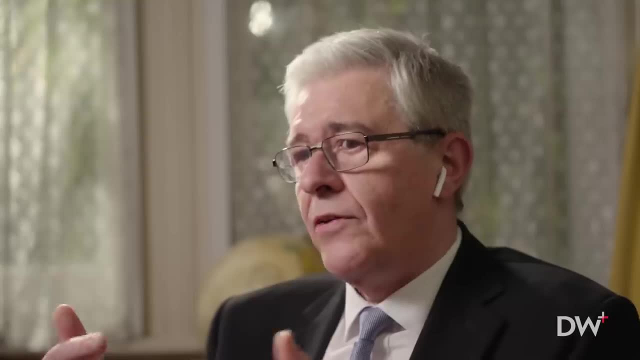 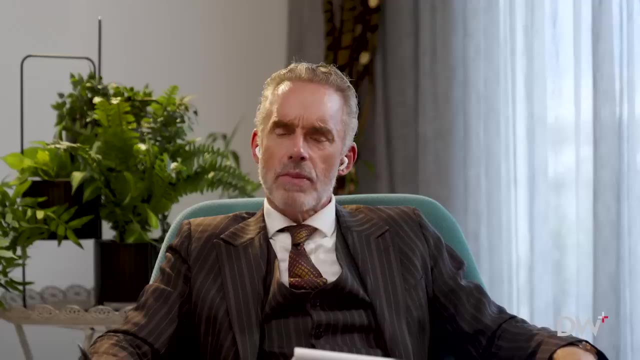 issue was quite hot in the days of Grey at the Moresley as an, as a possible correlative, things like schizophrenia, yeah well, I mean. Goldberg, who was a student of Lurius, suggested that the right hemisphere was specialized for processing certainty, and so it might be. 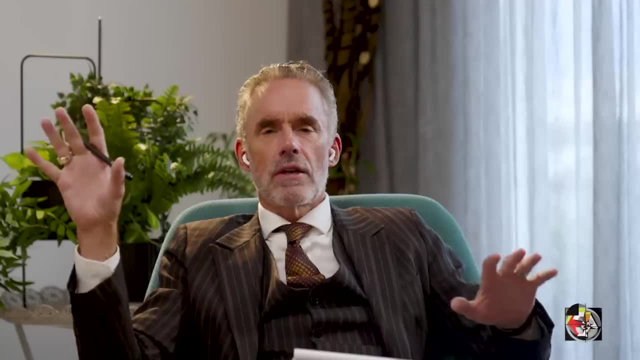 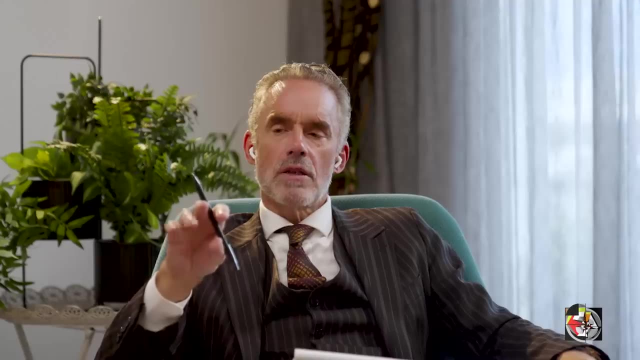 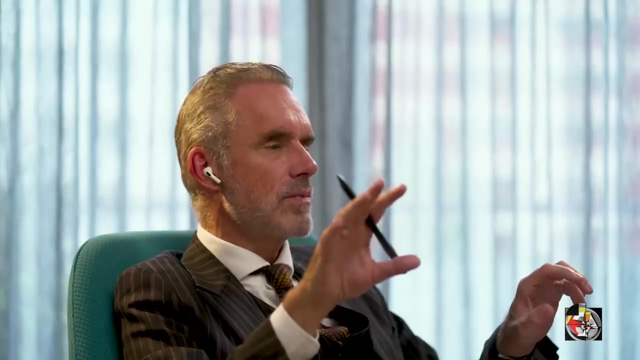 something like: the more novel it is, the more likely the right is to attend to it, and that sort of maps onto Gilchrist McGilchrist conceptualization of hemispheric specialization, with regards to both predation and predator detection. so the right hemisphere seems to be. 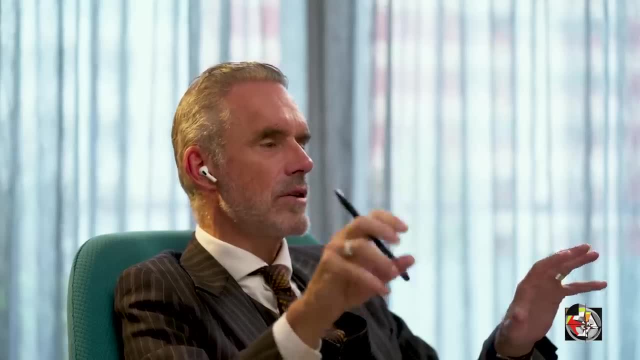 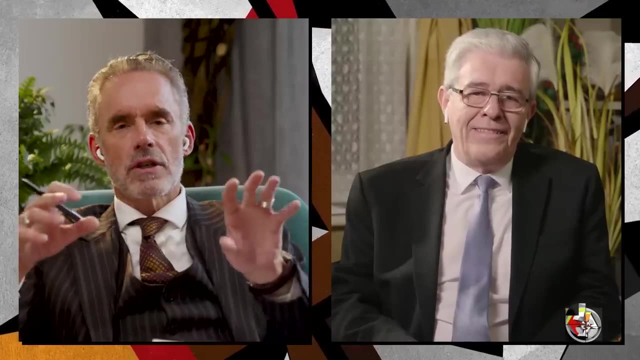 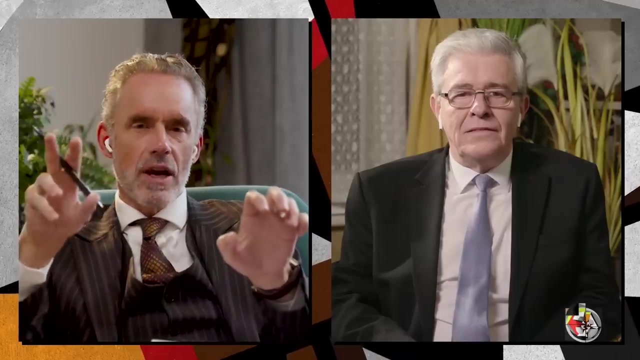 specialized for contextual evaluation and the spotting of predators, and the left for focused attention in the service of predation. so a bird, for example, will attend preferentially with the prey detection system well eating. but the right hemisphere and the other eye are scanning the environment for signs of 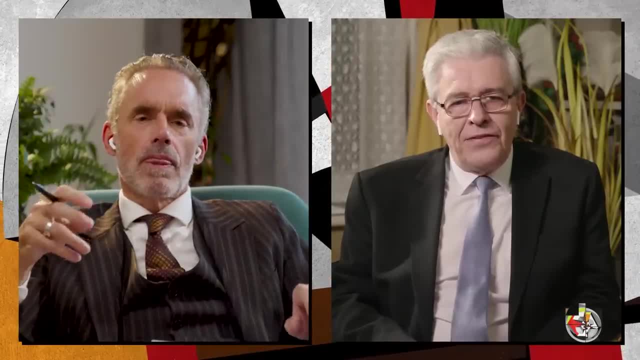 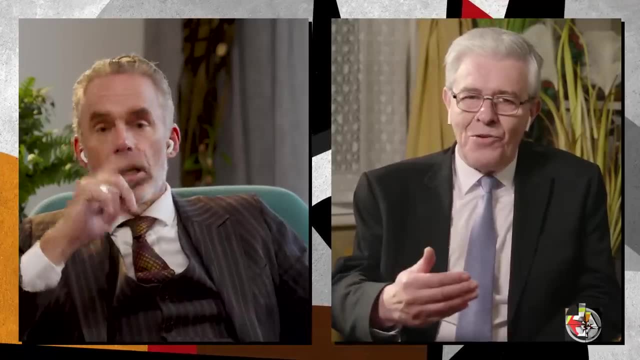 context: dependent signs of predation on the bird. okay, I didn't know, I didn't know that that's very interesting, so I was just thinking. of course, the obvious example of lateralization is language and if you look at language as really predation, so if you think of 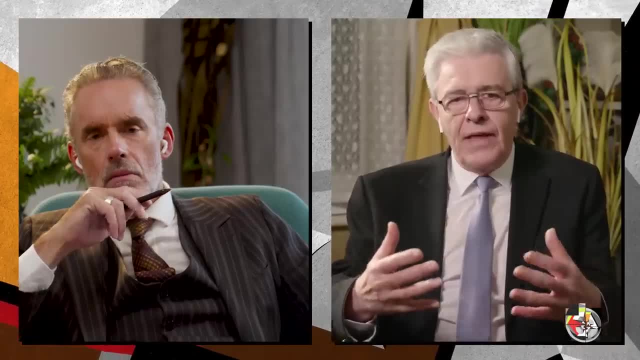 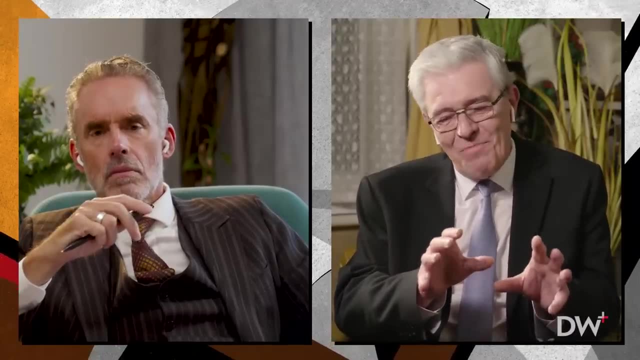 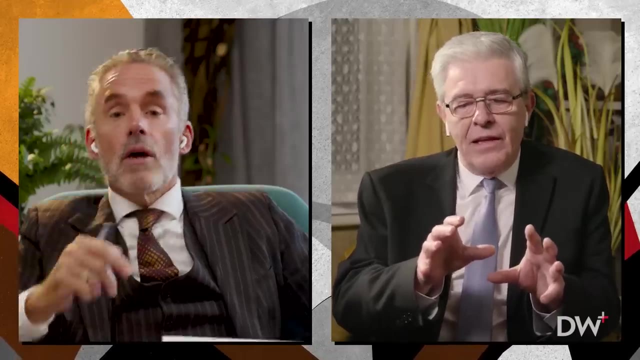 language as the way of asking questions. that is the tool that we use to predate, for information, so that makes entire sense. I didn't know that about the comparative ethology anatomy of predators, but yeah, well, if McGilchrist's new work, McGilchrist's 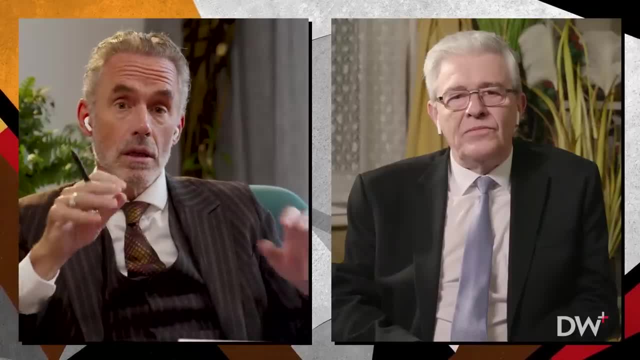 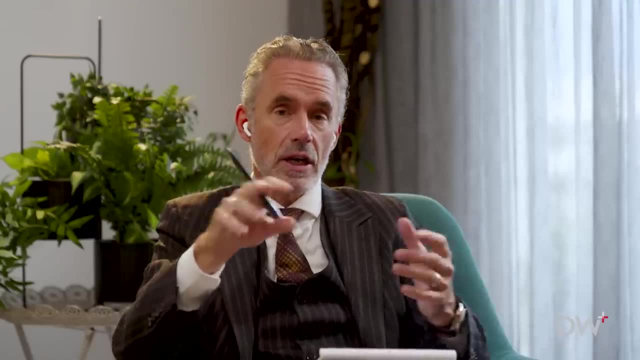 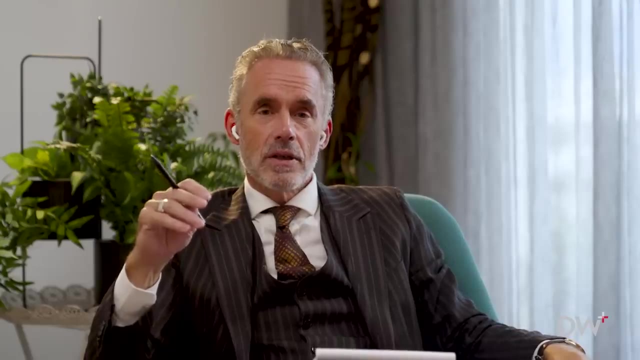 new work details that out in some at some length, the relationship between attentional and specialization. it's quite nice and it maps very nicely onto the concepts that we've been discussing today. so shall we take a brief foray into psychedelics, and then we'll have to close. 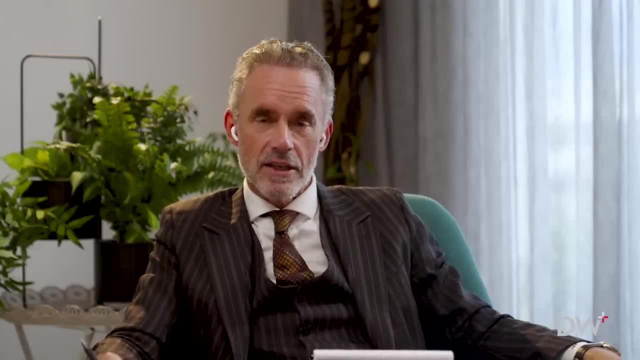 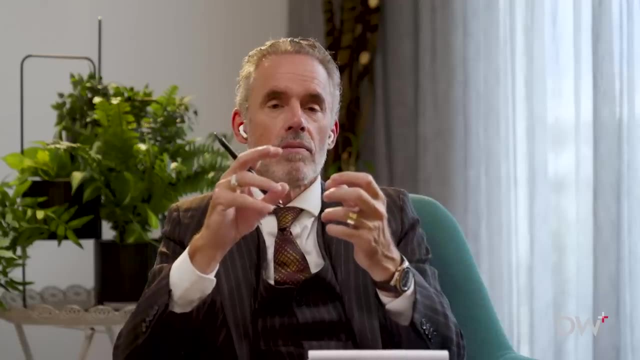 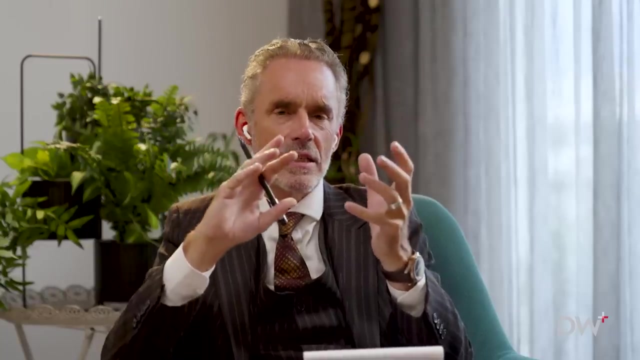 this part of the conversation, unfortunately, although there's about 50 other things I'd like to discuss with you. but well that's. I guess we've covered a fair bit of territory for one day, but I'd be. I'm very interested in your conception and its antithesis. 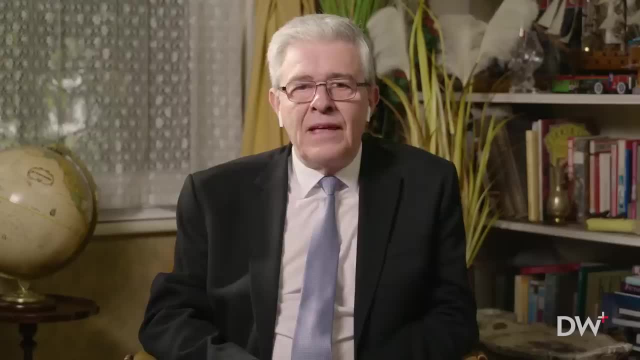 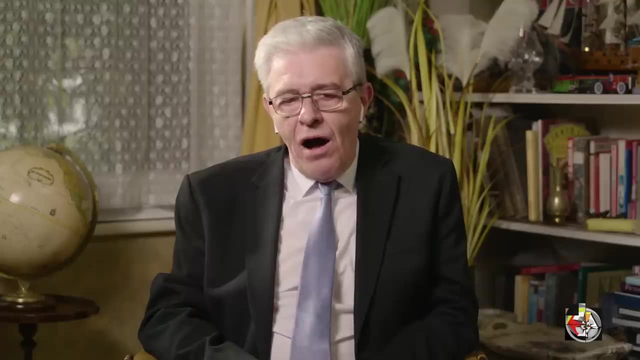 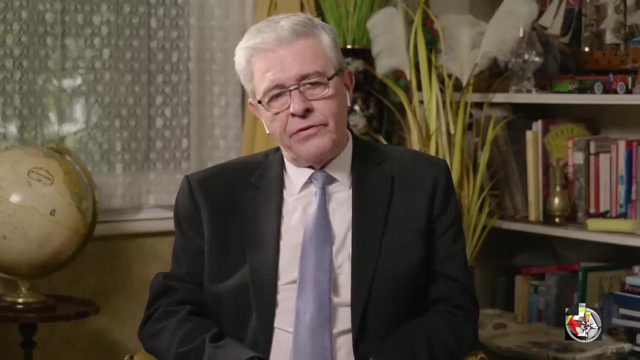 in some sense, if I've got this right, with the action of antidepressants, yes, well, yeah, I'm not sure it's an antithesis because you know there are in the past few years, and indeed months, an increasing number of papers looking at sort of 5H2A. 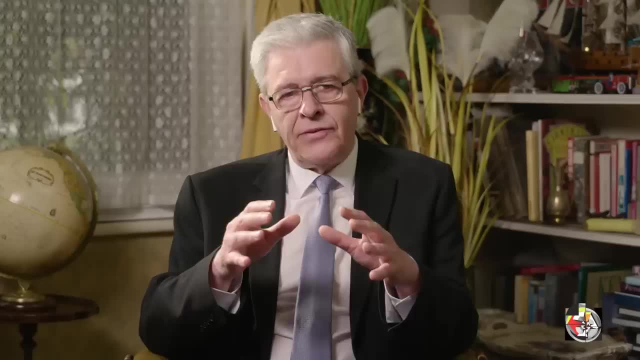 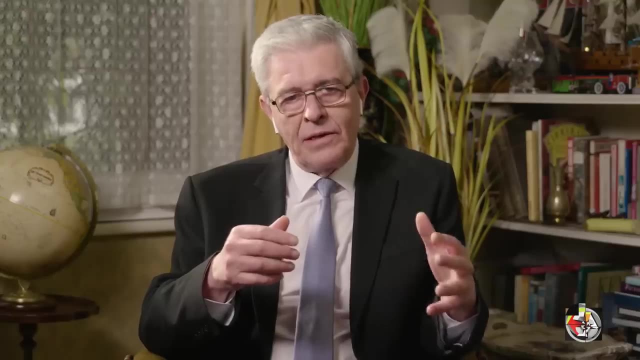 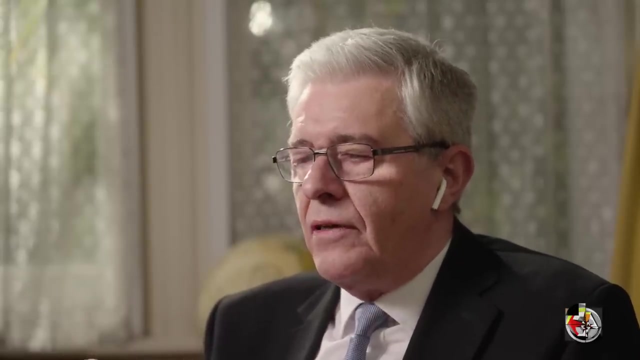 agonists and partial agonists, and drugs that act upon psychedelics and their ability to remediate certain conditions that would have, you know, a pronounced- usually pronounced- affective state. so the game is very complicated, but what we certainly know at the moment is that the 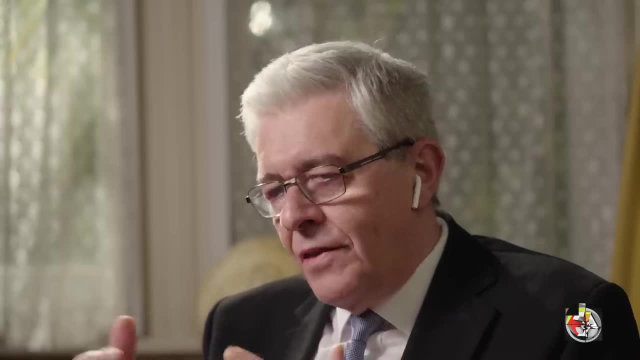 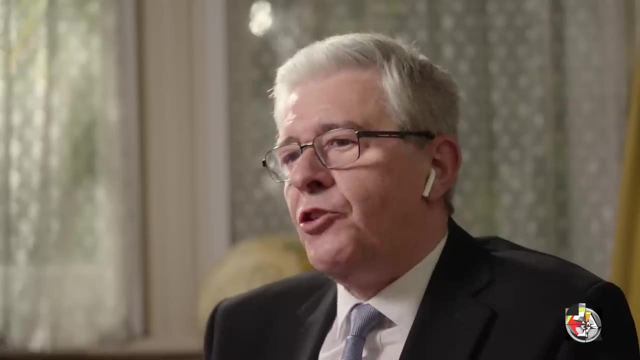 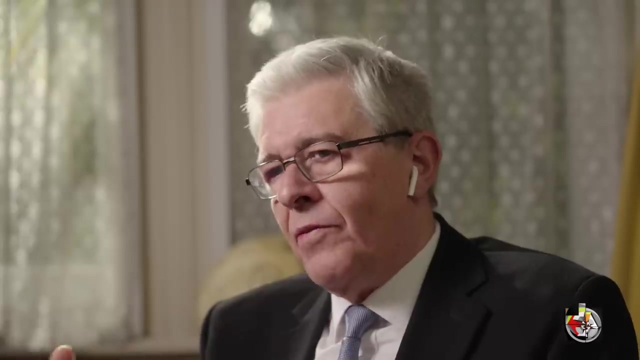 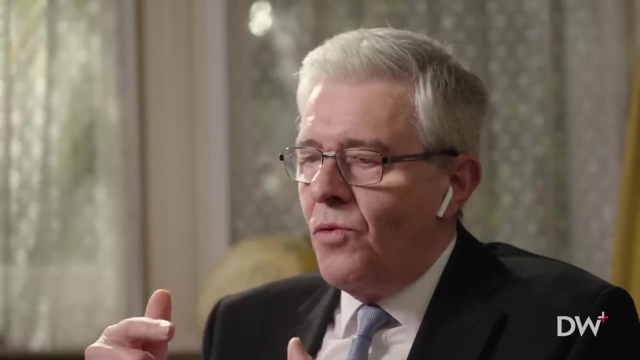 actions of psychedelics from the point of view of their definitive effects on the brain, namely, you know, the abnormal perception and the characteristic way that you, you can't attend from the microstructure of your sensations. we, we do now know that that is probably best explained. 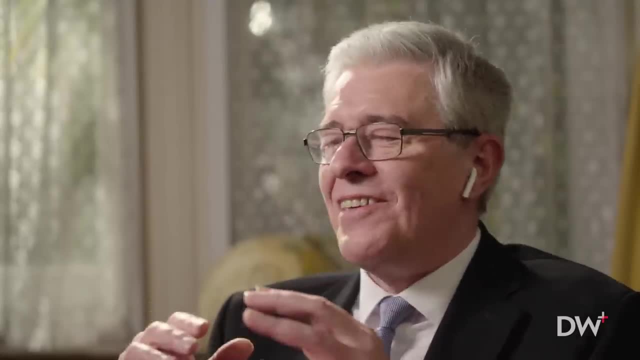 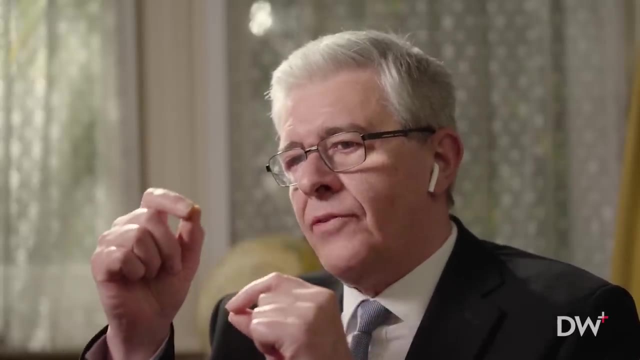 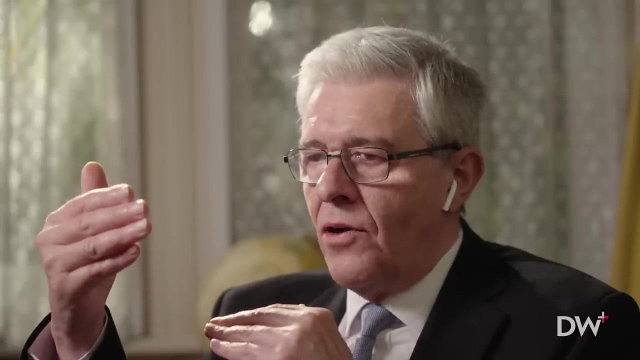 when I say we know, we conjecture that it is nicely explained by exactly the same kind of mechanism that you were talking about before, which is a sort of changing the balance of recalcitrant or precision or sensitivity away from these high level constructs deep in the hierarchy. 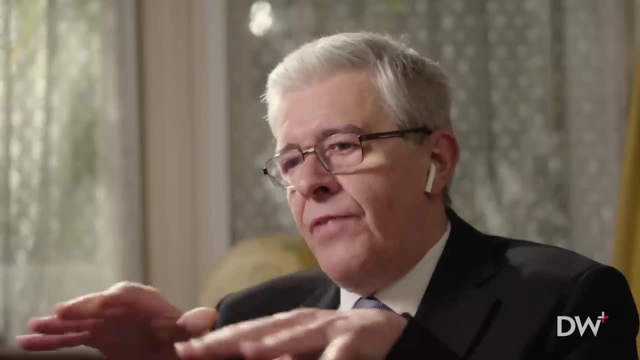 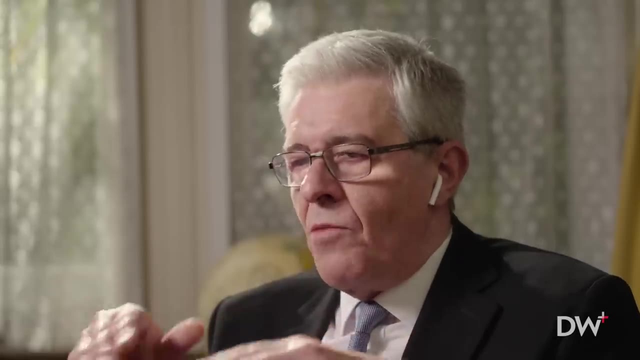 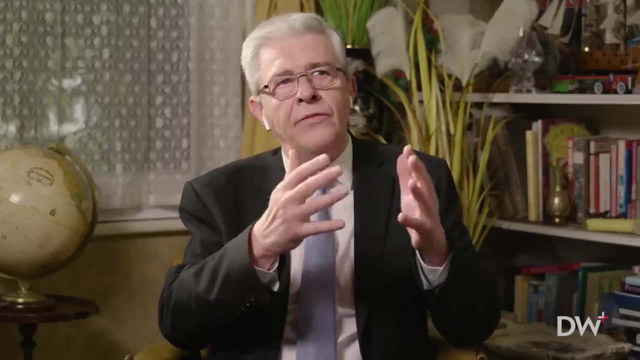 at the top of the hierarchy and reinvesting that kind of precision or sensitivity under predictive coding models to prediction errors much lower in the hierarchy. so this would look basically like I'm now going to ignore my prior beliefs about the narrative that I'm currently committed to. 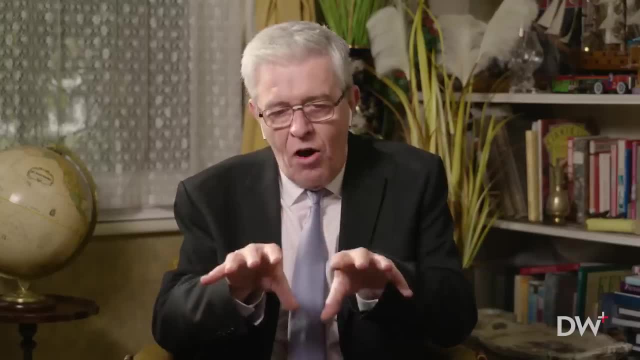 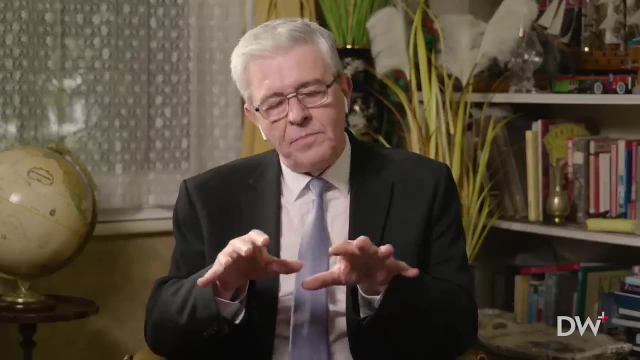 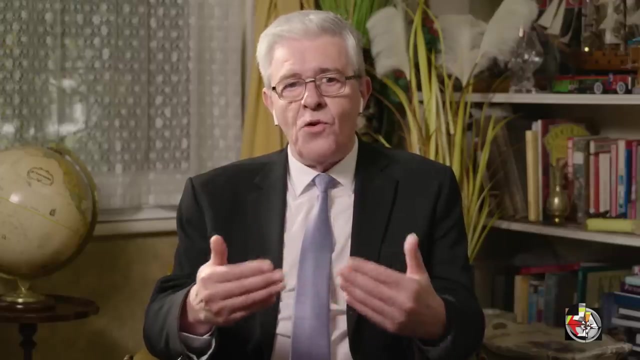 in terms of this interaction and I'm just going to focus in on you know what can I sense? so you're talking before about sort of a mother's predisposition to be very sensitive to cues that could engage or could represent really important affordances for responding. 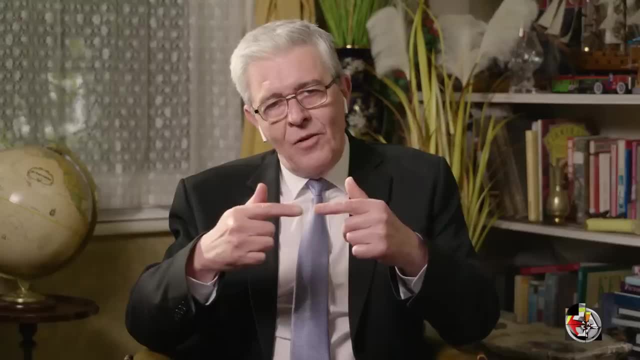 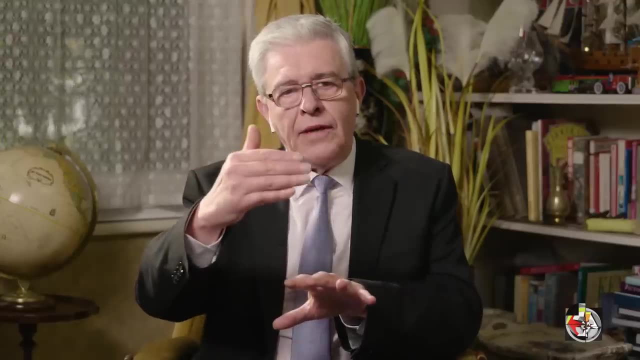 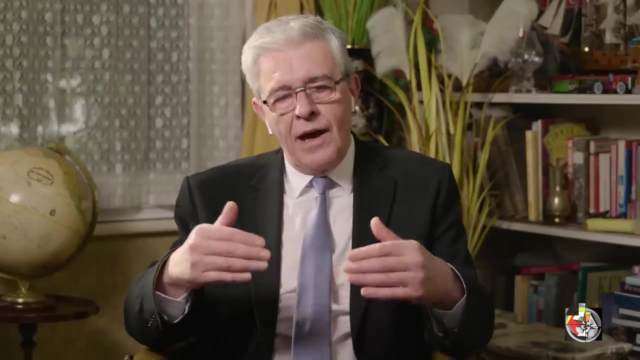 like responding to a baby crying. so this would be, you know, one way of viewing the effects of psychedelics that you are forced to, by reducing or relaxing the decision of the high level beliefs in relation to the lower level evidence or belief updating or evidence accumulation. 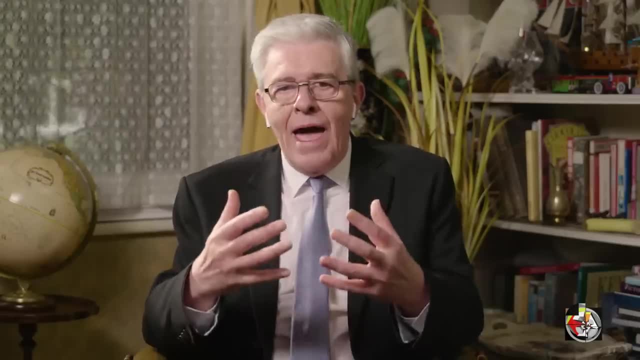 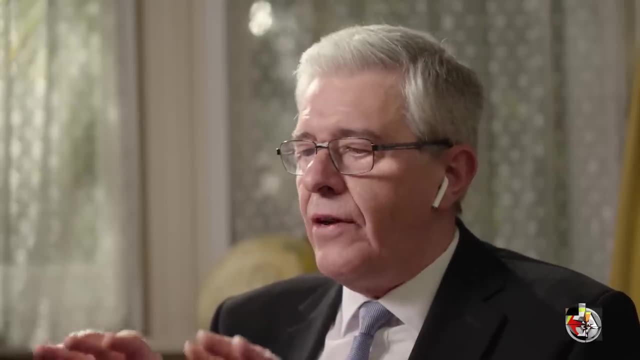 you are putting yourself in an intentional set where everything is interesting. you can't attend away from it at a very elemental level. and it just struck me that this is, you know, very, very similar to what you were talking about before in terms of the, you know, neuroticism. 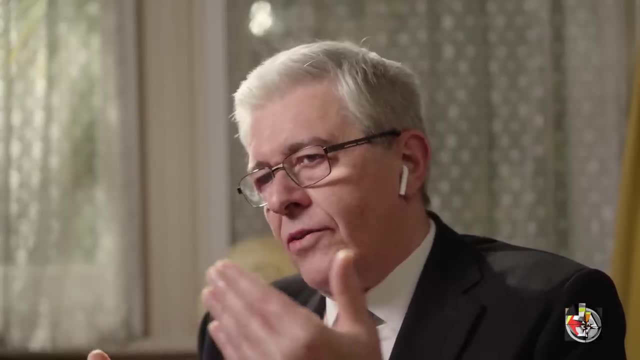 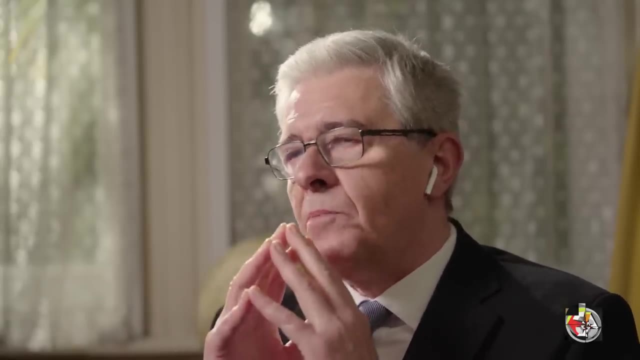 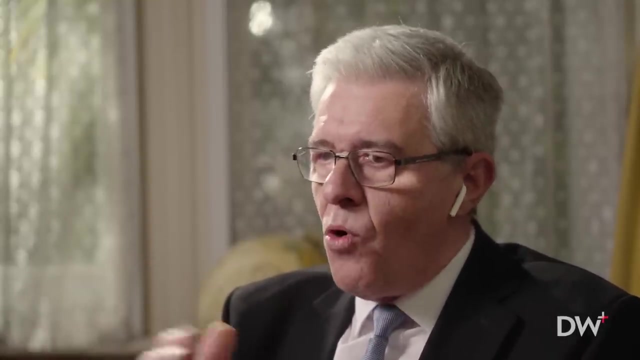 I presume this is sort of an einsynch like where you know you would have some people who are just jolly confident that their prior beliefs are the most apt explanation and they will ignore lots of evidence to the contrary simply by suppressing the precision or the importance. 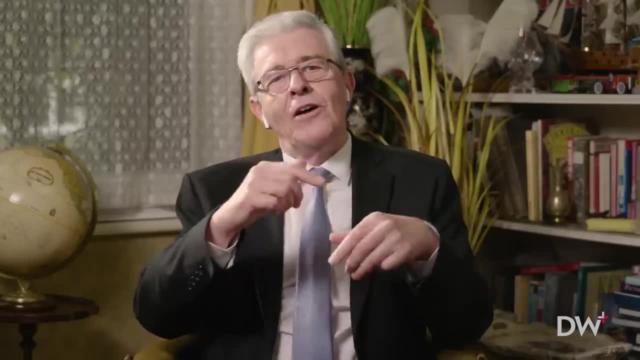 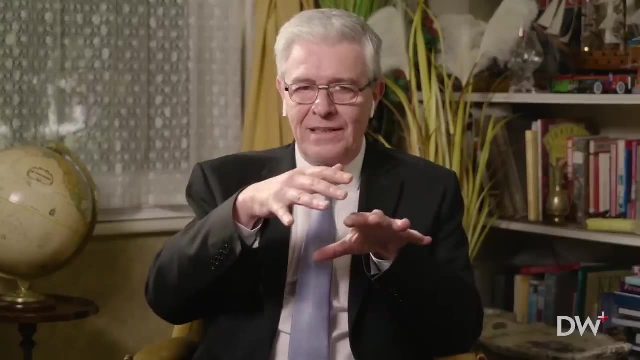 or turning down the gain on that kind of thing. but you can't do that if you get more than three errors that you can't explain. so you know there is an adaptability built into our brains that will actually say: well, no, actually, let's just attend. 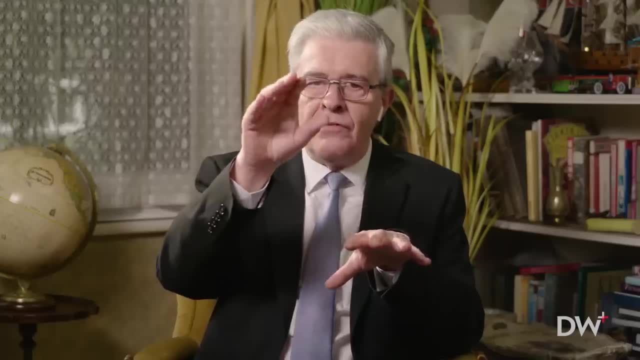 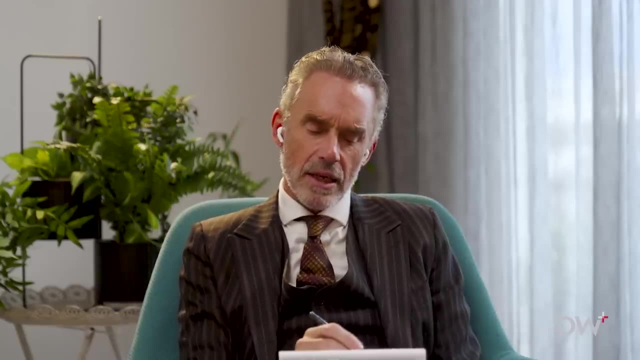 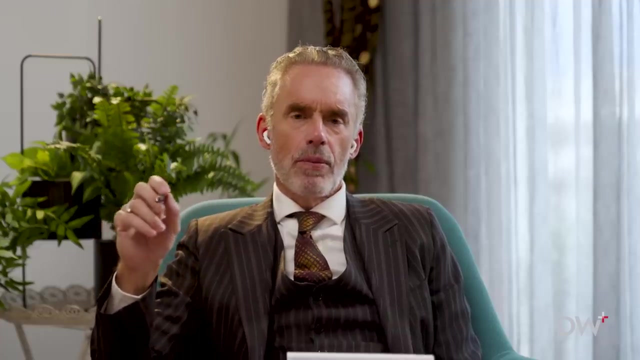 to these lower level beliefs and at that point you're going to have to relax the higher level and become more flexible and more adaptive. well, that okay. so that ability to relax at that level seems to be indexed by the personality trait openness, and open people are more creative. 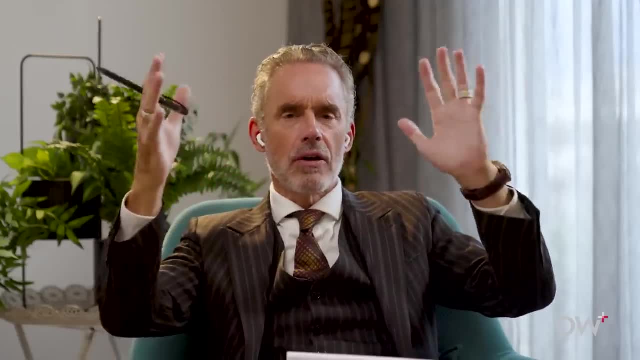 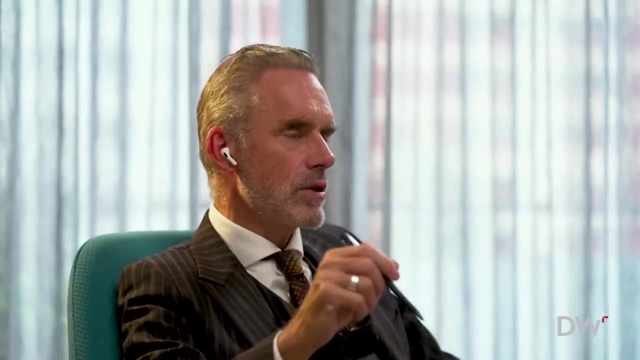 and so creative people have more play in the higher order conceptualizations. and one of the solid empirical findings emerging out of the research on psilocybin is that a single mystical experience induced by psilocybin produces something approximating a one standard deviation increase in trait openness. 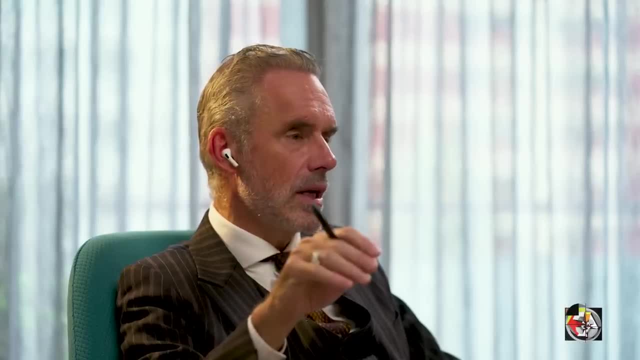 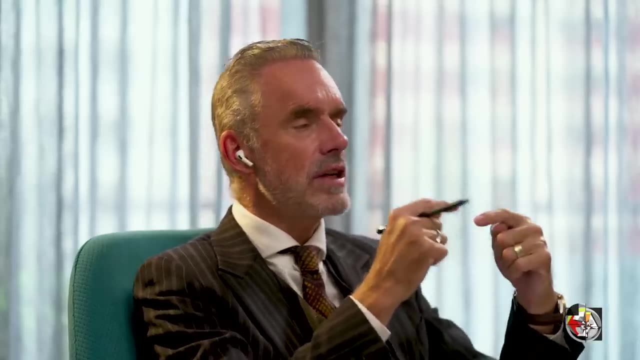 that's permanent, it never goes away. yeah, yeah, and so it doesn't look exactly like it's a reduction in, or say, an increase in, neuroticism, so that error messages can propagate upward. it's, it's something akin to that, because if you're more open, 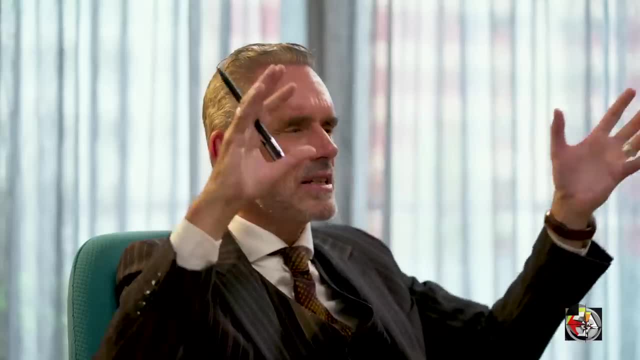 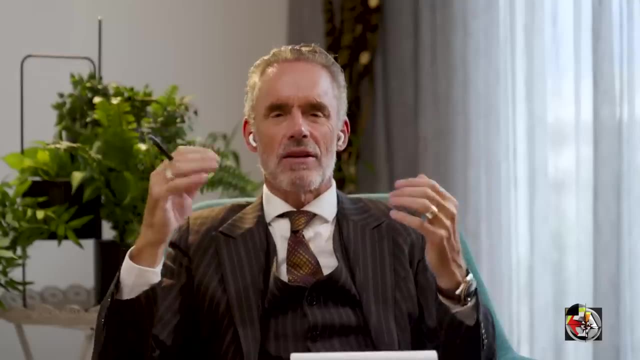 then there's more play. there's more play in the system, but it doesn't seem to be tied exactly to error per se and negative emotion, and I can't puzzle out the distinction. exactly right, because if you're high in neuroticism, you're going to propagate. 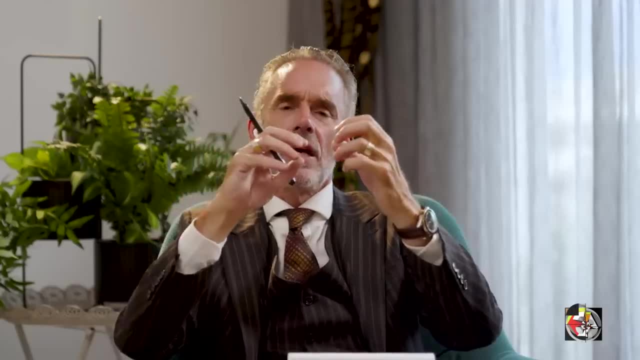 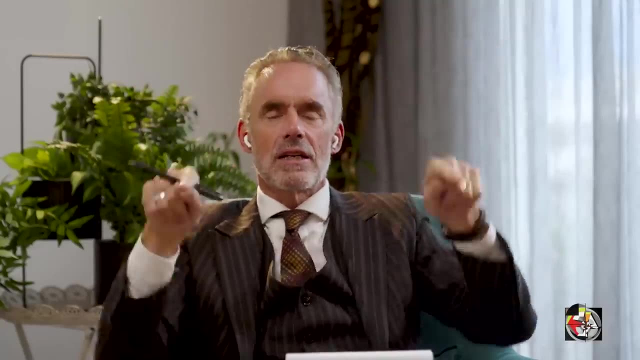 error messages, but then things are going to collapse. if you're high in openness, the error messages propagate, but you generate alternative theorems at a very rapid rate in order to re contextualize the anomaly. I didn't know that that is very interesting, so I think then 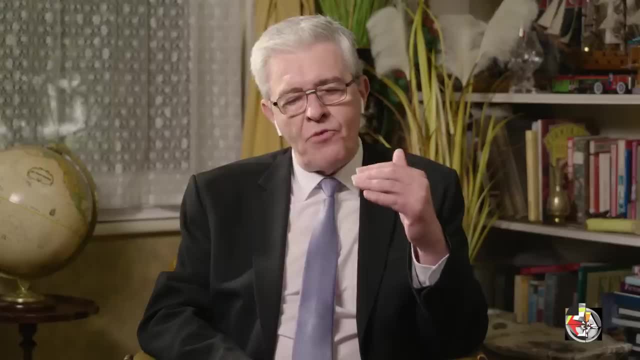 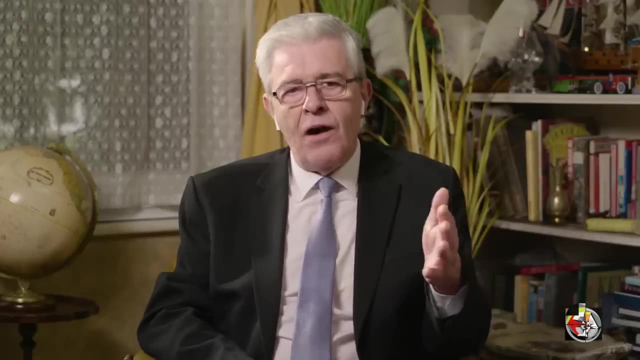 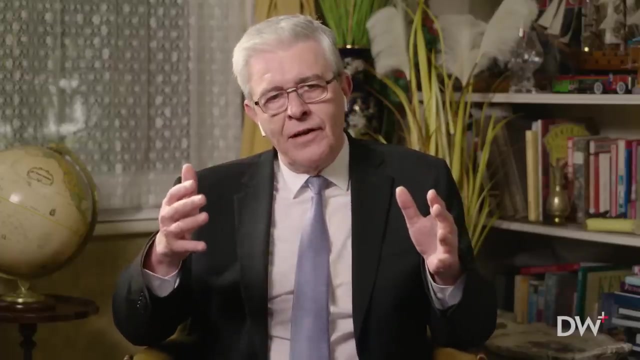 it's the openness that we're talking to, and certainly that's the aspiration or the motivation behind the use of these chemicals in, say, end of life care or indeed in terms of psilocybin assisted psychotherapy. it's really to open you up to new possibilities. 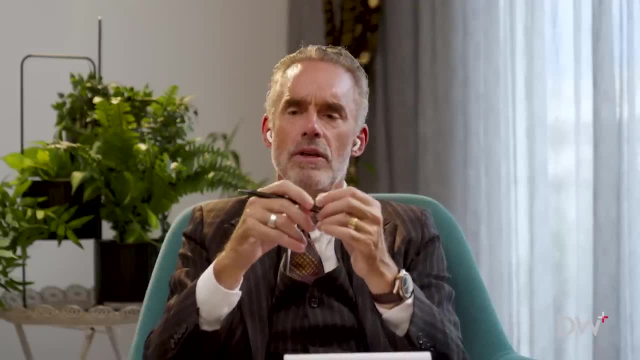 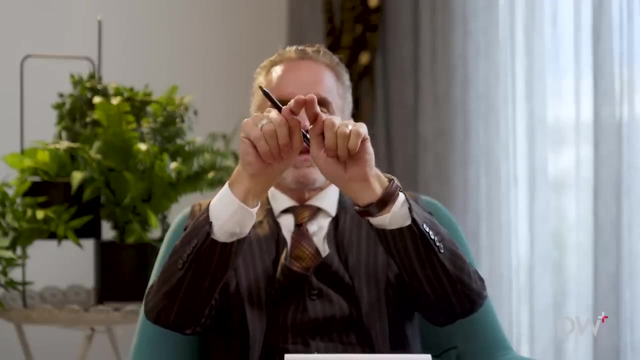 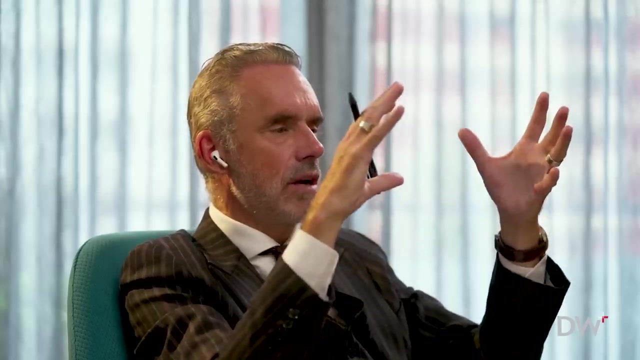 well, maybe with with creative people, what you see. so imagine category rigidity, and category rigidity might be something like the probability that activation of one category will activate adjacent categories. so imagine that constraint is the constraint of openness: the more open you are, the more flexible those boundaries. 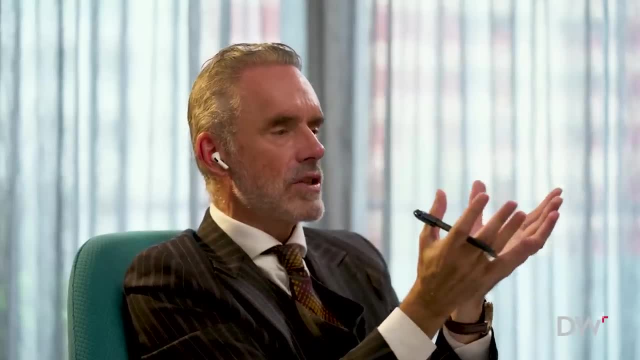 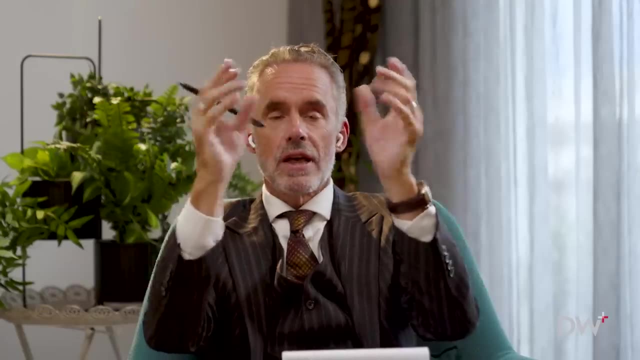 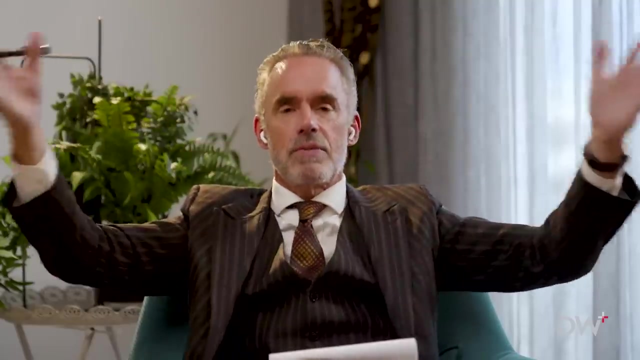 the more when you activate one category, you're going to co-activate a network of associated categories. so then, imagine, you dump psilocybin into the system, and what happens is the barriers between adjacent categories become more permeable. and so then, as information propagates up, 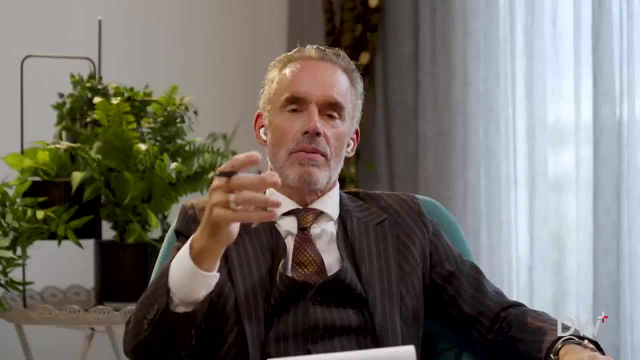 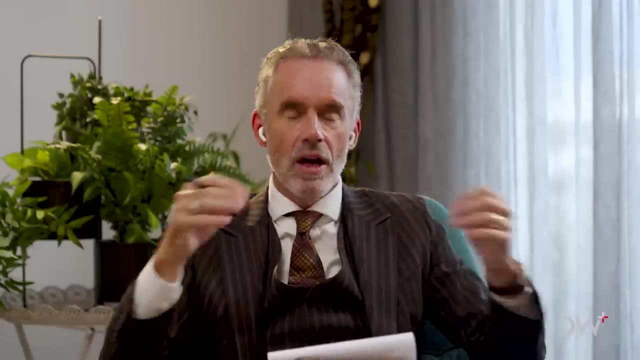 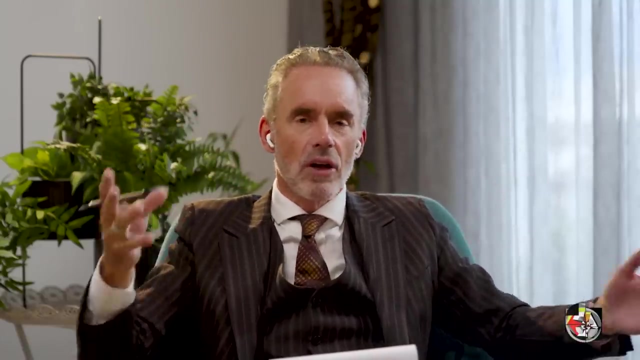 there's more play in the systems, and that would increase your probability of a false certainty right which is on an idea derived from insight. that's wrong, but it would also increase the probability that you'd get some true positives out of the deal, which is really what creative people 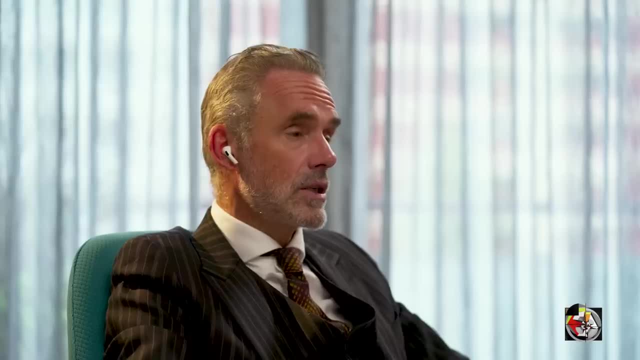 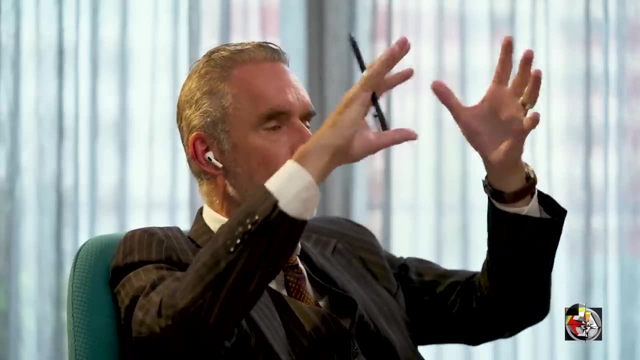 are doing all the time a lot of creative ideas just aren't functional, but some are crucial and so it's a high risk, high return cognitive strategy in some sense to generate, to have looser categories at the higher levels, and certainly that is akin to what people 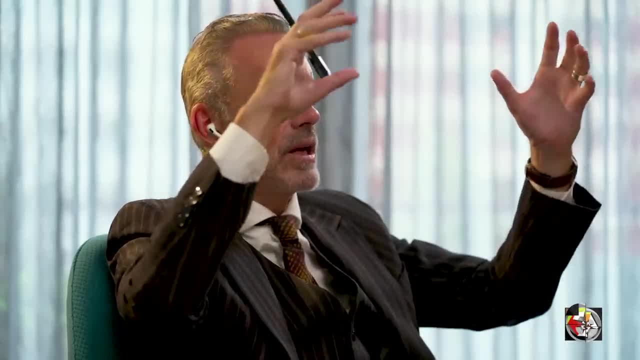 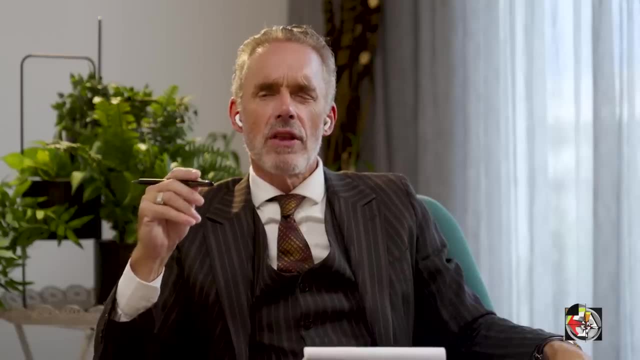 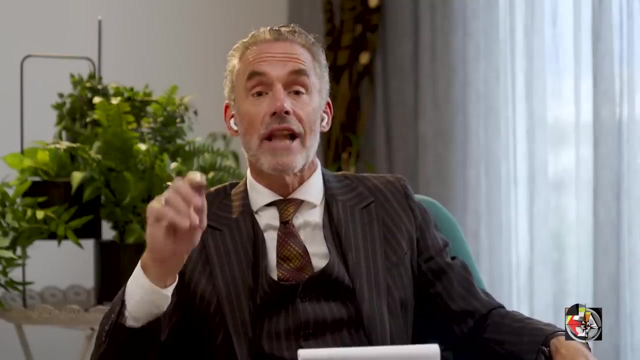 report in psychedelic experiences that ideas flood in on them and they see how things are connected in ways they couldn't perceive before, and so that's different than the flexibility that high neuroticism in some sense produces, because that's more like the probability that a conceptual system 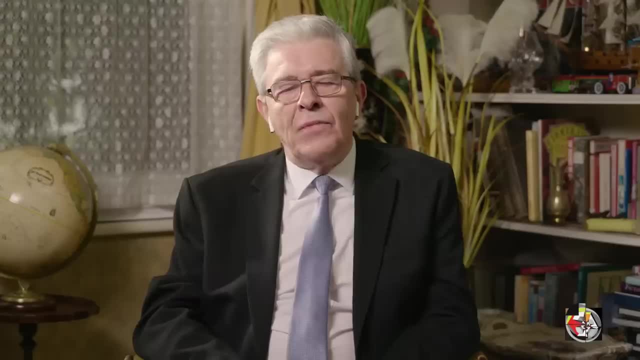 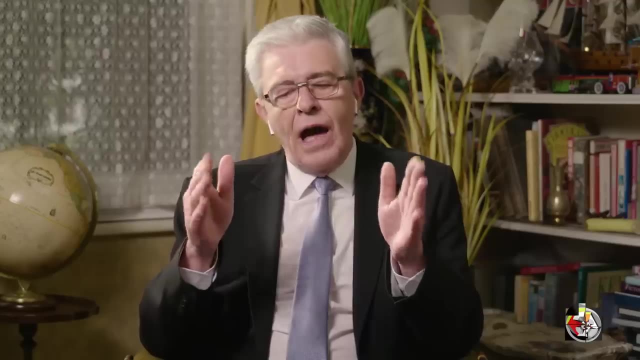 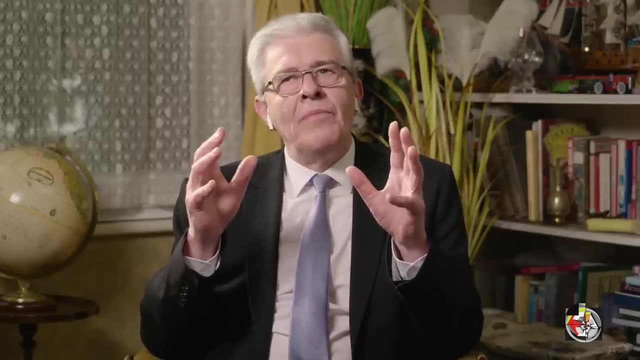 will collapse rather than it will expand. but your use of the word barriers, I think, is very nice, and I'm just wondering- and certainly I think you'd enjoy speaking to Robin Kaha Harris, who has described, I think, effectively what you've just described, but instead of 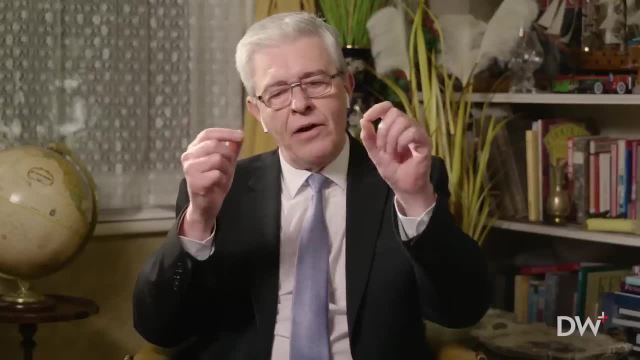 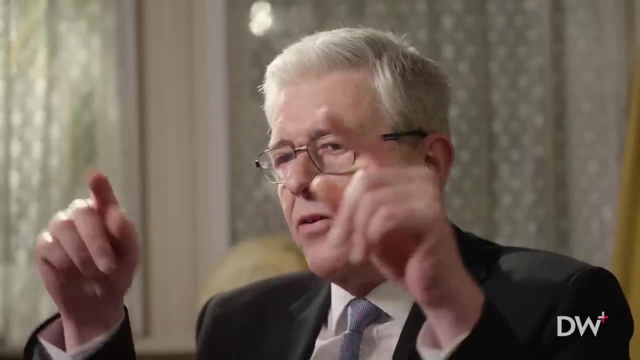 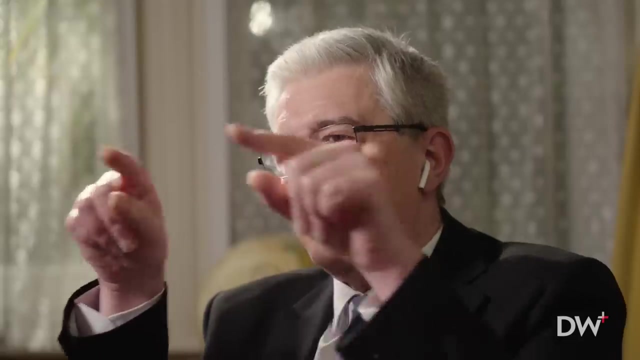 casting it in terms of jumping through barriers, he would describe it really as a reduction in the height of a barrier. so if you can imagine- and it's in my world- it would literally be a free energy landscape, and our ideas, our prior beliefs are basically sitting at the 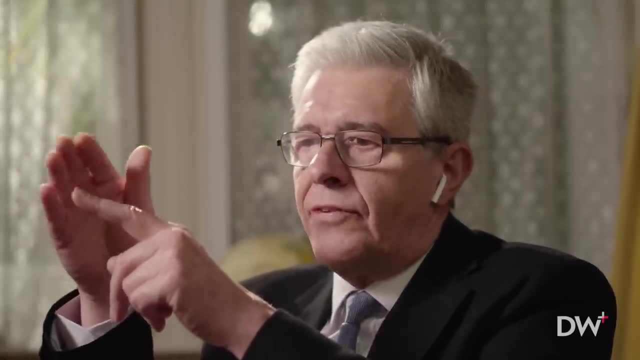 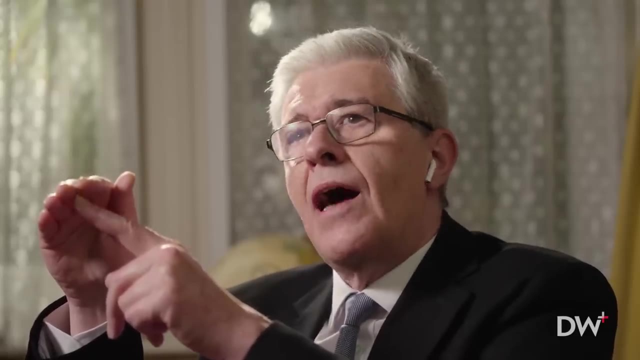 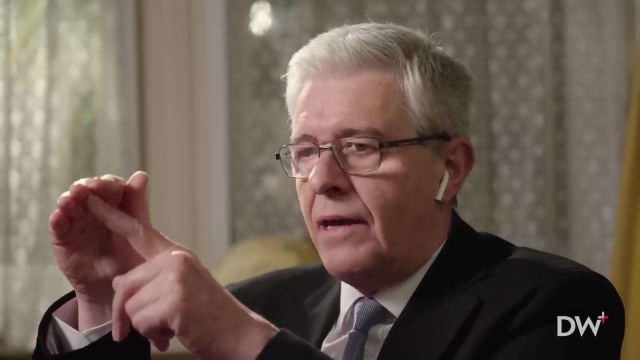 minima at the bottom of a well, and sometimes we can get stuck in a rut. I see, and you know, for example, you say I was depressed or I had the hypothesis I am going to die. and this is how things that are going to die behave, and this is how 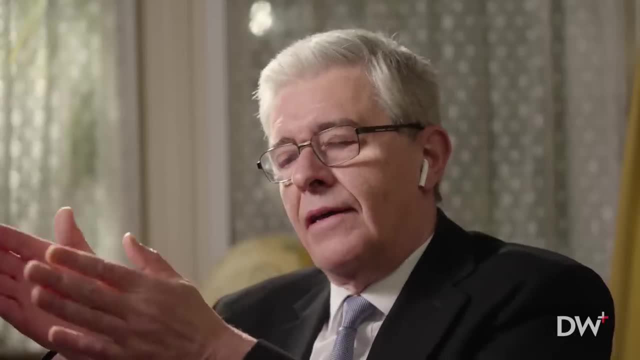 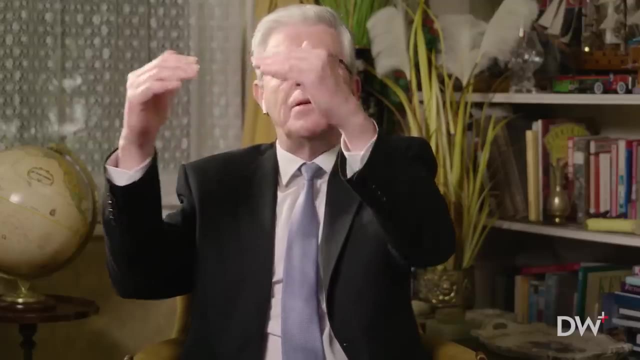 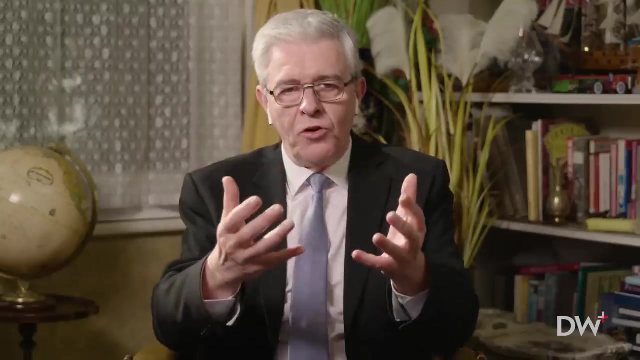 I'm going to behave and that may not be the most functional way of that kind of end of life, and that's what I'm talking about and I think, I think we are moving forward, and I think we are moving forward in terms of the, the, the. 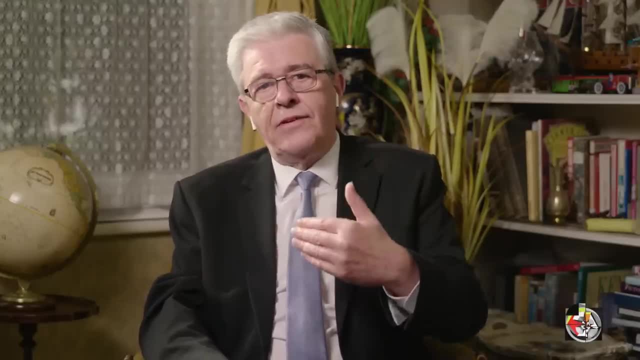 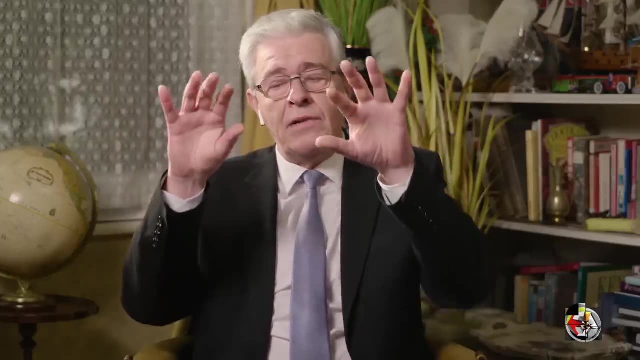 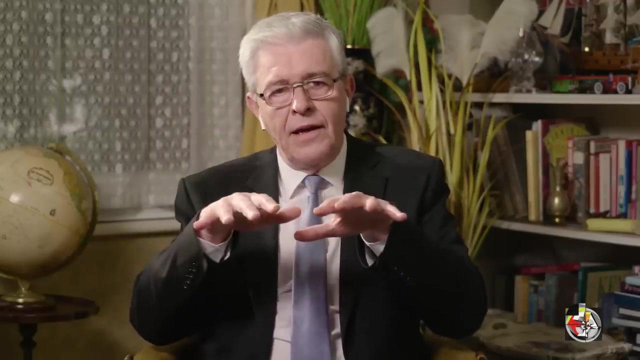 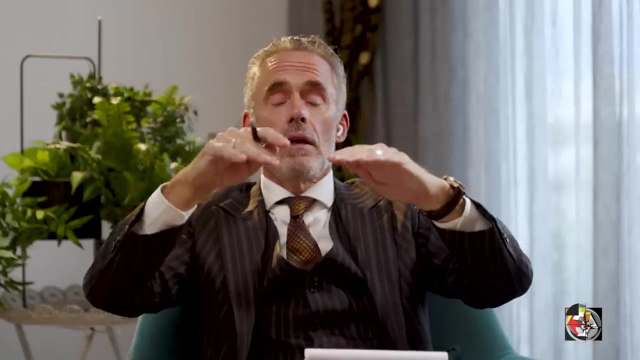 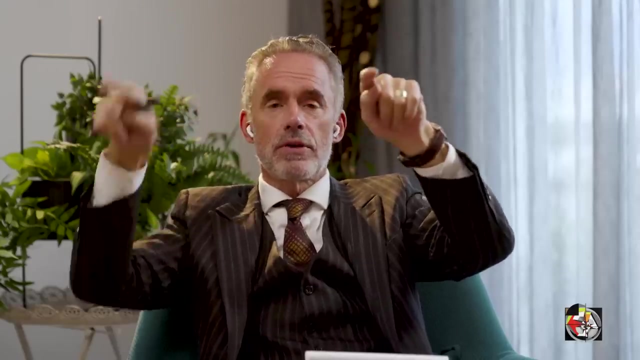 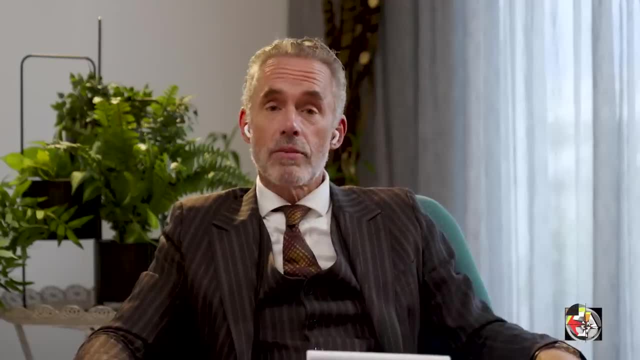 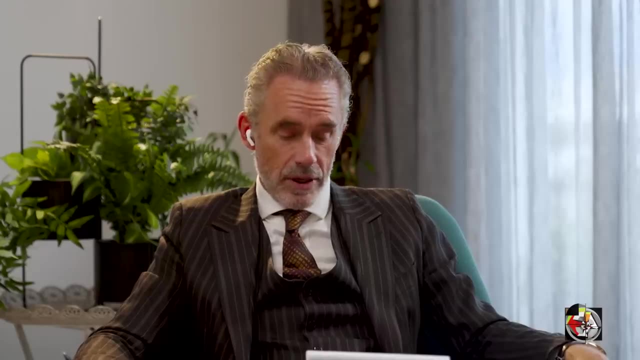 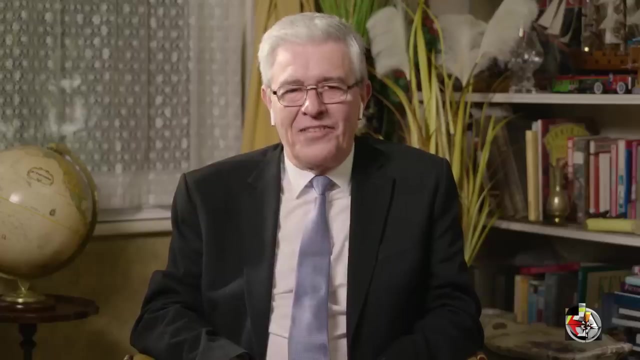 let's break the title on a また the most important thing, that ズ, but two of four points and three other topics I would love to discuss with you. I would very much appreciate it if you would consider putting me in touch with. is it Carhartt Harris? Indeed, yes, I will do that. Yes, yes. 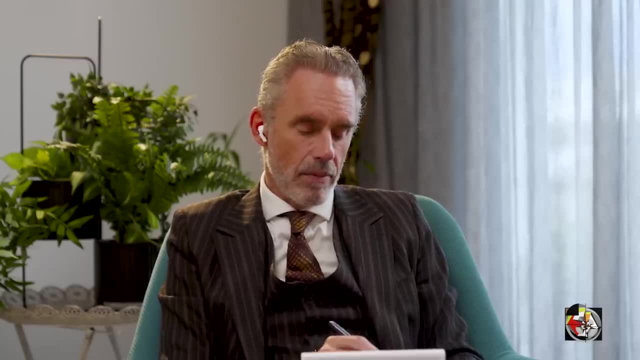 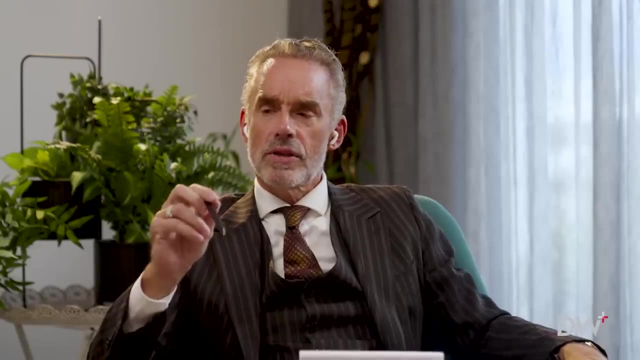 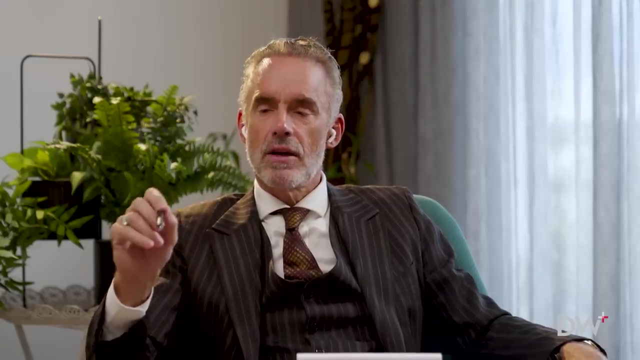 because I know some of the papers that you've written jointly and I would like to discuss those further. Maybe I close with an observation, if you don't mind, is that one of the most functional narratives, as far as I can tell, is predicated on the idea that you should conduct. 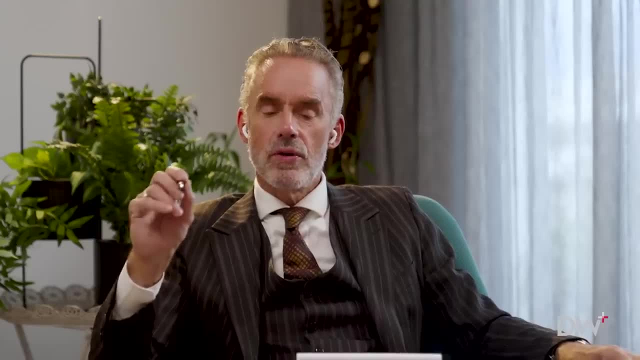 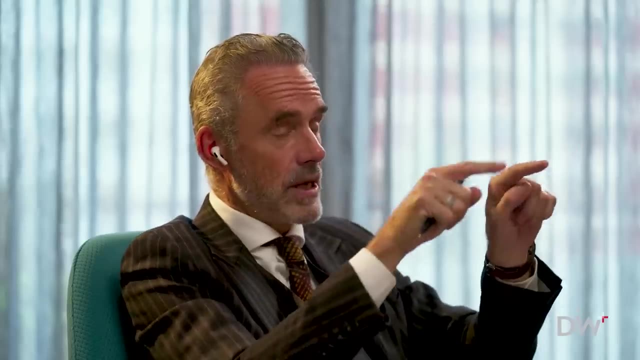 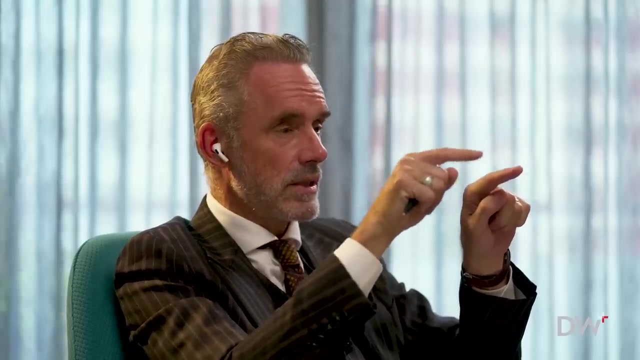 yourself in a manner that leaves you open to exposing yourself to information that will allow you to update your narratives right. So it's a weird loop, It's like. well, narrative itself is dependent on exploration, and so the best narrative, in the most fundamental sense, is: 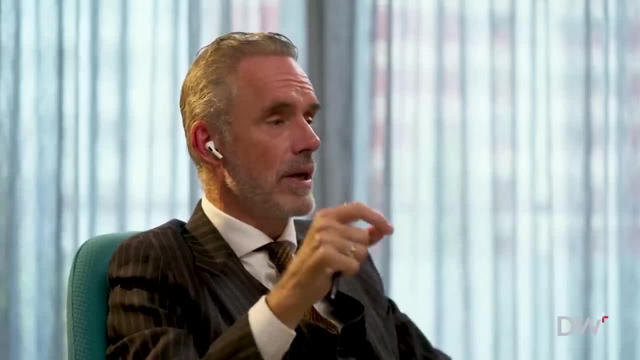 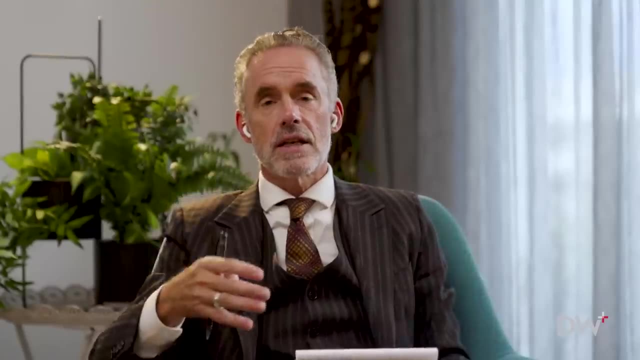 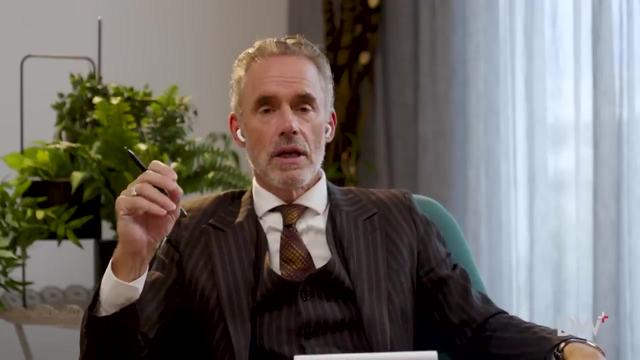 one that leaves the option of exploration continually open, and that's something like a voluntary confrontation with the anomalies that characterize existence as the central pattern of the narrative Adaptive being. It's something like that and that's existence on that border between chaos and order in some fundamental sense. So, anyways, I appreciated the conversation very much. It would 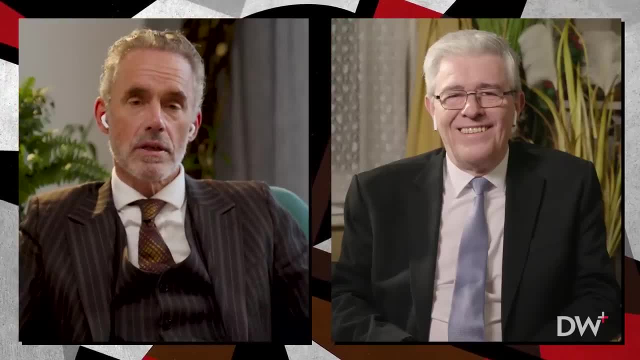 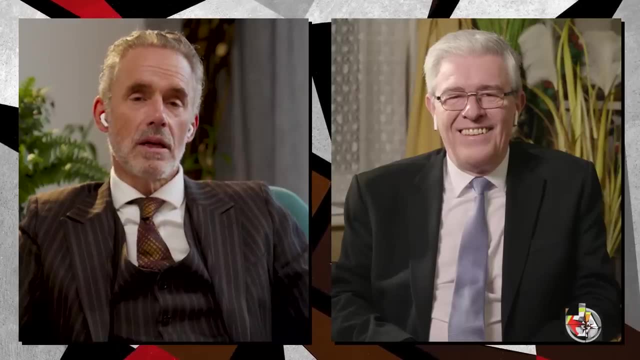 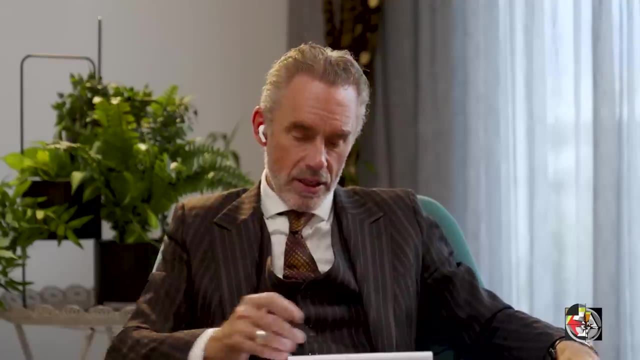 be fun to meet in person sometime. I think we could probably talk for about 36 hours, and I'll be in London again in January, and so maybe we could meet then if you'd be amenable to that. And in the meantime I would like to let everybody watching and listening know that I'm going to 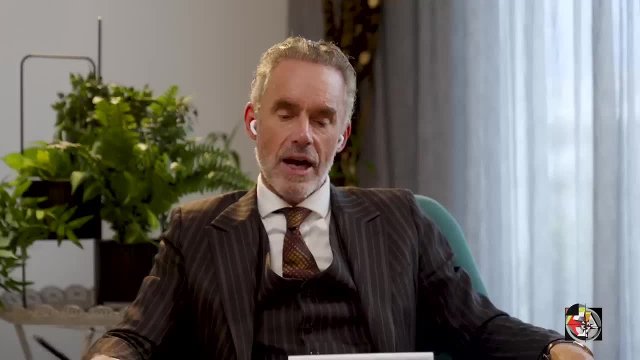 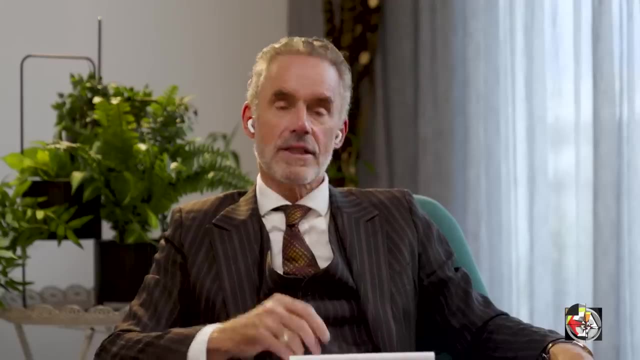 continue my conversation with Dr Friston for half an hour on the DW Plus site. I like to go behind the scenes with people and to investigate the process by which their narrative unfolded, the process by which they made their path through life their successful path through life, because